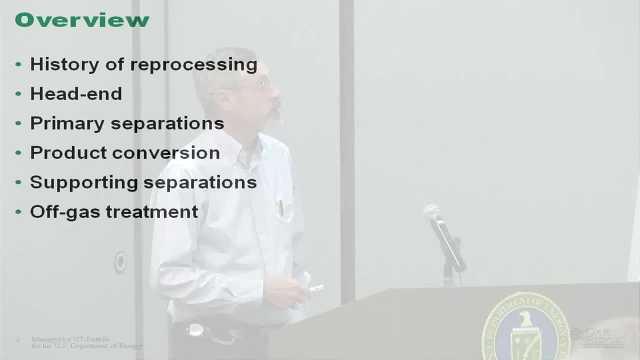 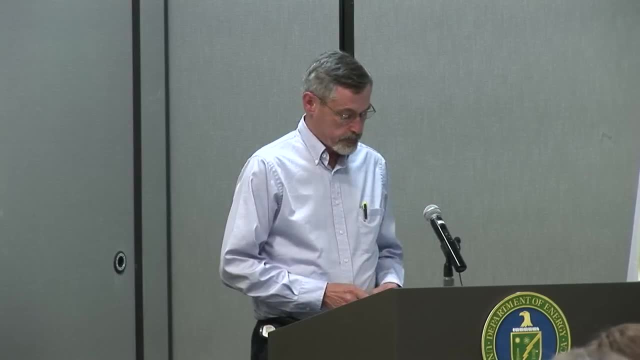 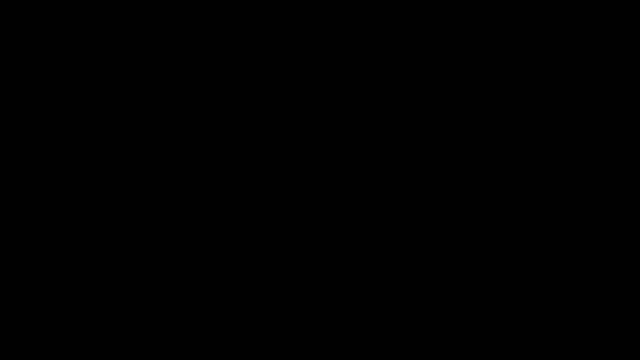 We'll begin with a brief history of reprocessing and talk primarily about commercial reprocessing. We'll talk then about the major steps of the reprocessing. We'll talk about the reprocessing facility, beginning with the head end primary separation steps that we go through the product conversion supporting operations. 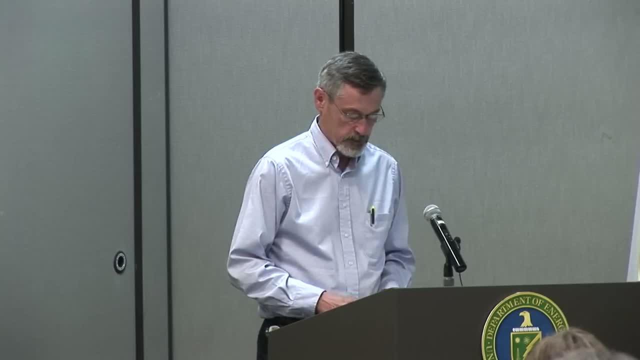 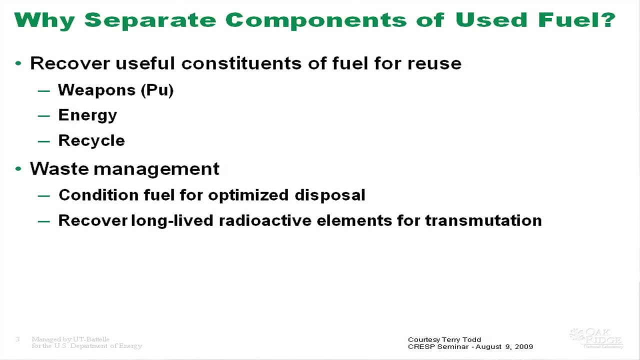 and one of those that will focus on fairly extensively, the off-gas treatment. So why would we want to separate the components of used fuel? Well, there are several reasons, First being that we, historically, the primary reason was to recover plutonium for weapons use. That's the origin of reprocessing. Second reason is because there's still energy value in the fuel, And so we'll be recycling certain components back to the reactor. We may also want to recycle some of the fission products to transmute those into shorter half-life materials. 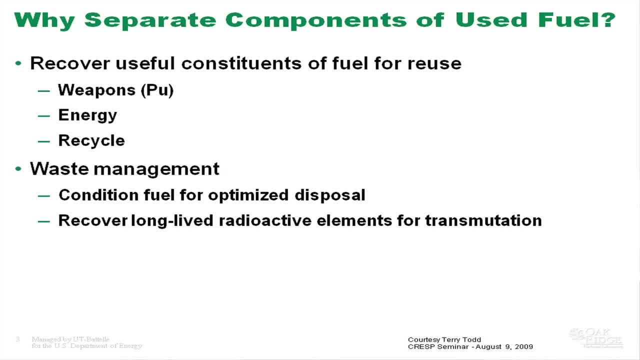 So it can also be used as a waste management tool. You might think that the fuel is a pretty suitable waste form, but we also sort of believe that in reprocessing you can produce potentially a better waste form or a waste form where of a smaller volume. 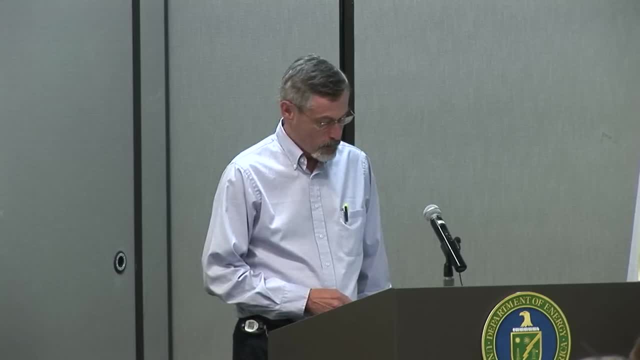 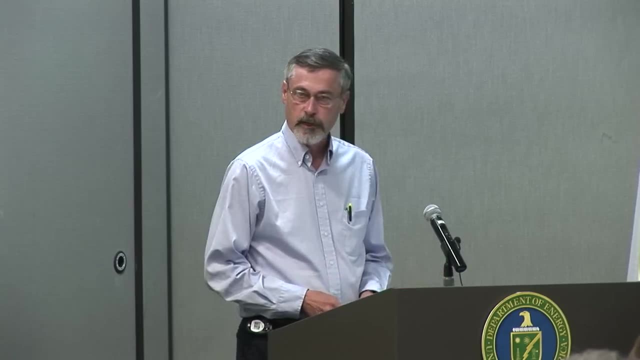 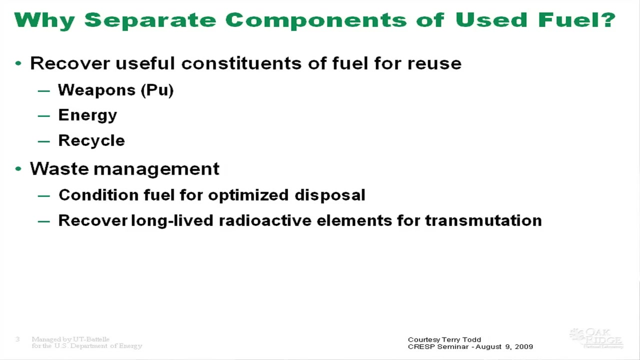 There's still some that's certainly subject to some debate And I mentioned already to recover some of the long half-life radioactive elements for transmutation, To get rid of those- and, as you saw from Alan's talk yesterday, there are some of those that have very, very long half-lives. We're talking about tens of thousands of years. 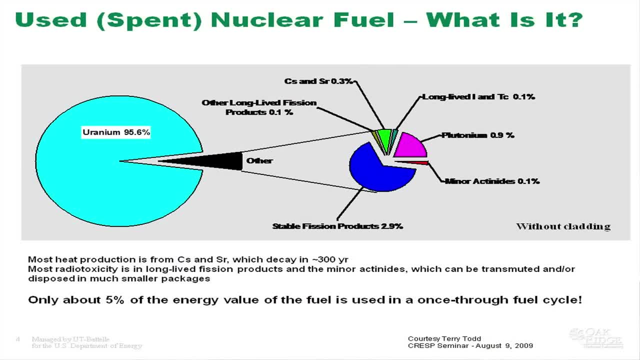 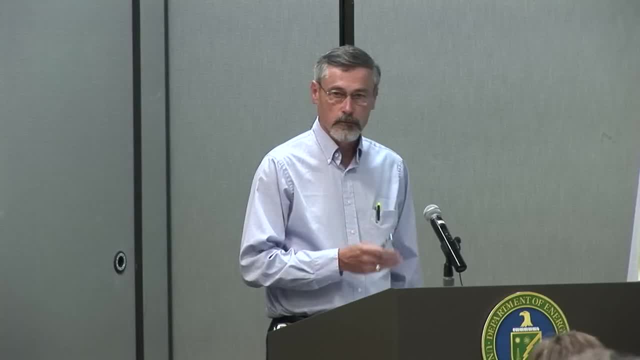 So if we look at the fuel itself coming out of the reactor and this sort of repeats- the material that Alan had- the bulk of that is still uranium. about 95 to 96 percent of the fuel coming out of the reactor is is still uranium. 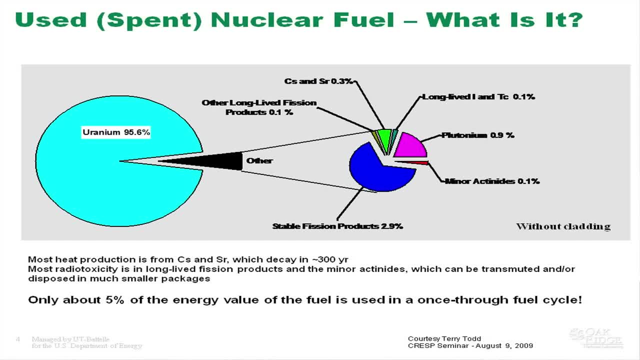 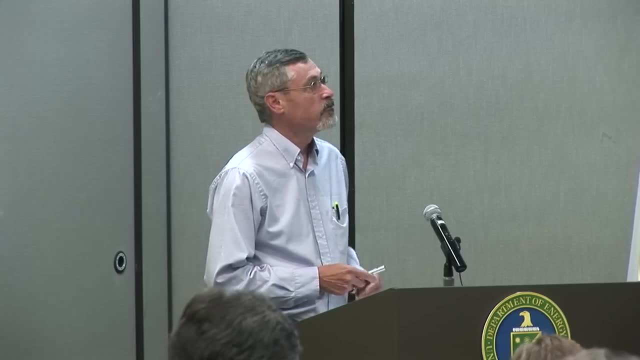 Primarily U-238.. That remaining part of the fission products- about 1%, is plutonium. You have some minor actinides. They're primarily the neptunium, the americium and the curium. You have some stable fission products. You have some of the long half-life materials: the iron, the technetium. The primary heat sources are less than a half a percent, That's the cesium and strontium, And then you have a few other long half-life fission products. Well, the history goes back to the Manhattan Project, and the goal was to recover plutonium 238, or 239.. 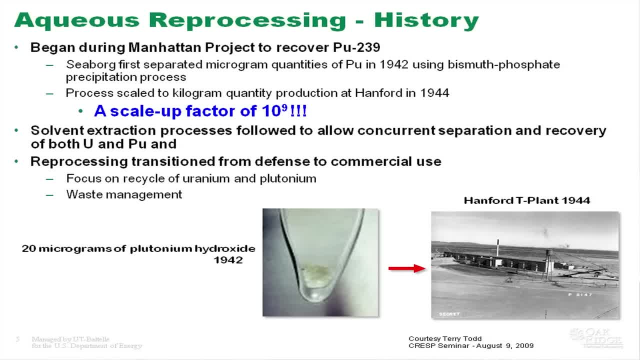 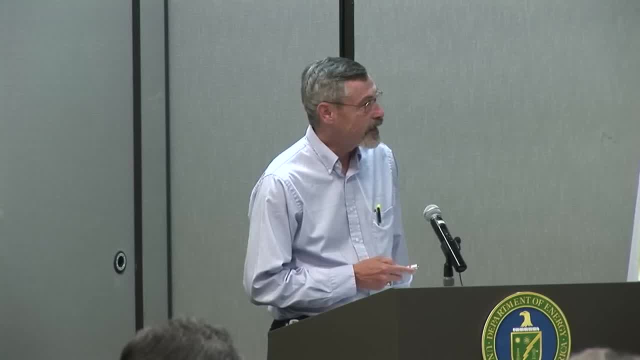 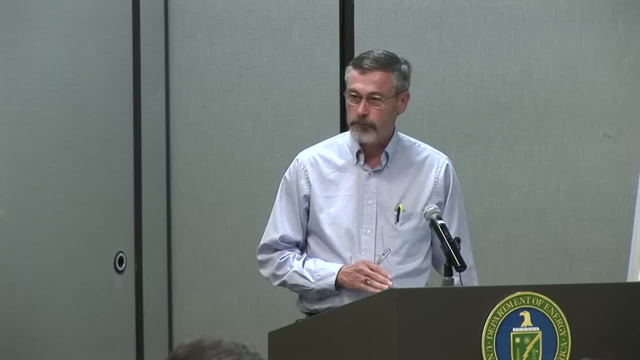 Len Seaborg separated the first microgram quantities using a bismuth phosphate process in 1942.. That's the first 20 milligrams. Two years later that process was scaled up to produce kilogram quantities at Hanford Two years. 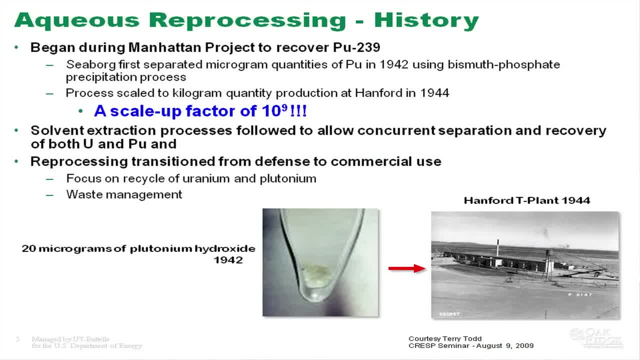 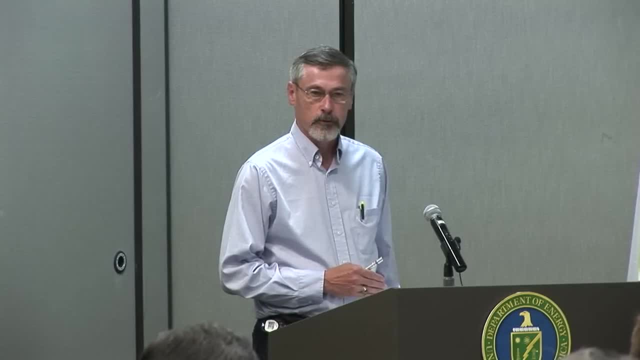 That's a scale-up factor of 10 to the ninth. Today we can hardly write a specification for a facility in two years. So it was sort of remarkable what was done during the wartime effort to scale up these processes. Facilities built at Oak Ridge. 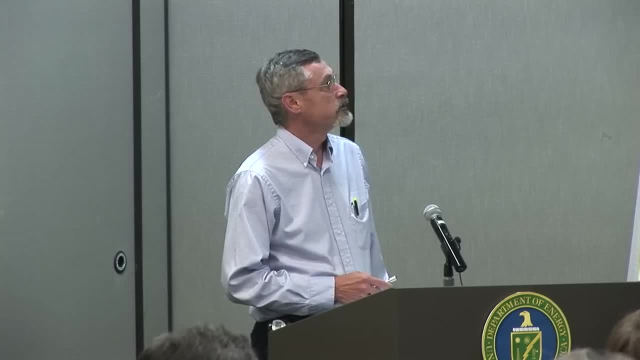 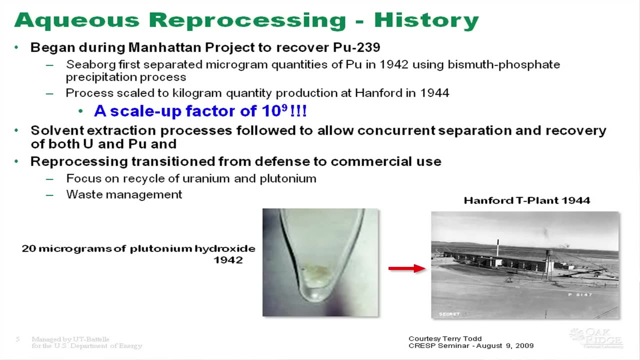 ones built at Hanford and others built at Hanford. Just phenomenal efforts, Solvent extraction followed the development of the bismuth phosphate process, and that became the workhorse of the separations for uranium and plutonium From the defense side. it was then transformed into commercial use. 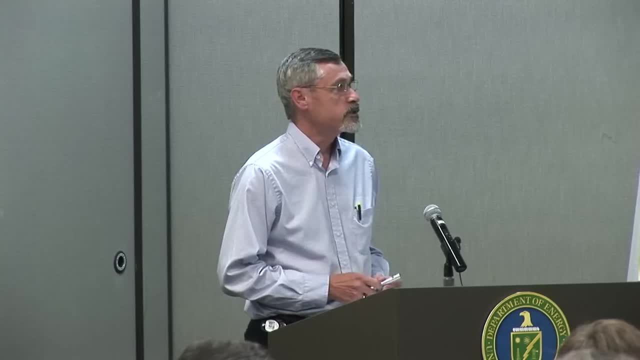 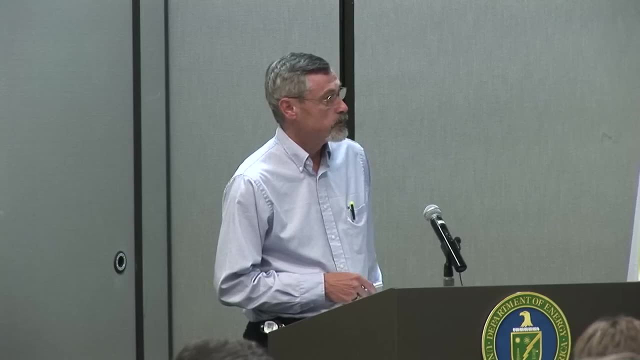 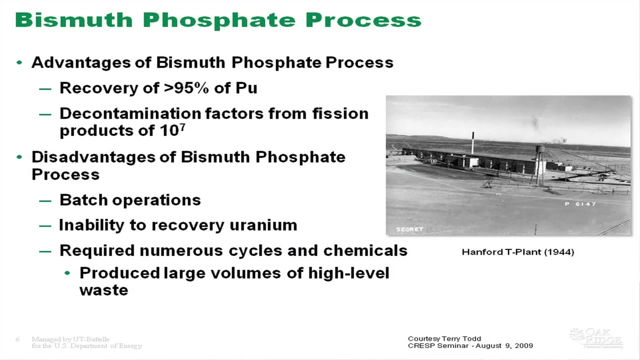 And the focus there was on the recycle of uranium as well as plutonium, And I already mentioned waste management. This is the tea plant at Hanford, So the first process that was used- I already mentioned- was the bismuth phosphate process. 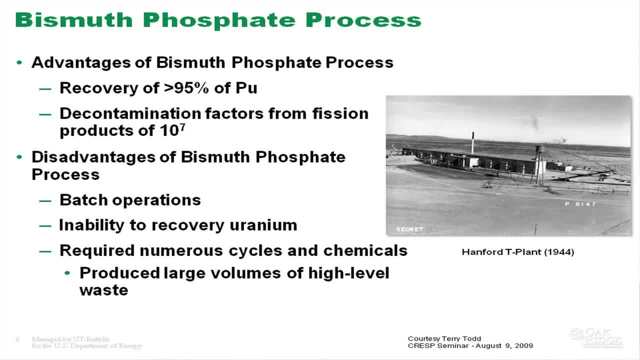 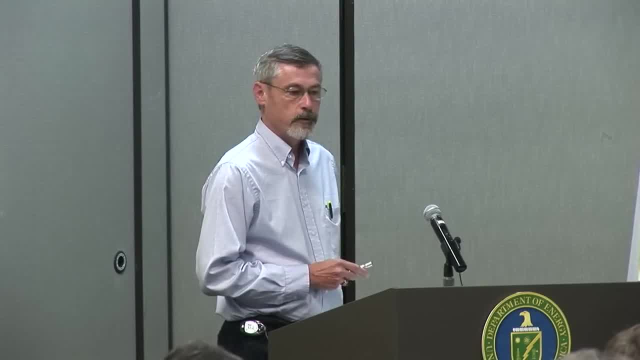 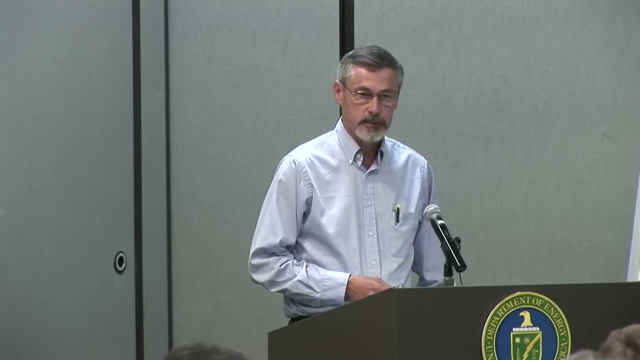 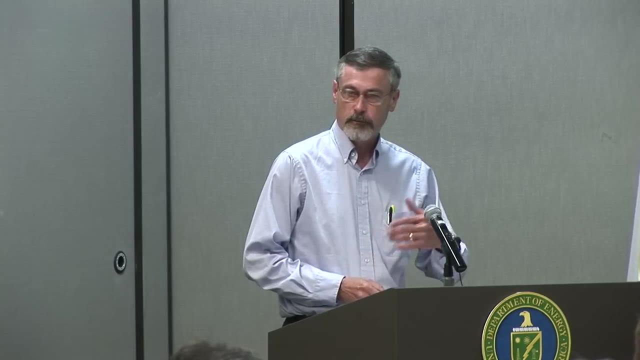 This was an extension of an analytical chemistry process where the radiochemists would try and recover very small quantities of an element from a very dilute solution. using a carrier precipitation process. They were able to get very high decontamination factors and that's the separation from the unwanted components. 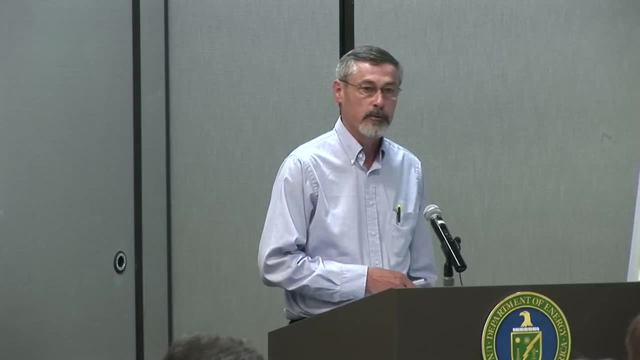 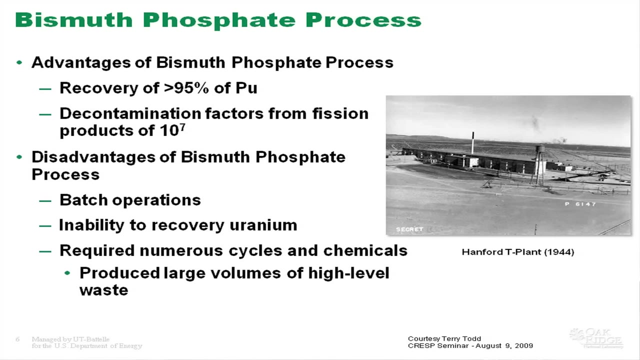 so a factor of about 10 to the seventh And at the same time recover about 95% of the plutonium. Now there are some disadvantages to the process that was developed. Certainly it was a well-understood chemistry process. 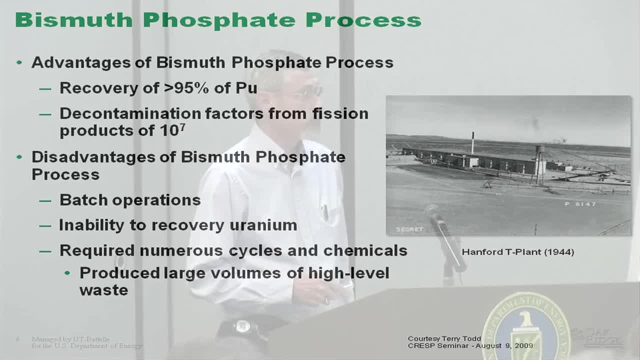 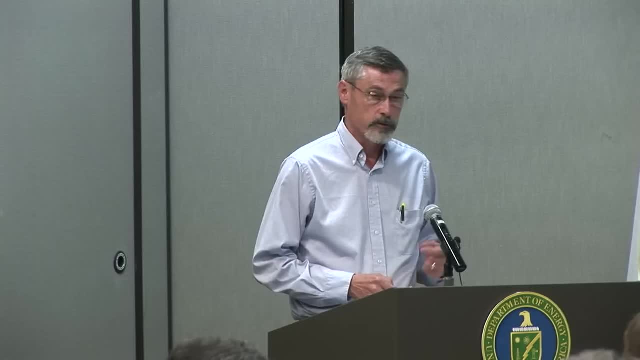 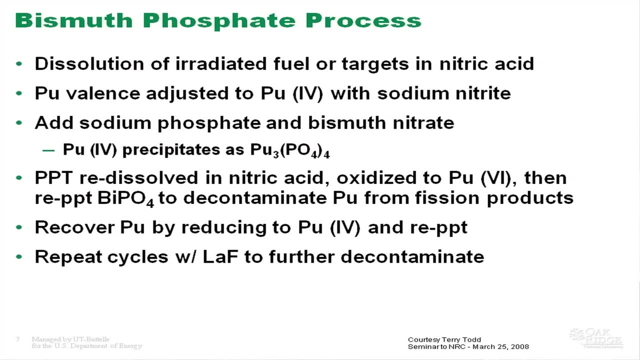 but it was a batch operation. It didn't recover any of the uranium and it had a great number of cycles and chemicals that were added and produced a very large quantity of waste. The process itself begins with the dissolution of the material in nitric acid. 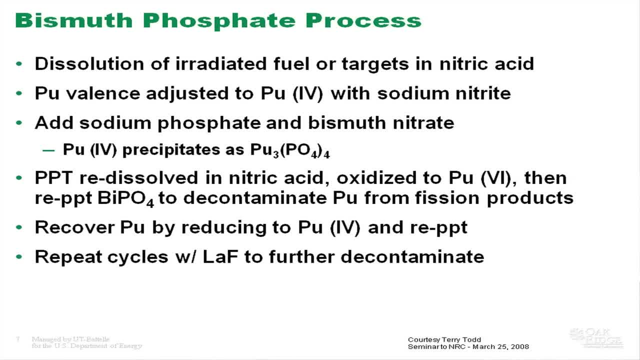 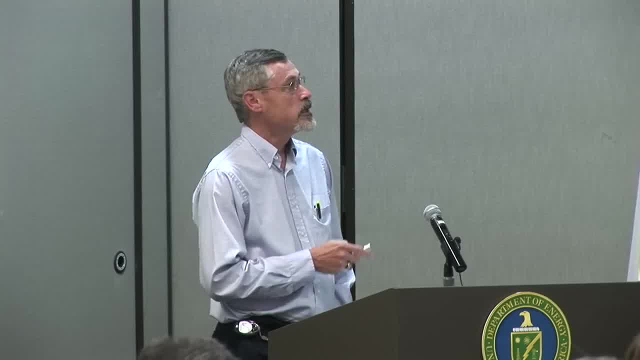 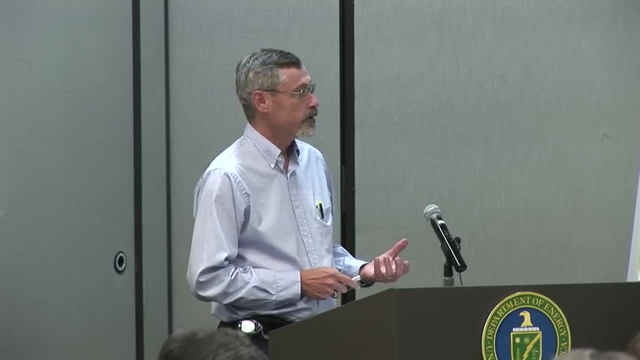 You then adjust the valence of the plutonium to four. with sodium nitrate You add sodium phosphate and bismuth nitrate to precipitate the plutonium with the bismuth phosphate. Then you re-dissolve, that precipitate, You oxidize at the six-valence state. 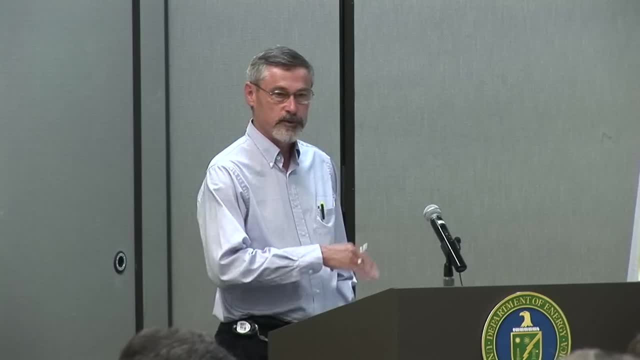 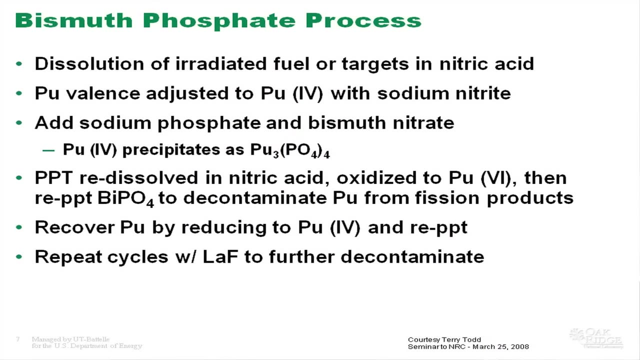 You re-precipitate with bismuth phosphate to remove the fission products that were carried over with the precipitate. to begin with, You reduce the plutonium, You re-precipitate, You repeat that process several more times And finally you do a final precipitation with lanthanum fluoride. 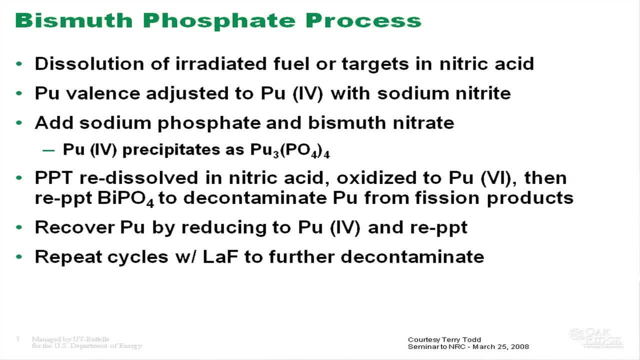 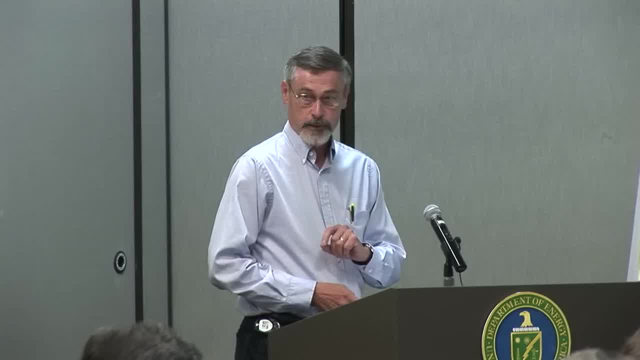 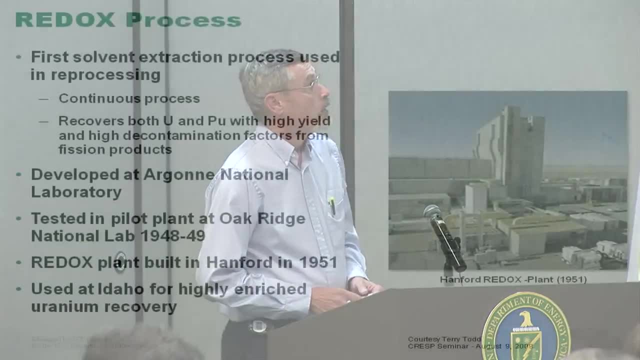 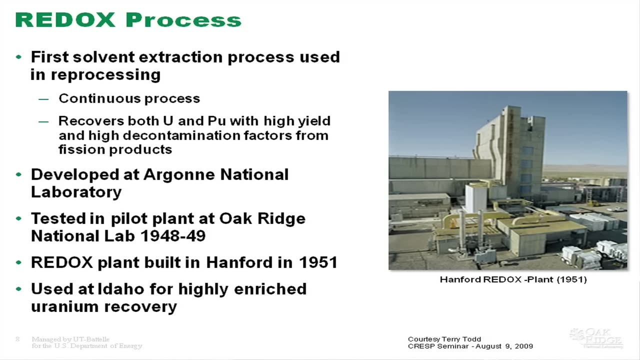 lanthanum fluoride to decontaminate from additional fission products that were carried over by the first three precipitation processes. Remember, this is all batch but they scaled it up to produce kilogram quantities of plutonium. Well, the first then solvent extraction process was the redox process. It was a continuous process. That's a big advantage. It recovered both the uranium and plutonium with high yield. It was developed at Argonne National Laboratory, tested at Oak Ridge in 48 and 49, and the first plant was built at Hanford in 51.. 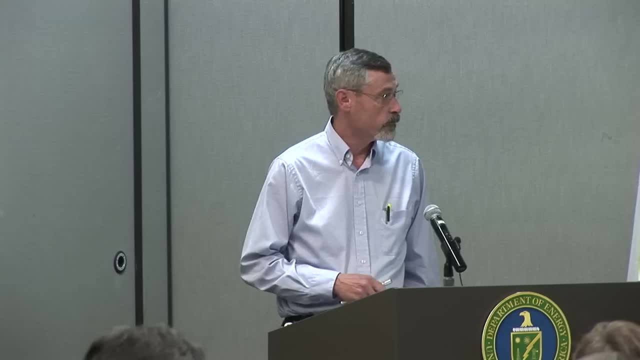 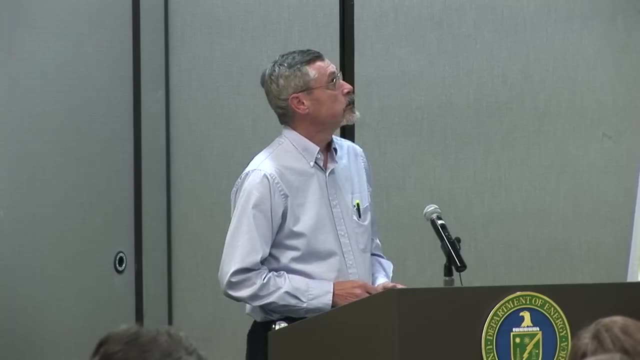 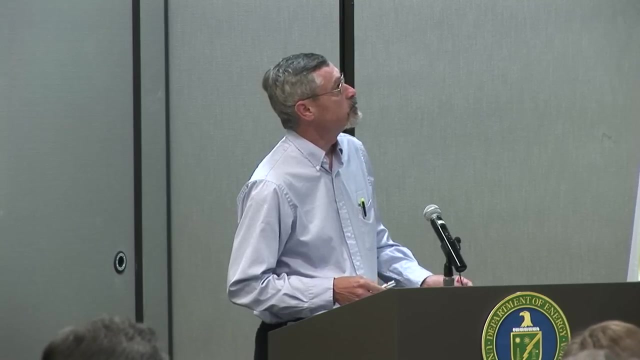 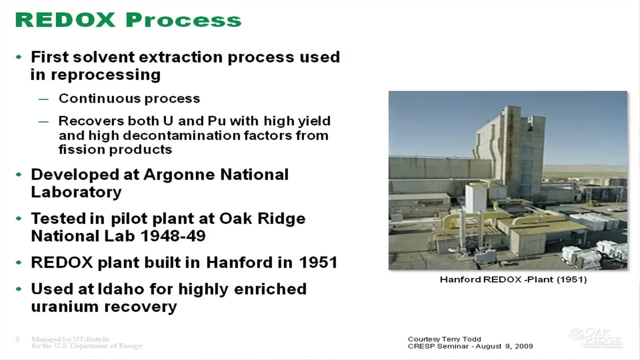 It was later used at Idaho for the recovery of highly-riched uranium. The redox process used hexone as the extractant. The advantage in all solvent extractions is the extractant has to be immiscible with the aqueous phase, so you have the ability to separate the two phases. 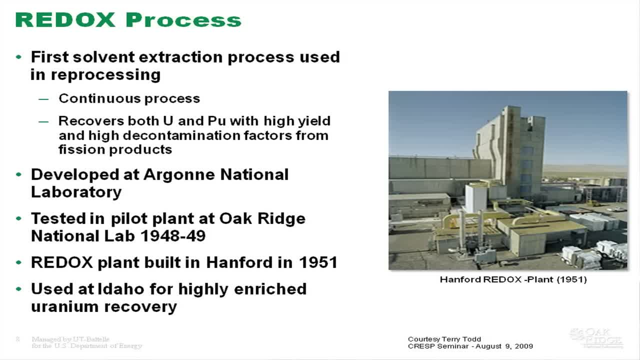 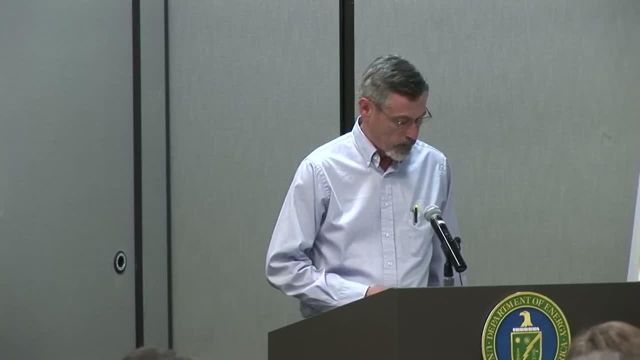 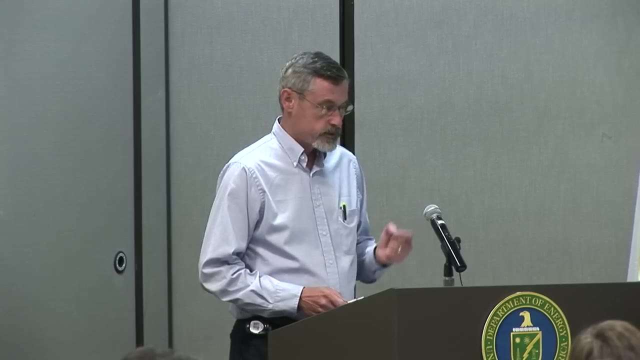 The plutonium is again oxidized to four for the highest recovery, and this is done by the addition of aluminum nitrate, another chemical that's added but results in a large quantity of this aluminum waste. The other downside of that is that the hexone is highly flammable. So you've got a large volume of waste, you've got a highly flammable solvent, and so it wasn't used. It was used for a great many years, and later another process was developed called- let's back up one- the Butex process. 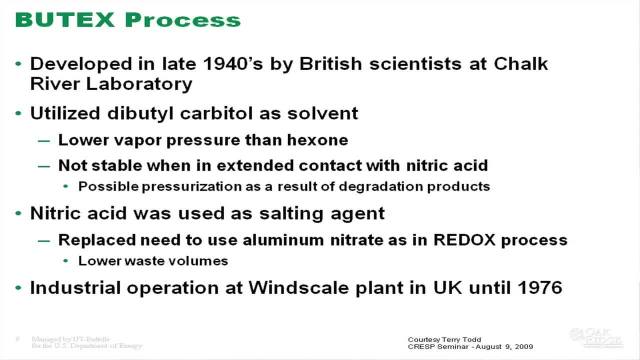 That was developed in the late 40s by some British scientists working in Canada at the Chalk River Laboratory. This used dibutylcarbotyl as the solvent has a lower vapor pressure than hexone. that's a plus, but it's not necessarily stable when in extended contact with nitric acid. 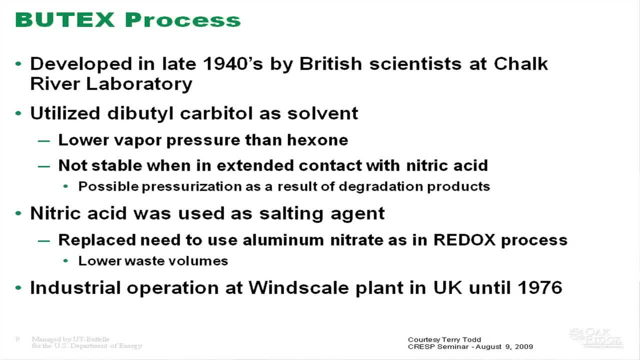 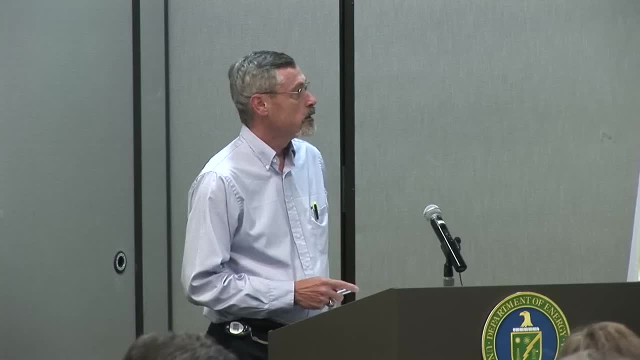 So that results in a partial possibility of a pressurization due to degradation products. Ultimately, that's what happened down here at the Windscale plant in about 1976.. Nitric acid was used as a salting agent That replaced the need for the aluminum nitrate. 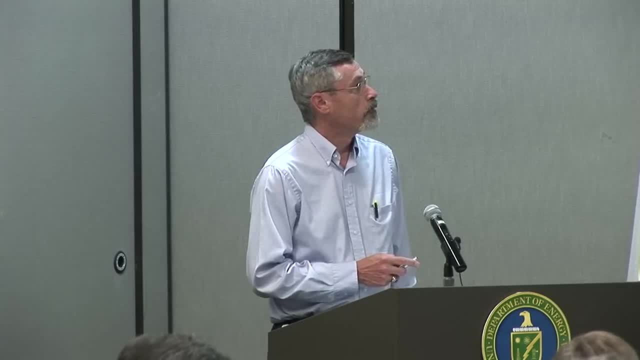 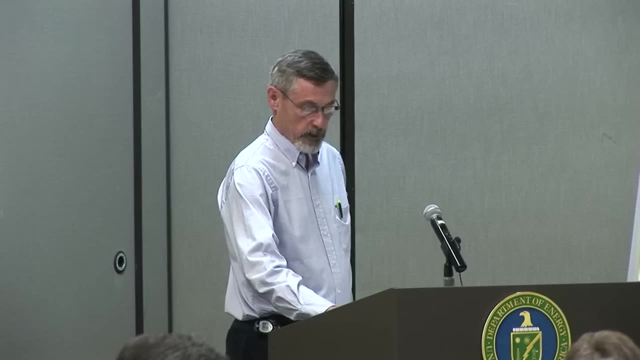 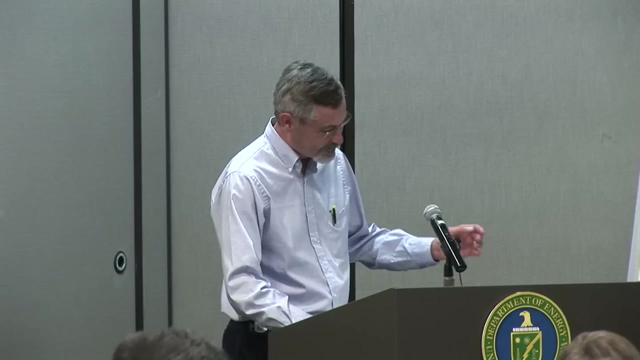 So again, there's an improvement here: lower vapor pressure and you were able to eliminate the aluminum nitrate, So you have a lower waste volume Now. thank you. The process that's probably most well known is the Purex process. 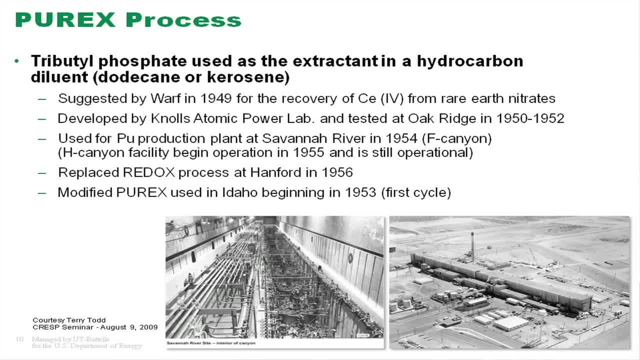 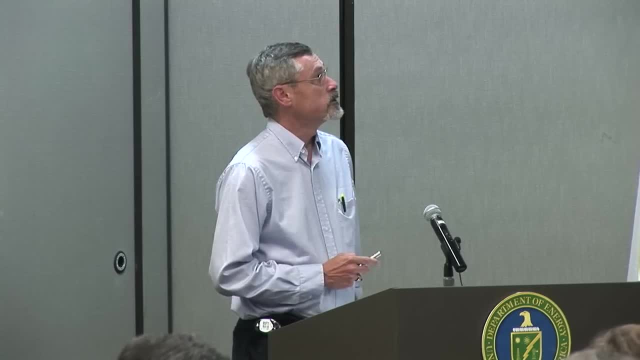 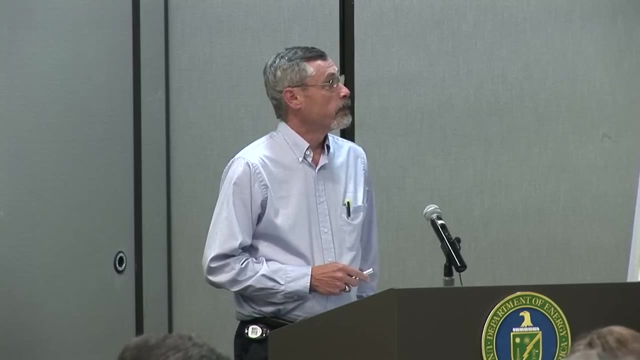 This uses tributyl phosphate as the extractant And it's put into a diluent to primarily control the density of the extract, the the organic phase, And that diluent is dodecane or kerosene. It was suggested in about 1949. 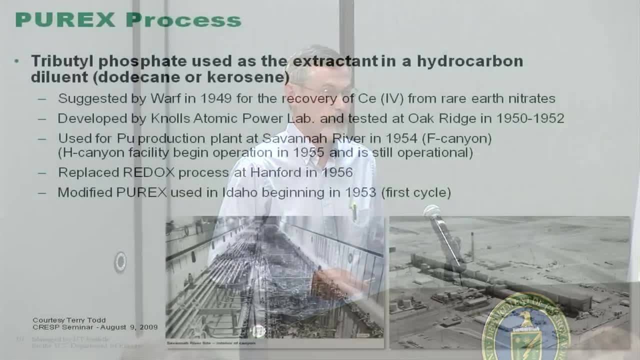 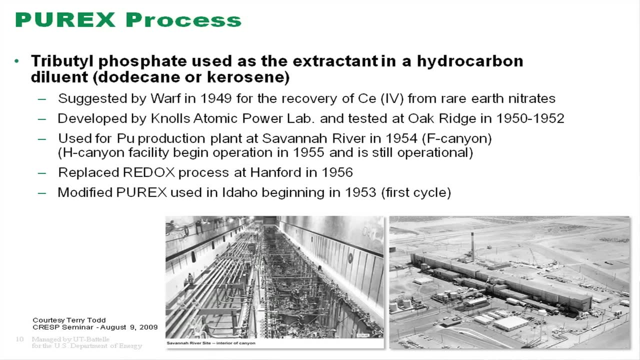 for the recovery of cerium-4 from rare earth nitrates and then extended to the recovery of uranium and plutonium. It was first developed at Knowles Laboratory and then tested at Oak Ridge. So many of these processes you can see. 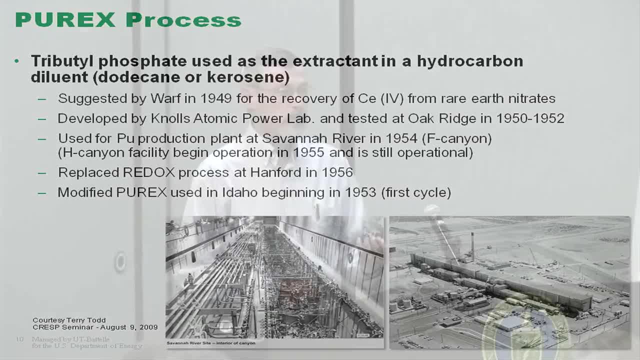 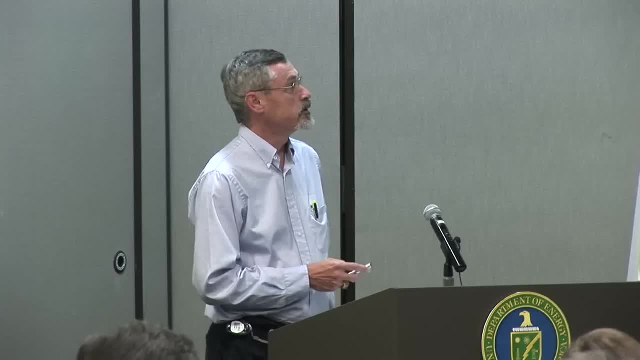 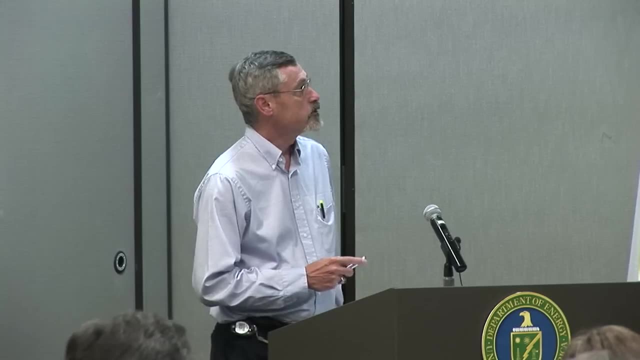 they're sort of a progression from a very small scale to some pilot plant work at Oak Ridge to later demonstrations and industrialization at the Savannah River plant, the Hanford facility and at Idaho. This replaced the redox process at Hanford in 56. 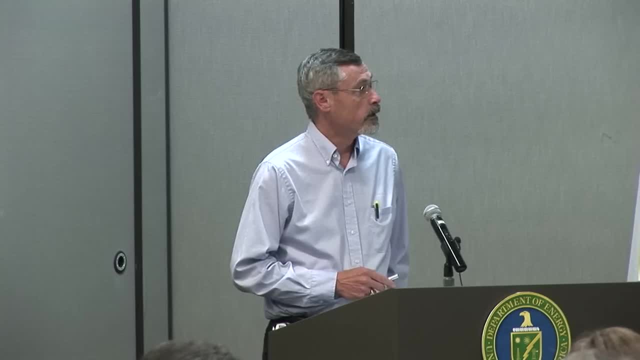 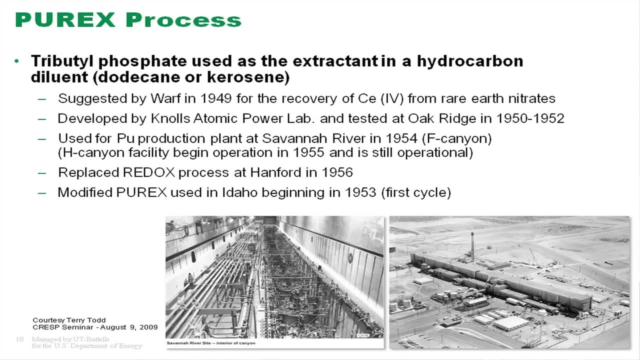 and was used as in a modified form, using a set of 30% tributyl phosphate and about 7% tributyl phosphate in the Purex process at Idaho in 53.. This is a picture of the one of the canyons at Savannah River. 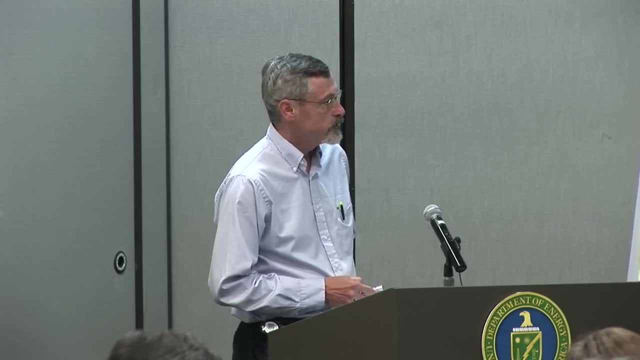 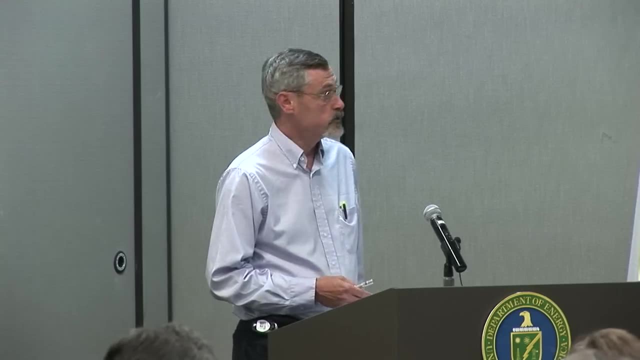 This is the Purex plant at Hanford. What you can see from here is that it's a. there's an awful lot of equipment in these canyons. A lot of piping to transfer equipment solutions from a piece of equipment to equipment. 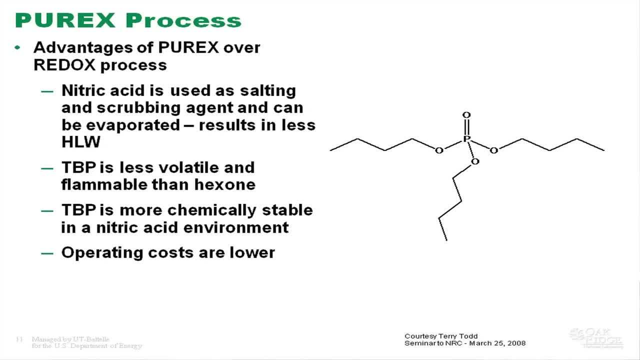 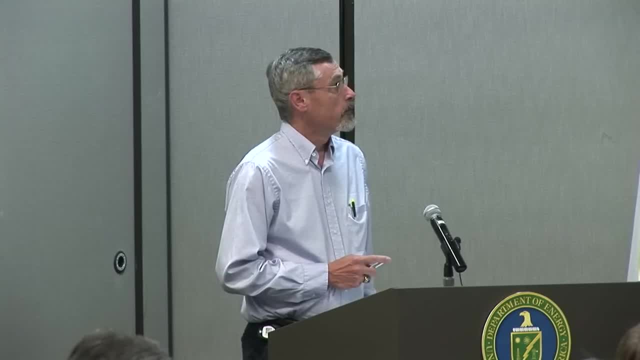 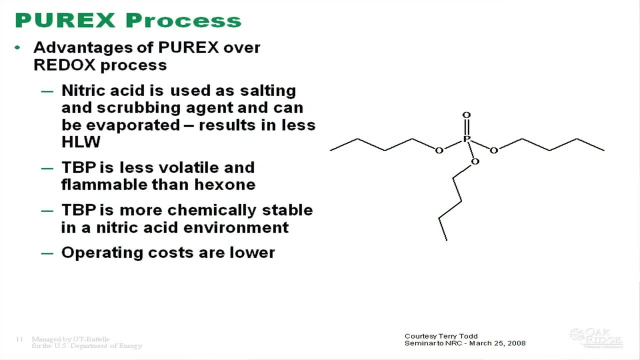 There are a number of advantages of Purex over the other processes. The nitric acid is used as a salting agent. This can be recovered and recycled, so it results in less high level waste. TBP is less volatile and less flammable than hexone. 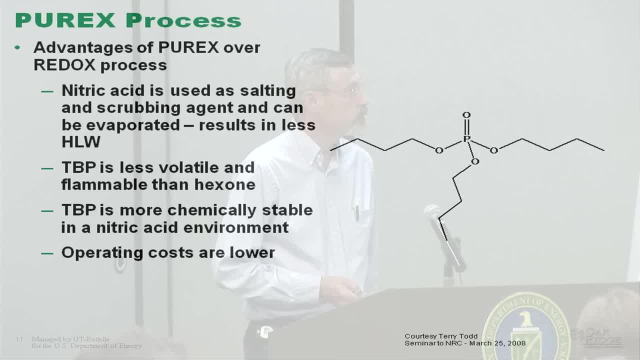 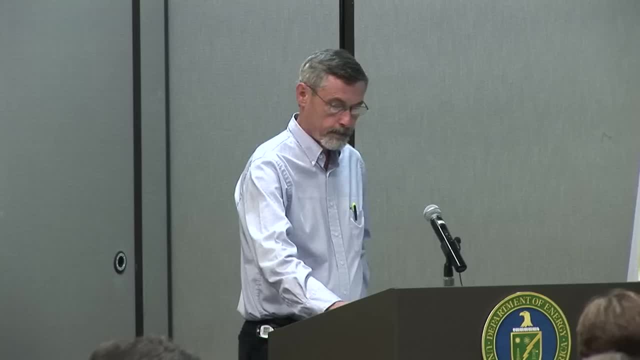 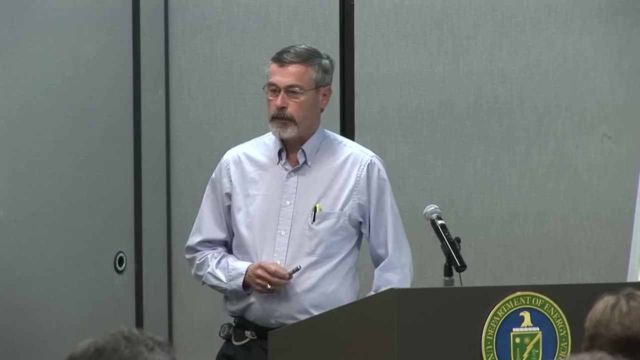 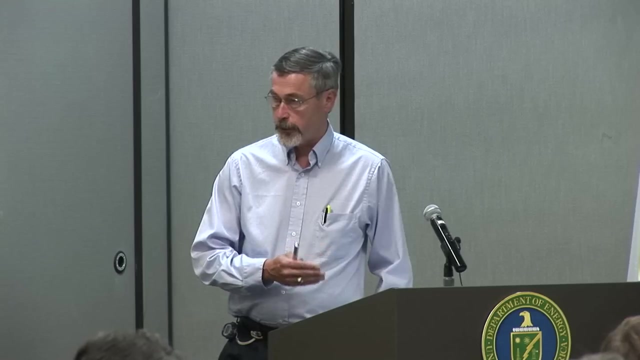 It's more chemically stable in a acid environment and thus the operating costs are lower than any of the other processes. Why are the operating costs lower? Because you are able to recycle more of your solutions. You don't have to always add and send to waste all the salting agents. The first commercial plant in the US was West Valley. It's also the only plant in the US that has ever reprocessed commercial fuel. It went into operation in 1966 and operated until 72.. Relatively small capacity in the 200 to 300 metric tons of heavy metal per year. 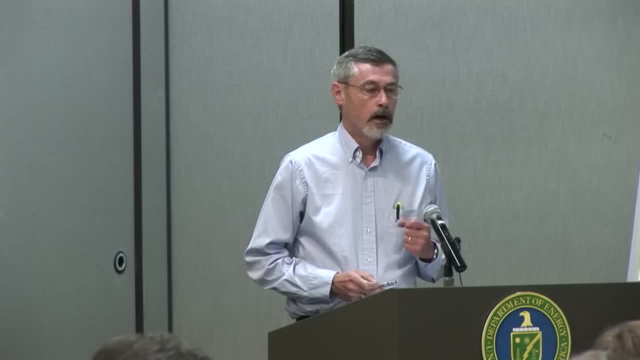 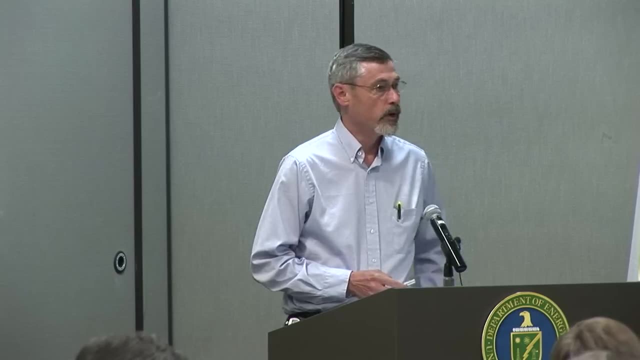 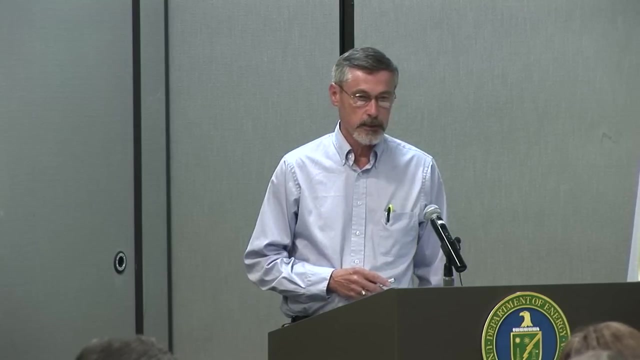 It was ultimately shut down due to some upgrades, for seismic reasons and for waste processing, And at the same time there was the construction of the Barnwell facility in South Carolina, which is a much larger facility, and it just did not seem to make economic sense. 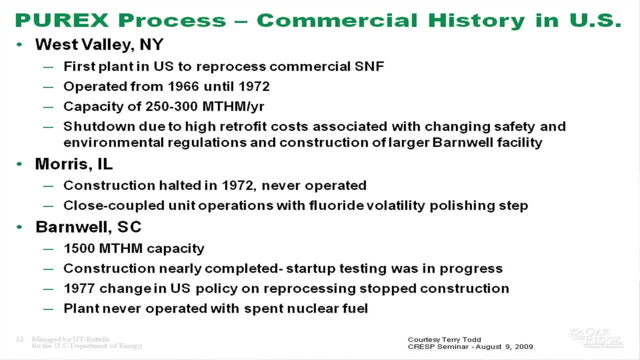 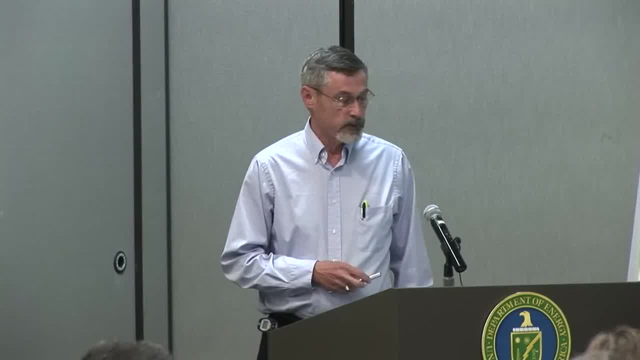 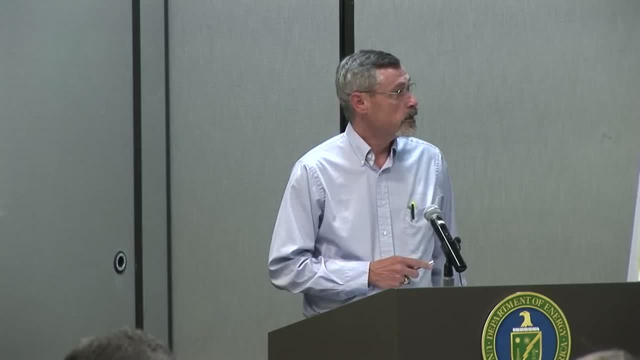 to complete the upgrades. at West Valley There was the facility at Morris, Illinois, built by General Electric. Construction was halted in 1972. It was never operated. One of the issues, as I understand that plant, was it was a very closely coupled facility. 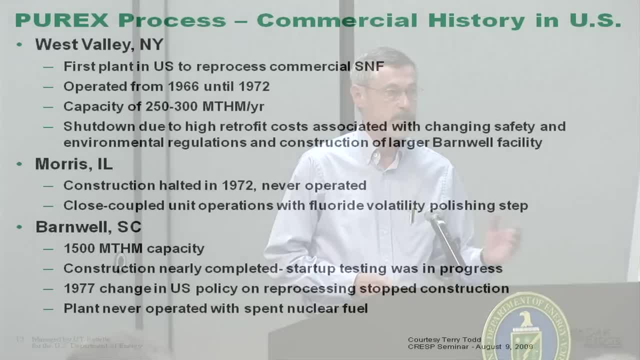 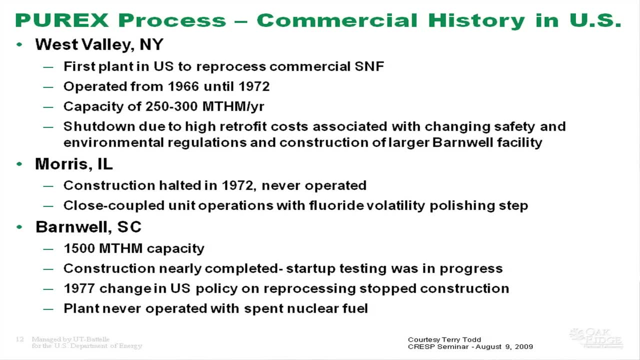 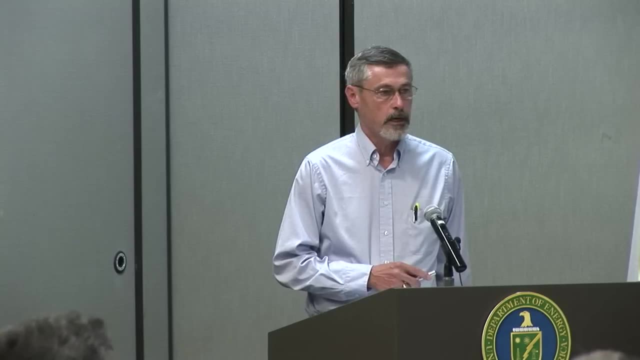 Meaning that there was very little surge capacity between the various operations in the facility. It used fluoride volatility as a polishing step to do the final cleanup of the uranium. This process fed a solid into the reaction vessel where the fluoride volatility occurred And it was at that solid transfer step. where the pipe kept plugging. So it was really a mechanical issue rather than a chemical operation issue that ultimately caused the failure of that design. The Barnwell facility was to be a 1,500 metric ton per year plant. The construction was nearly completed. and startup testing was in process when the policies of the US changed in about 1977. And for primarily proliferation concerns, the decision was made never to that we would not proceed with commercial reprocessing, And so the plant never operated with commercial spent fuel. 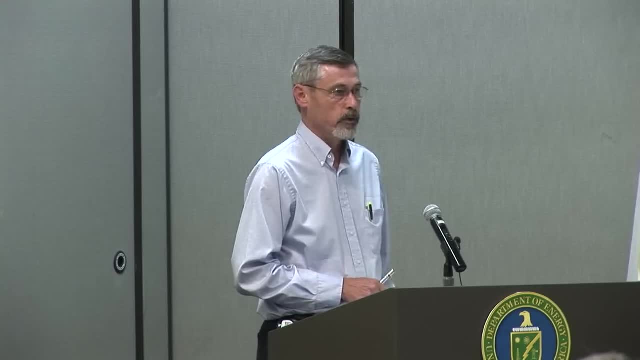 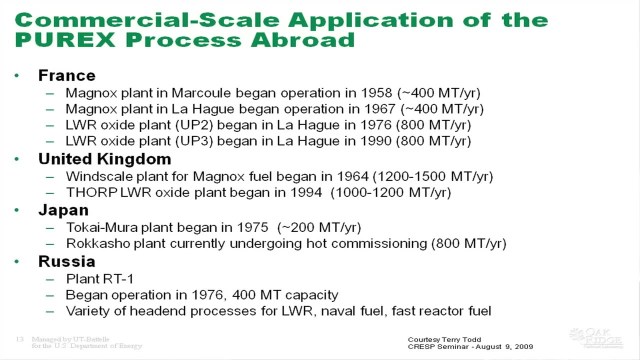 All of the testing that was done was basically culled with uranium. Throughout the world, though, the PUREX process has been used in a number of facilities. In France, they're currently operating two facilities with a combined capacity of 1,600 to 1,700 metric tons per year. 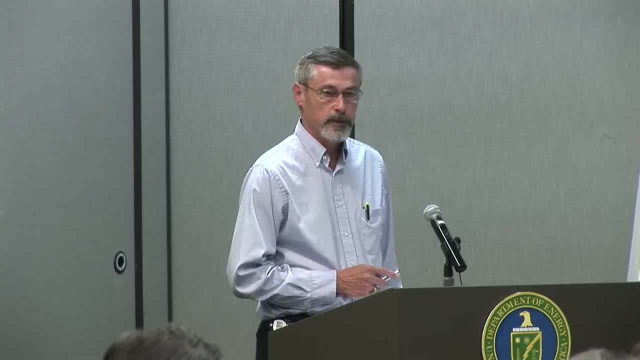 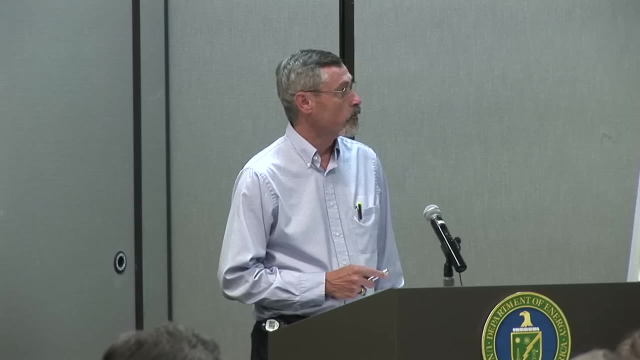 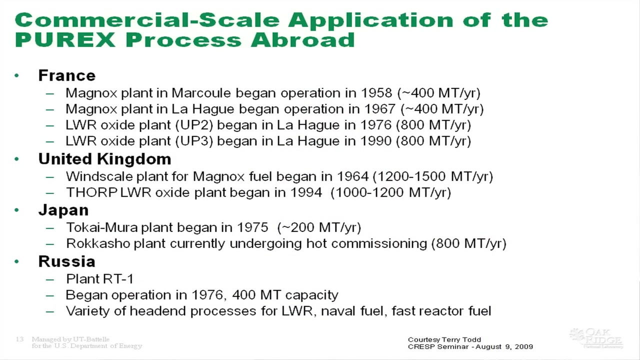 These are the UP2 and UP3 facilities. at La Hague, Windscale is currently operating the Thorpe facility, which is roughly 100 or 1,000 metric tons per year. Tokai Miura began operation in 75, and the Rikashio plant. 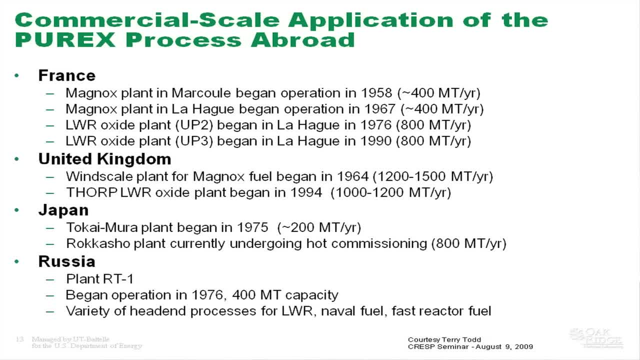 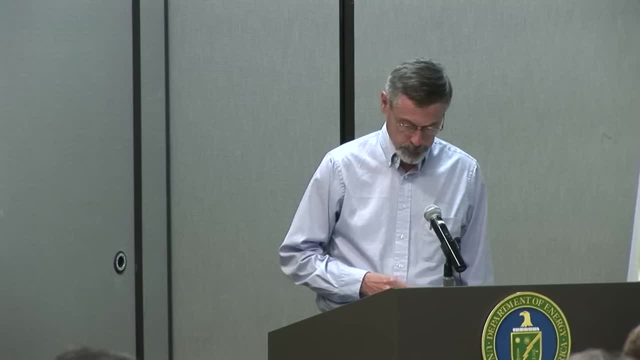 which is the Rikashio plant, which is patterned after and built by Arriva, patterned after the UP3 facility, is undergoing hot commissioning. Russia has the RT1 facility which, primarily, was built originally for defense purposes. It began operation in 76. with a 400 metric ton per year capacity. Head ends were added to handle light water fuel, naval fuel, fast reactor fuel. There was plans and work began on a RT2 facility, which was larger. That was never completed and there's now talk of an RT3 facility. 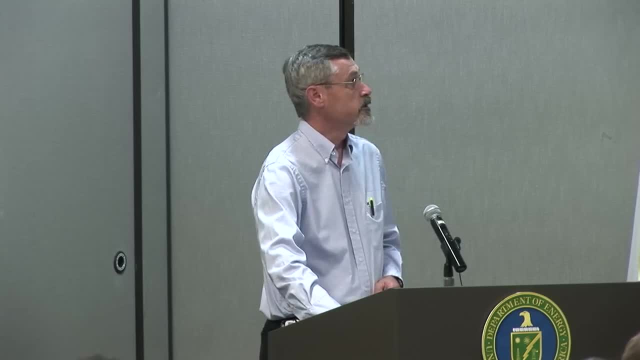 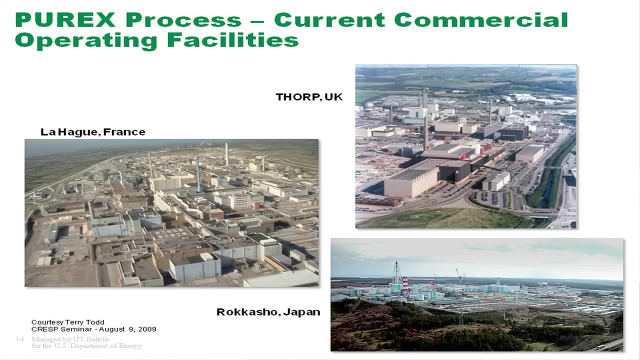 but that is still in the talking stages. These are photographs of the facilities at France. This is the La Hague facility, the Thorpe facility in UK and Rikashio. These are facilities I've drawn in to scale a human being. 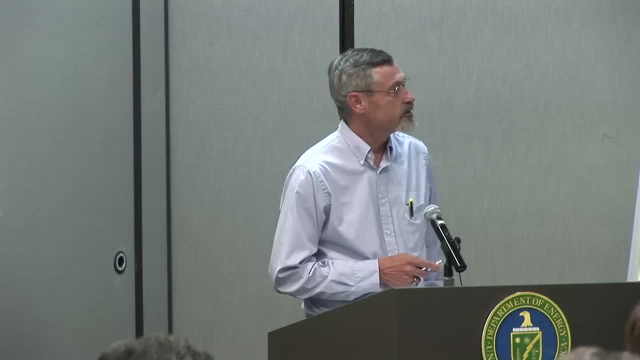 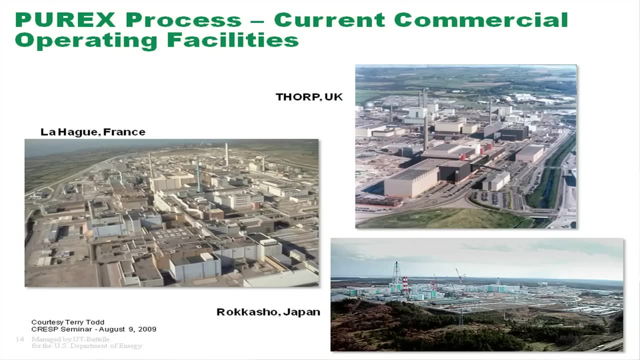 so that your job is to find Waldo in each of those three facilities. But what? just kidding on that? but they are massive facilities And you're talking about 800 tons per year. This is 1,600 tons. But think about what that means. 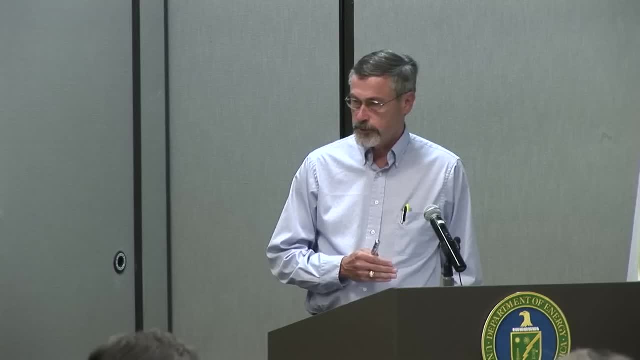 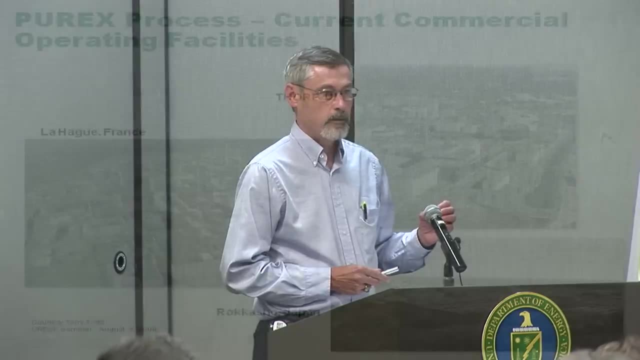 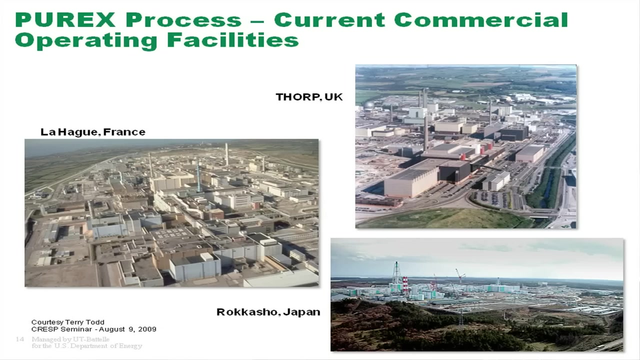 That's roughly eight fuel assemblies per day. Those aren't. That's not a huge amount of material if you're looking at those assemblies, but it takes a large infrastructure to support those operations And that goes anywhere from the head end, the receipt of material. 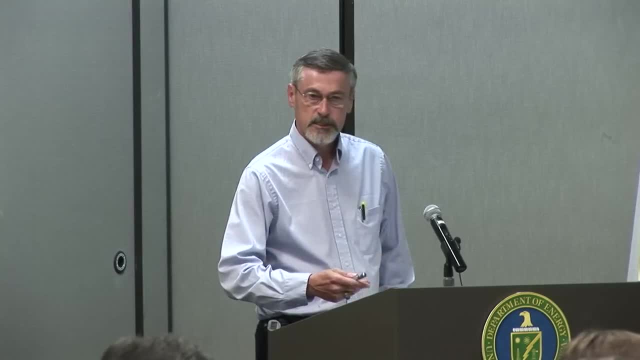 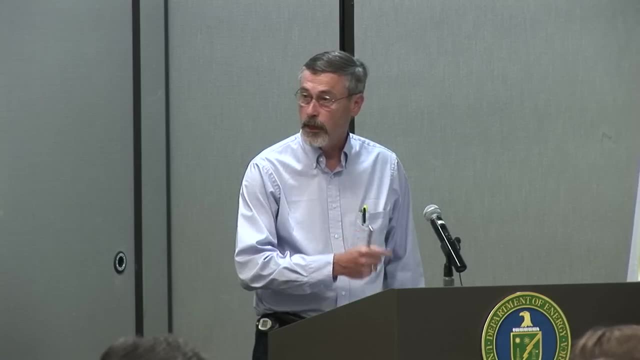 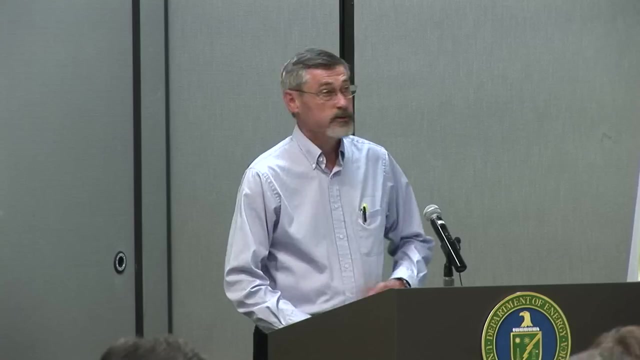 through the processing itself, the conversion back into a solid material and then the processing of the waste. So there's a lot of infrastructure that goes with fuel reprocessing And if you'd back up another slide I'm going to maybe let you handle. 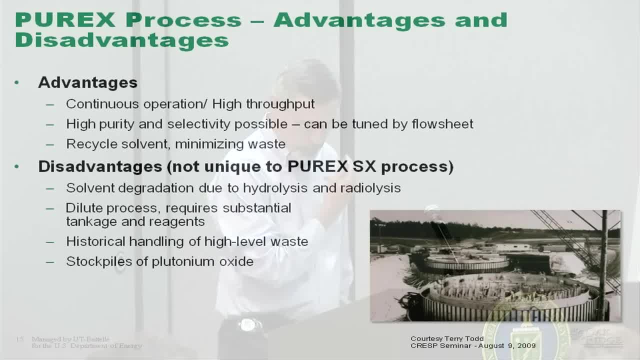 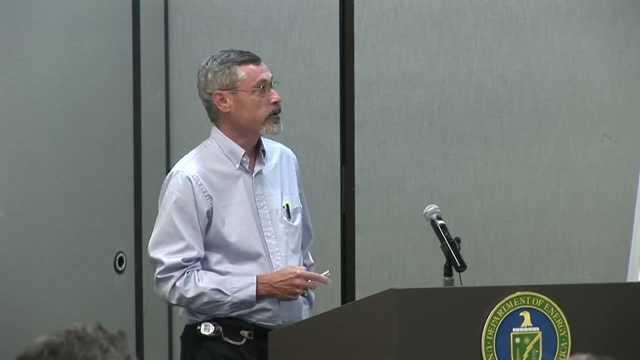 all the slide flipping. The PUREX process, as I said, has been implemented in a number of places. The advantages are certainly it's a continuous operation, very high throughput relative to some other processes. You can have high purity, very high selectivity. 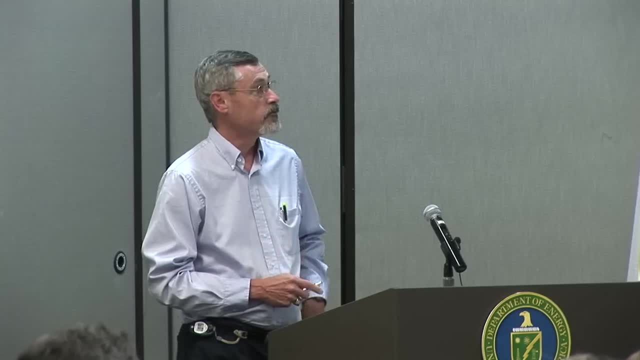 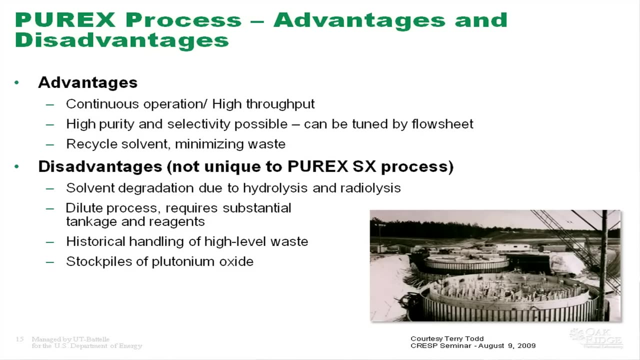 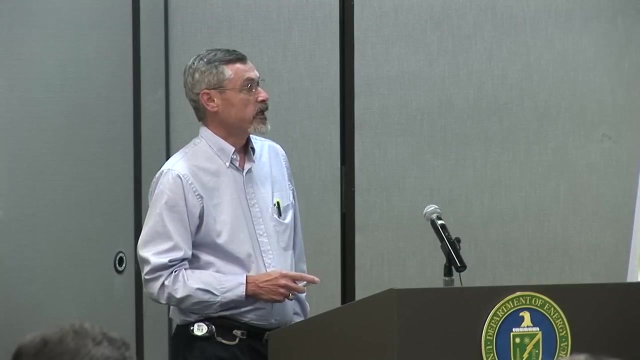 You can tune that selectivity and the purity by the flow sheet design and you can recycle the solvents, minimizing the overall waste. The disadvantages- And these disadvantages aren't limited to the PUREX process itself- Solvent degradation due to radiolysis and hydrolysis. 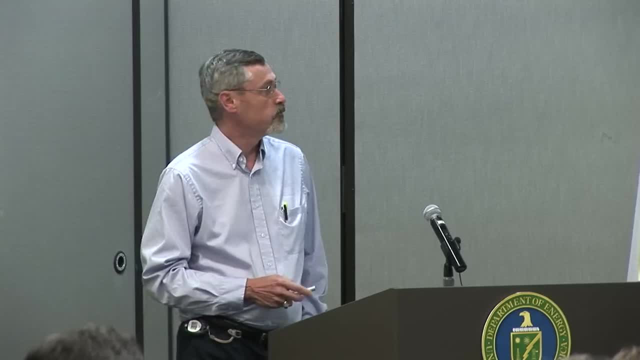 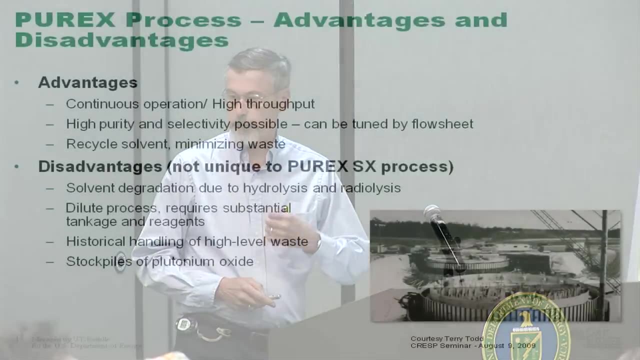 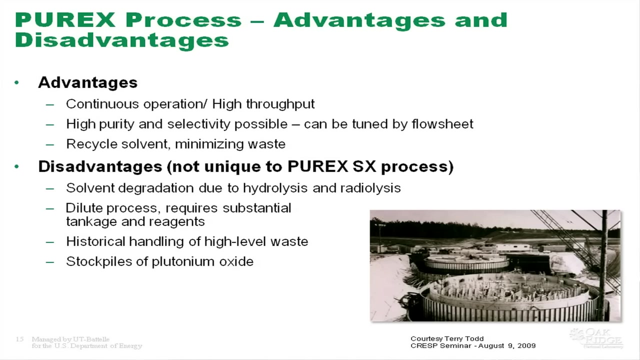 The solvent will break down into these very extreme radiation fields. It's a dilute process that requires substantial tankage. So you're talking about you dissolve material and then it's diluted down to hundreds of grams per liter, or in processes, many times far less than that. 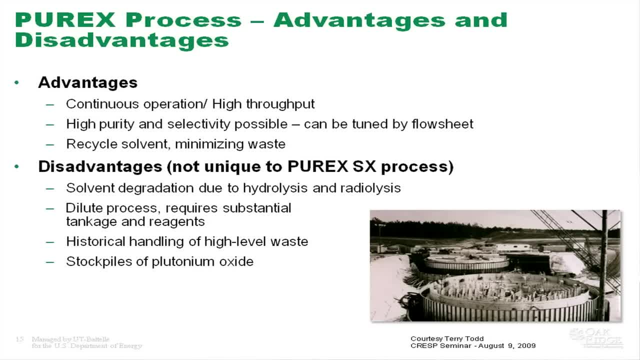 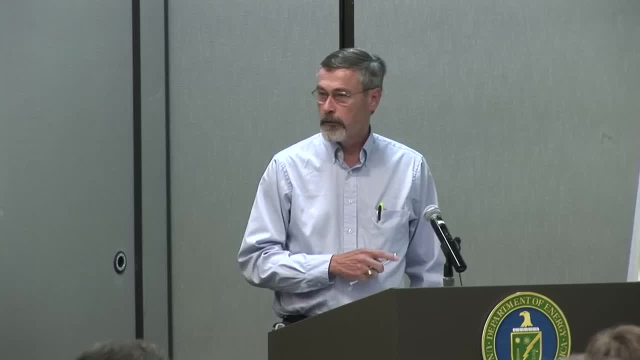 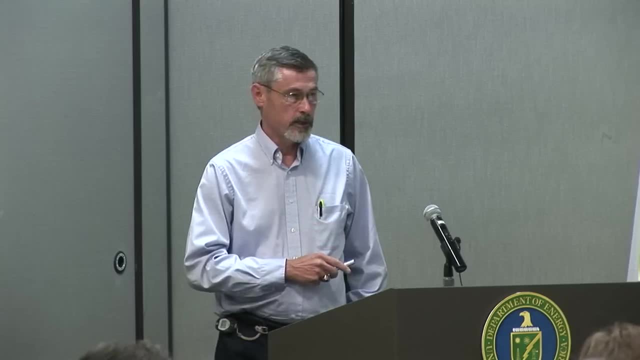 And then what people tend to think of more than anything else when you talk about the PUREX processes are the tanks at Hanford. At Hanford, the purpose was primarily to recover weapons grade plutonium, And there was sort of the waste treatment. 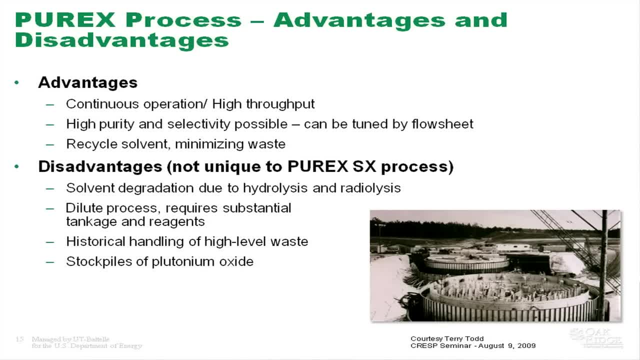 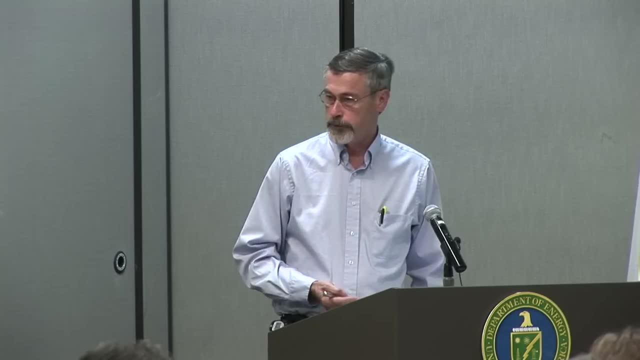 was almost an afterthought. It was put in tanks. So it's the historic handling of high-level waste that tends to be, I think, maybe inappropriately associated with the PUREX process itself, And then coming out of that is the stockpile of plutonium. 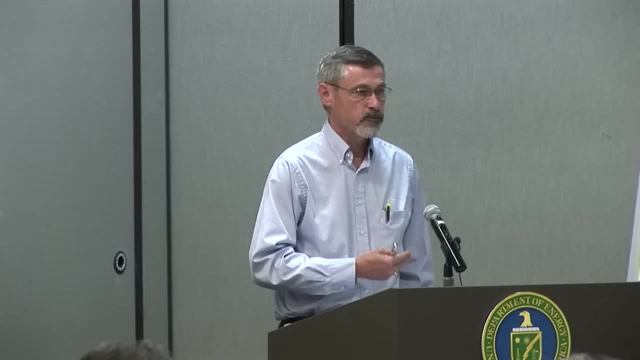 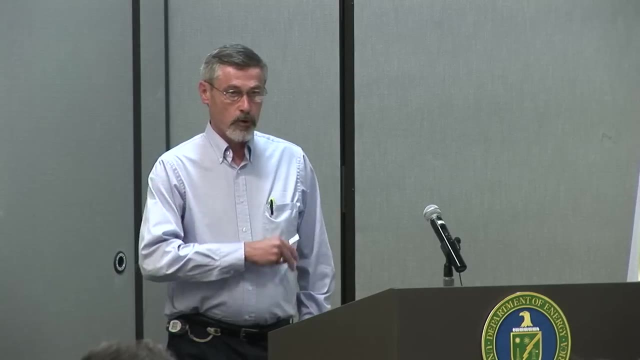 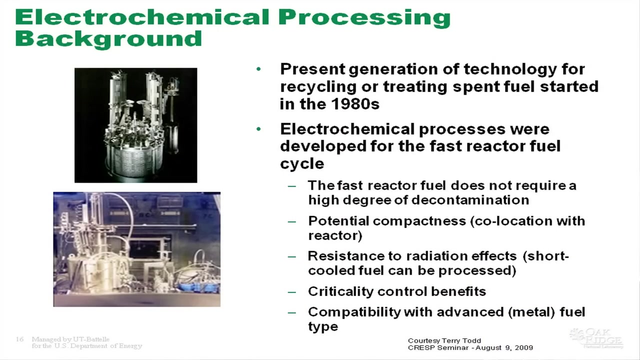 So it tends to bear with it a legacy from the weapons programs. What you'll hear a little bit more about later this morning or this afternoon is the electrochemical process. I'm not going to talk much about these. In fact, this is the only slide I have. on electrochemical processing. It was a technology for an alternate technology, basically for reprocessing or treating of spent fuel. It started that development in the 1980s And primarily it was used for the fast reactor fuel cycle. That fuel cycle tends not to require. 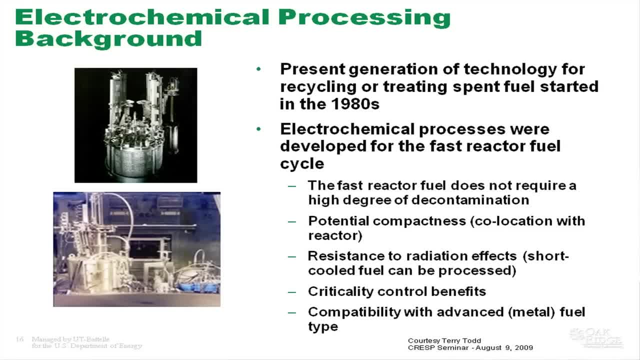 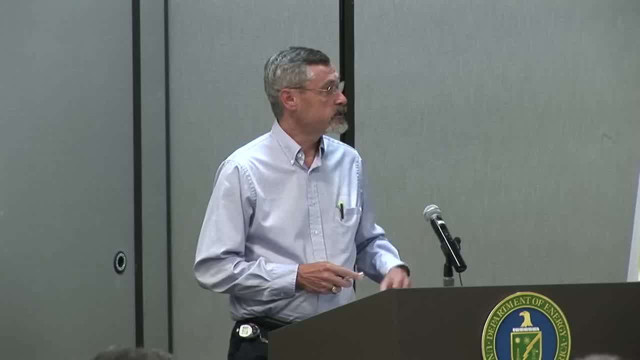 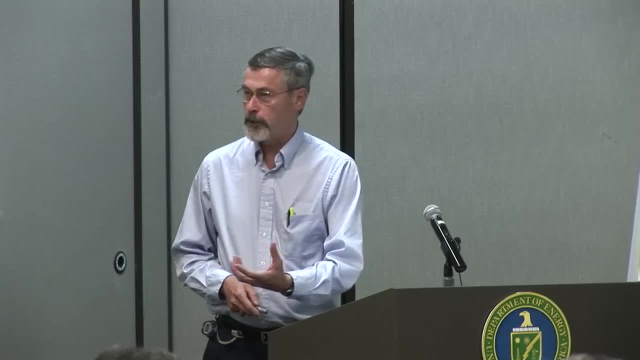 quite as high of a degree of decontamination of the product. It's a compact process, certainly more compact than the PUREX process, with the idea that this could be co-located with several fast reactors. The fuel from fast reactors treated on site. turned back into fuel and put back into one of the reactors in that integral fast reactor site. The materials itself that are used are radiation resistant and so short, cool fuel can be processed. The size lends itself to criticality control benefits and it's compact. 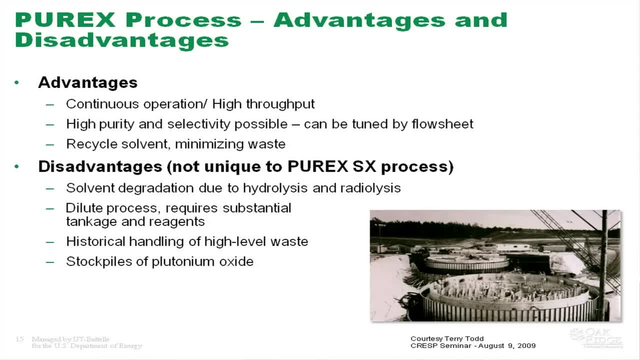 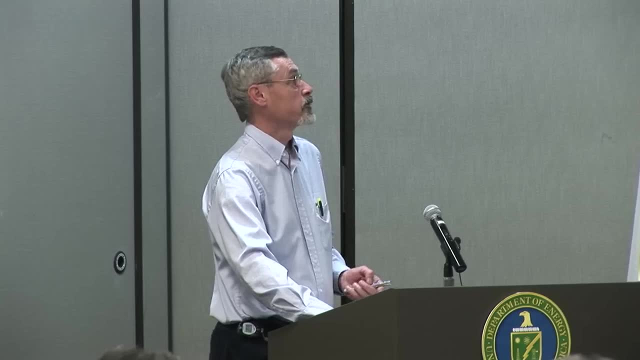 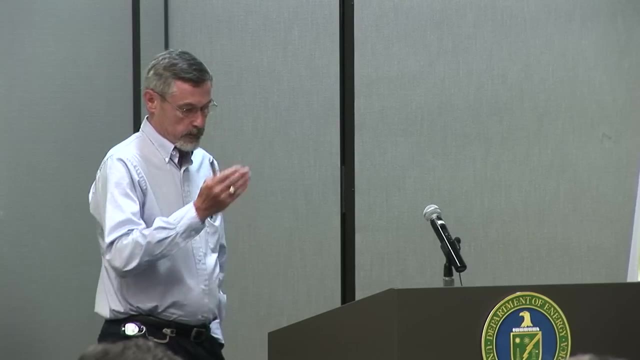 and compatible with the advanced metal fuel types. If you're going to process oxide fuels, you have to have an additional step to convert those oxide fuels into a form that's suitable for salt or electrochemical processing. So now that was sort of the historical perspective. 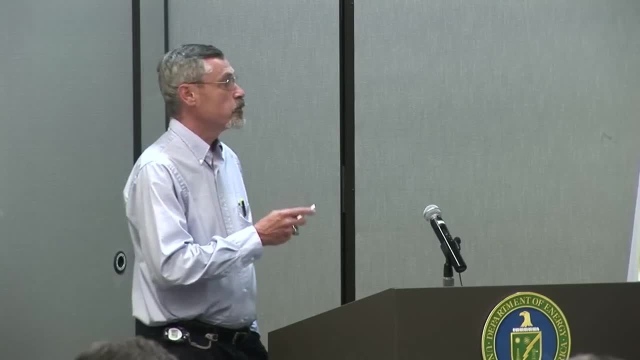 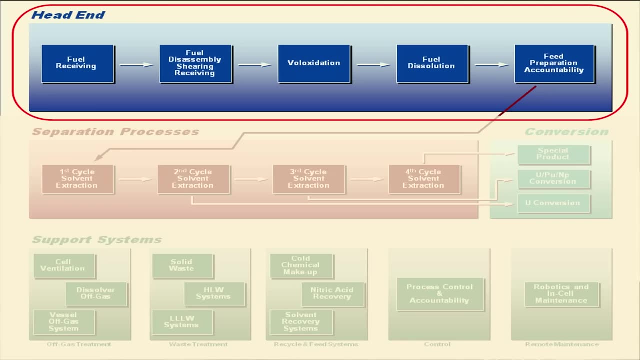 and now we're going to look in a little more depth at each one of the steps of the reprocessing facility. These are sort of divided into the head-end processes, which include fuel receiving, the fuel dissolution, an optional step called biloxidation. 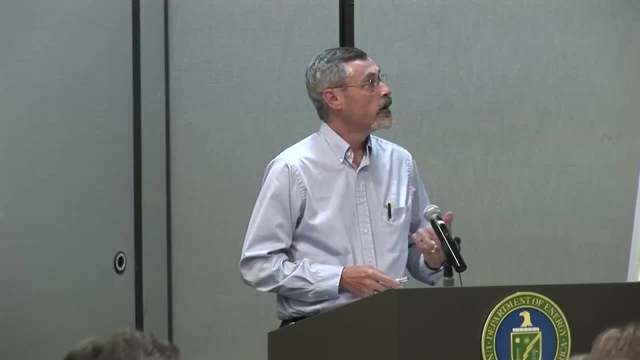 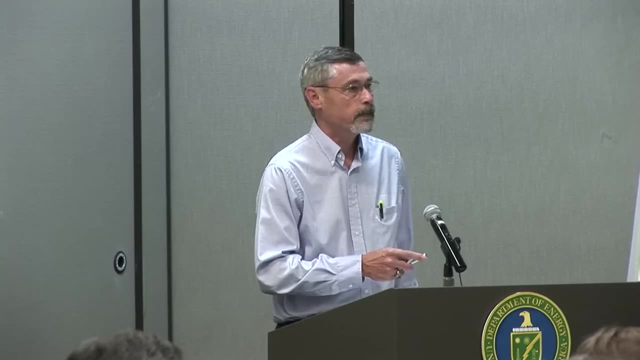 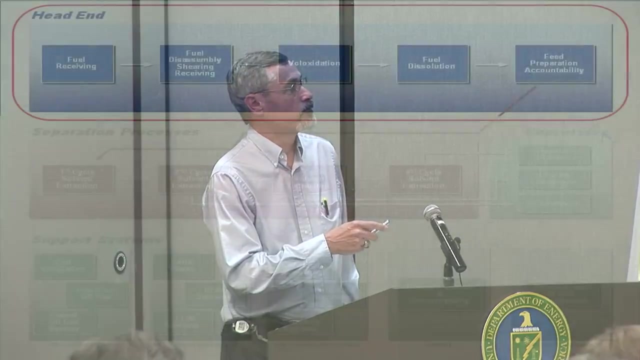 fuel dissolution and then feed accountability and feed preparation. So this takes us from the fuel assembly to a liquid. You then go into separation processes and this is not necessarily the order that they're: first, second, third cycle. In reality you have uranium cycles. 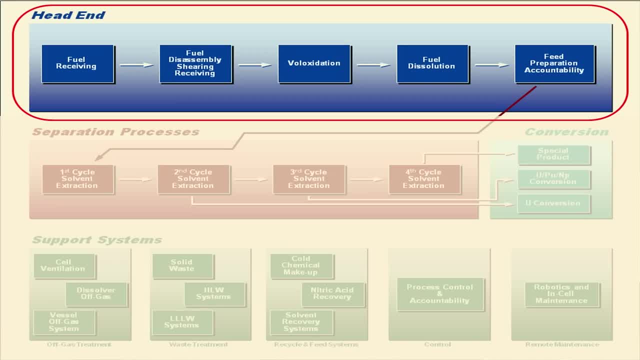 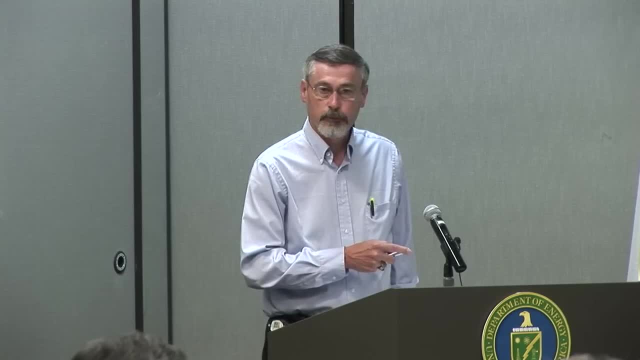 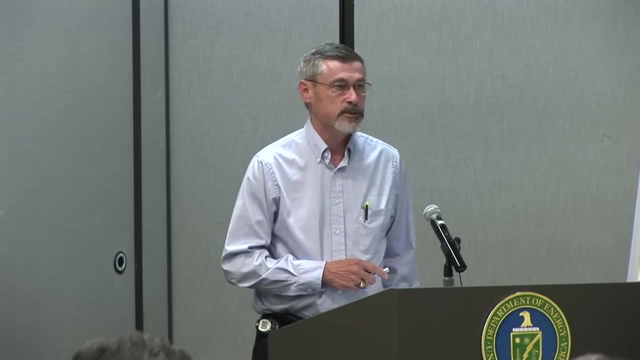 plutonium cycles, but you have multiple cycles- which is all this is intended to represent- of solvent extraction. This does your separation into recovering your uranium plutonium, separating your fission products away from that. Then you have conversion steps. You're still in a solution form. 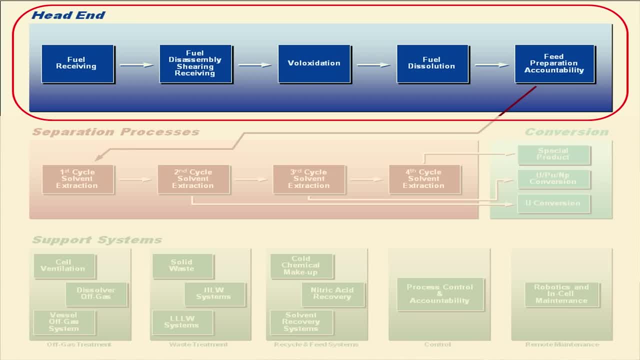 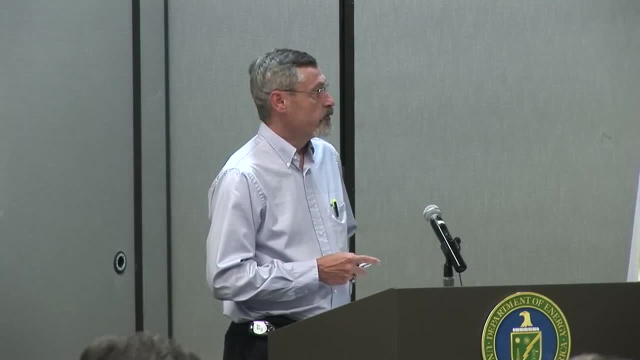 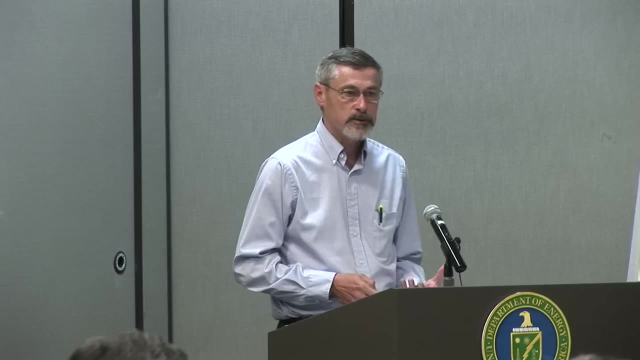 Your next step is: you've got to convert that back into a solid. Then there are a number of support systems that are required. You have ventilation systems for off-gas treatment. You have waste treatment systems. You have recycle systems. You have cold chemical makeup systems. 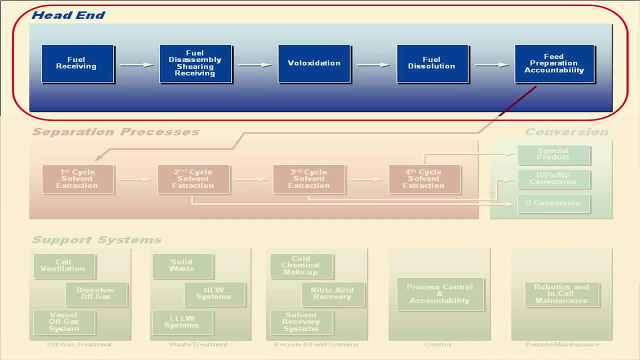 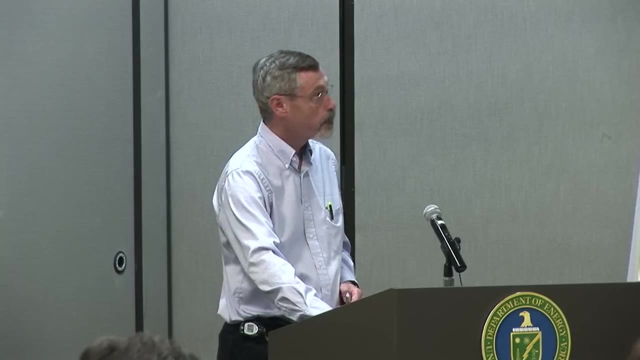 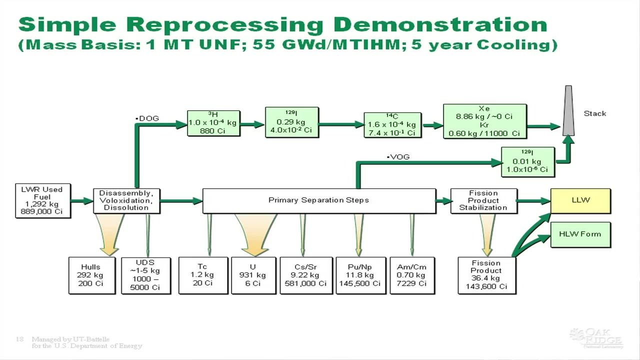 We have process control and accountability systems, Robotics. You have analytical chemistry systems that support all of this, So we'll try and touch on most of these over the next roughly an hour. We'll start with the head-end And we'll look at a very simplified flow sheet. 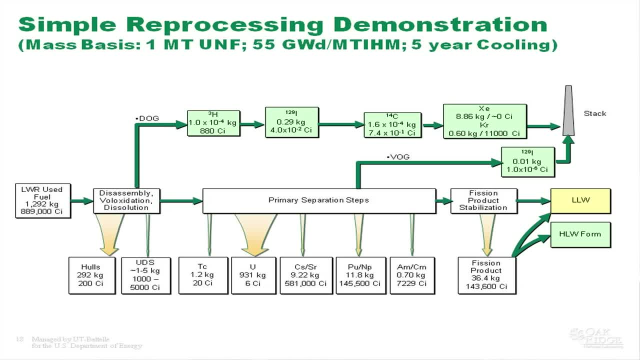 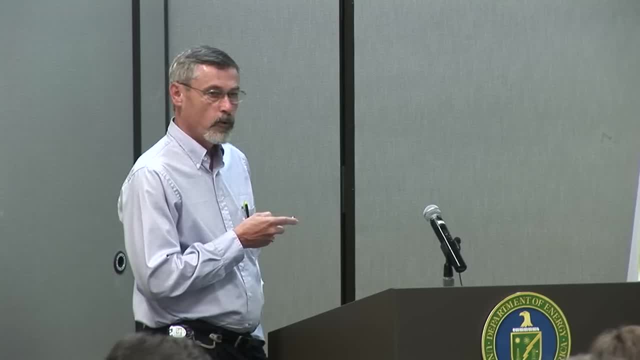 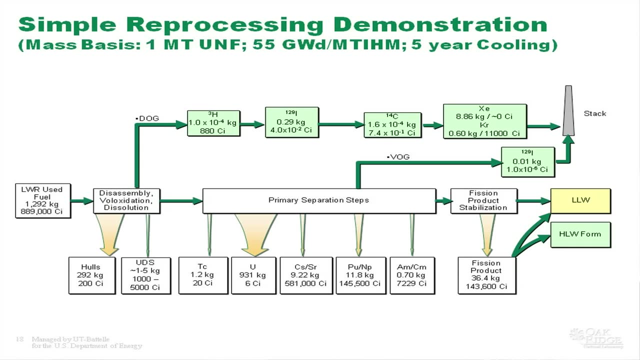 looking at what are we going to separate and how big are these streams. So if you take a metric ton of heavy metal now, that's really more than a metric ton when you get it because you've got the hardware. So out of a metric ton about 300 kilograms are holes and hardware. 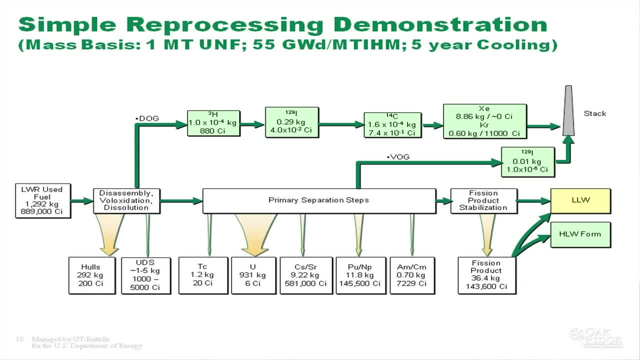 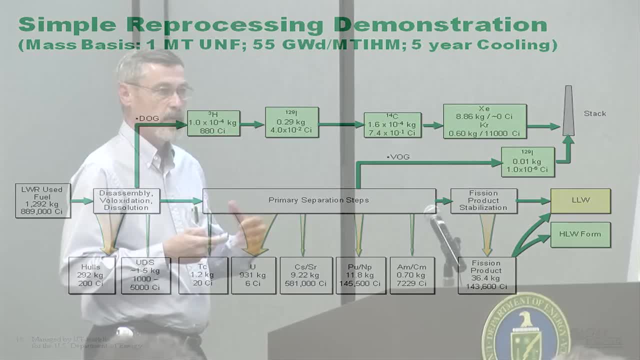 It has to be dealt with. That's paneled in the head-end. This is all your head-end steps. You have a little bit that you never dissolve. Those are your undissolved solids. Maybe one to five kilograms of undissolved solids. 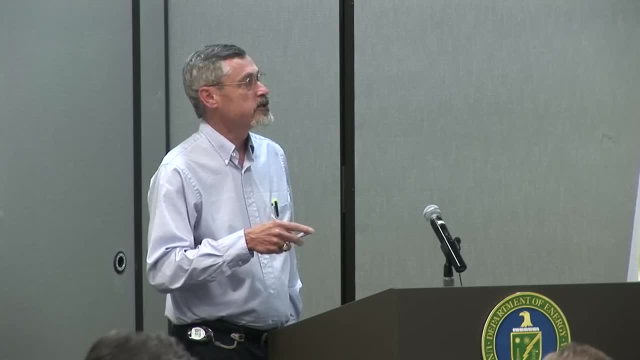 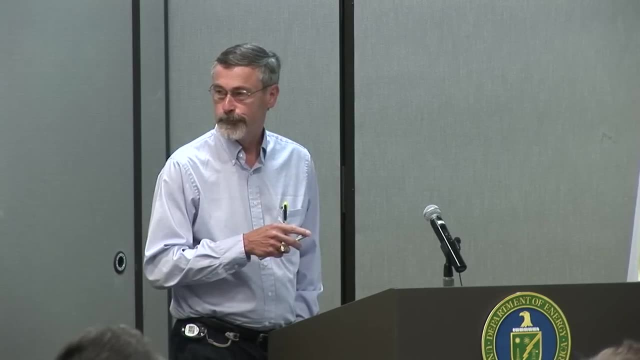 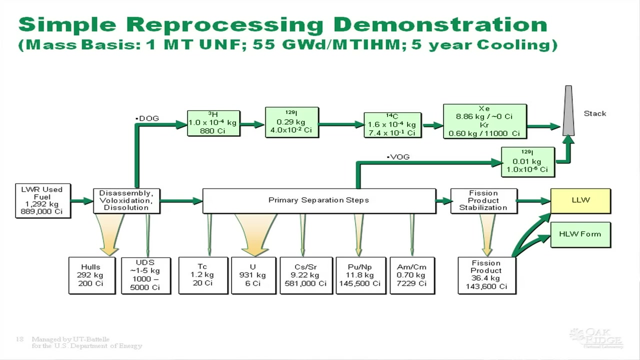 In these dissolution steps, you've got an off-gas stream. All the volatile components come off: A gram of tritium Mm, 300 grams of iodine, Maybe less than a tenth of a gram of carbon-14.. Kilogram quantities of xenon and krypton come off. You have some technetium that comes out of your separation steps. The bulk of it is that uranium stream, So once you remove it, everything else is pretty small. The total amount of fission products about 34 kilograms. Plutonium, about 11 kilograms when combined with the neptunium. So these streams, with the exception of this one, are really pretty small, And small doesn't necessarily mean they're easy to deal with. We'll come to that in a little bit. 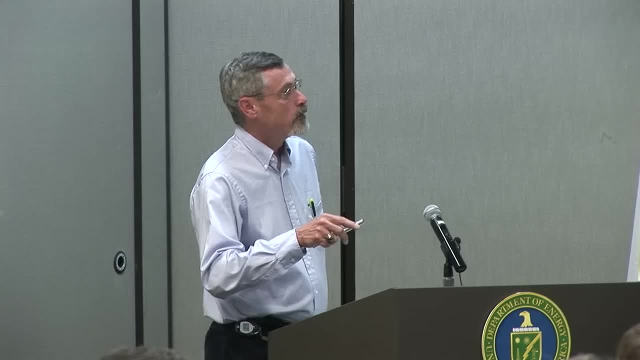 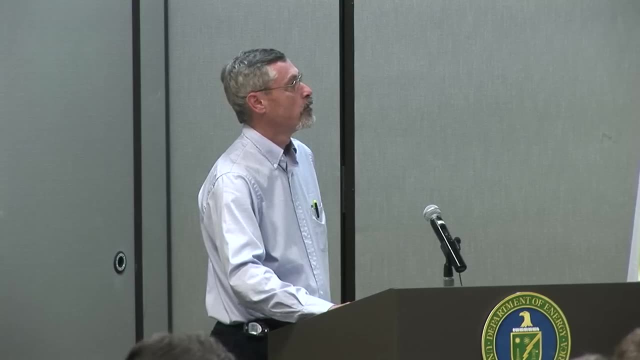 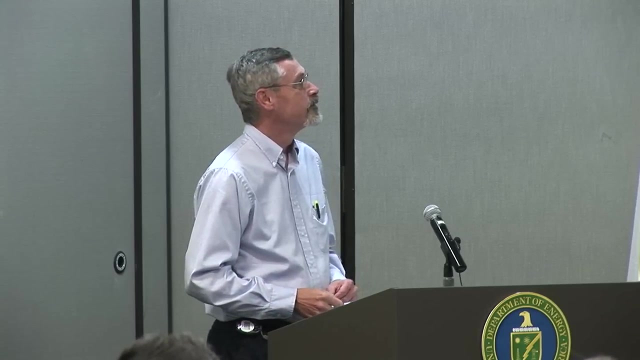 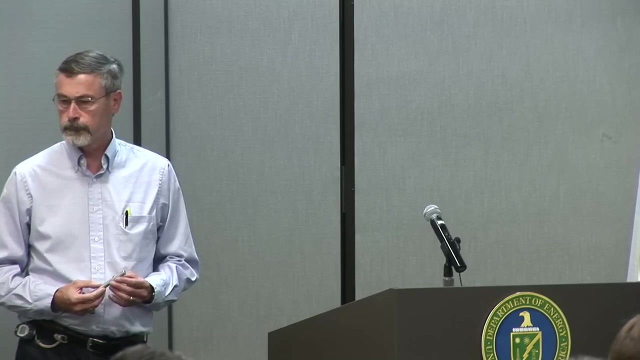 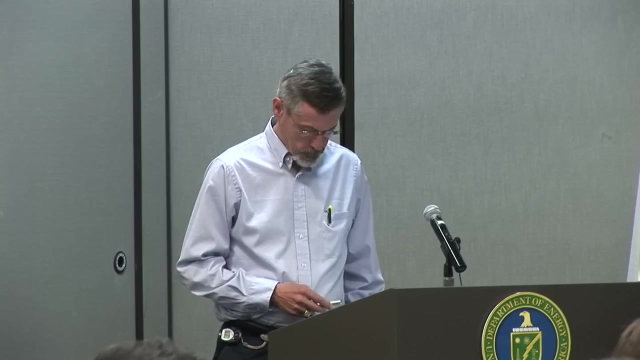 Now you've got this. We'll come to the vessel off-gas in a little while, So we won't talk about that now. Okay, I'm trying to advance. The question was: could I comment on what is the low level waste? 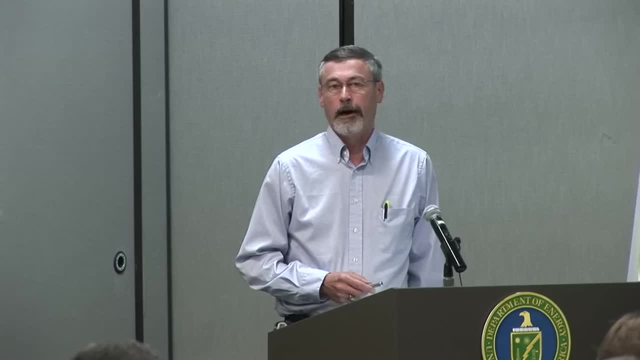 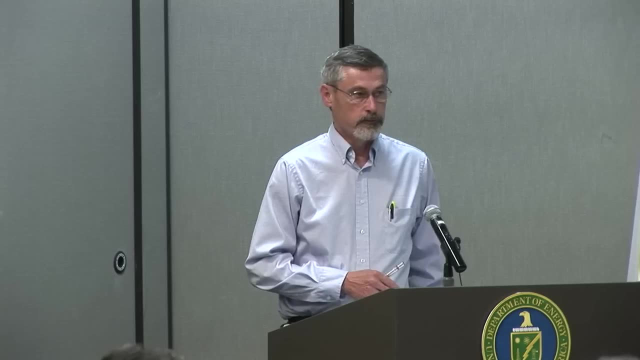 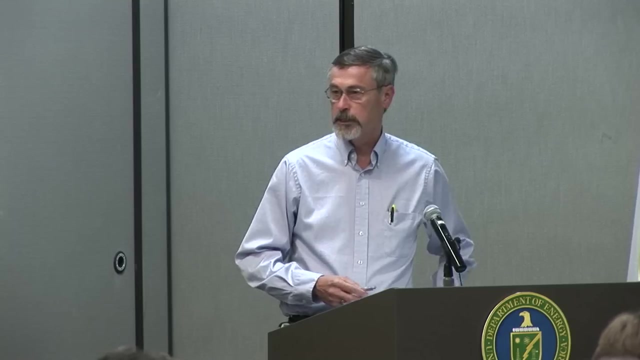 Is it greater than Class C waste? You can have many types of low-level waste coming out of a reprocessing plant. This can be shoe scuffs would be low-level waste. Some of this is incinerable materials. There certainly is a stream that is greater than Class C waste. 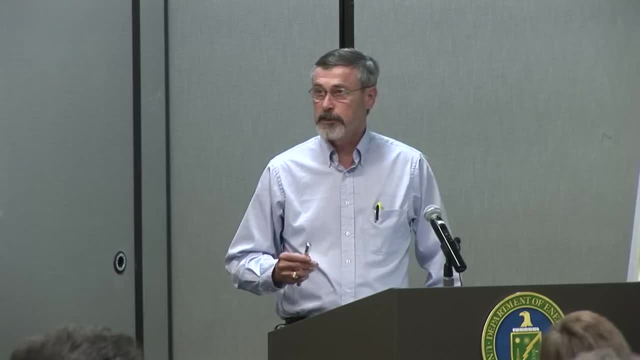 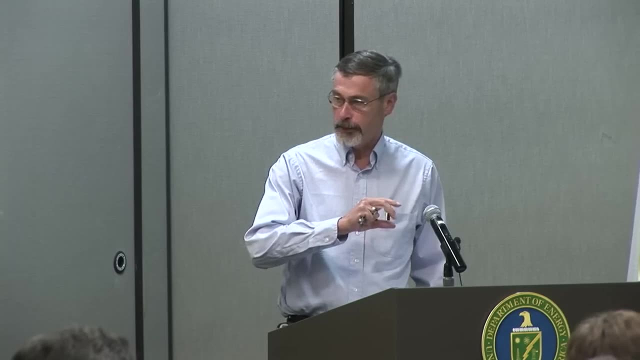 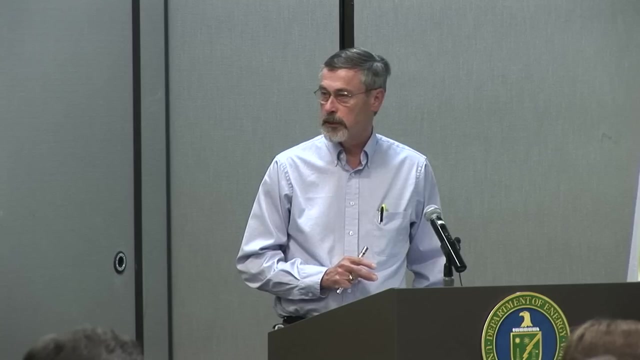 Many of those would be from the defense side- be considered true waste, the type of waste we would currently send to WIP. That's one of the streams that is a little more problematic for us to deal with under the current waste definitions. 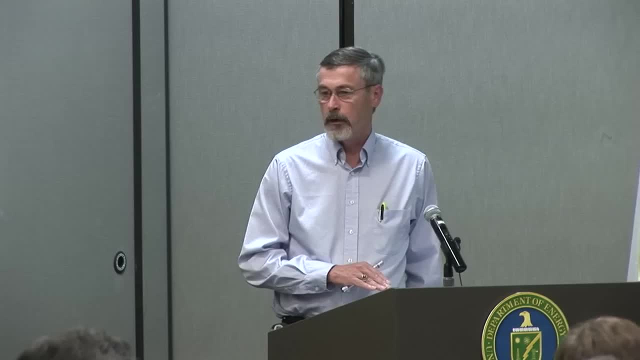 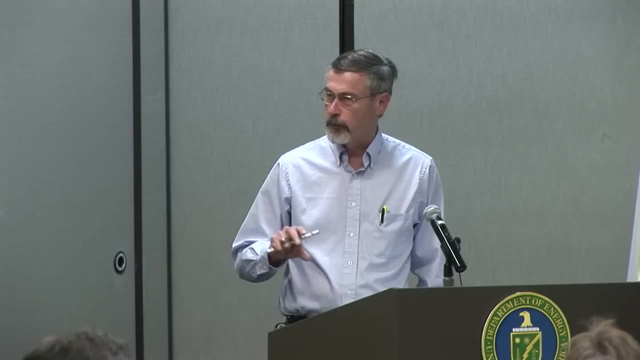 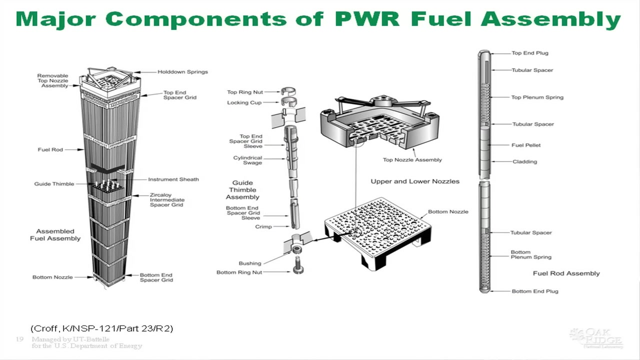 In the US we don't have that category of low and then there's moderate waste. We don't really have anything in that moderate waste category. Alan showed this slide yesterday looking at the fuel assembly. The reason I'm showing this again is in that disassembly step. 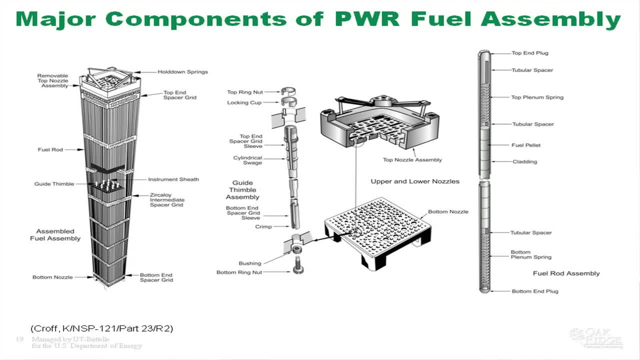 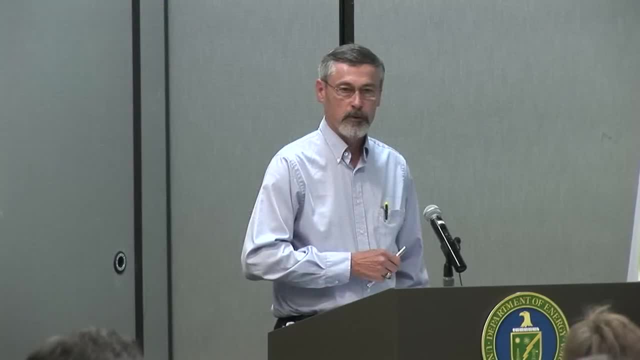 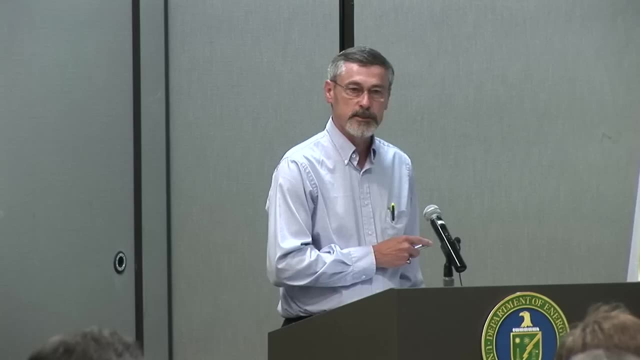 what we're interested in are these fuel pellets. We've got to get those out of all of this hardware. We've got to make a way to get access to chemicals. We've got to make sure that we can effectively reach these so we can do the separations. 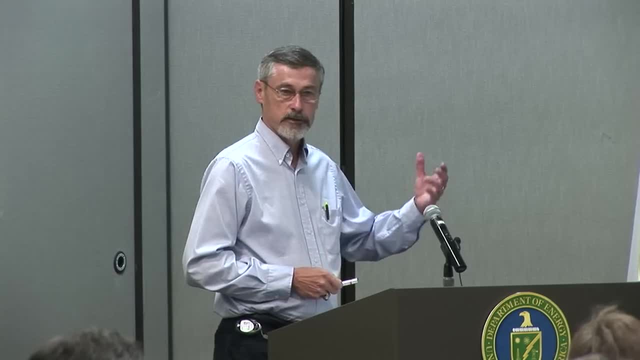 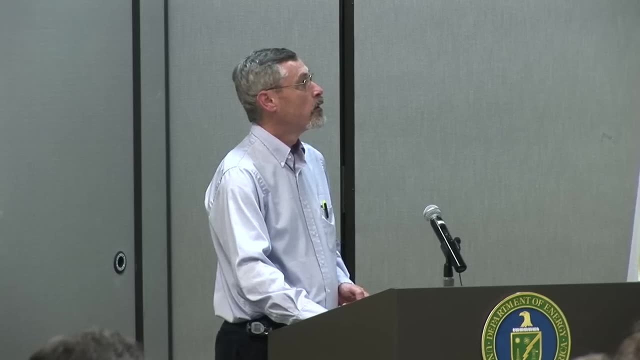 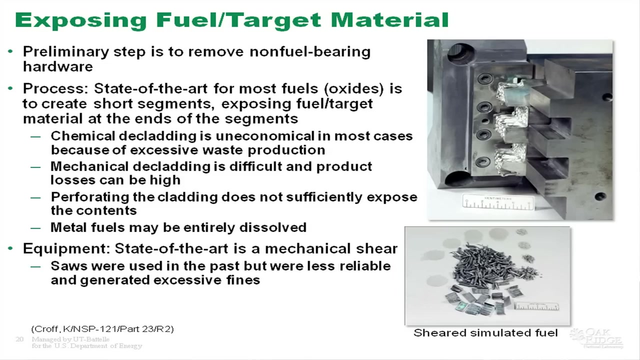 We've got to get rid of all of this and we've got to handle all of this remotely and in a continuous way. feed this into a plant. The major job is to how do we expose that fuel of the target material? The whole head-end step of fuel disassembly is 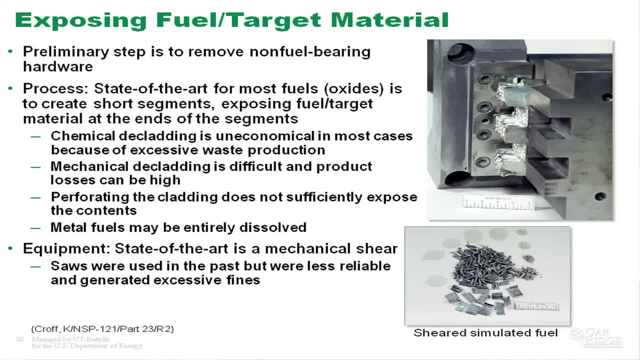 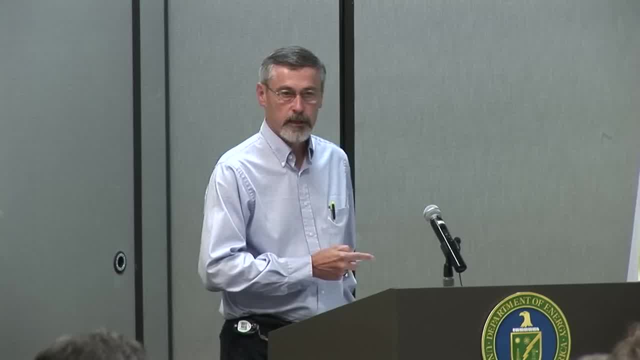 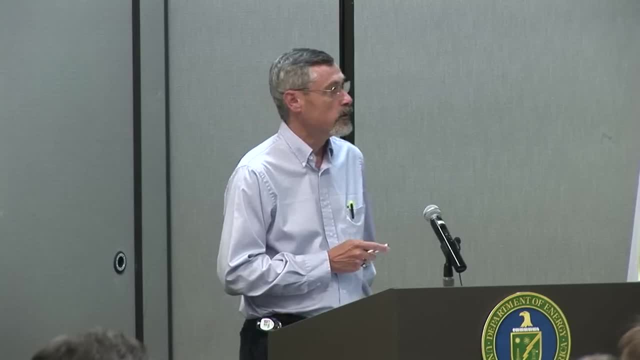 making the fuel into a form that we can attack the uranium oxide, the plutonium oxide, the fission products chemically with nitric acid. The state of the art in most cases is to shear this fuel into small segments. There have been lots of different designs for shears. 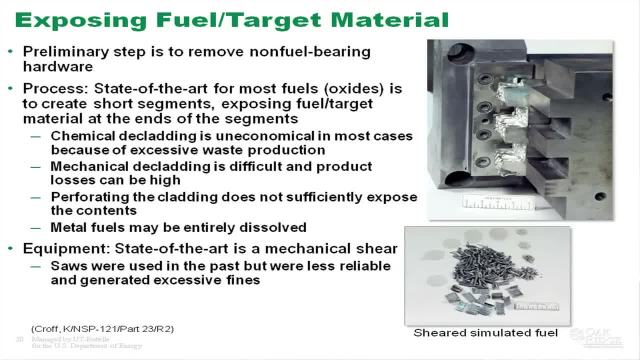 This one is sort of has the pinking shear type of approach. You take an entire bundle of fuel, you compress it with mechanical rams and you take the shear blade and you cut across it. Well, the problem with that is you've got to be very careful in design. 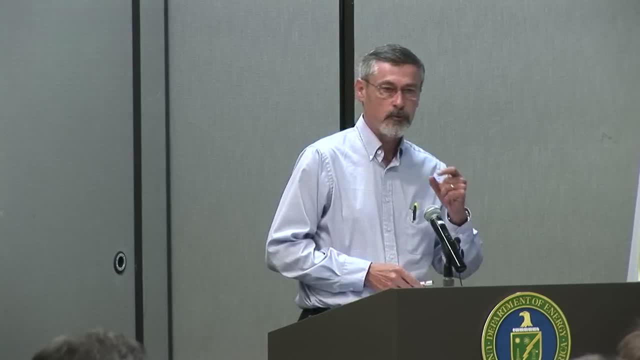 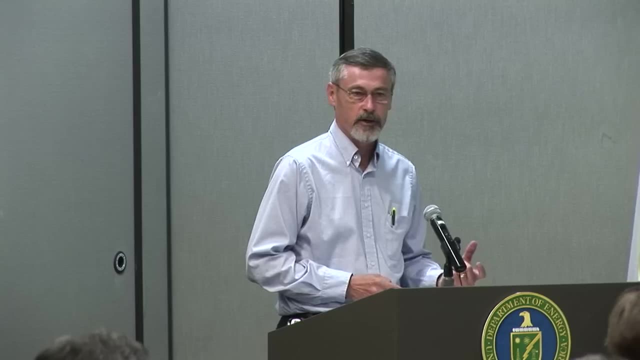 that you don't crimp the ends of those fuel pins, Because if you crimp the ends of the fuel pins then you can't get to the fuel meat inside of there with your nitric acid. So the design is fairly important that when it's cut, 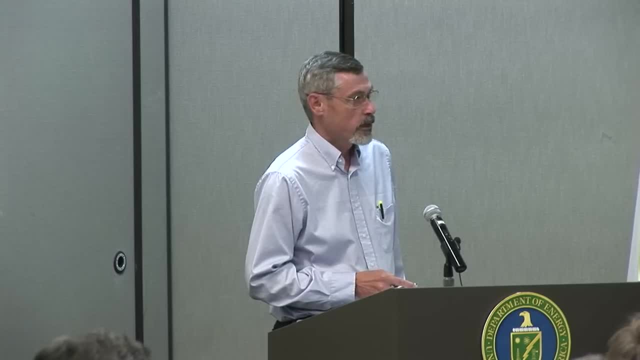 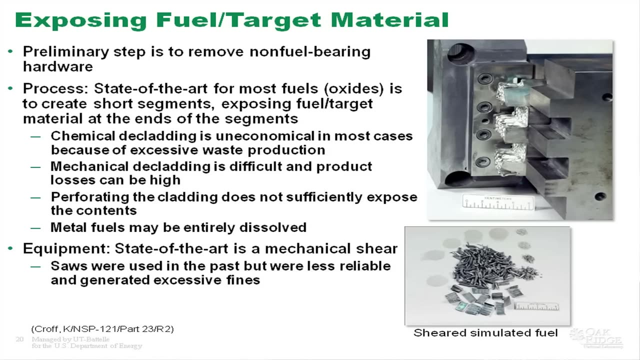 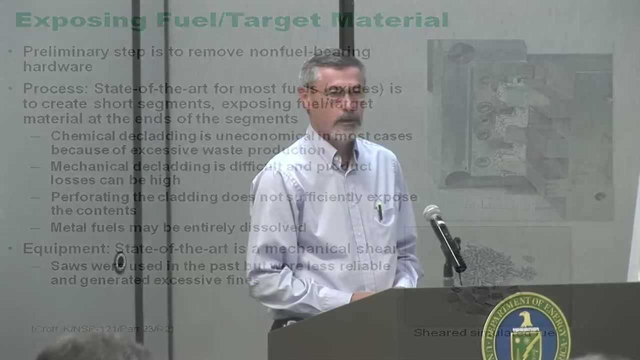 you've still got open ends of that But you may also get lots of other hardware. You produce some fines that come out. They've tried. many methods have been tried to mechanically de-clad the fuel. run it through like can openers. 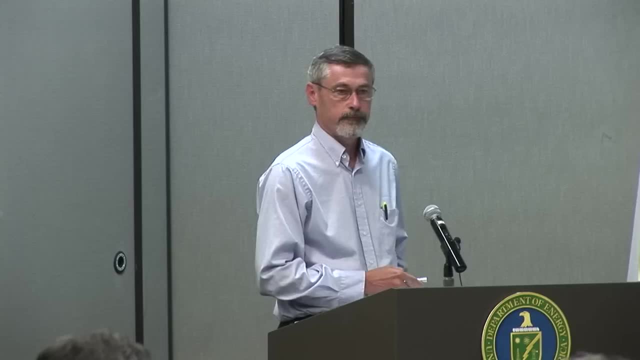 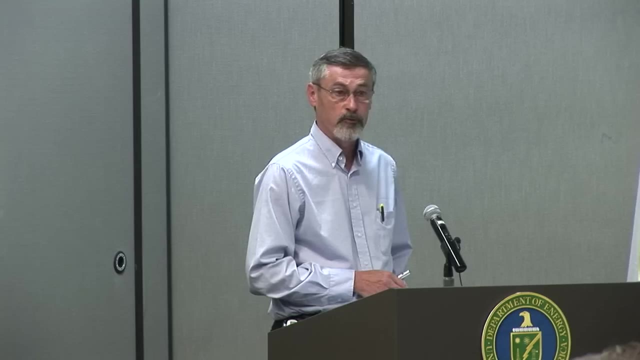 You've got the fuel that has a shroud on it. That further complicates this, because now you have a larger piece of stainless steel or zirconium that wraps around the whole fuel bundle. In fast fuel that's a stainless steel hex shape that comes around. 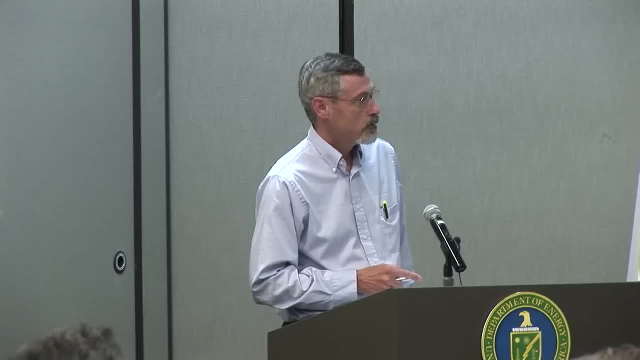 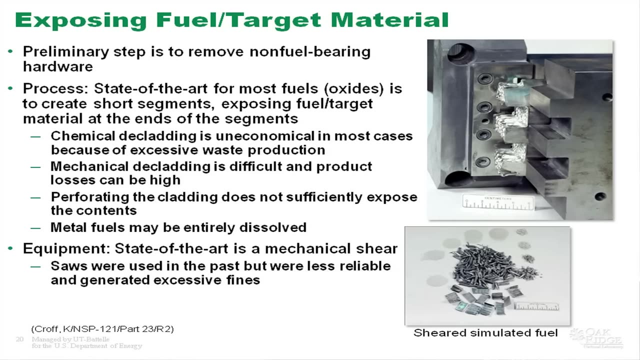 This is actually some simulated fast reactor fuel, And so the design of the shear was such that that was broken up into larger segments. Now, these all then have to be fed into the next piece of mechanical hardware, whether that's the veloxidizer or the dissolver. 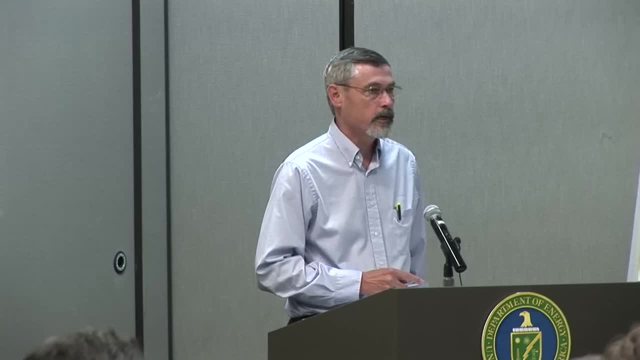 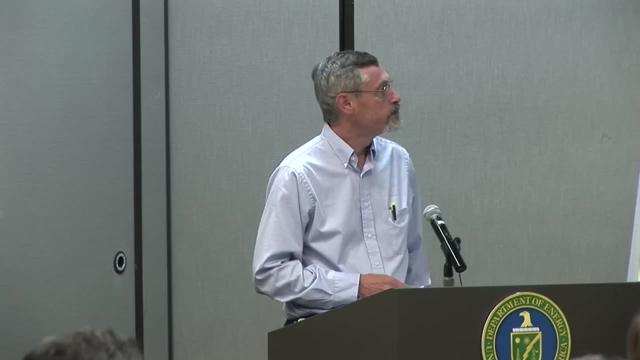 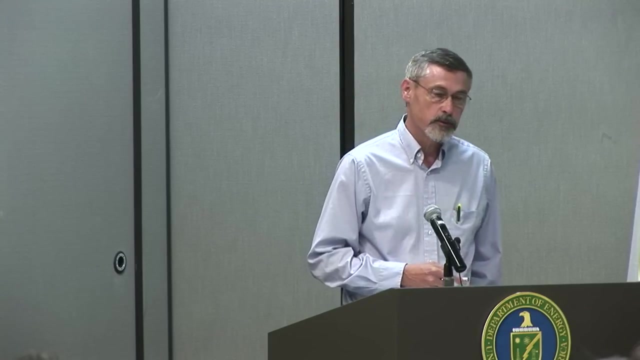 So now you're handling, and solids handling tends to be a problem. It's not quite as easy as transferring solutions. Saws have been used in the past, but they tend to be less reliable than the hydraulic shears and they produce a lot of fines. 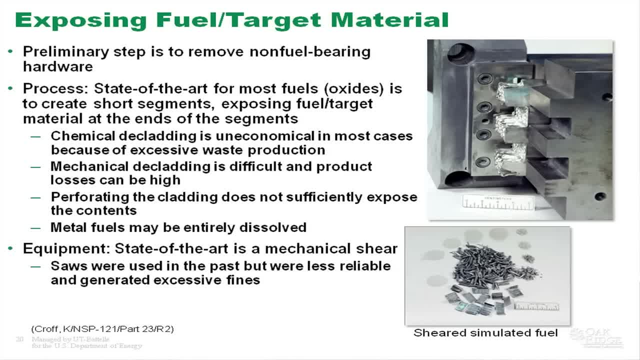 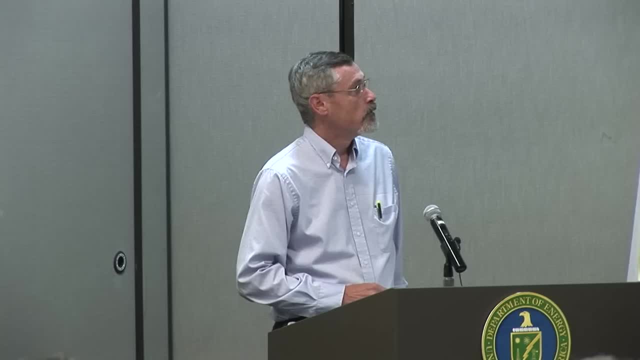 So that's sort of the. I could talk a long time on what design of disassembly equipment. We've used lasers in the past to make cuts down the shroud of fuel bundles, But the others? I guess one of the things I ought to talk about is chemical decladding. Some fuels- aluminum clad fuels. you do dissolve the cladding. That produces additional waste. You could dissolve the cladding on fuel You don't really want to do that. That's another 300 grams per metric ton of liquid waste then. 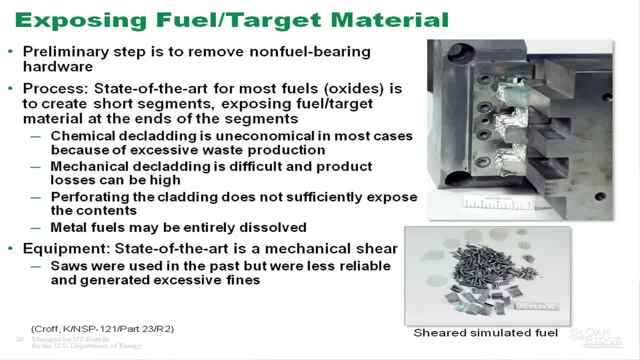 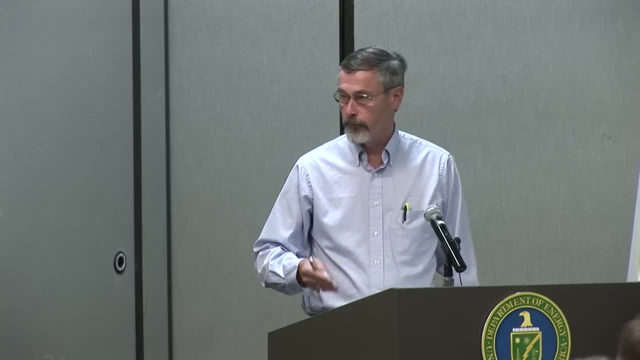 that you have to solidify. If you can remove that intact now and then clean it, there may be some other things you can do with that: cladding rather than, or you compact it as metal and not go through all the vitrification processes. 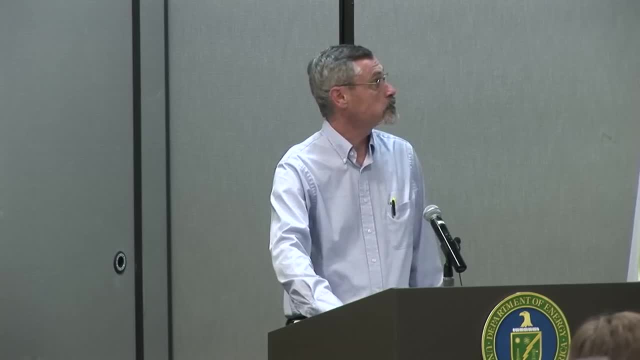 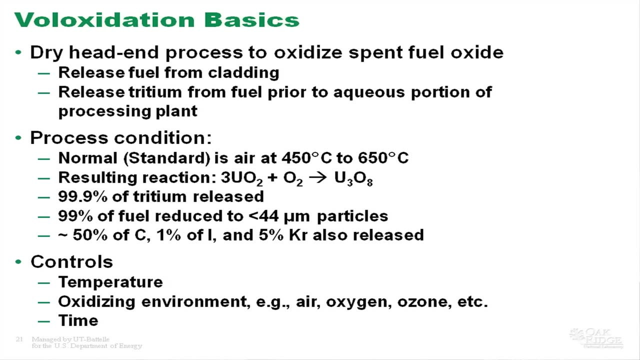 and things like that, to dispose of this high-level waste. Veloxidation is an optional step that would follow the shearing of the fuel. Veloxidation has two primary purposes. One is to reduce, to release the fuel from the cladding itself. 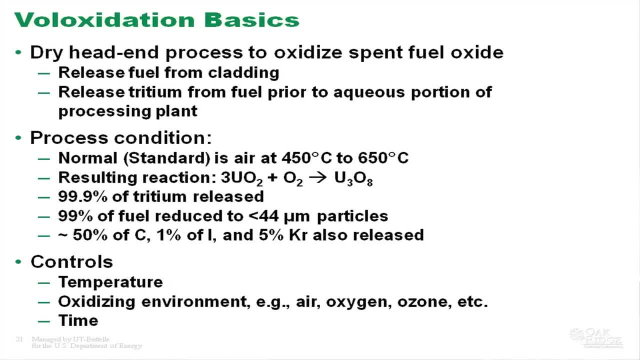 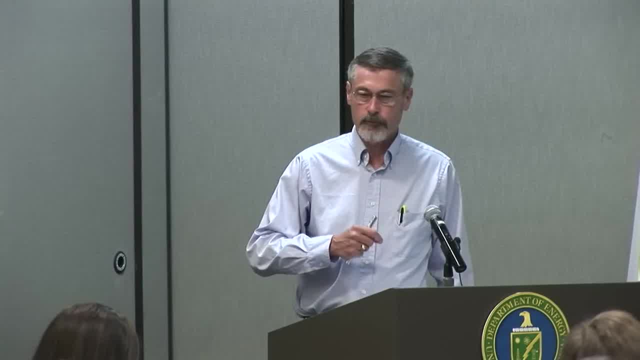 and to release the tritium from the fuel prior to it going into the dissolution process. That's an important aspect in the sense that if the tritium- and if you remember back a couple of slides, that was a fraction of a gram per metric ton. 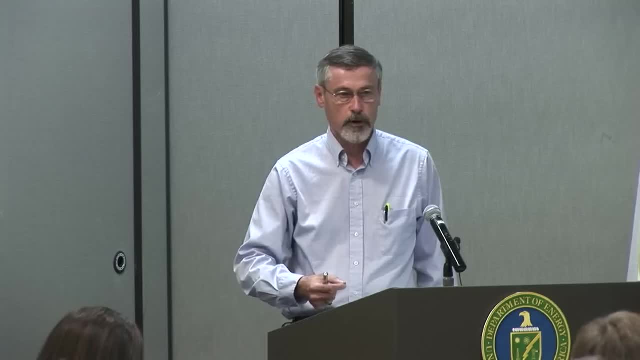 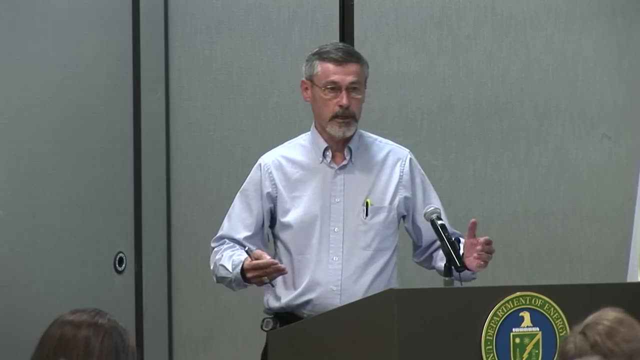 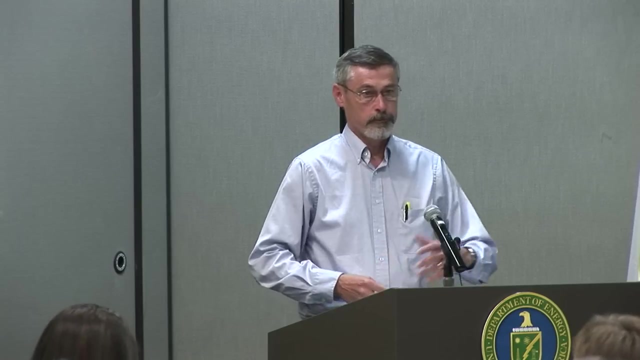 If it gets into the aqueous part of the system. now that tritium becomes tritiated water and mixes with all of the aqueous streams in the plant and has to be dealt with with all of your liquid waste, What do you do? you know you may evaporate. 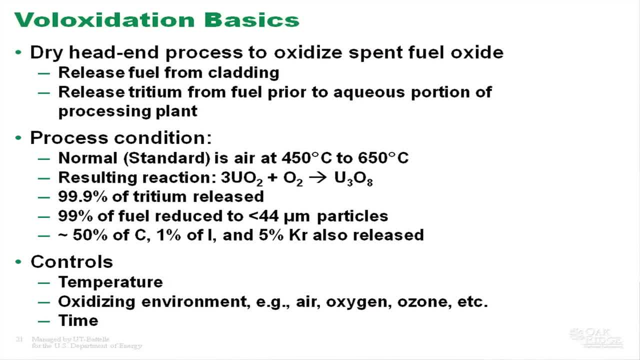 What do you do with the water? You've got the tritium in the water. Now you can't get rid of it, So it would be nice to remove the tritium before you get into the aqueous part of the system. 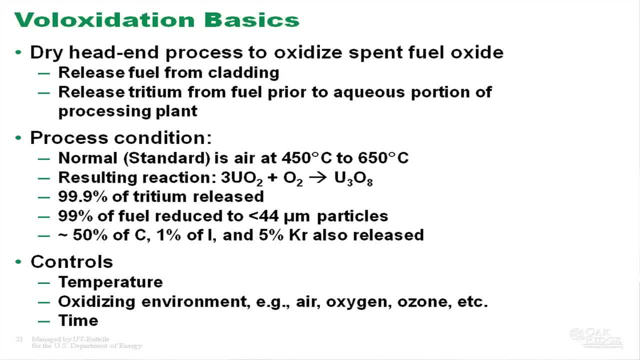 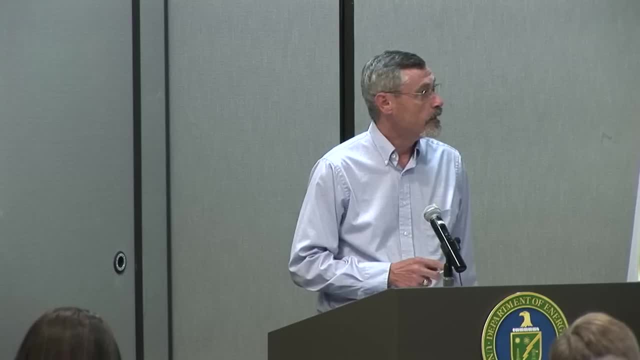 Using air. you can, in essence, burn the fuel from U02 to U308 by the addition of oxygen. When you do that, about 99.9% of the tritium is released into the off-gas stream And the fuel, as it changes, crystal structure expands. 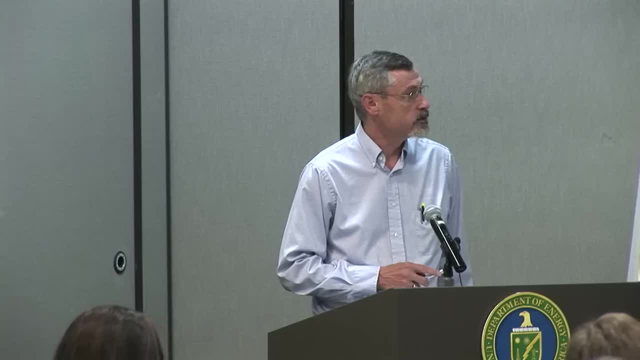 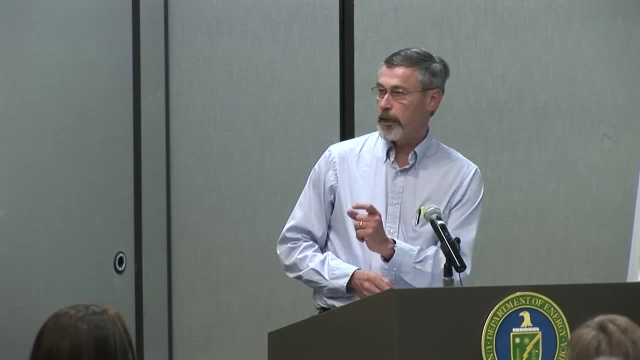 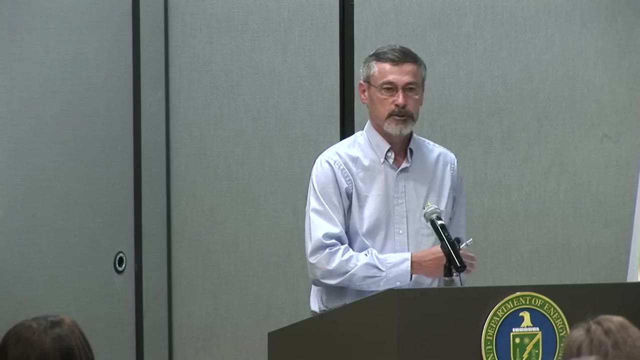 forms relatively small particles, about 44 microns in size, and comes out of the cladding. So now we've got the fuel, which was a solid pellet in terms of a powder That can be separated from the hardware, just a sieving process. 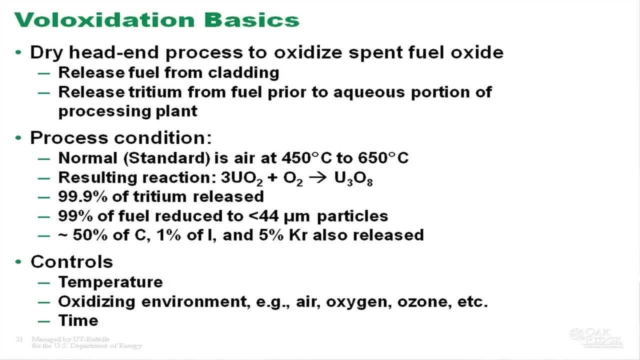 At the same time, we release a fraction of the carbon dioxide, the carbon-14 in the fuel, a very small fraction of the iodine and some of the noble gases. The process itself is controlled by the temperature. The higher the temperature, the faster the oxidation rate. 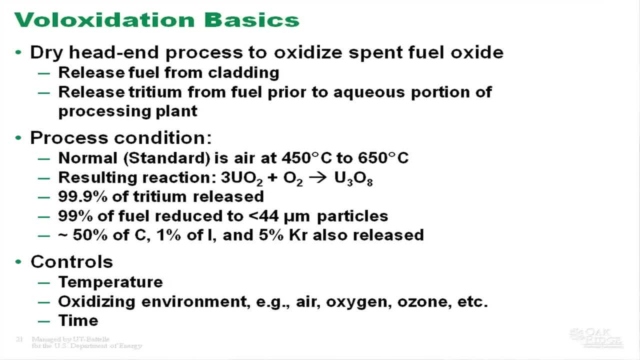 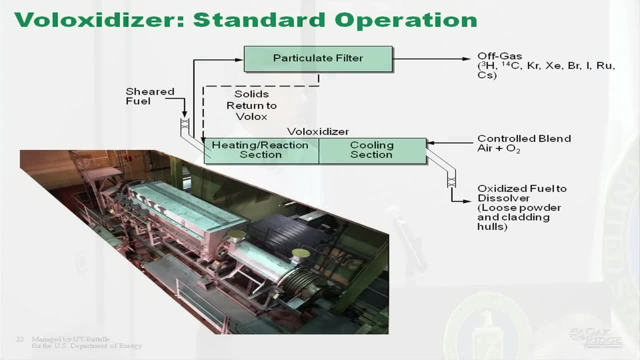 We can change the oxidizing environment by adding oxygen or ozone And time. These are all kinetic processes, Time and temperature And the reactant's composition. This is a picture of a prototype veloxidizer. That's about 12 feet long. 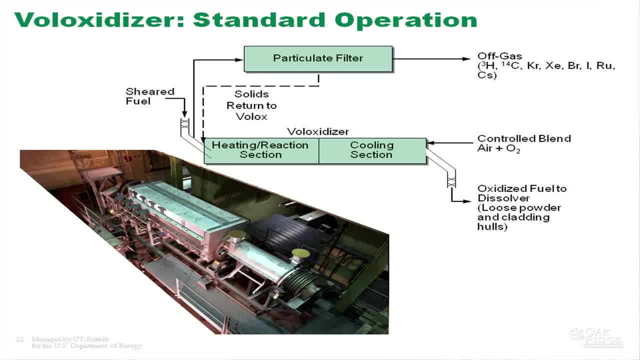 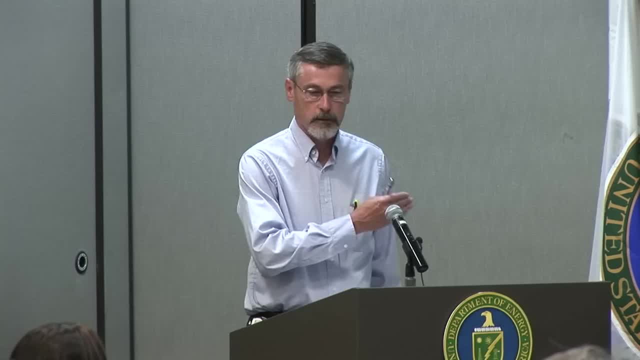 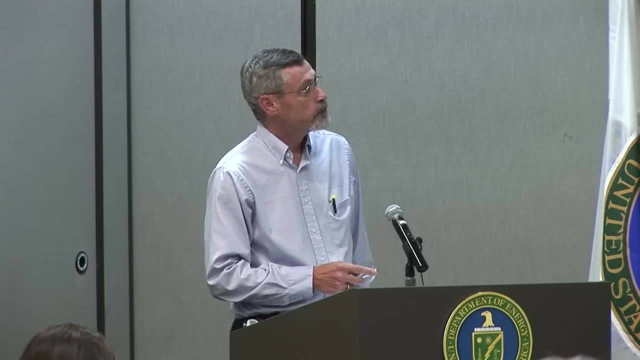 This is scaled at about a half ton a day. throughput. The fuel is fed into the heating end And the best example this was a commercial kiln. It's a rotary kiln. There's a heating section and a cooling section. Air and oxygen is fed in. 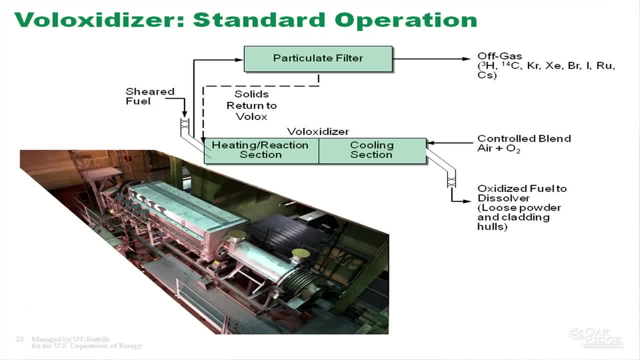 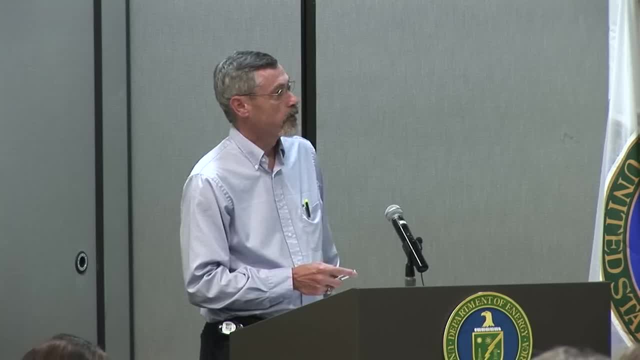 countercurrent to the flow of the solids, As it does. as I said, the U02 is oxidized to U03, U308, excuse me- and the oxidized fuel powder and the claddings are discharged at the far end. 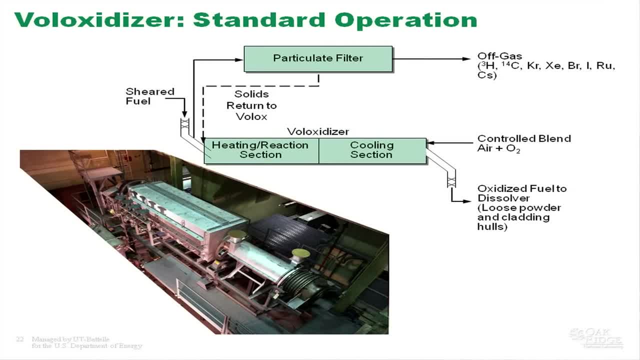 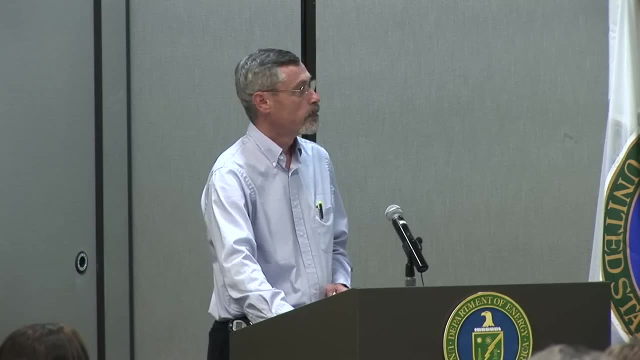 The airstream carries some particulates out that have to be recovered in a particulate filter and returned back to the veloxidizer, And you have an off-gas stream that contains your volatile components. That has to be treated before release to the atmosphere. 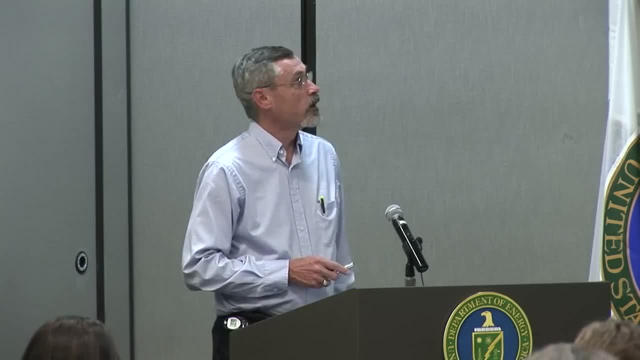 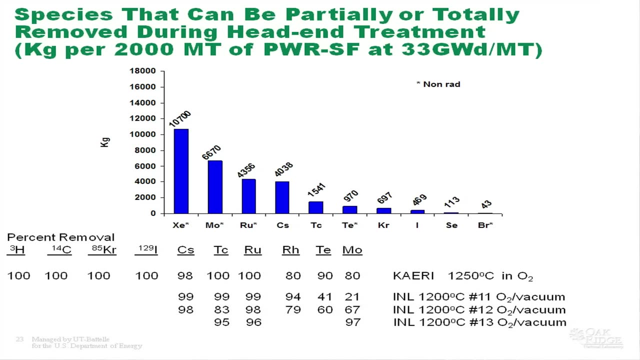 There is some additional experimental work going on on. as you increase the temperature of veloxidation, you can drive off a number of additional species. Work in Korea using oxygen at about 1250 degrees C has shown, whereas we at 500 to 600 degrees. 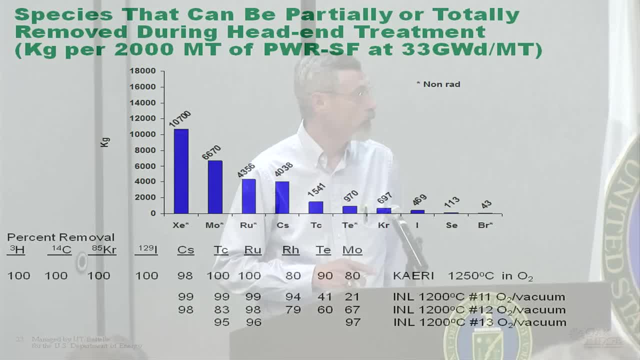 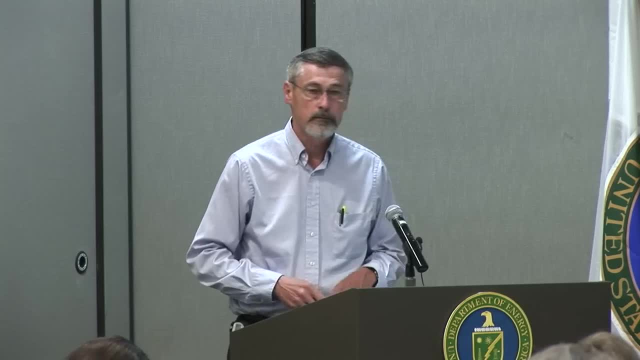 get about 1% of the iodine. they get 100% of the iodine, all the krypton, all the carbon-14, and substantial fractions of the cesium, technetium, ruthenium, moly and others. 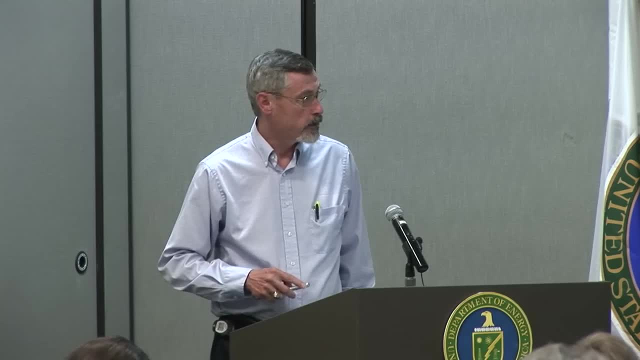 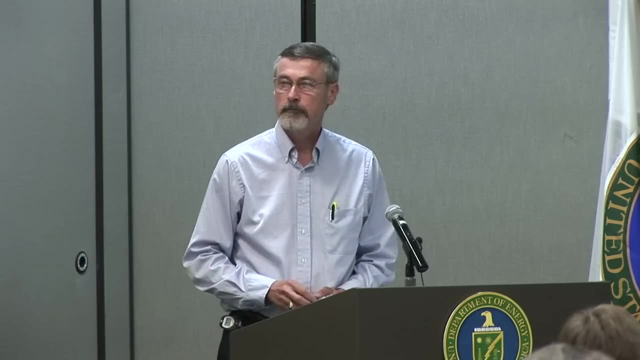 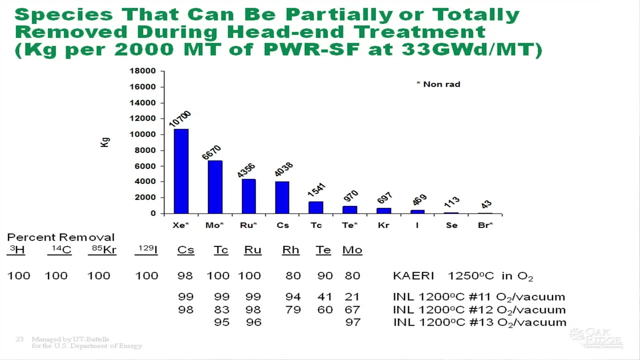 Some additional work at Idaho has shown very similar results for these other species. This is veloxidation process has not been employed commercially to date. It's under investigation for a future reprocessing plant, So this is experimental work that's been taken to. 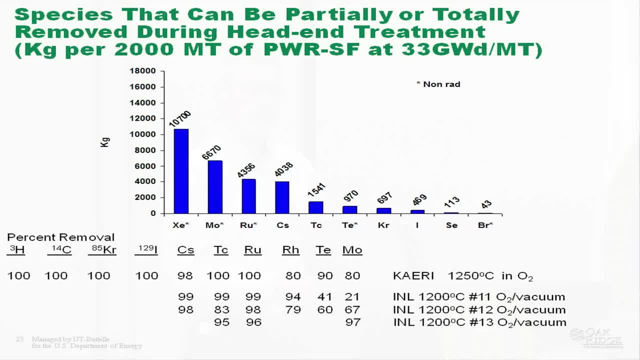 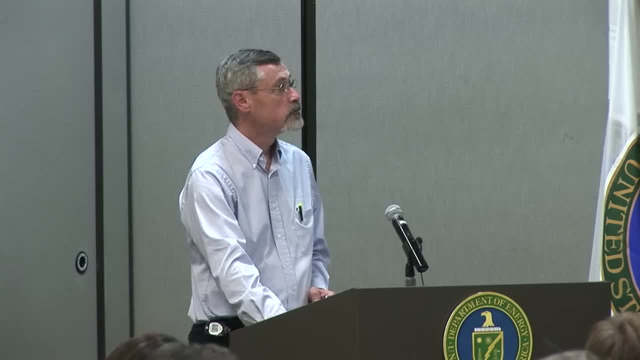 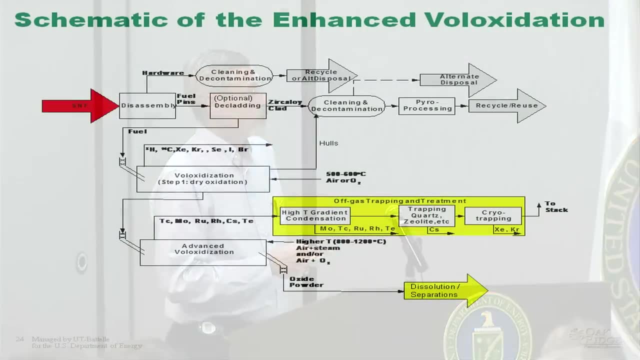 to a reasonable scale- cold, but on gram and kilogram levels or gram and kilogram scale- hot. So how would you implement some of these advanced veloxidation steps? You'd probably have a standard veloxidation process to separate the bulk of the tritium. 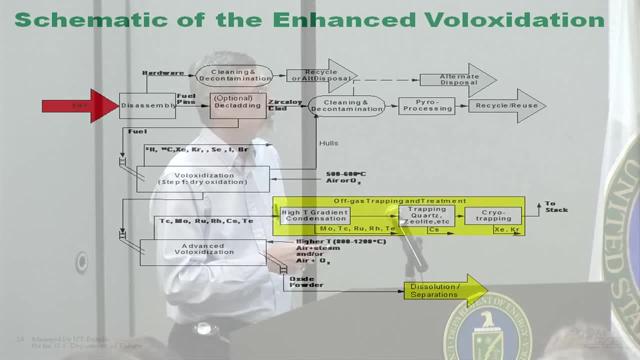 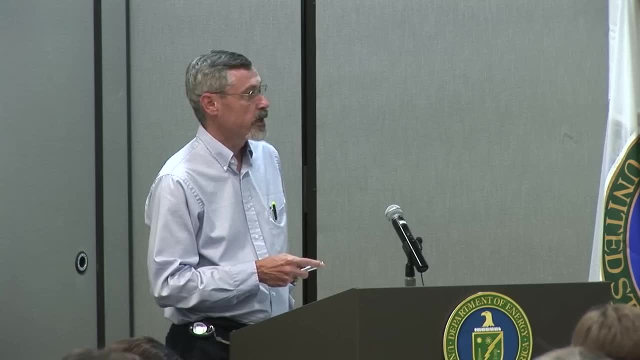 and separate the cladding at this point. You could then go to the advanced veloxidation, where you go to higher temperature operations. As you do that, you have a different off-gas stream. These are the semi-volatiles, and you'll separate those primarily. 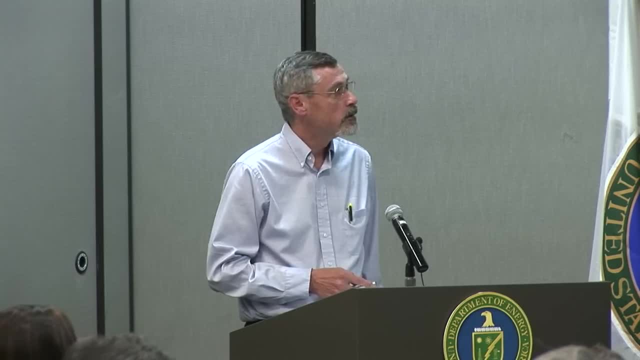 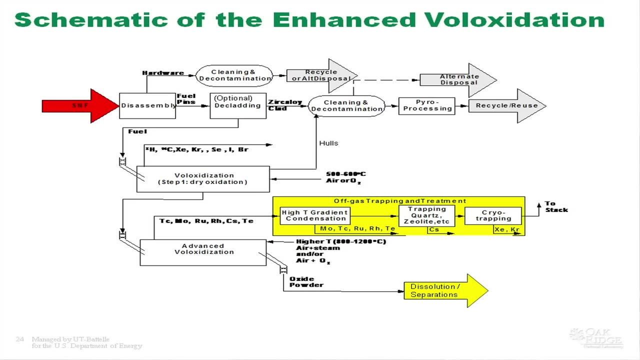 with a high-temperature gradient condensation process. There is some krypton xenon that will probably come off and you'd use cryotrapping for that. There are potential advantages If one could remove some of these. that might simplify the downstream processes. 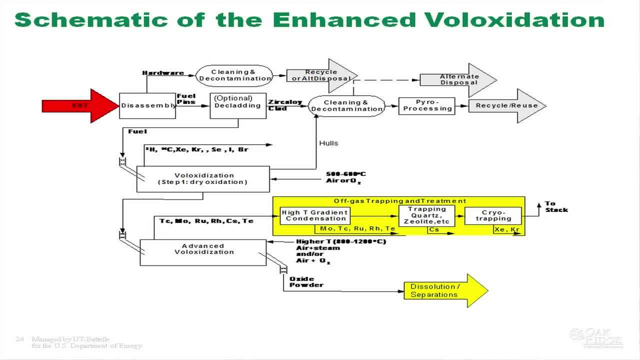 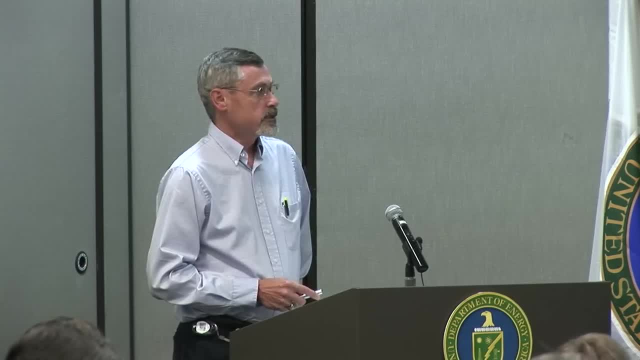 This is all in the developmental stage. Is that cesium? Is that cesium particulate? Pardon me, Cesium particulate In this case, it's not necessarily particulate. It would be a volatile compound and then be solidified. 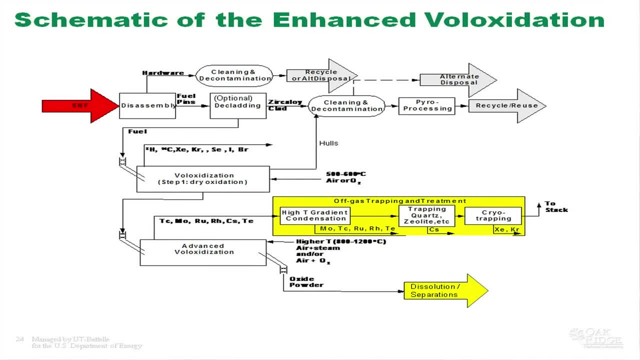 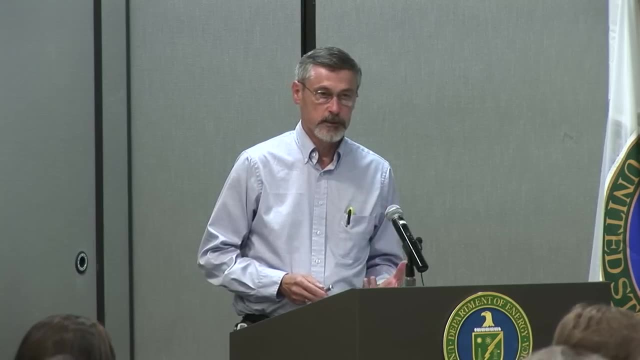 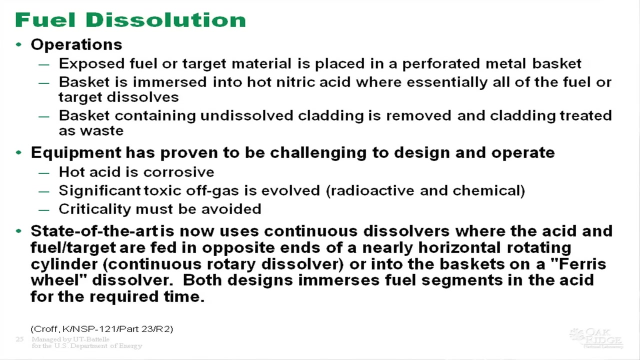 It would plate out, It would be gaseous. Yeah, it would be gaseous at these temperatures. Now, whether you do veloxidation or not, the next step is fuel dissolution In the reprocessing plant. you've exposed the fuel material. 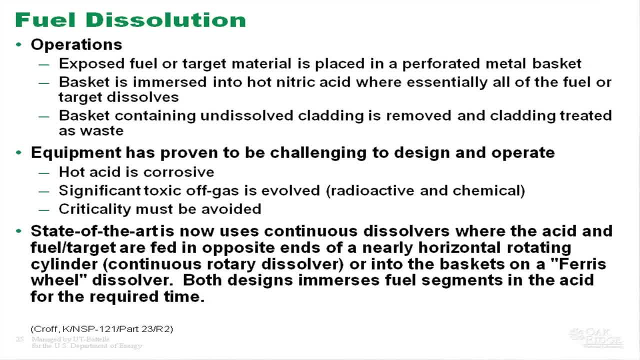 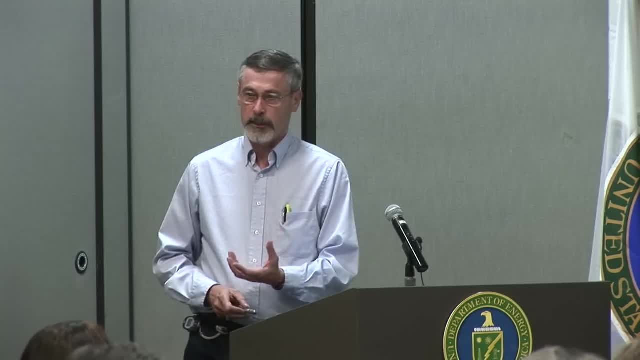 and typically it's placed in a perforated basket. This basket's then put into nitric acid, where essentially all the fuel in the target or the fuel bundle or the fuel piece dissolves out. The cladding stays in that basket unless you've separated it beforehand. 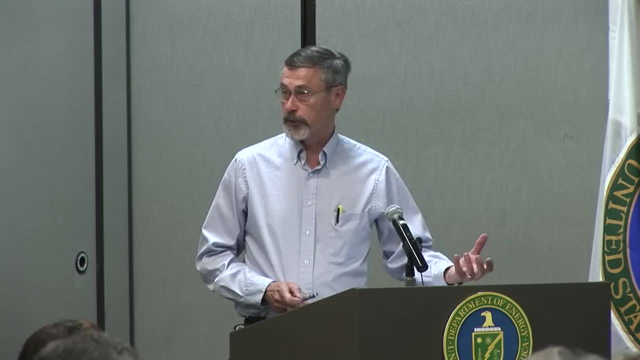 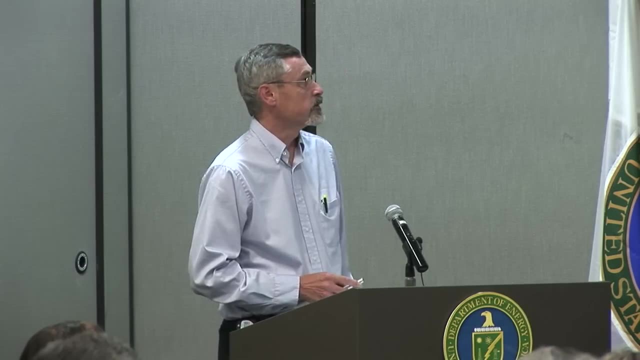 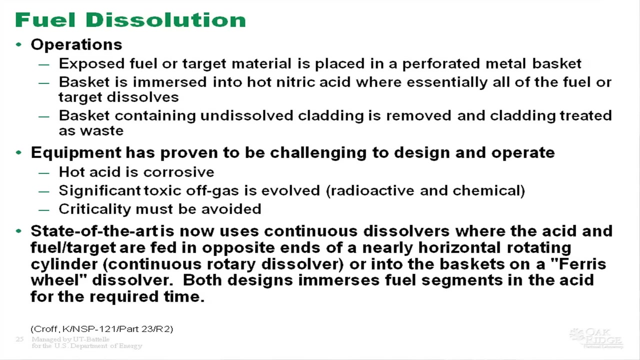 and the cladding then is treated as a separate stream. You may wash that. You may subject it to additional acid washes to remove the last traces of the transuranic materials. Hot nitric acid's very corrosive, so the design of this tends to be a challenge. 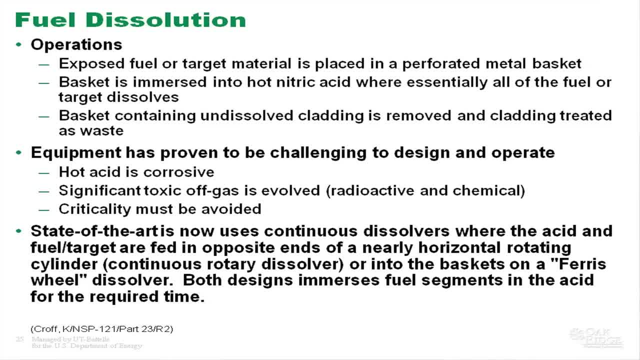 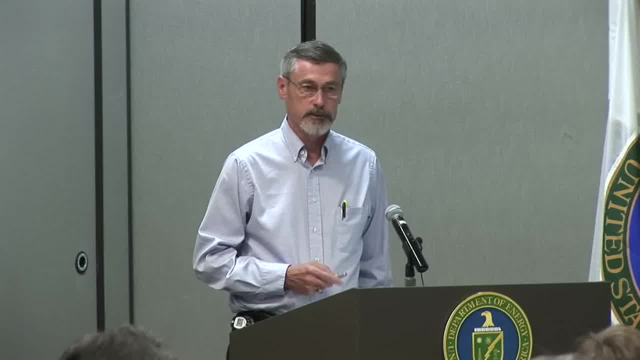 You have a lot of off-gas that come off of the dissolution process. Those have to be treated and this criticality of this becomes a very important issue. You have lots of liquid and you have all of your fissionable materials. 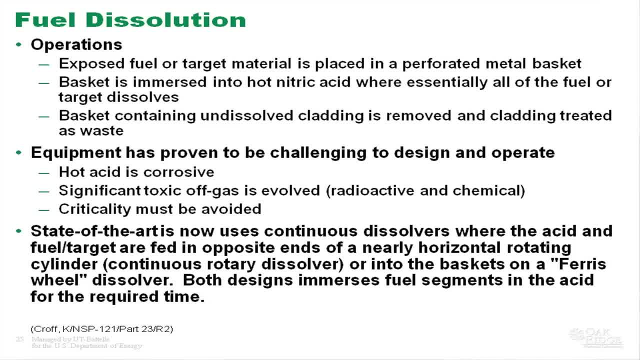 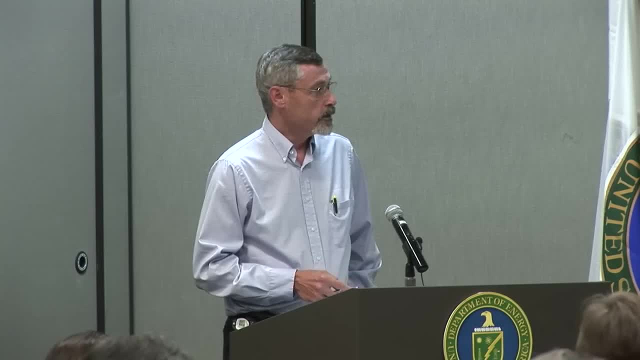 State-of-the-art is moving from the batch dissolvers to a continuous dissolver process where the acid and the fuel is being fed at the opposite ends of a dissolver or into a Ferris wheel dissolver, and I'll show both designs in a second. 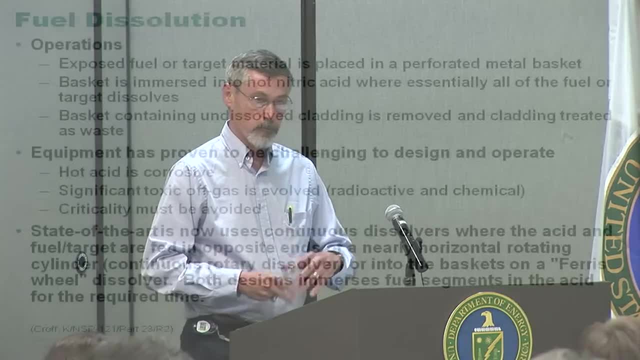 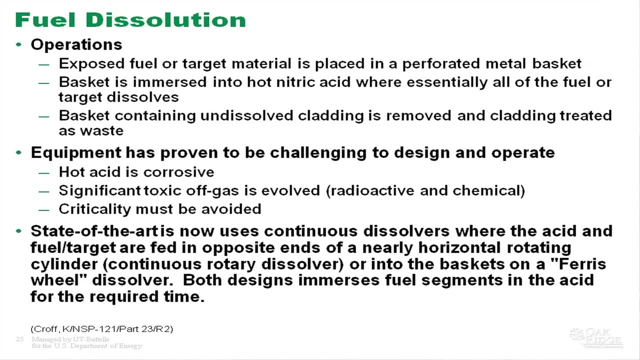 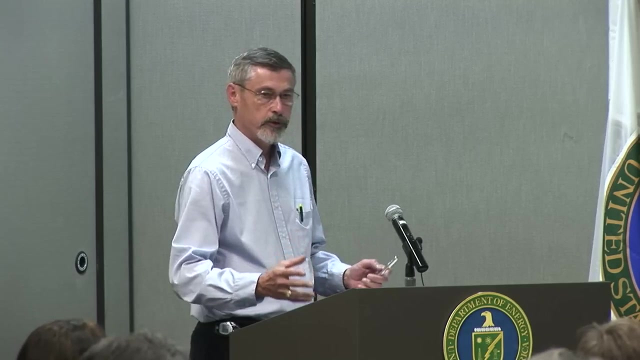 Both designs immerse the fuel in the acid for the required amount of time and then allow you to separate them and distribute those solids from a liquid stream. But you can operate these in continuous rather than the basket mode. In the basket operations you tend to have multiple baskets. 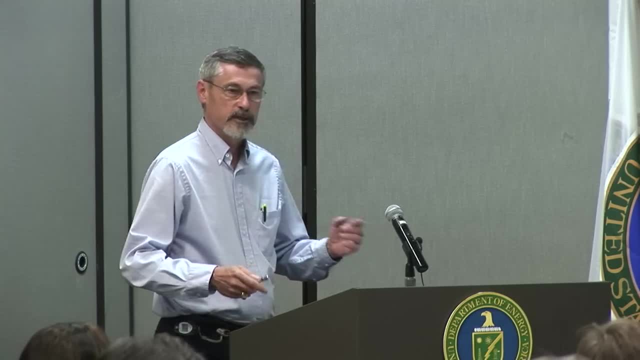 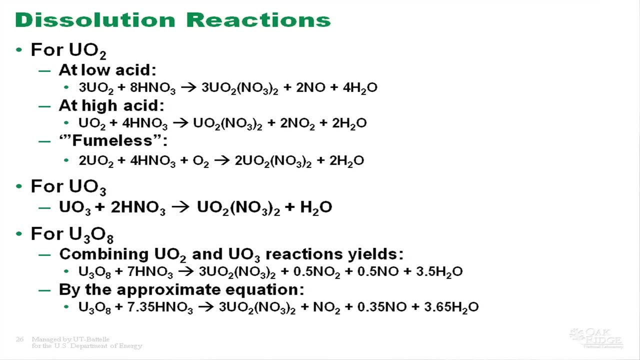 or multiple dissolvers in the plant. A little chemistry. Everyone wants a little chemistry early in the morning. For the dissolution of UO2, this would be in the case of non-vol oxidation At low acid. this reaction applies At higher acid. 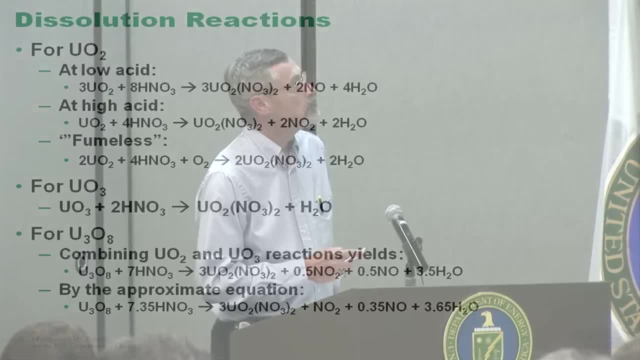 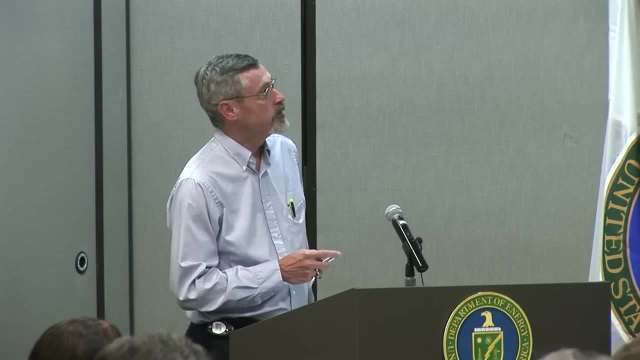 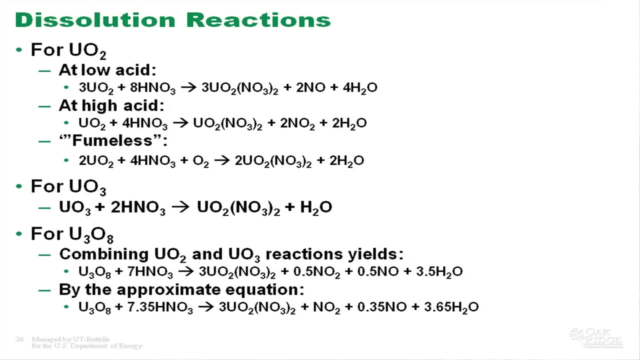 you'll note that you use maybe a little more acid in this case, but the important number to look at is how much of this acid ends up as NO2 or NO. Half of the nitric acid here ends up as NO2.. That's going up the stack. 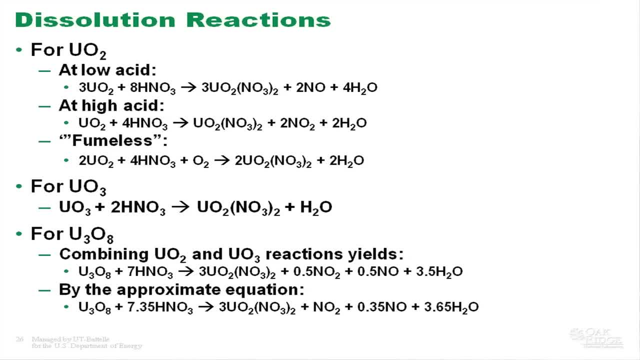 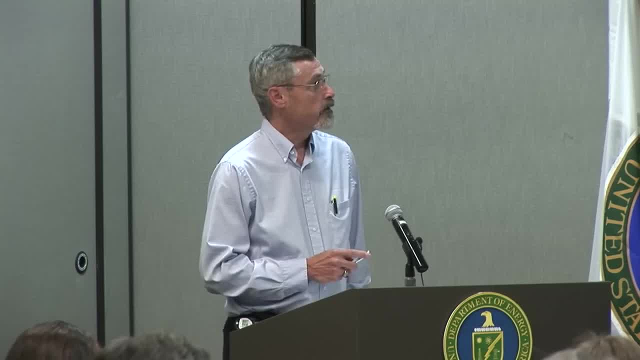 And water. Here about a quarter of the acid is consumed. If it's not recovered, it's just lost the stack. One could add oxygen to the dissolver. If one does that, you have what's called fumeless dissolution. 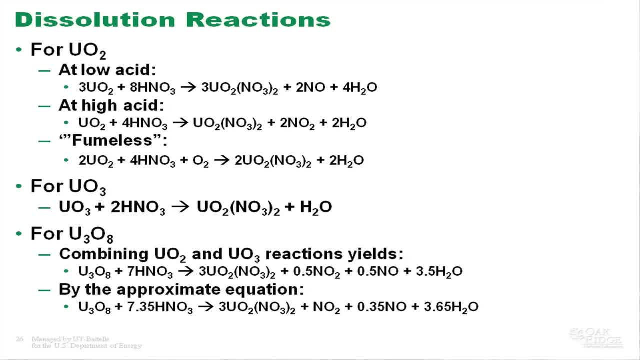 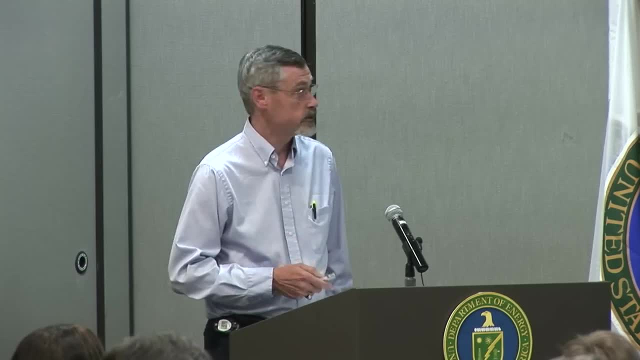 It's called fumeless because this there is no NO or NO2 produced. In reality, this reaction tends to dominate below 10 molar nitric acid. but both reactions occur simultaneously, It's just they have different rates If we have voloxidation. 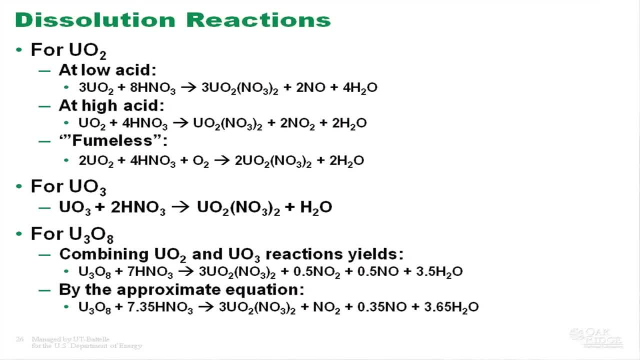 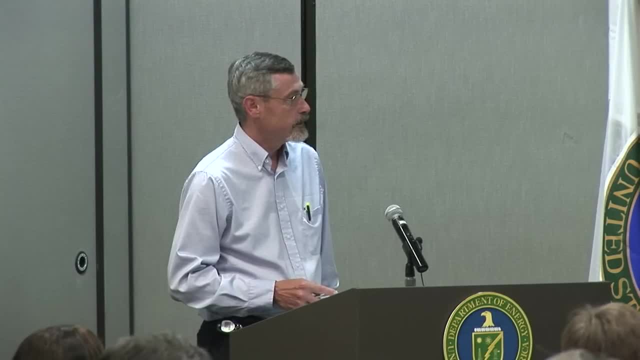 and you oxidize the fuel all the way to UO3, you can also have fumeless dissolution, but the product in all cases is a uranyl nitrate For U308, the product from voloxidation. this reaction is sort of 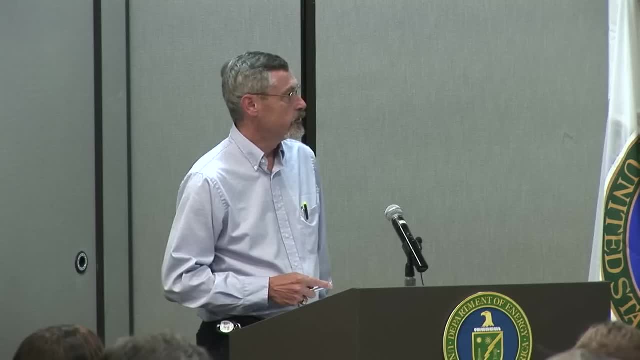 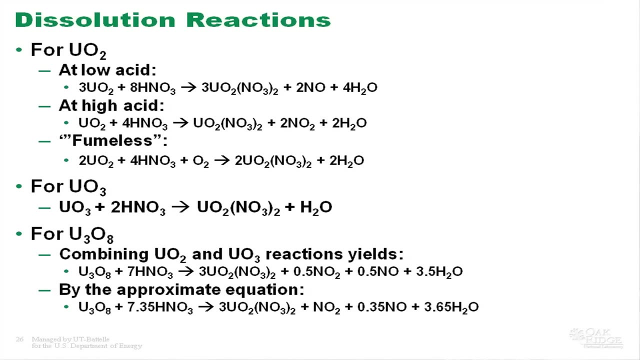 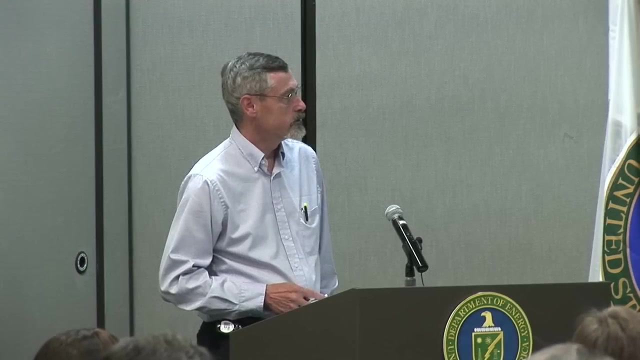 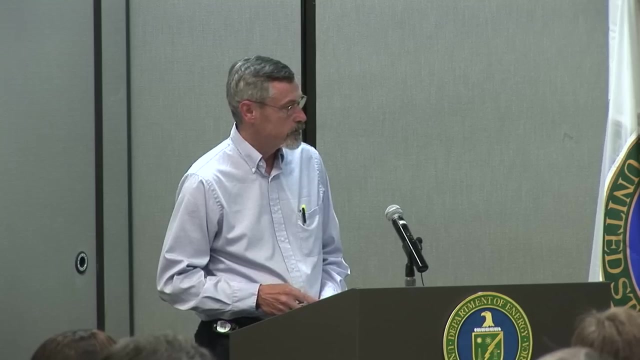 these are both sort of pseudo equations. This reaction is the same as the sum of that equation, that equation and eight times this equation and magically you have this reaction. This reaction is developed out of experimental observation of the process. You'll notice if you look at the material balance on this carefully. 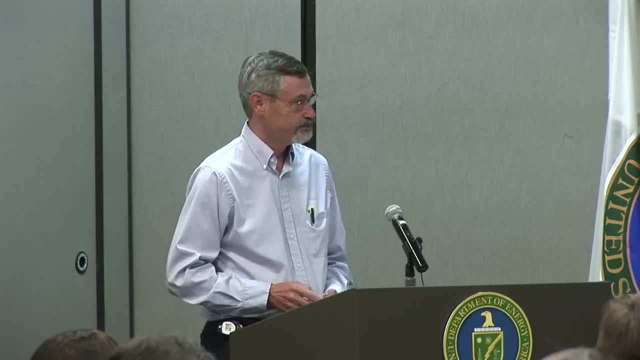 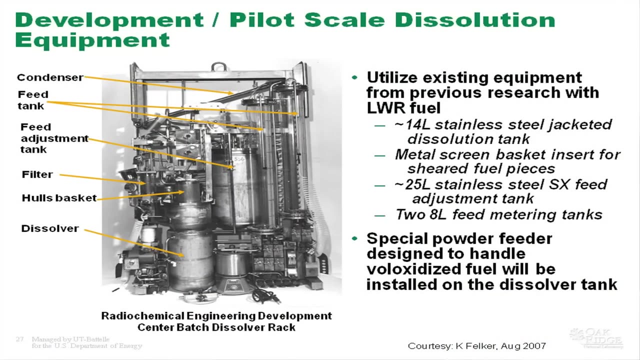 and try and balance that equation. it doesn't quite balance. What's this equipment look like? This is the photograph of a small-scale dissolver located at Oak Ridge in the Radiochemical Engineering Development Center. This is the dissolver itself. It's a 14-liter dissolver. 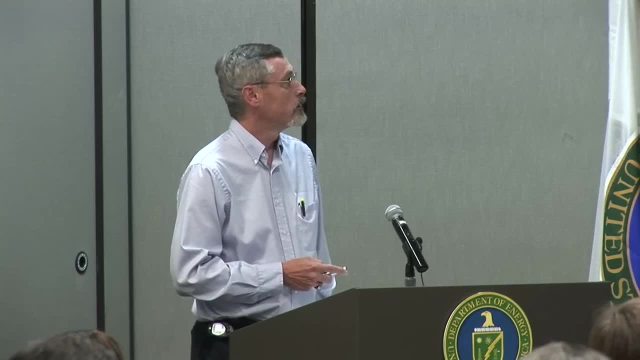 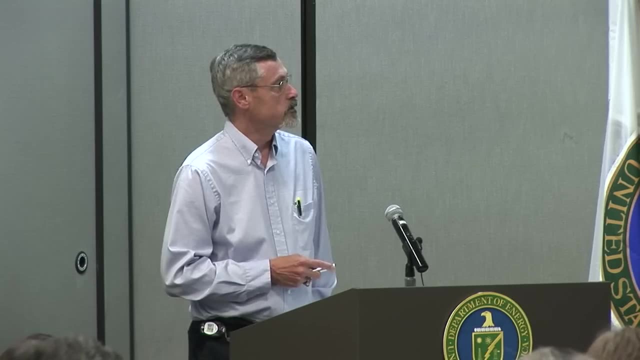 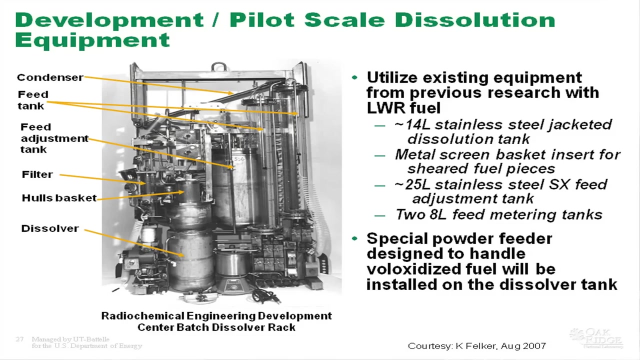 We process in this kilogram quantities of fuel. Here is that Hall's basket. There's a filter for taking the solution from the dissolver. These tanks are feed tanks then for doing feed adjustment and feeding to the subsequent solvent extraction process. This rack is about three feet across. 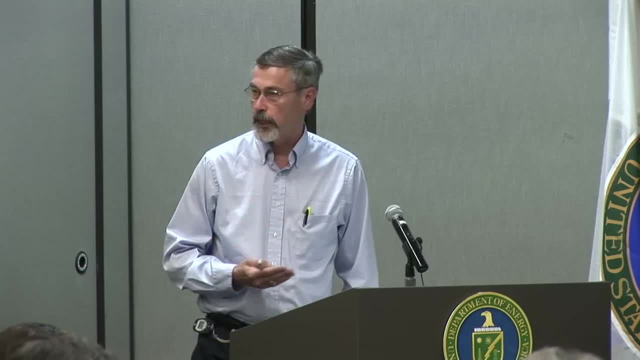 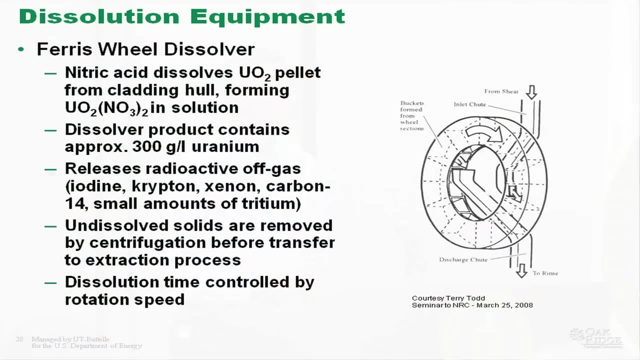 and about six feet tall, just to get an idea of size for kilogram quantities of processing The Ferris wheel. dissolver, in this case what you have in a batch dissolver. you feed a quantity of nitric acid into the dissolver vessel. 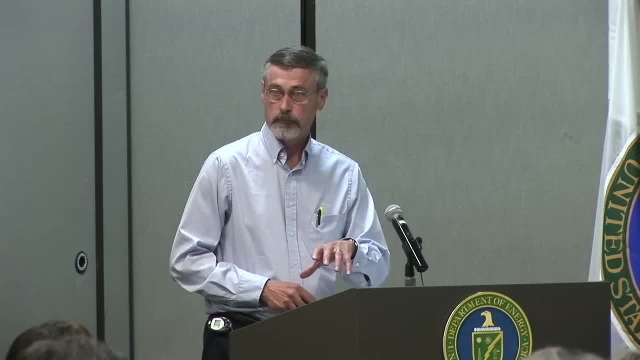 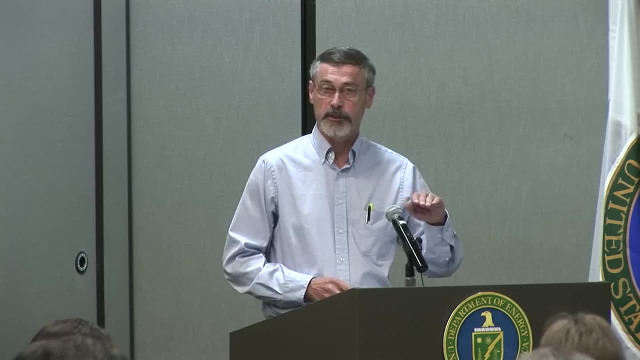 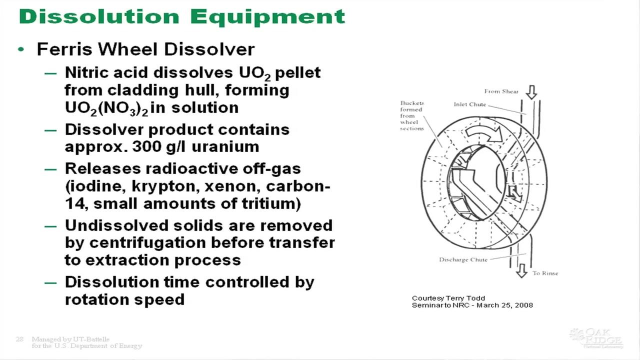 and you add your uranium oxide to that, What happens is you start with a fairly high concentration of nitric acid. Those reactions, what you saw in those: the nitric acid is consumed, producing the uranyl nitrate. The acid concentration is constantly going down. 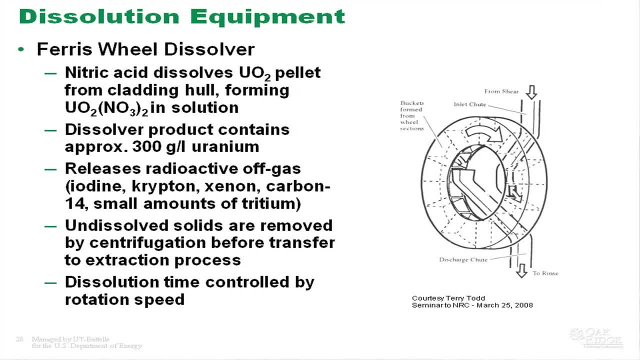 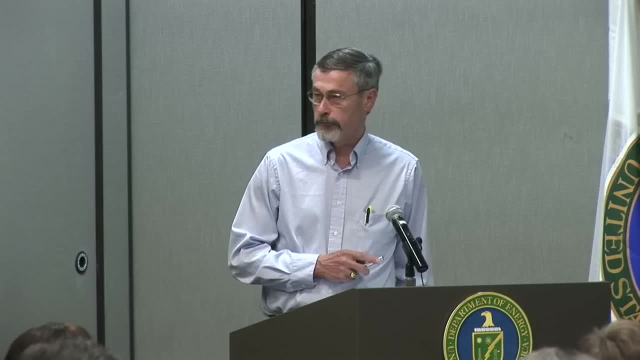 as the dissolution process proceeds In a Ferris wheel dissolver, you have what's not shown here. This is encased in another vessel. You have a bath of nitric acid here. That is now a continuous process and that nitric acid concentration stays constant. 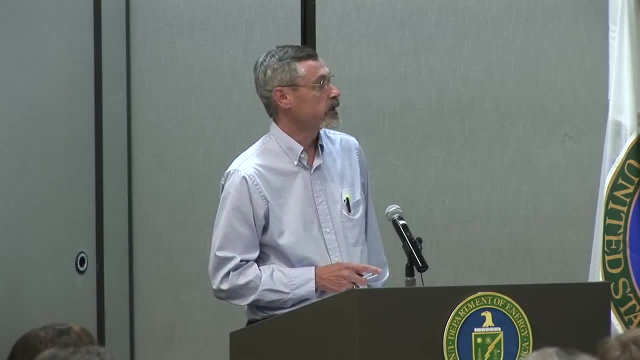 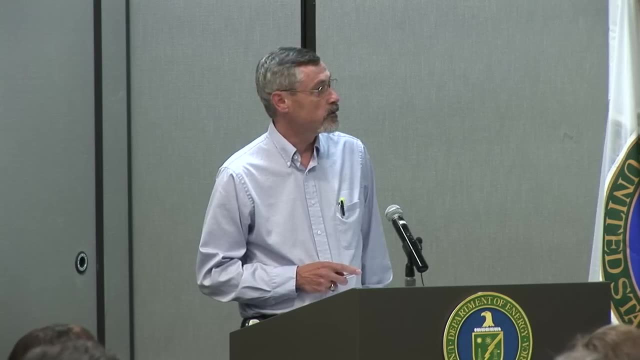 You have constant addition of nitric acid and constant withdrawal of the nitric acid. The fuel is fed in through a chute and it's captured in a chamber of this Ferris wheel. The Ferris wheel is turning this direction. It comes in. 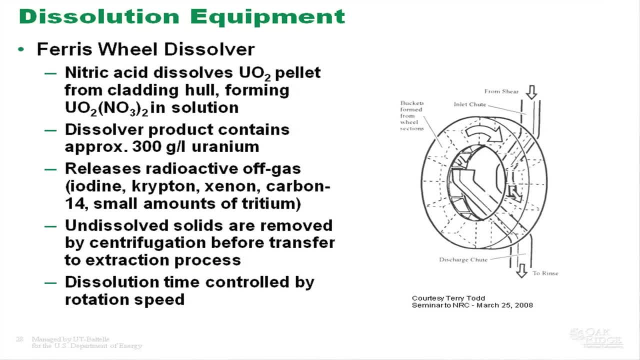 and it's immersed into the nitric acid. The amount of time it's in the nitric acid is controlled by the rotation rate of the Ferris wheel. At some point the fuel is dissolved out and the hulls continue to proceed up in each of these chambers. 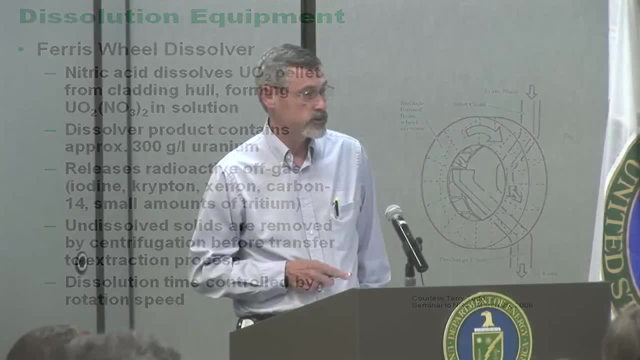 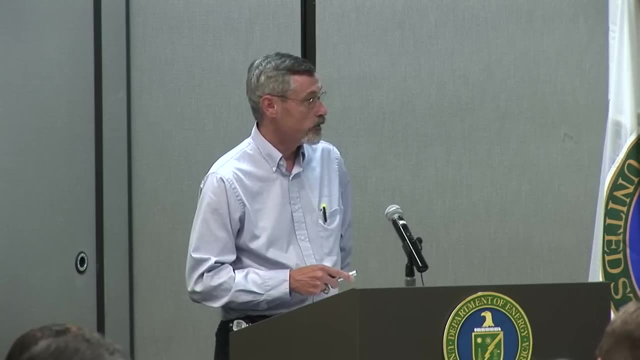 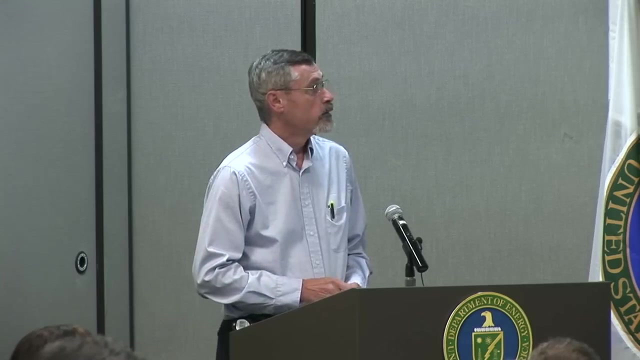 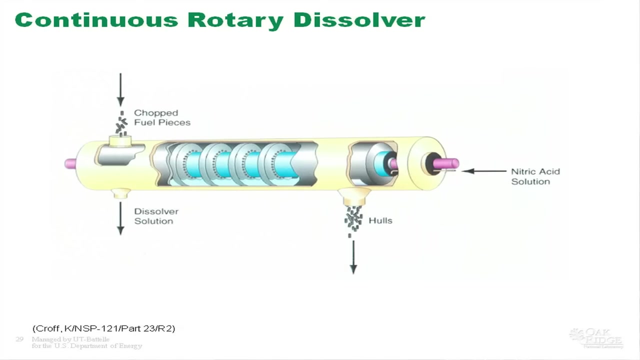 until finally they slide out and are discharged down this chute for the capture of the solids. So dissolution time in this case is controlled primarily by the rotation speed or the nitric acid concentration. Next slide: Okay, The continuous rotary dissolver is in a way very similar to that. 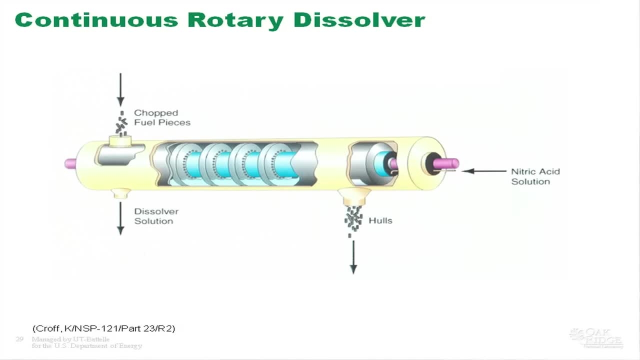 except that in this case this is an enclosed chamber. This chopped fuel is fed at one end, Nitric acid solution is fed at the other end. The fuel stays between these two rotary flights. It's basically a screw down the center of this. 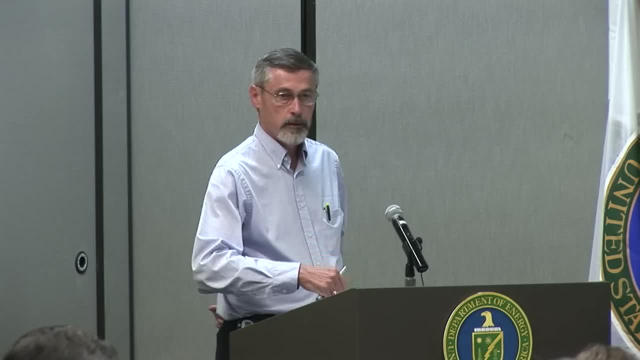 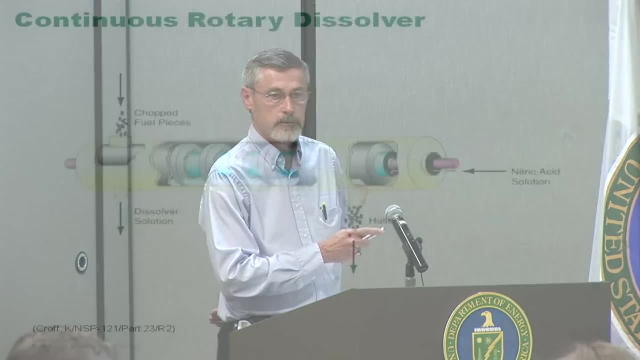 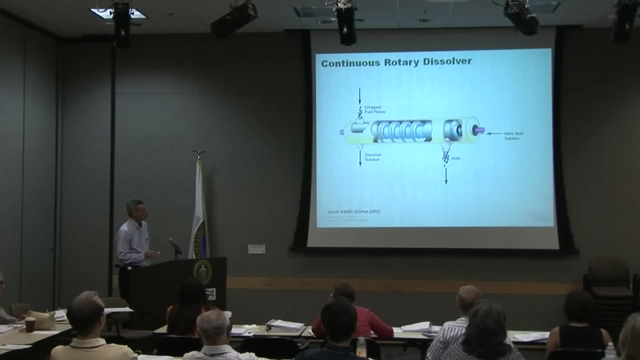 This is rocked back and forth for a period of time, Then it's turned one complete rotation. This advances the fuel from this end to this end, step by step. The nitric acid is flowing in here. As the fuel advances, it's seeing higher and higher concentrations of nitric acid. 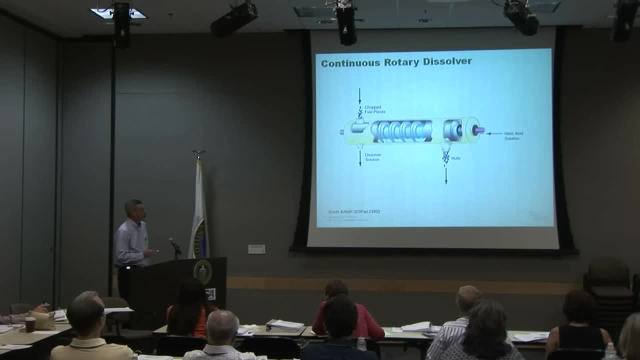 The bulk of the dissolution takes place down at this end. The harder-to-dissolve material moves this direction. It sees the higher nitric acid concentration because the acid has not been consumed by the dissolution process. The acid continues to flow down. It sees higher and higher quantities. 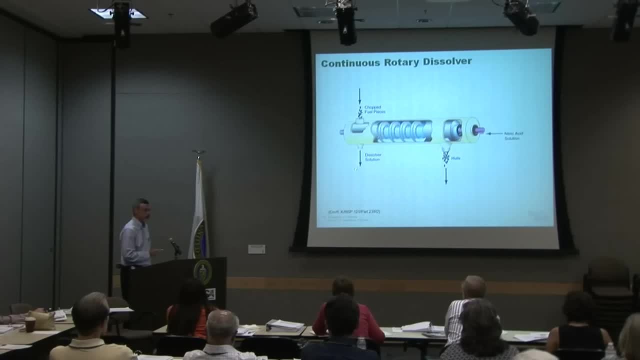 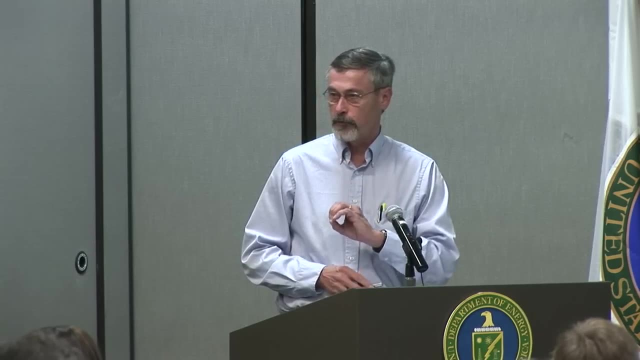 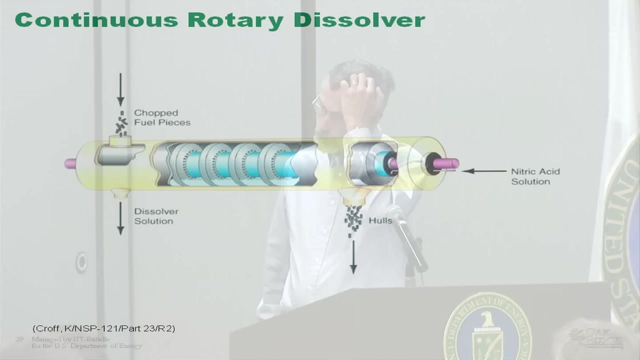 of uranium and plutonium dissolves those and the dissolver solution finally leaves here. The advantage of this is that you have the most difficult-to-dissolve materials, are seeing the most concentrated nitric acid. Excuse me, Terry, What's all this made out of? 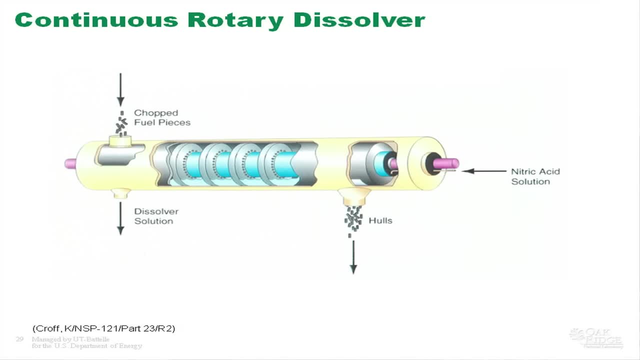 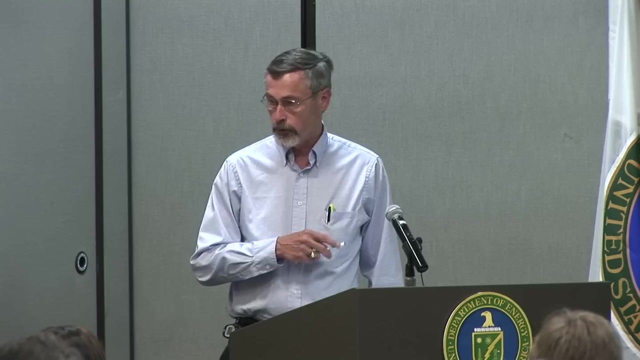 Last slide. No, this is primarily made out of stainless steel- Stainless In this case. one of the things we installed in this is a. One of the concerns is certainly criticality, And we looked at putting a borated core down the center of this dissolver. 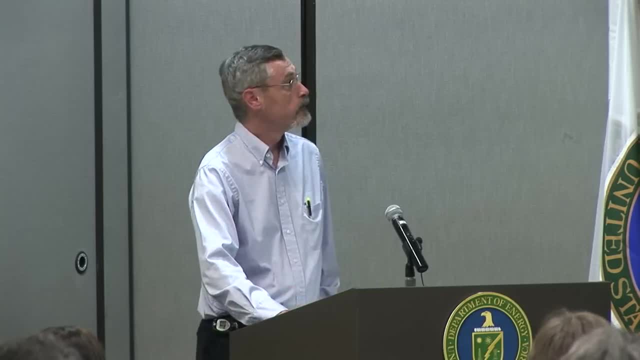 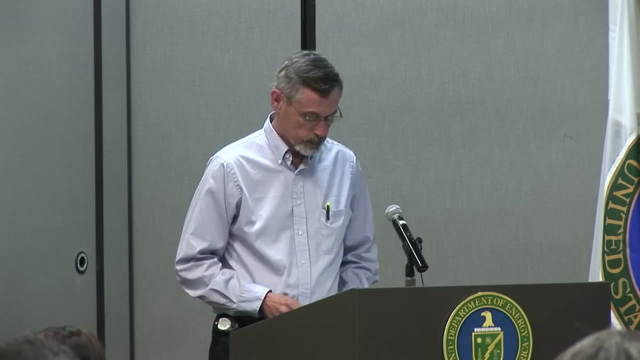 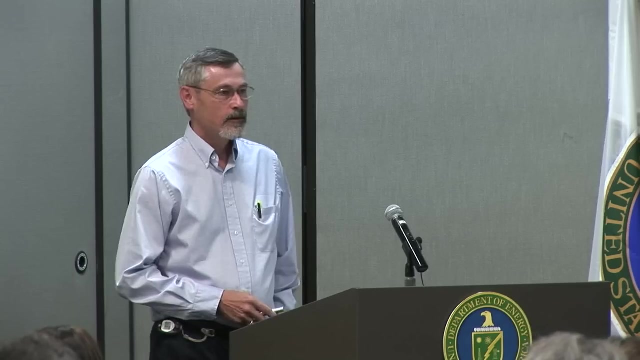 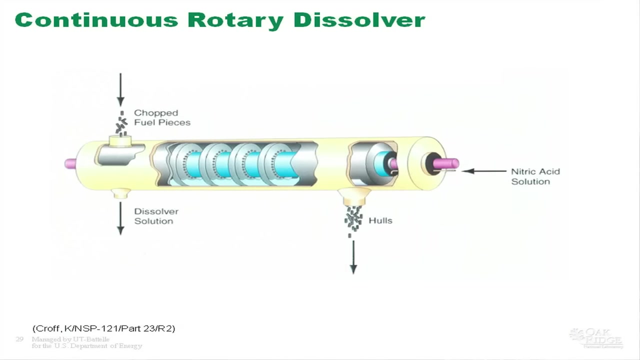 to deal with criticality issues. What is the size of the equipment that's all drawn on the board? It's about yay, big. It's about, Lengthwise, about three of the tables put together There. again, it depends on what you're looking for. 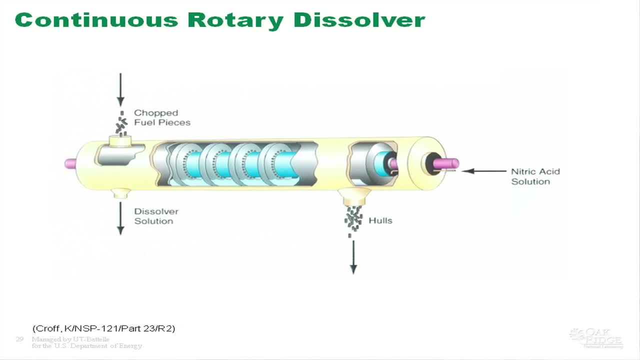 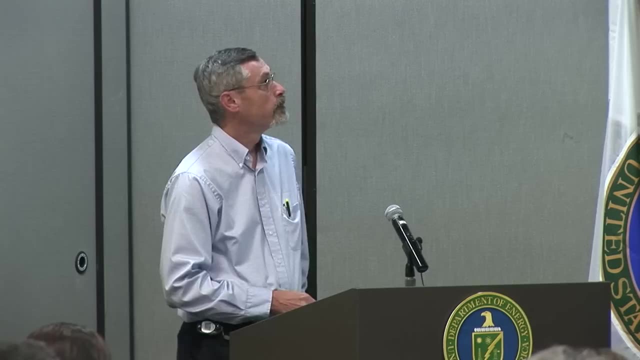 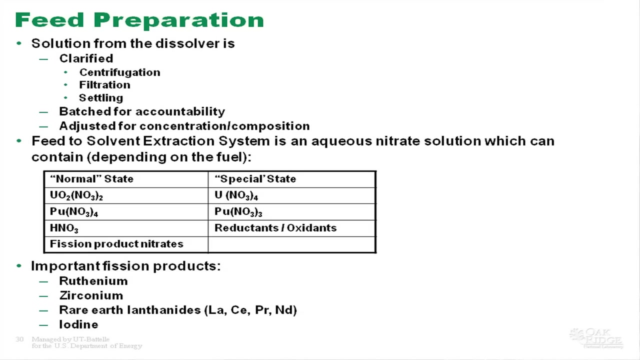 in terms of throughput, What I'm talking about is a unit that was designed for about a quarter of a ton per day. Well, once we've dissolved the fuel, the last couple of steps are to prepare that fuel, then for the solution for solvent extraction. 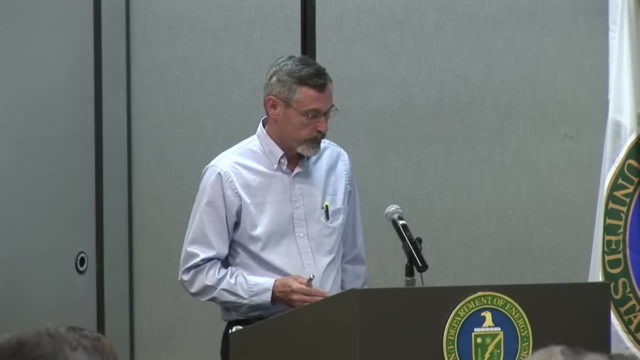 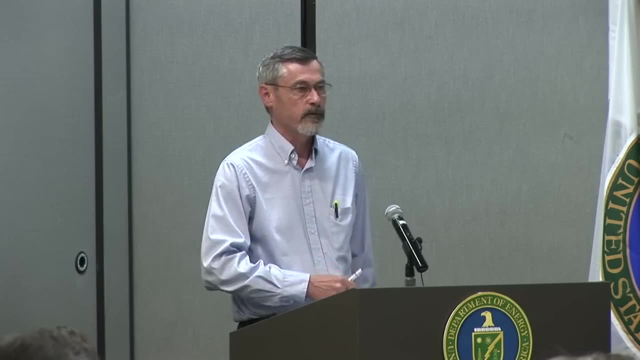 Well, what do we need to do in that One? we need to clarify it. There's material that you cannot dissolve. There could be some stainless steel fines. There could be some zircaloy fines that make it through the process and they're in the fuel. 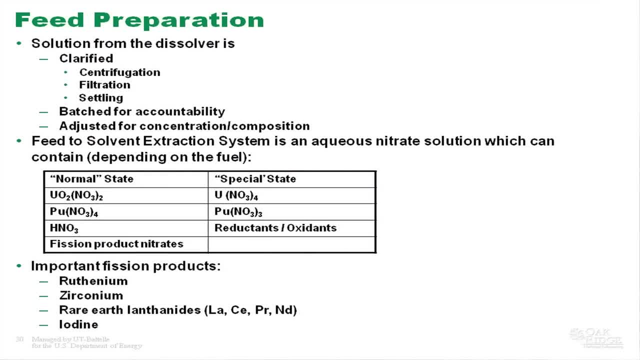 So you'll remove that by centrifugation or filtration, You will put it in a tank and you will do accountability. You're going to determine at that point exactly how much fissile material you have in the process. You have a known volume. 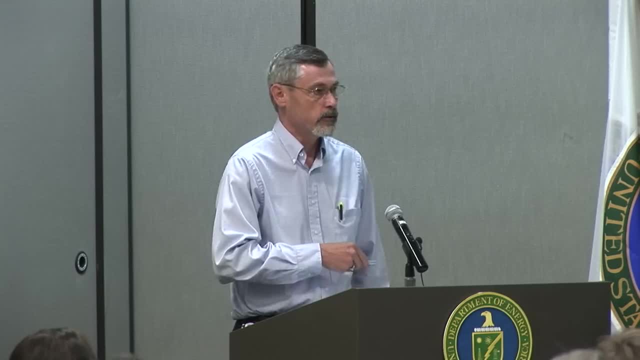 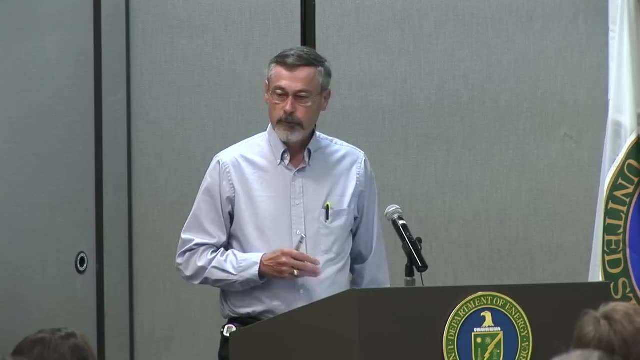 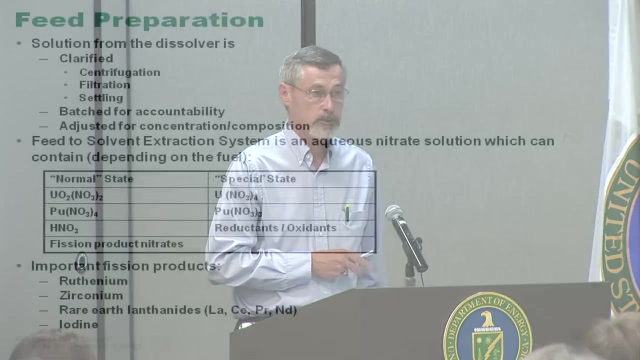 You take your analytical measurements and you do your first accountability at that point And you adjust then the material to get to the desired concentrations for solvent extraction and for the desired composition. You may change the valence state In the normal state, uranium's in the plus six. 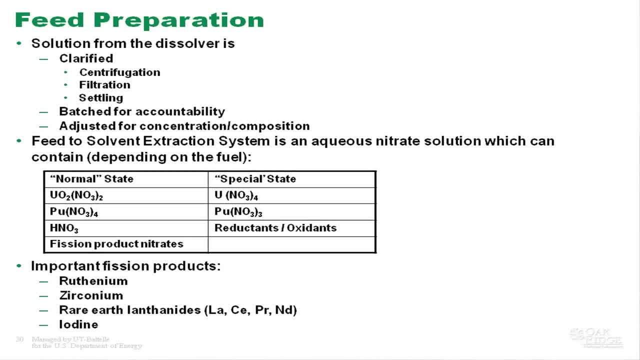 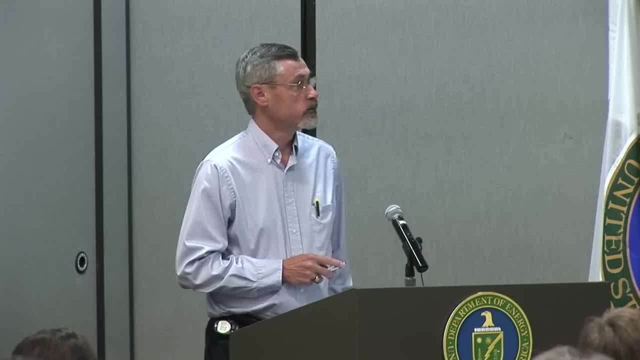 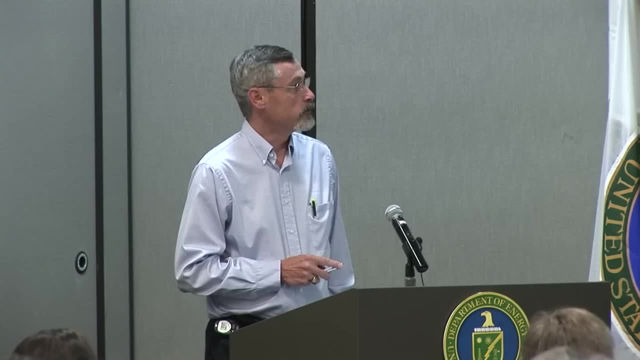 plutonium's in the plus four, You'll have nitric acid and you'll have your fission product nitrates. You may add some uranium-4 as a reductant. You may have your plutonium reduced to a PU-3 state. 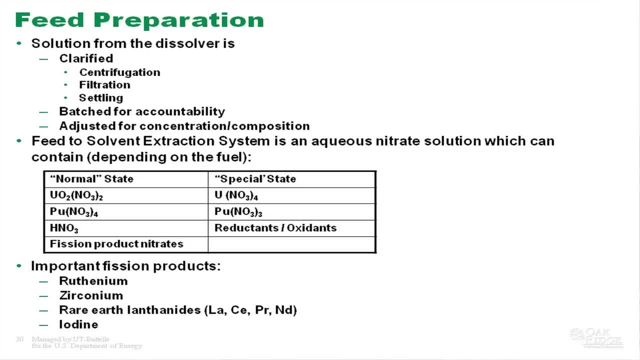 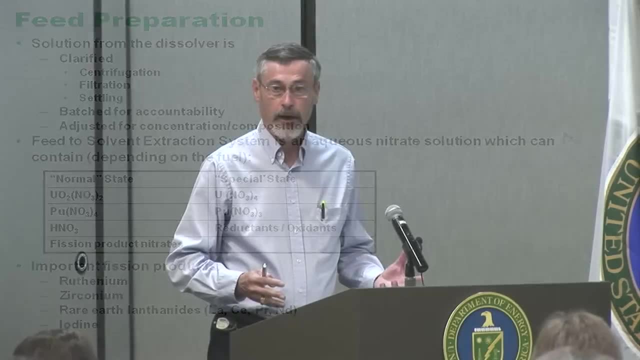 You may add other reductants and oxidants to adjust the chemistry depending on what you want to do in solvent extraction. This solution contains all the important fission products: Lithenium, zirconium, rare earth, lance and iodine. These are the things you want to get out of it. 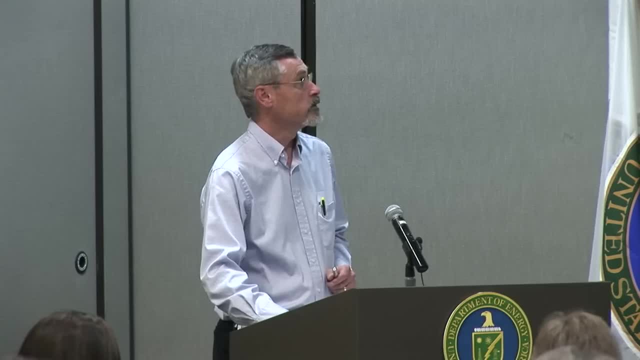 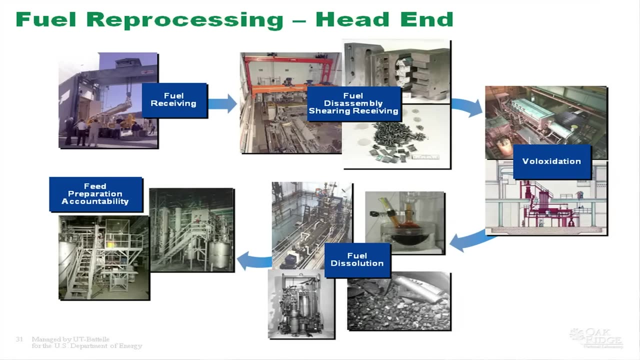 You want to recover that uranium-plutonium and strip away everything else. So a bunch of pictures of what the head end looks like: Fuel receiving. There's a dissolver. There's a shear. There's that biloxidizer. Here are various dissolvers. 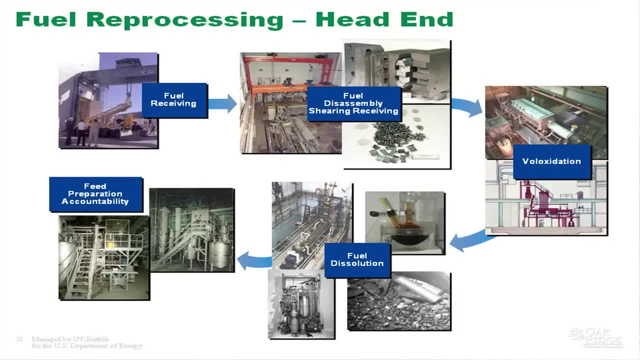 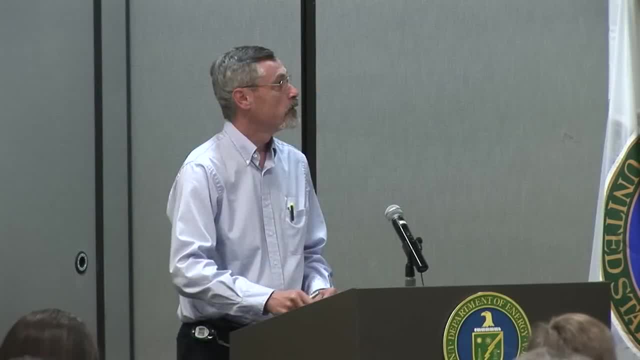 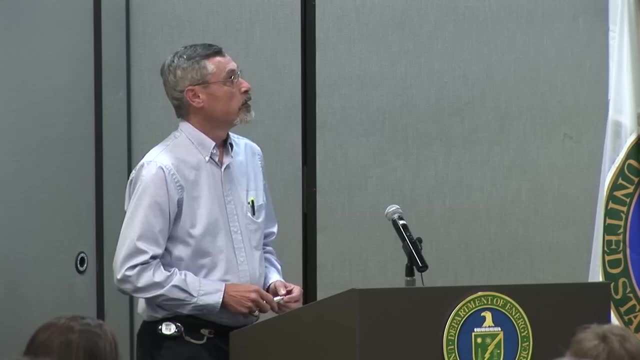 There's a picture of that large dissolver And accountability equipment. It looks like tanks- All stainless steel, primarily. So now we'll turn to the solvent extraction portion. Basics of solvent extraction. You're going to contact two immiscible liquids. 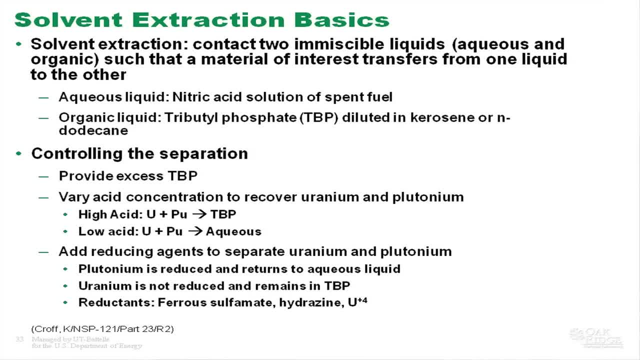 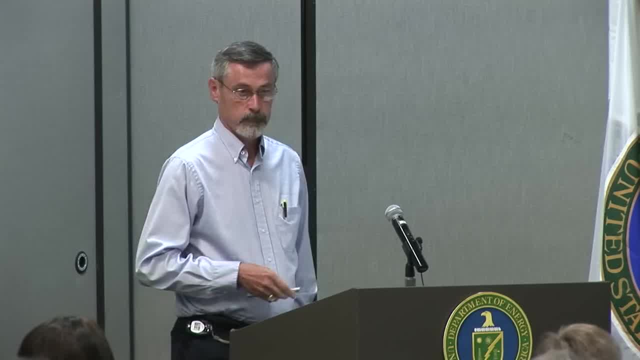 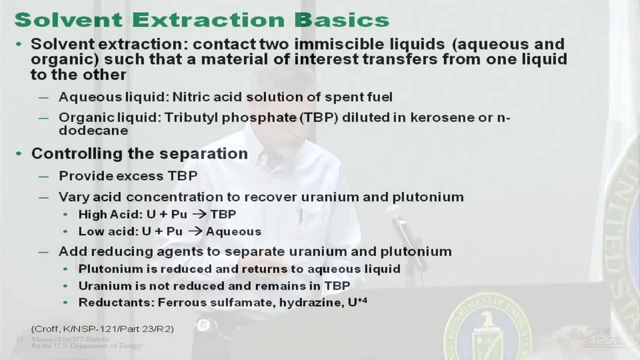 an aqueous organic typically, such that the material of interest transfers from one phase to the other and then you move it back. So typically in this case our aqueous phase is nitric acid and the organic phase is tributyl phosphate and kerosene or endodecane. 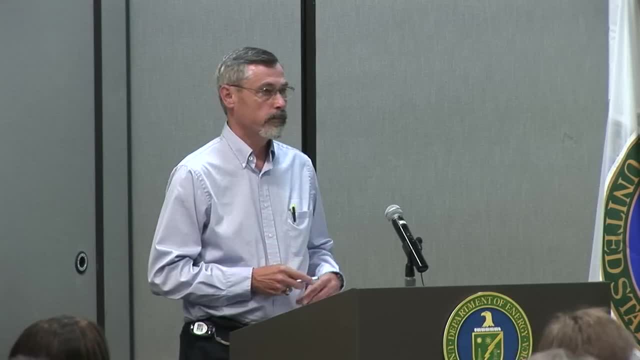 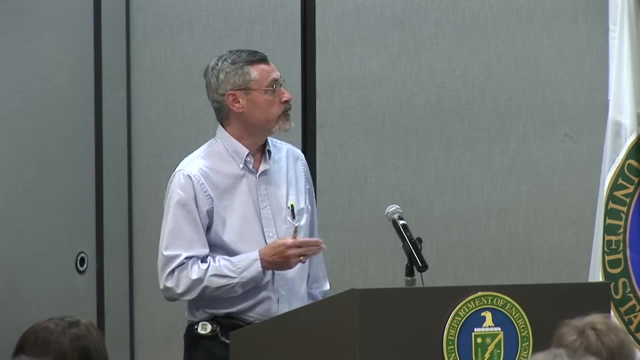 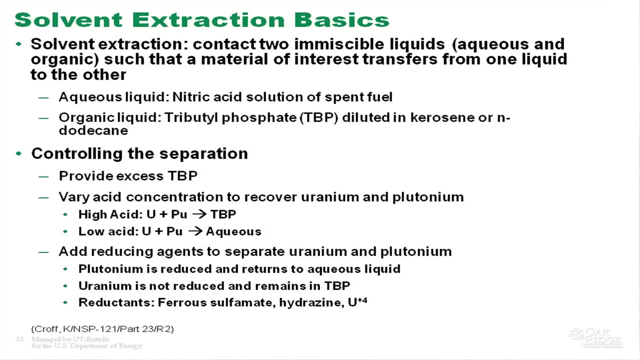 And we control the degree of separation by having excess TVP. We vary the nitric acid concentration to drive the process to either strip, to extract one of the species or to strip it out of the organic phase, And then we add reducing agents to allow separations of uranium and plutonium. 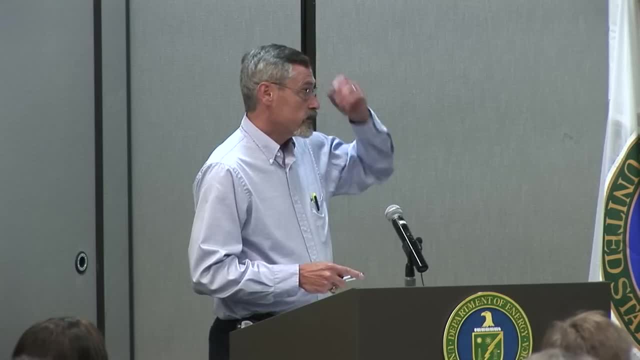 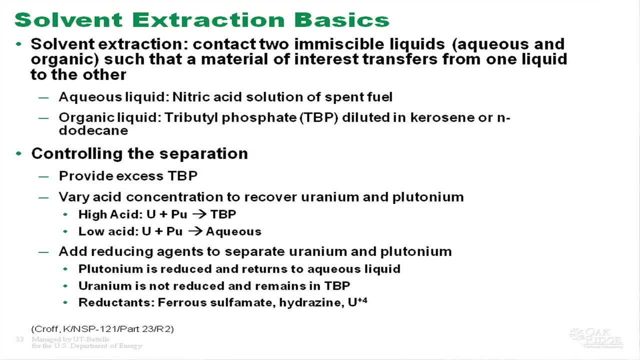 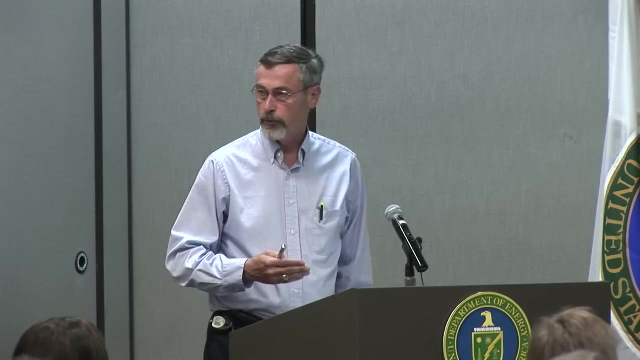 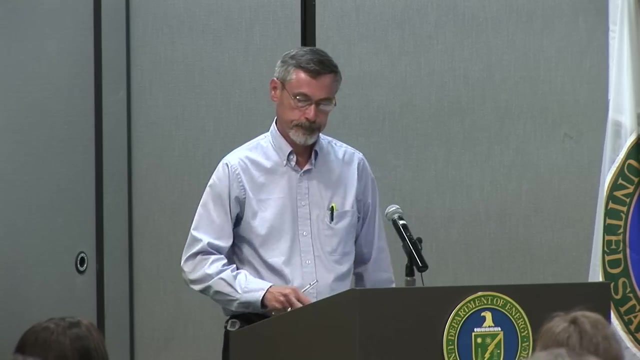 Various reductants: ferrous sulfamate, hydrazine U4.. Ferrous sulfamate results that ferrous ion and sulfur ion ends up in the waste stream. These two you end up with no additional waste products. It will be destroyed. 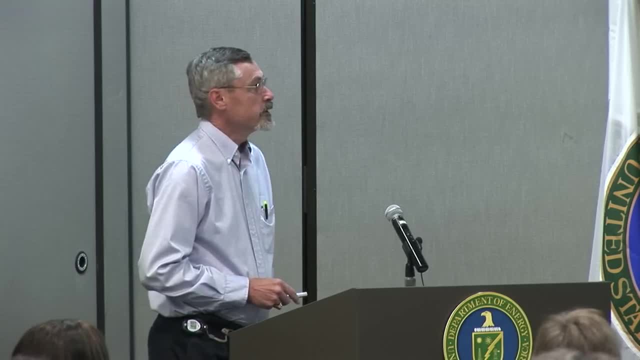 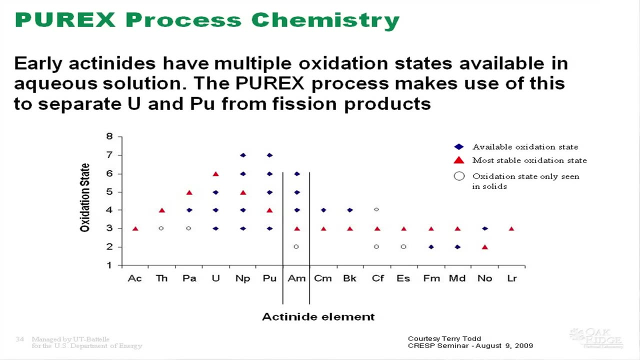 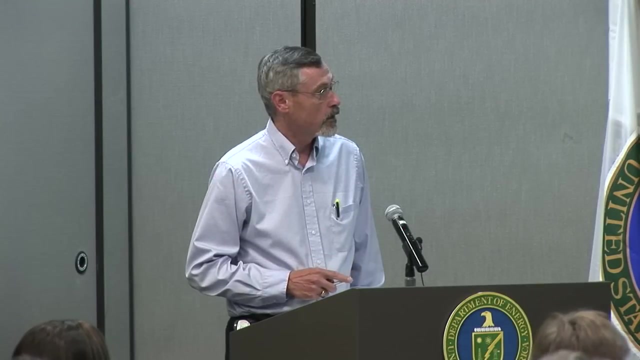 Valence states. The whole game of separations tends to revolve around the valence states of the process. The PUREX process works because it extracts species in the valence state of four and six. The red triangles are the most stable oxidization states of the actinide elements. 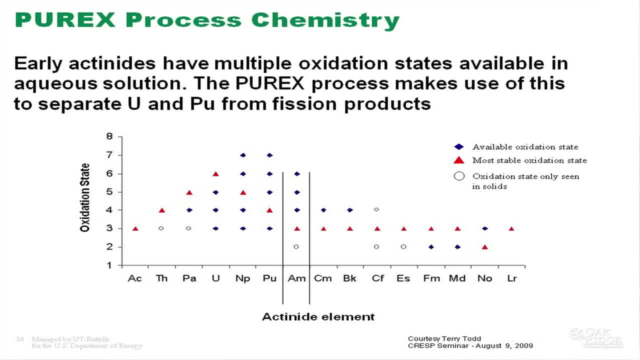 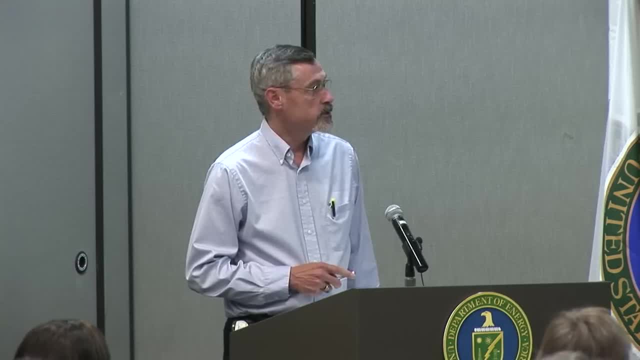 Here's uranium: It's in the six, Plutonium's in the five, Plutonium's in the four. Now you can, by changing the chemistry, drive these to other valence states. That's how we make some of the separations occur. 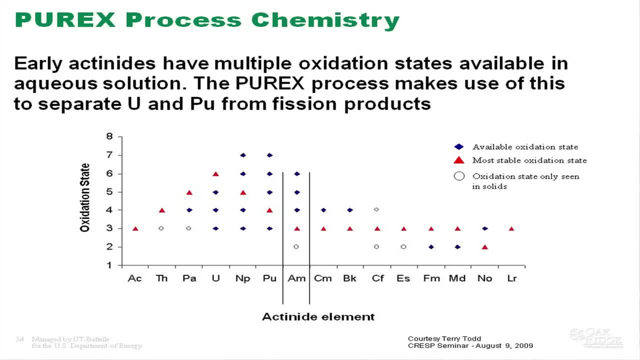 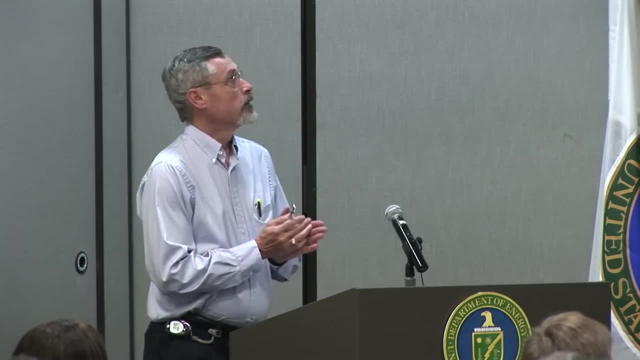 Notice that all of the higher actinides typically are in the three-oxidation state. They should not be extracted, And very few of them have other oxidation states that we can drive them to. All right, All right, so as a general rule, 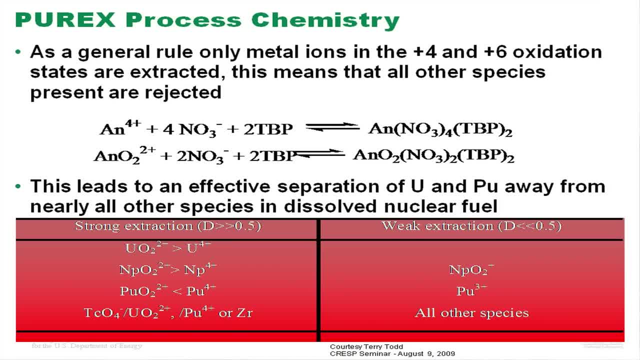 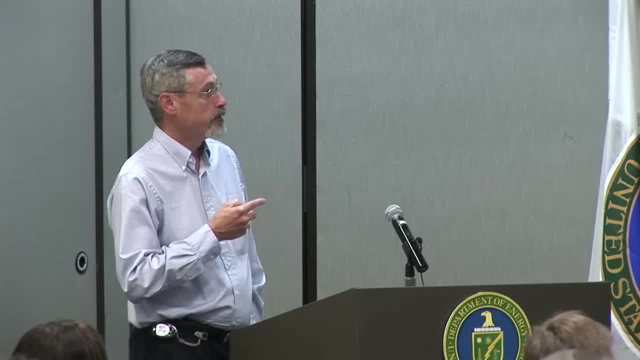 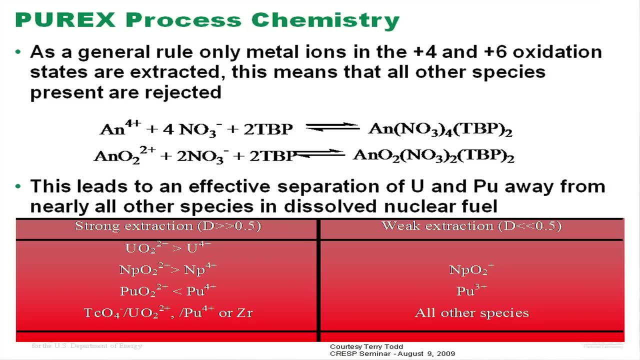 only four and six are extracted, And so when we extract those, they are complex with tributyl phosphate and, under the right conditions, are moved to the organic phase. I'll get to what distribution coefficients If it's a high number. 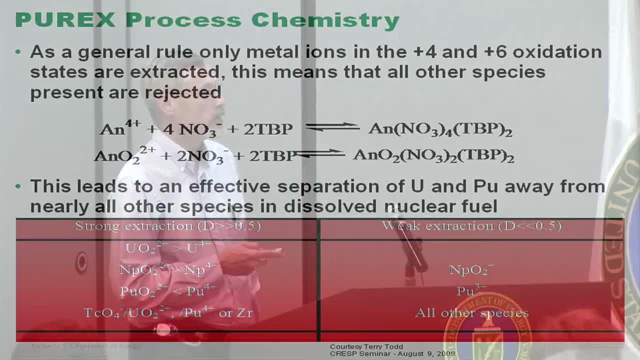 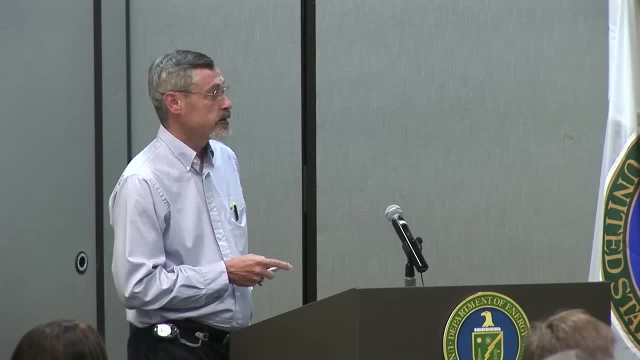 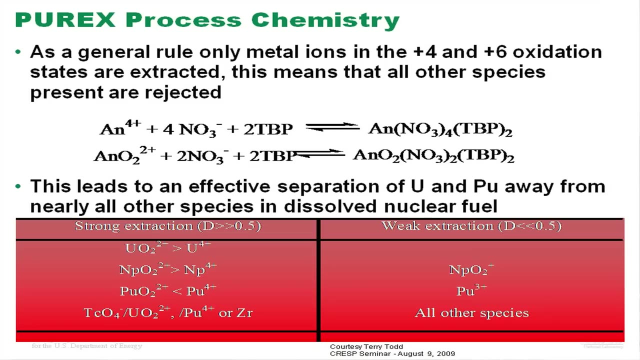 it tends to be extracted to the organic phase, A low number. it's not So. the U6 is more strongly extracted than the U4.. Neptunium 6, more than the neptunium 4.. Plutonium 6, less than plutonium 4.. 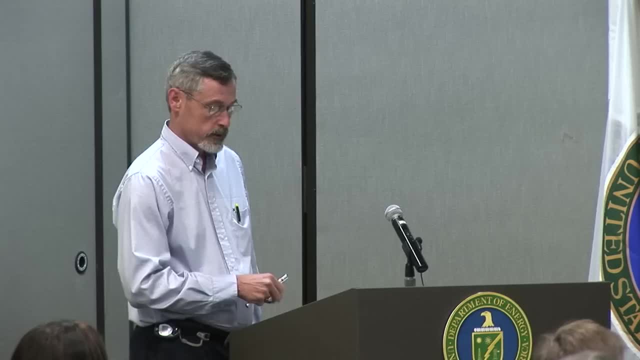 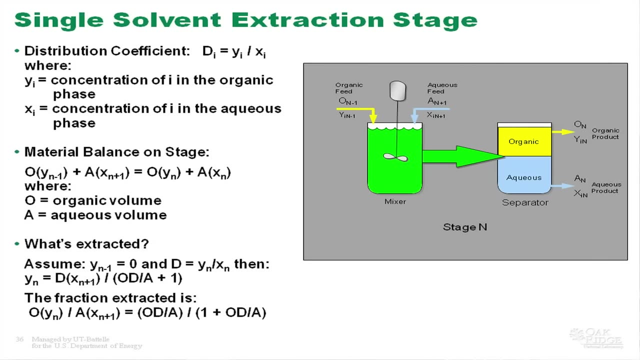 These species tend to be very weakly extracted. Well, not exactly chemistry here, but more material balance issues. A key term in solvent extraction is something called the distribution coefficient. Distribution coefficient is nothing more than the ratio of the concentration in the organic phase. 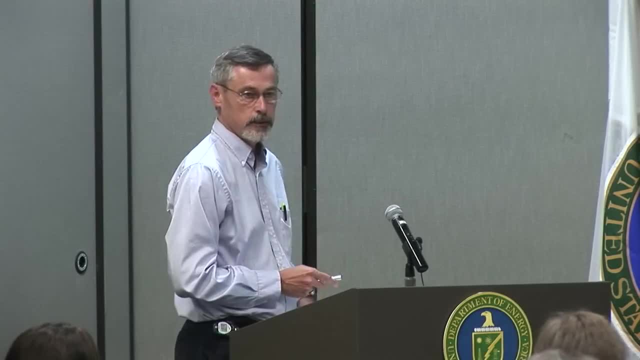 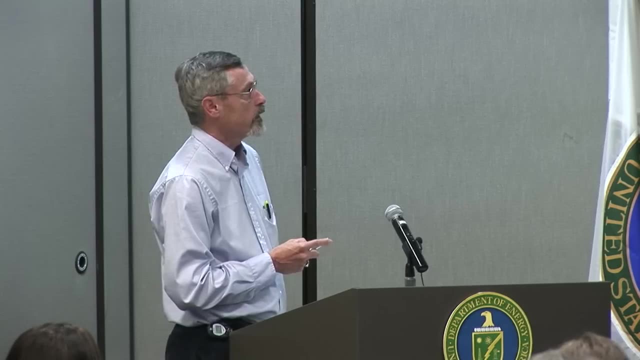 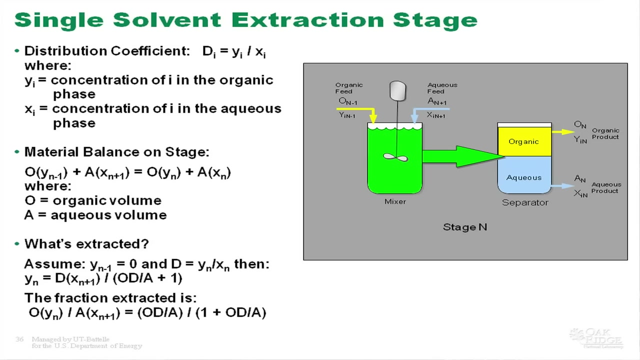 divided by the concentration in the aqueous phase. The higher the number, the higher the concentration in the organic phase. So with that one can write a material balance. around a given stage Coming in, you have a flow rate of organic And a concentration of organic. 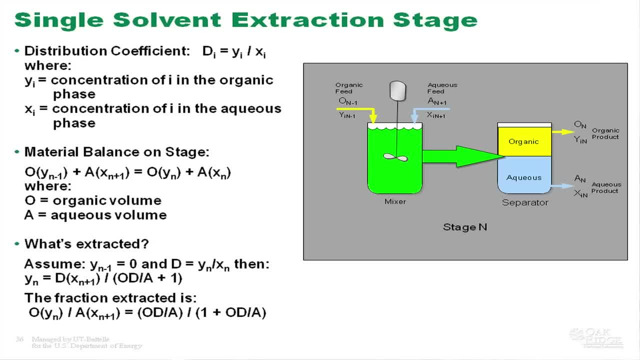 Of a species of interest- Let's say it's uranium. You have an aqueous stream and an aqueous concentration. Those are combined, They're intimately contacted and they're separated. So what comes in has to equal what goes out. If you do that, you can then relate that. 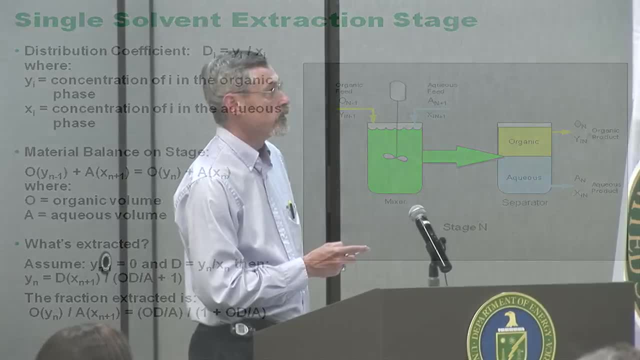 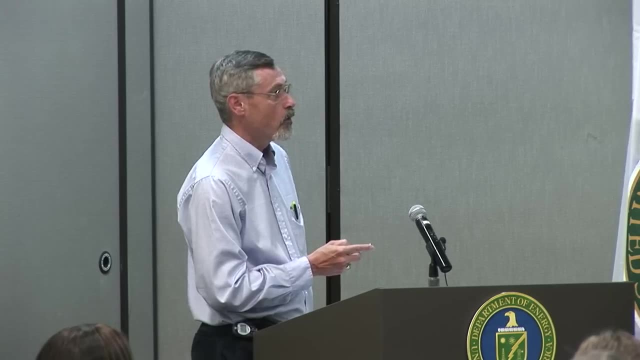 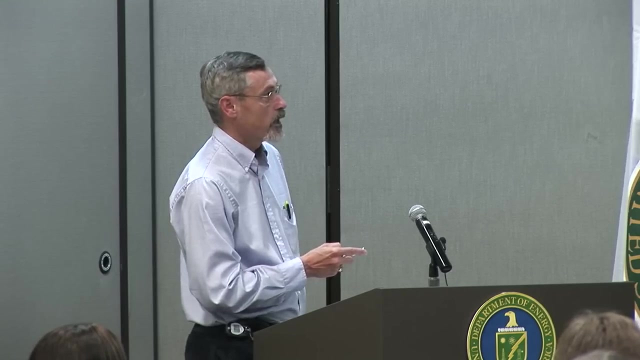 with the distribution coefficient. Let's assume for this case that there's nothing coming. there's no uranium coming in in the organic phase, So what is leaving in the organic phase here is nothing more than the distribution coefficient times, the phase ratios and the concentration of the organic coming in. 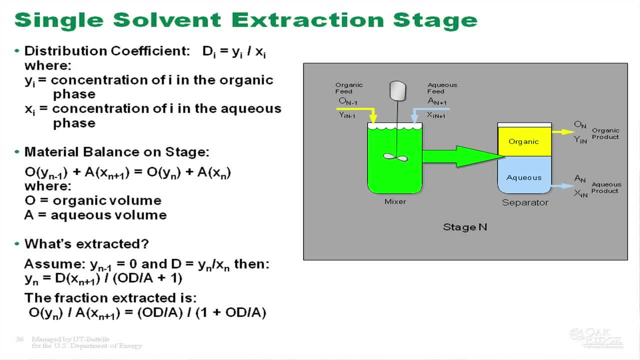 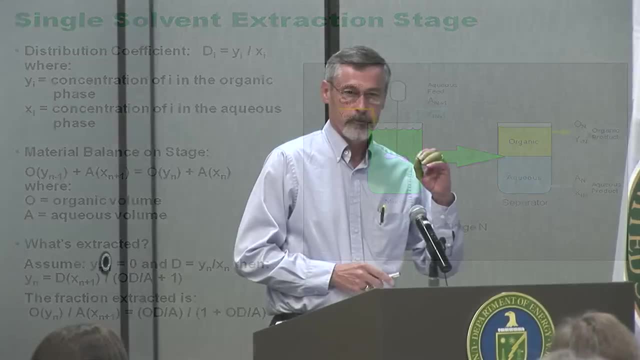 The fraction extractors can be expressed by this relationship. So do a little math, play a few games with this. If, let's say the simplest case, the distribution coefficient is 1 and the phase ratio is 1,, 50% of the uranium will go out with the organic. 50% with the aqueous. Pretty simple: If we take and double the distribution coefficient, what happens? More goes out with the organic phase. Precisely two-thirds will go out with the organic phase by doubling the distribution coefficient. It doesn't double, but it goes up to two-thirds. 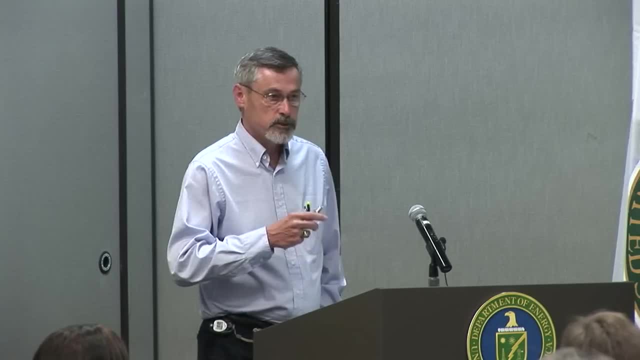 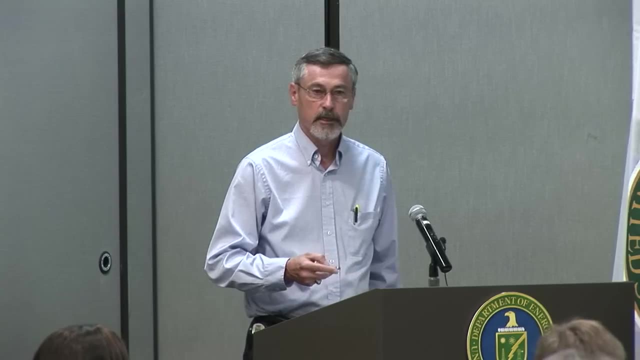 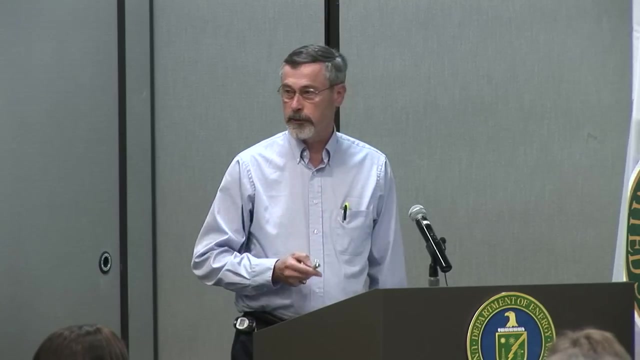 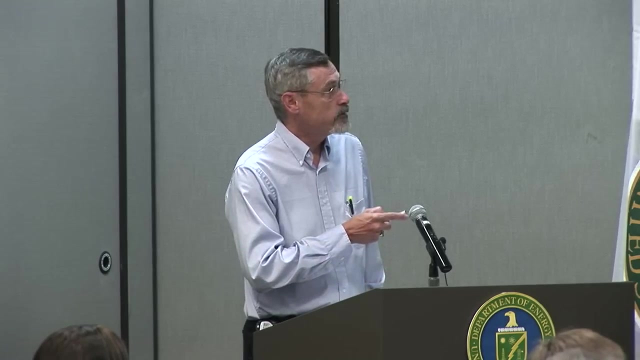 If, on the other hand, you keep the distribution coefficient at 1 and you double the phase ratio, the very same thing happens. You have two-thirds of the uranium goes out with the organic phase, but its concentration is cut in half. So you have some. 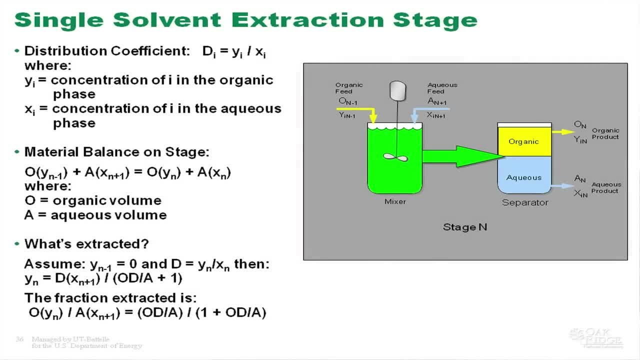 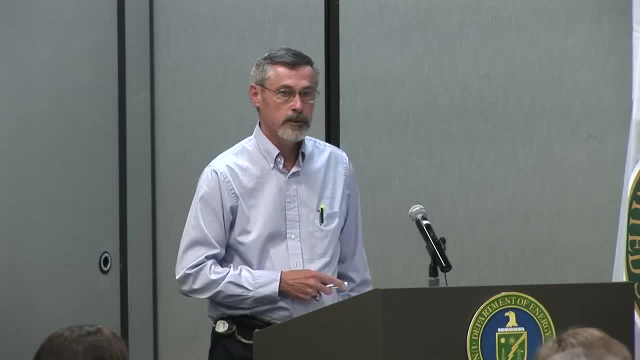 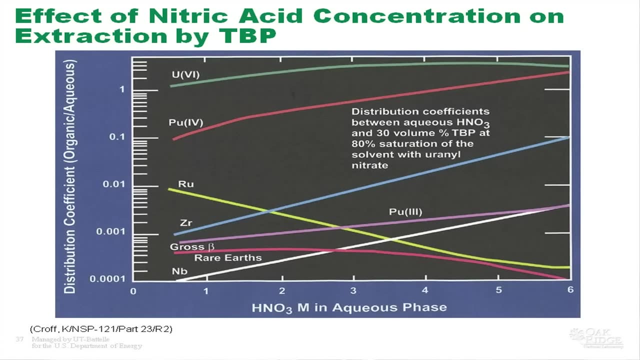 The chemist or the chemical engineer has some knobs to turn here. He can play with the flow rates, He can play with making some adjustments to the distribution coefficient, And he does that by changing the nitric acid concentration In the case of uranium-6,. 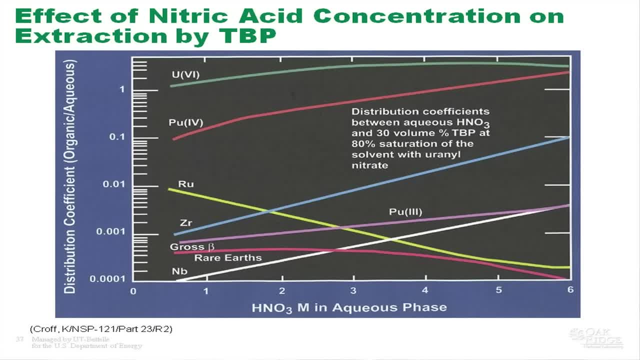 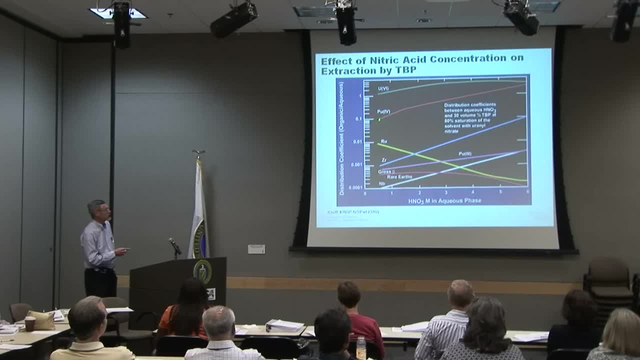 you see you have fairly high- This is a log scale- Fairly high distribution coefficients and acid concentration at both one mole, Plutonium goes from about 0.1 to above 1.. As you go from 1 mole to 6.9.. 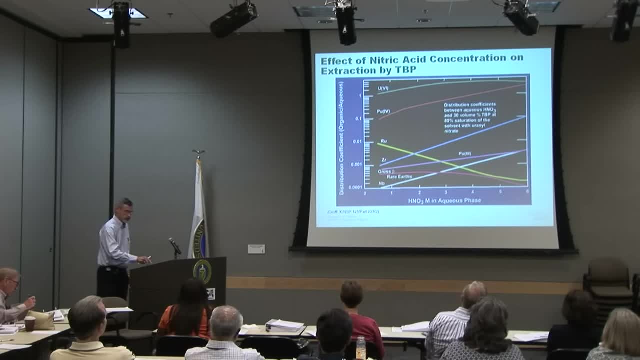 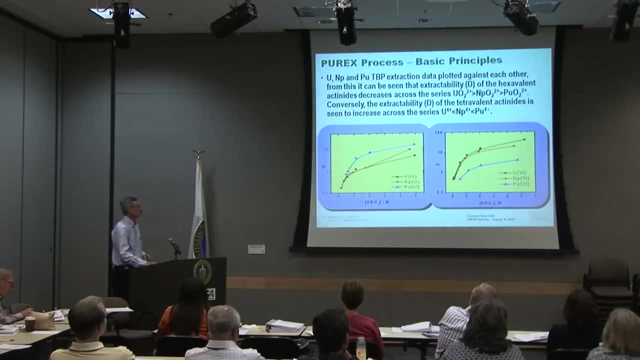 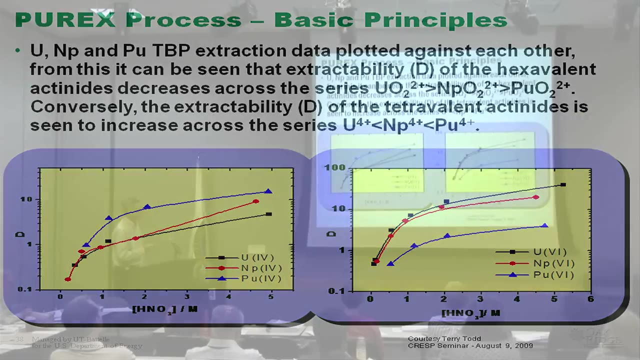 Notice how low many of these distribution coefficients are. They will not, They will extract, but a very small fraction of those will extract. This is sort of another way to look at that same curve, But here we're just simply comparing how those 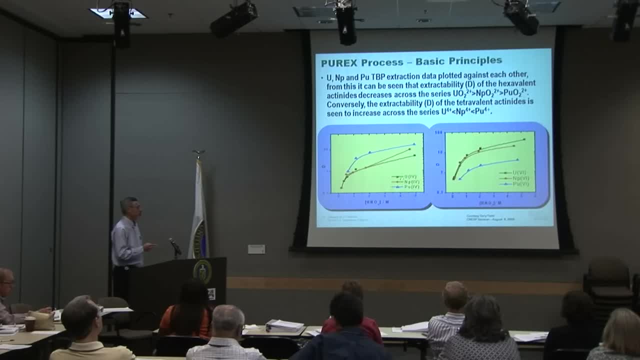 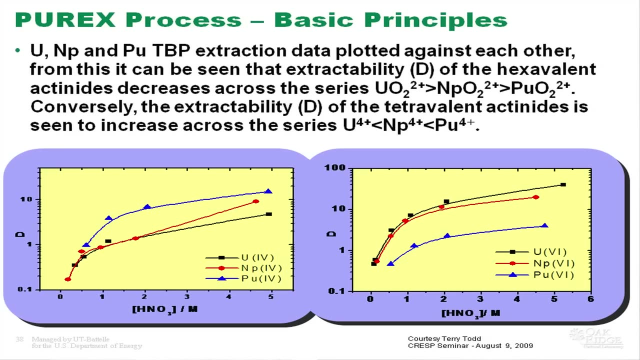 The uranium, plutonium and neptunium vary with oxidation state. So in the case of the oxidation state of 6, notice that the order is uranium-6, neptunium, plutonium. The oxidation state 4 is just the opposite. 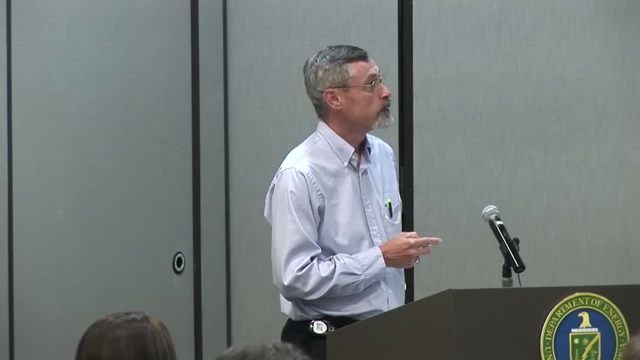 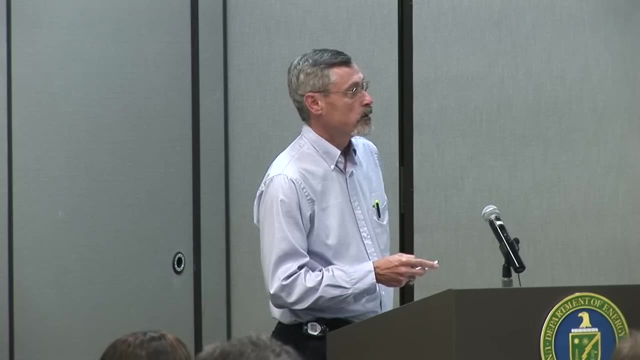 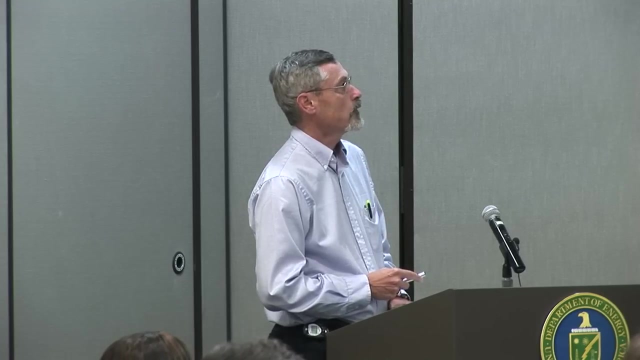 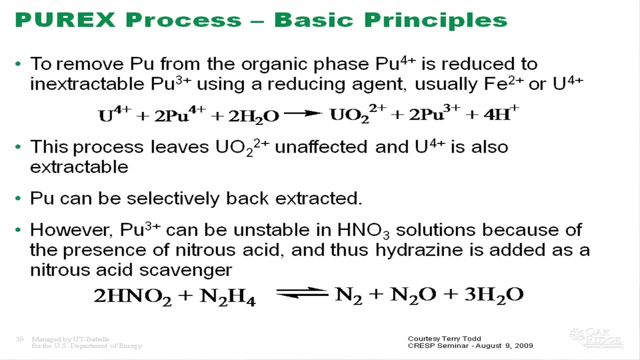 Plutonium, neptunium, uranium. Typically we're talking about extracting plutonium-4, uranium-4.. So to remove it, we extract the In the PUREX process, the classic PUREX process. you remove the plutonium. 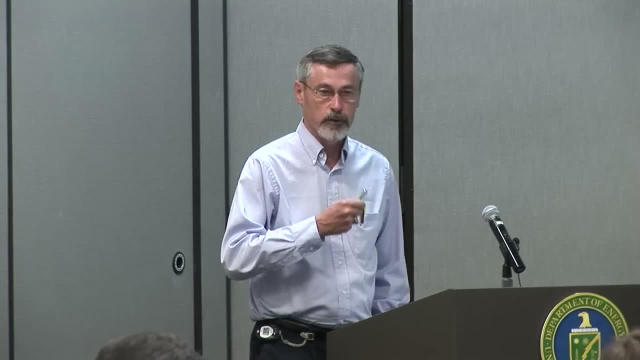 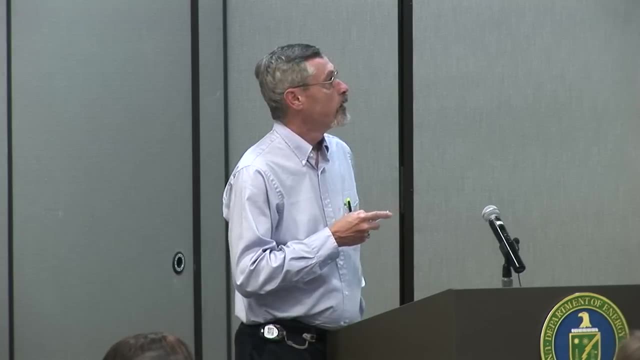 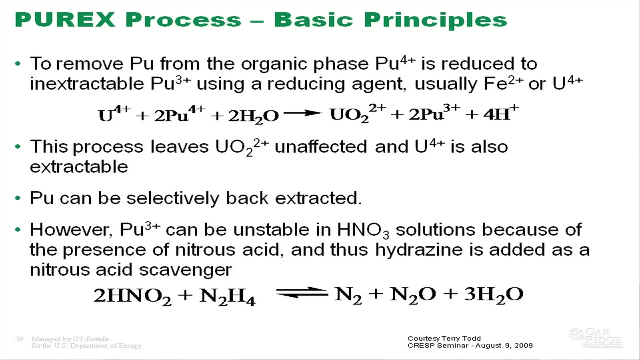 that's extracted in the organic phase by reducing it from 4 to 3.. If you reduce it from 4 to 3, it becomes unextractable And it goes back into the aqueous phase. So it can then be selectively stripped. 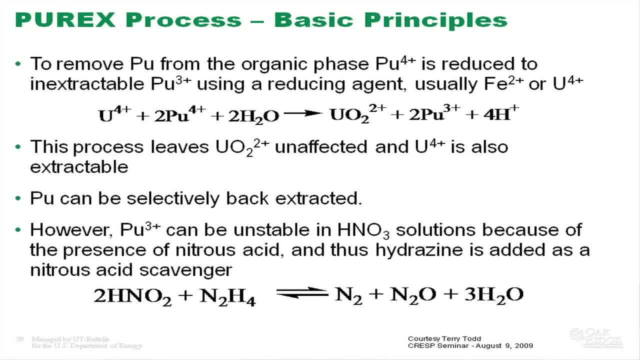 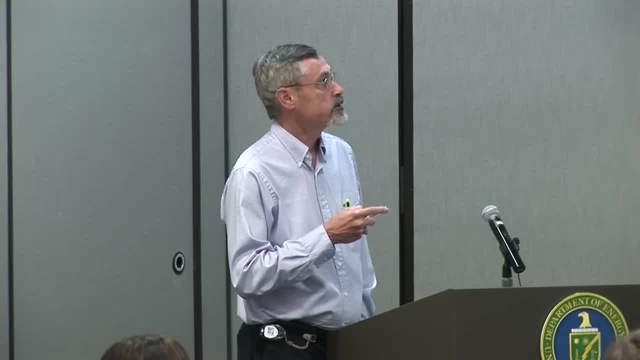 And you do that. You can do that by various ways. In this case, the equation's using uranium-4 to reduce the plutonium. This: you're using one of the agents that you currently have in the plant: uranium. No additional waste. 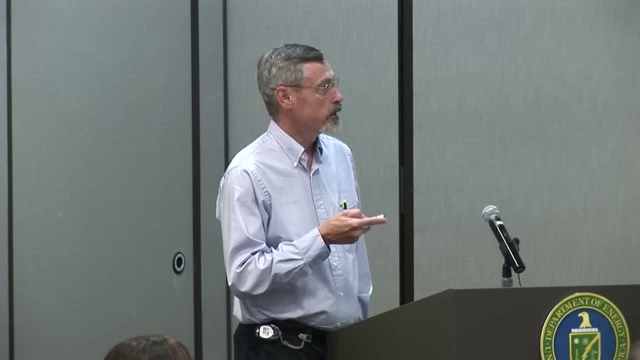 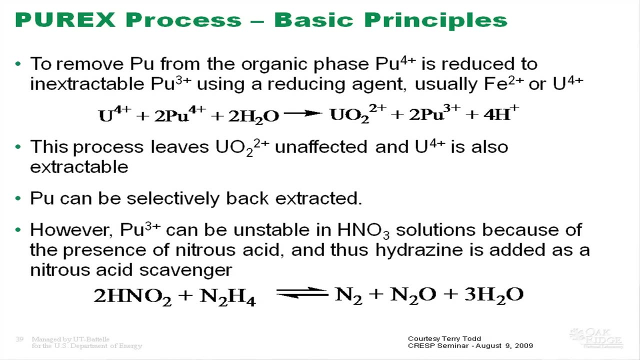 PU-3 tends to be unstable in nitric acid solutions. It wants to go back to 4.. It wants to be extracted, So we have to add some other chemicals to it If you've got nitrous acid and you always want to get. 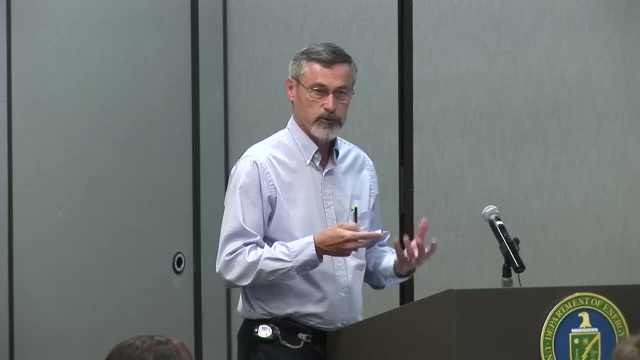 a little bit of nitric acid. you're going to want to use a little bit of nitric acid And you're going to want to use a little bit of nitric acid to hold that in the PU-3 state while we're trying to reduce. 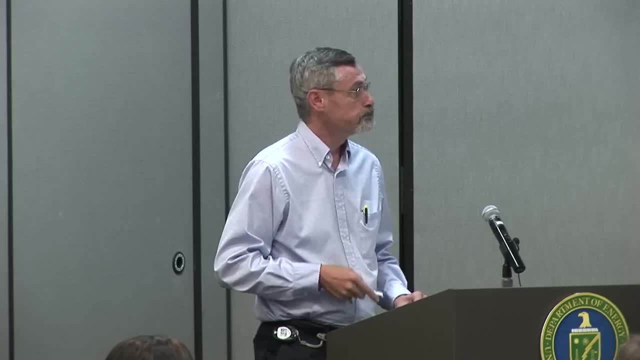 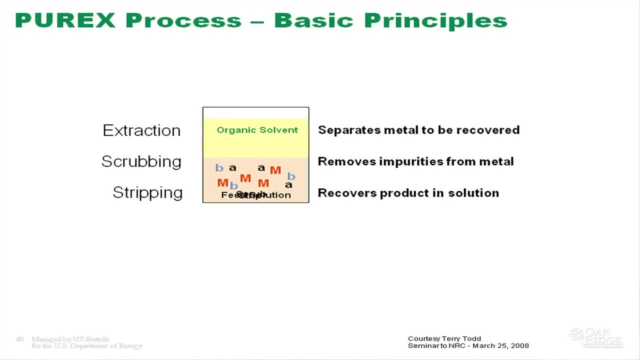 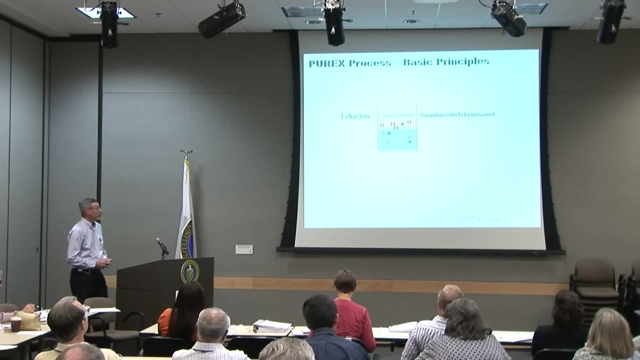 trying to strip it out. So that's where hydrazine may come in to scavenge that nitrous acid. All right, Let's go over that real quickly again. First step: you put the feed solution in and you add some organic solvent. 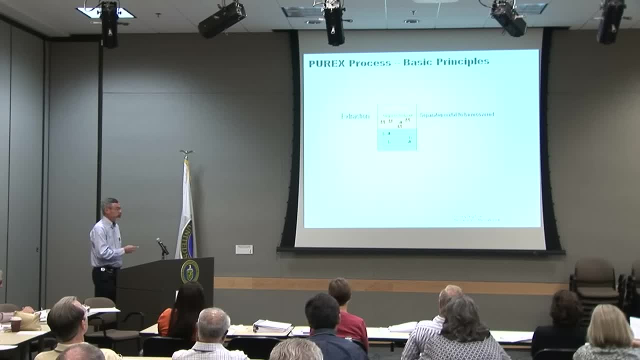 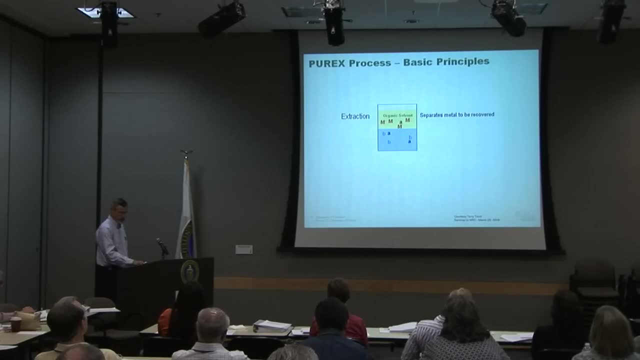 And what happens? Lots of things get extracted. Primarily you're going after those metals, that uranium and plutonium, But you get a few other things that come along just for the fun of it. So now we scrub. Now that removes the impurities from this stream. 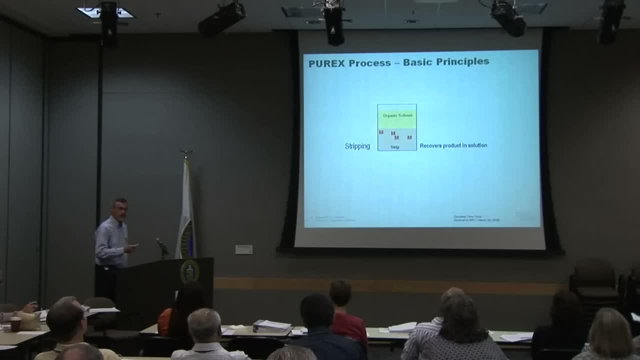 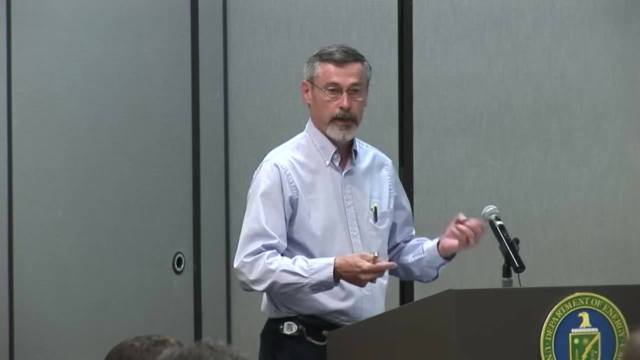 And then finally we add some, We change the chemistry a little, We change the nitric acid concentration and those metals go back into the aqueous phase. So we've done one cycle, That is a cycle of solvent extraction, And we do that in using pieces of equipment. 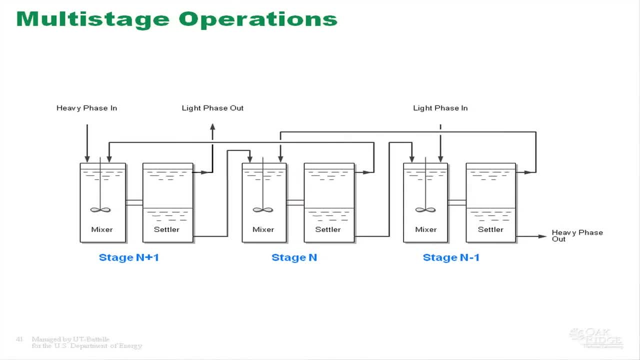 that we stage together. Each stage gets a little bit of the work done And if you want to get very high separations you have to string a number of stages together. So the heavy phase comes in at one end, light phase at the other end. 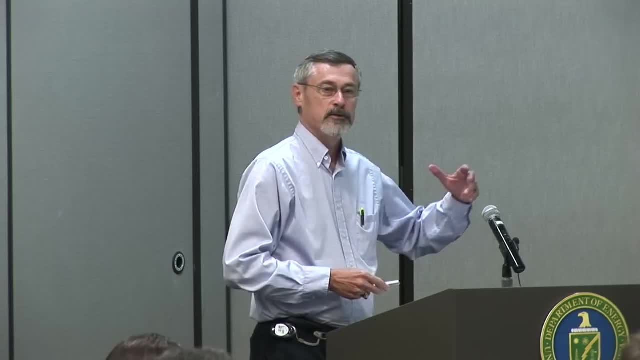 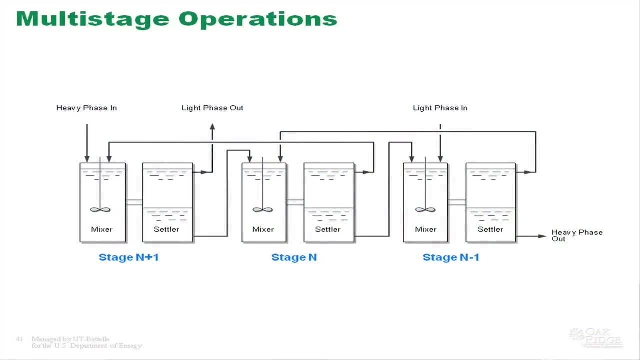 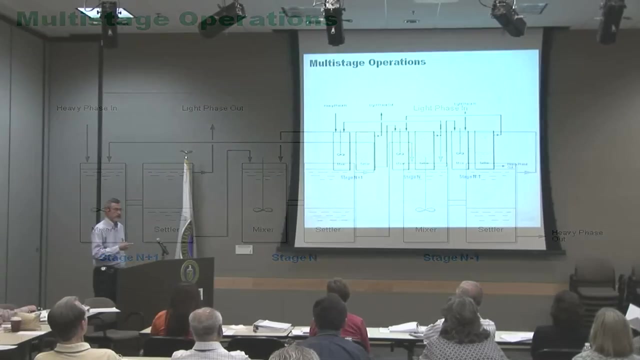 They move countercurrent to each other. Back to those equations we had earlier on. You get: What leaves these two stages from the settler is an equilibrium. What comes in is not, So that's how you make the separation. Like I said, light phase moves this way. 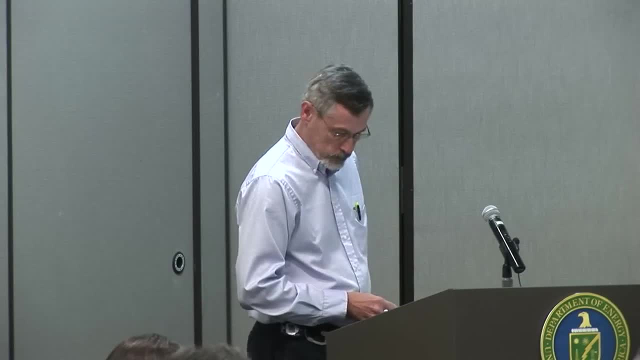 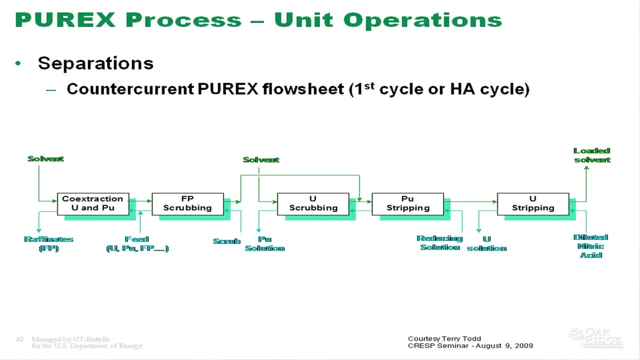 Heavy phase moves that way. So we put that all together with the chemistry and we have the first cycle of solvent extraction. This is co-extraction of uranium and plutonium. The feed stream comes in into a bank of contactors. The solvent is fed in one direction. 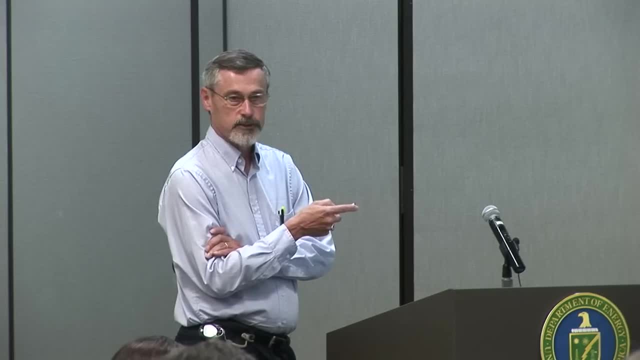 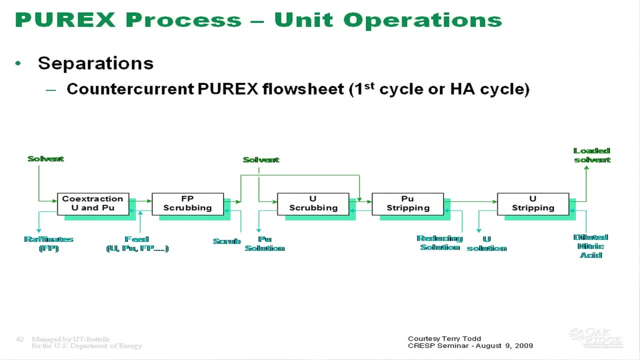 And we put a little scrub solution in. That was that second stage, the little cartoon where things moved. We extract the uranium and plutonium and we try and scrub out the fission products that came along for the ride And they go into the raffinate. 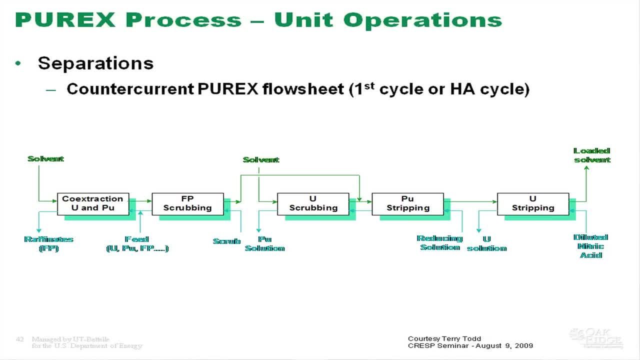 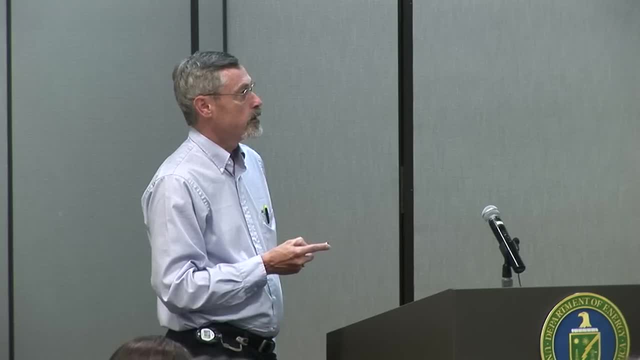 Raffinate tends to be our waste stream. That goes to the high-level waste tank. The solvent containing the uranium and plutonium moves to the second bank of contactors. Here we put a reducing stream in Trying to take that plutonium-4 back to plutonium-3.. 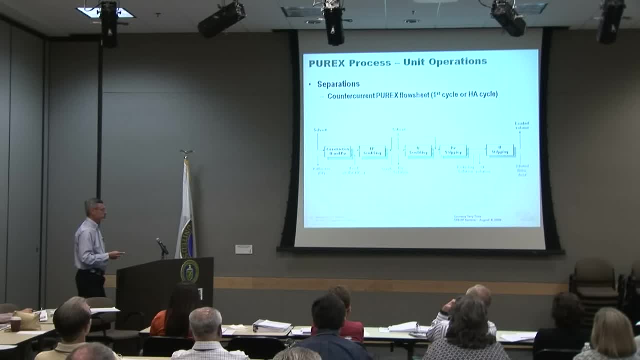 When that happens, it is It tries to move this direction, because that's the direction the organic is going. This takes it from the organic phase, moves into the aqueous phase and we come out with our plutonium stream. It may have a little uranium with it. 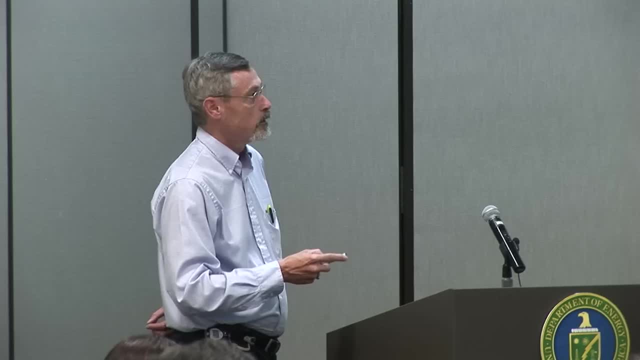 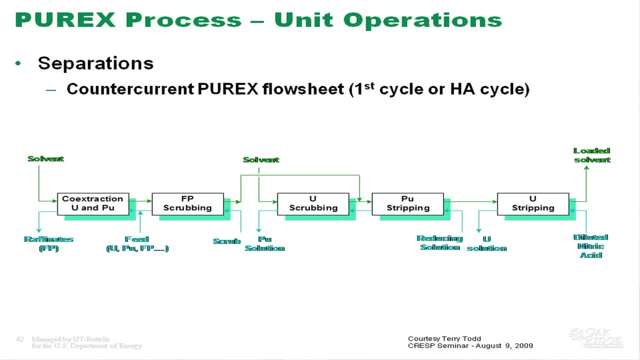 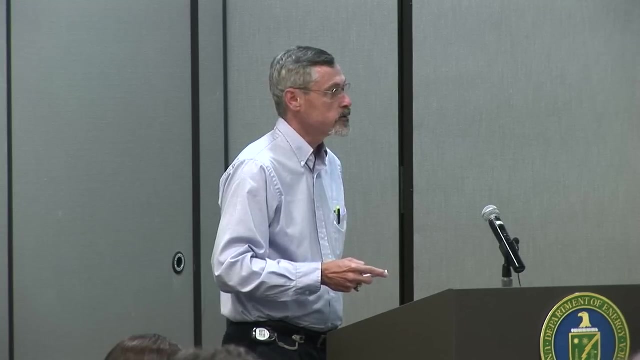 That's why it goes on to another cycle for further decontamination. This stream now contains primarily just the uranium and we strip that by changing the nitric acid concentration. We lowered it, so it has now a very low distribution coefficient. It wants to be in the aqueous phase. 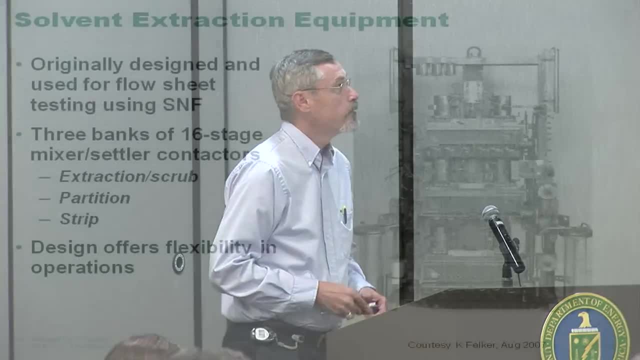 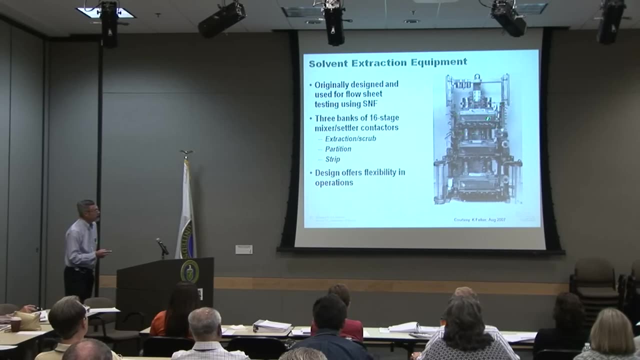 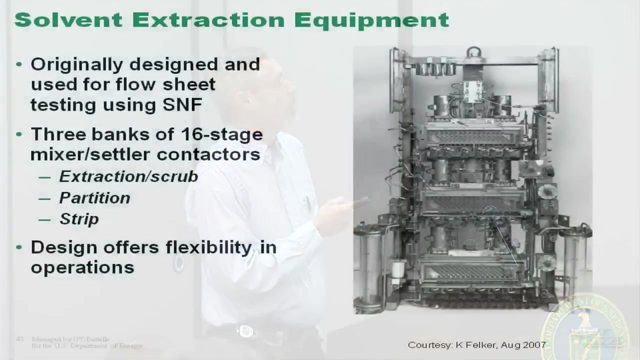 There's our uranium solution. Well, this is another piece of equipment located at Oak Ridge. Here are three banks of contactors, 16 stages each, Same size equipment as that dissolver, And we do extraction, partitioning and strip in these banks. 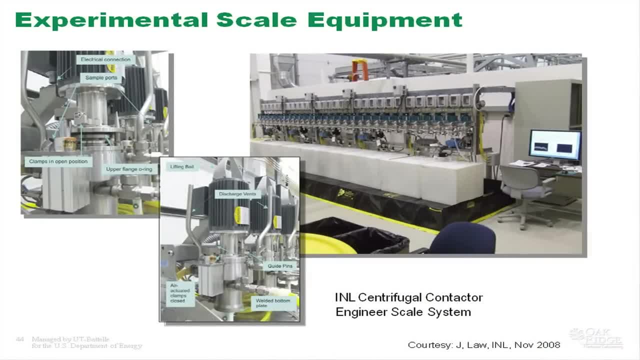 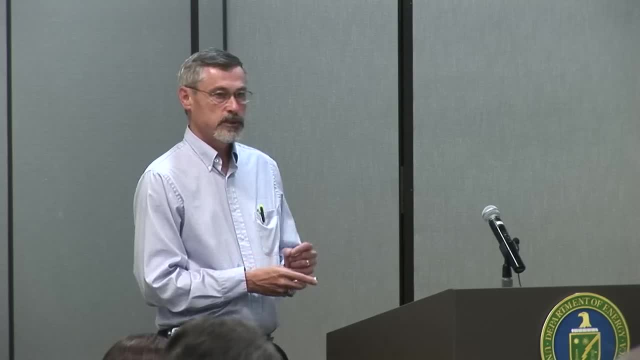 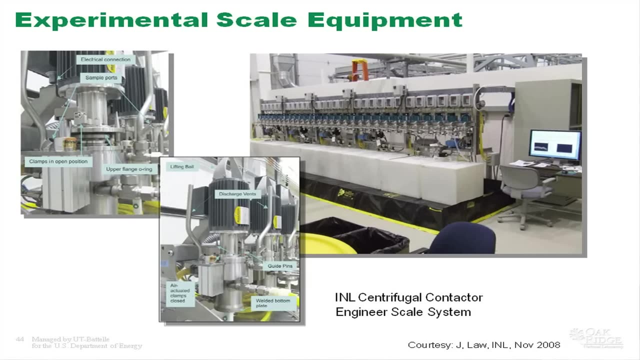 There are certainly other types of equipment. Jack Law will talk about the equipment designs later this morning. Centrifugal contactors: Each one of these represents one stage. These have a lot of advantages in that they come to equilibrium very quickly. They have very low inventories. 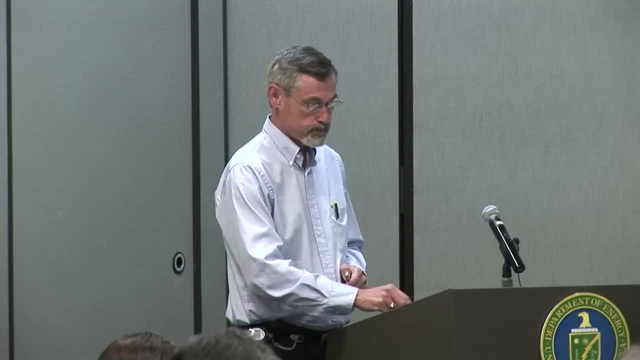 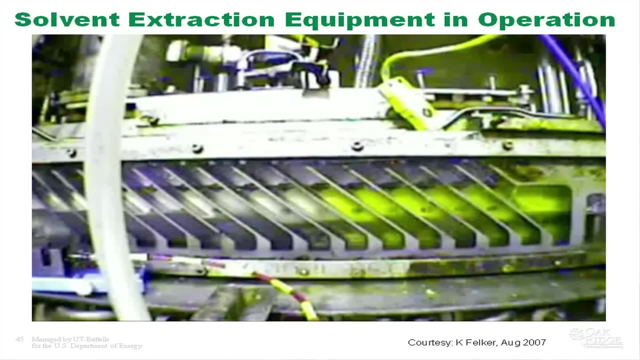 and I won't steal any more of Jack's thunder here- And this is sort of the picture of this equipment running. Here's gears turning an impeller behind each one of these. You're looking at the settling zone of the mixer settler. 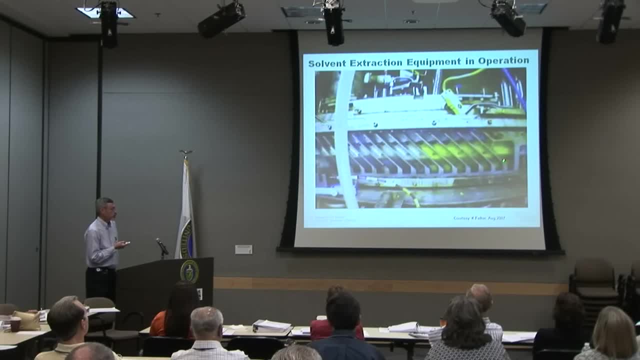 There are three ports on this. In this case we're looking at the scrub bank. Notice the color change. The loaded organic is coming in with uranium. It's moving in this direction. Our dilute acid is coming in this direction. It reaches about the middle of the bank. 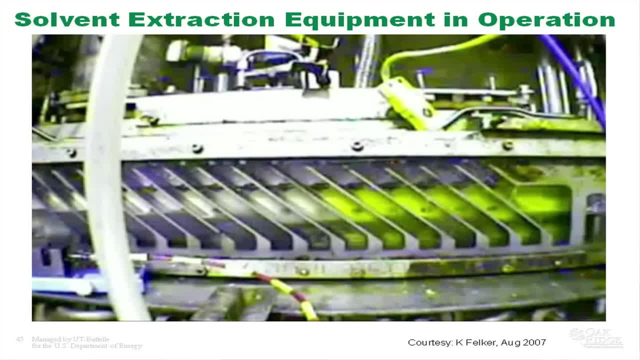 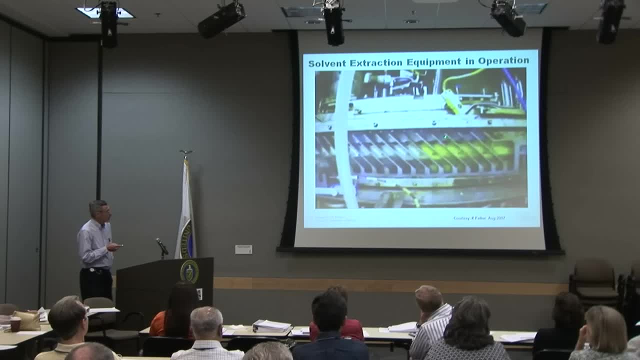 and it picks up the uranium. It's leaving this direction. Organic is flowing this way, Aqueous is flowing this way. The mixer is vertical behind each of these, So it's running. It's picking up the organic from here, the aqueous from here. 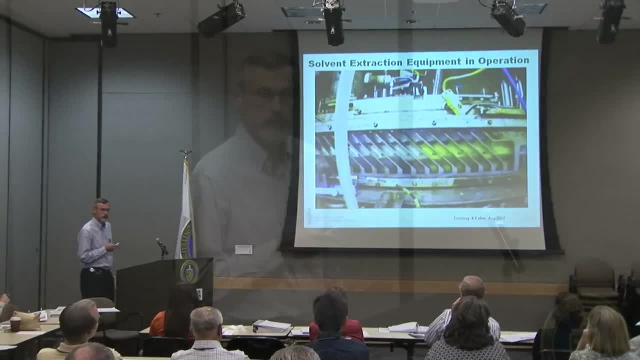 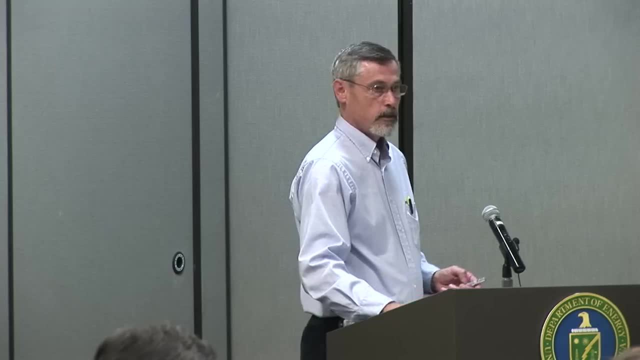 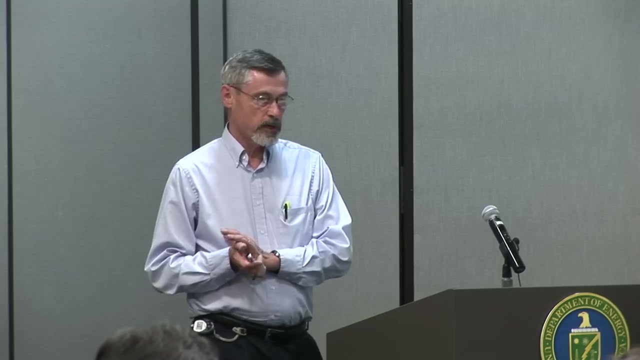 discharging it here. Organic goes this way, Aqueous goes this way. Pretty neat. You can actually see the separation taking place in this equipment And this is actually running in the hot cell. Well, standard Purex process separates uranium and plutonium. 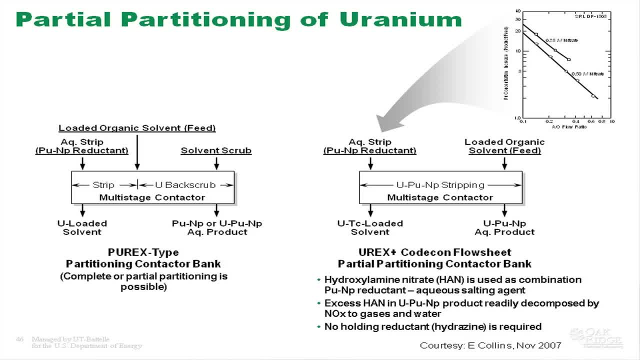 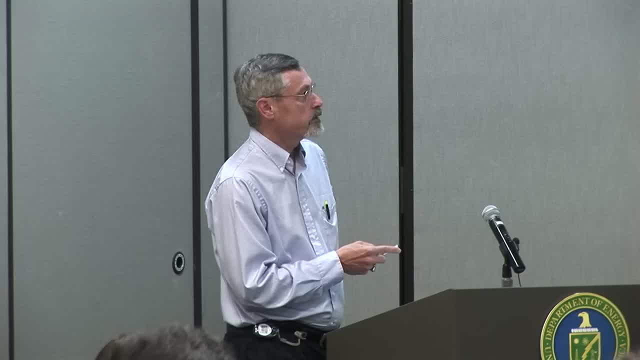 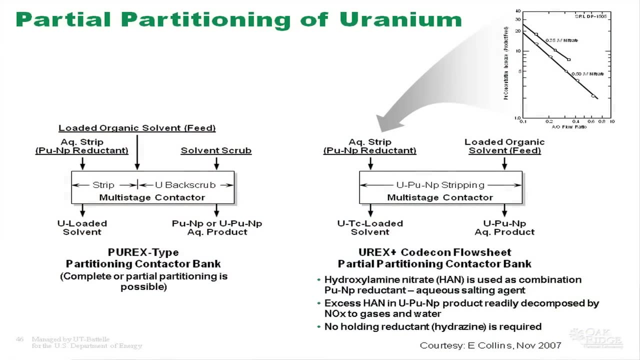 And there are some other ways you can do this. You can do what's called partial partitioning, And if you do that, what you eliminate is part of the partitioning bank. Here we have a uranium back scrub. We don't want any uranium. 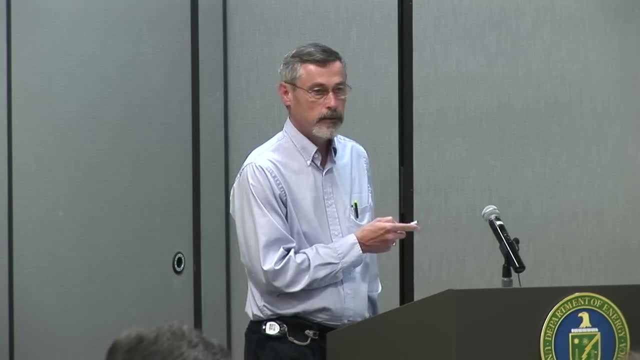 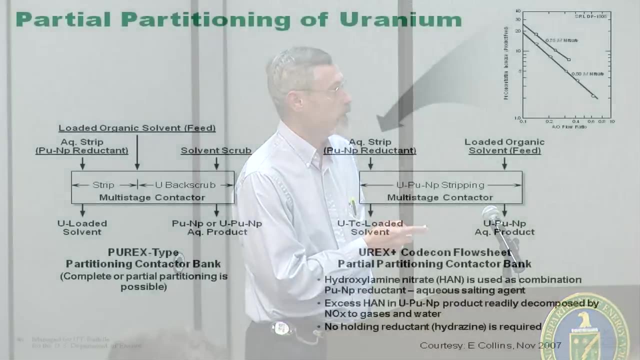 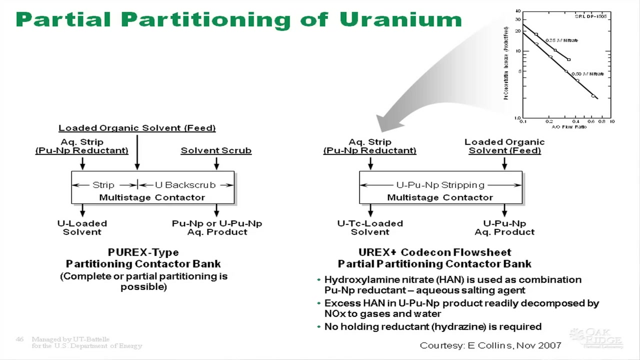 to get out with the plutonium product. We lop that off. If you do that, what happens is you end up with the uranium still comes out. this end. your reductant comes in, but coming out with your product is a fraction of the uranium. 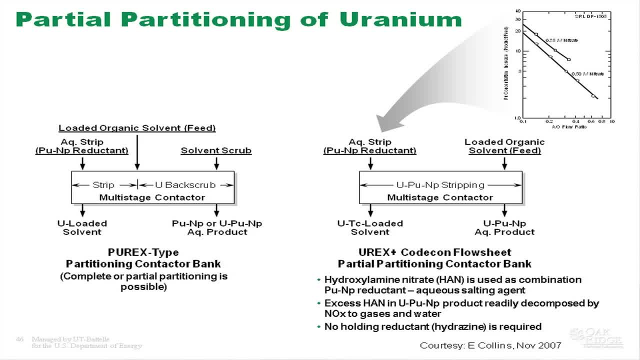 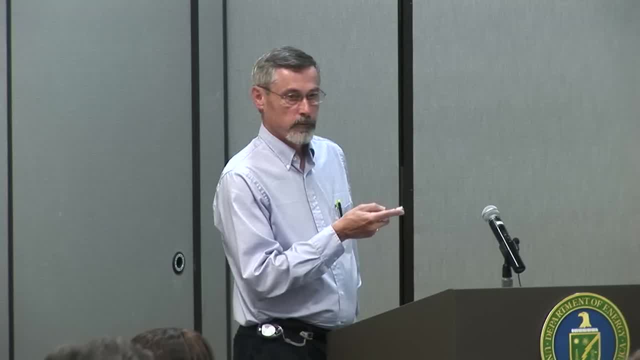 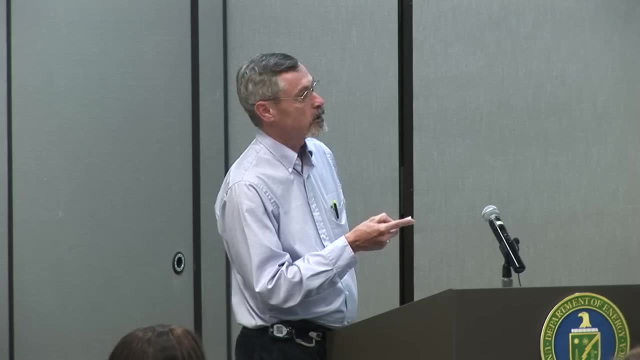 So you never produce any pure uranium, You only produce pure plutonium stream in a partial partitioning-type cycle And depending on what your phase ratio. remember the phase ratio goes along with the distribution coefficient, Depending on your phase ratio, and this is a little chart of the phase ratio. 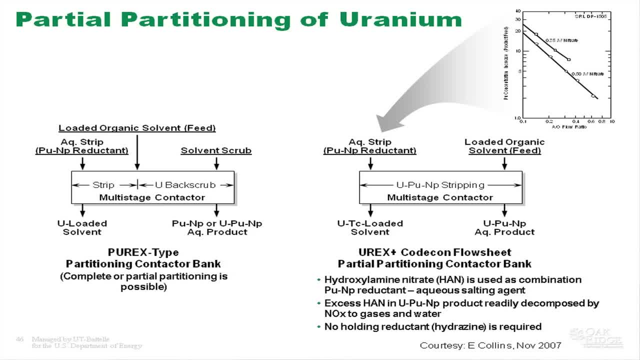 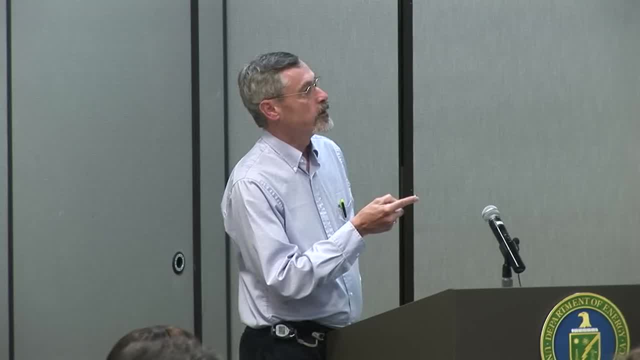 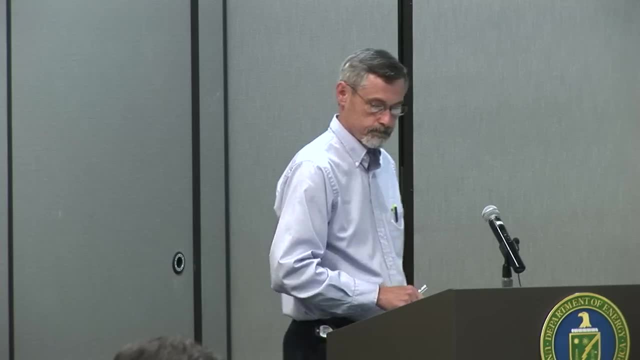 you can adjust the amount of uranium that comes out with the plutonium. So let's say we're looking to get about 10% of the uranium with plutonium. You take a phase ratio of about 2 to get there. Well, there are lots of other cycles. 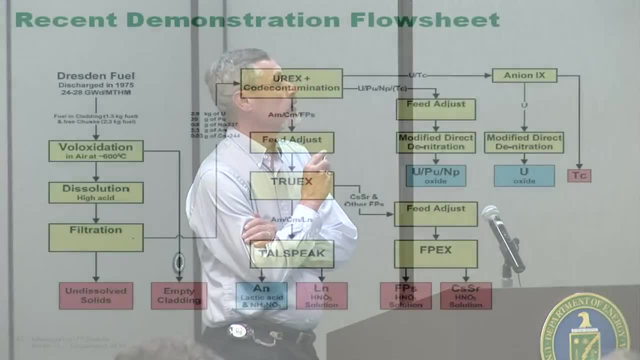 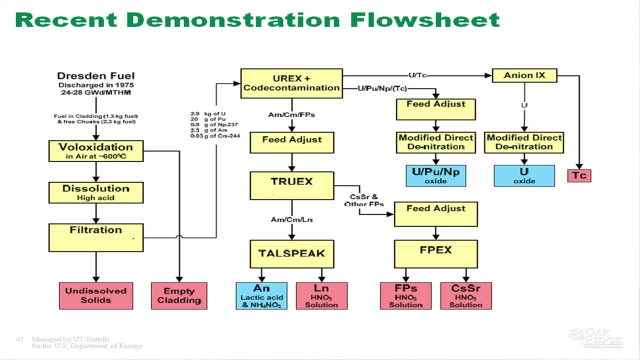 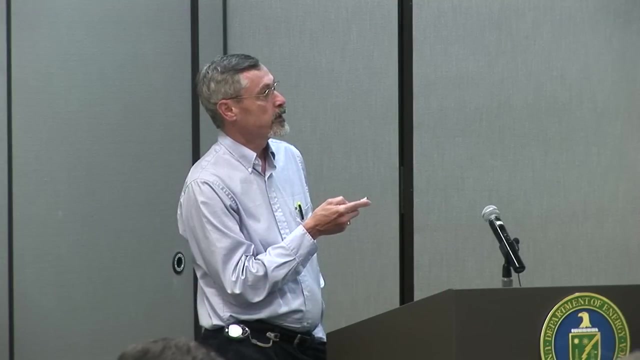 you've probably heard of, and this is a recent flow sheet demonstration- recent by probably 2 or 3 years now. We did veloxidation, did dissolution, filtration, We fed into this partial decontamination, We separated uranium. It came with technetium. 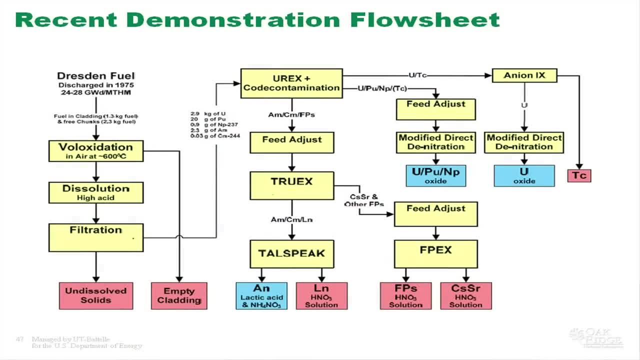 We purified the uranium stream. We had the partial partitioning the uranium, plutonium, plutonium, technetium. It was separated, converted into a solid Well, all of those fission products, along with the americium curium. 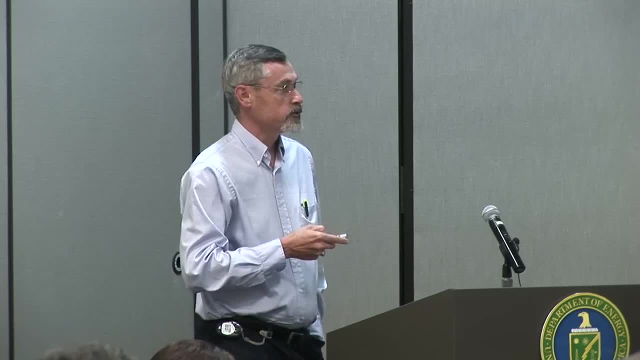 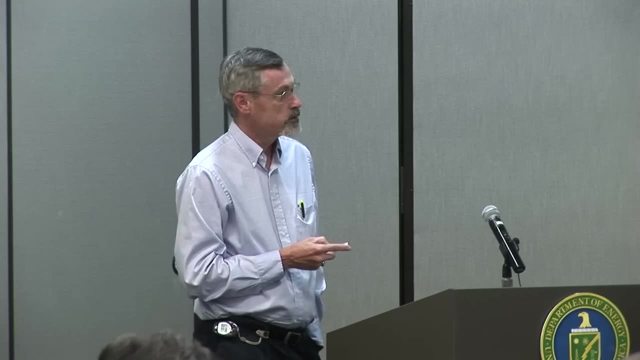 left in the raffinate. Here we separated in a Truex process the cesium and strontium from the uranium fission products. The americium curium lanthanides went to a process called Tallspeak. We separated the lanthanides. 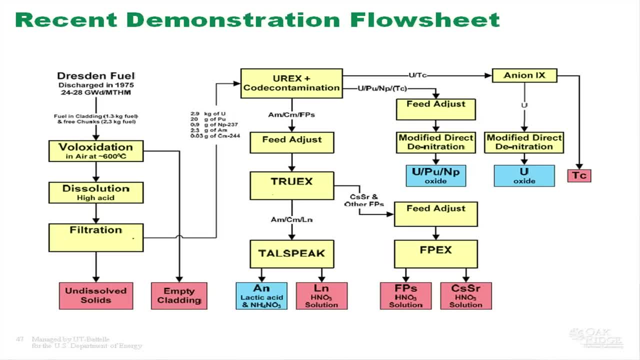 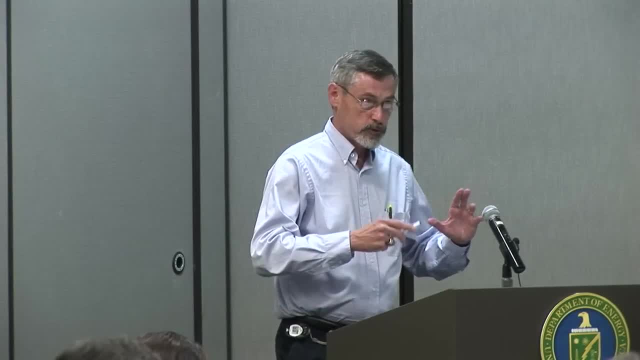 from the actinides. In a process called FPEX, we separated cesium and strontium from the other fission products Just to sort of demonstrate what you can do with various solvent extraction chemistry. The reason we did this, or at least we were at the time doing this: 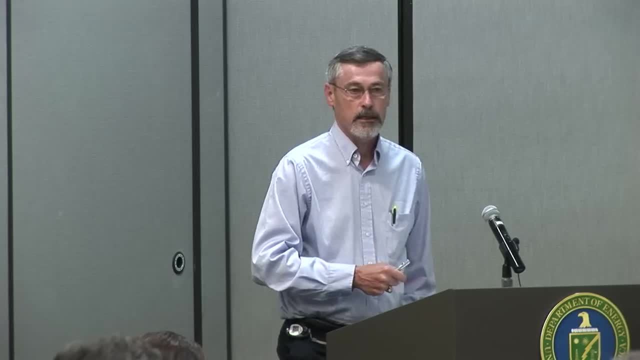 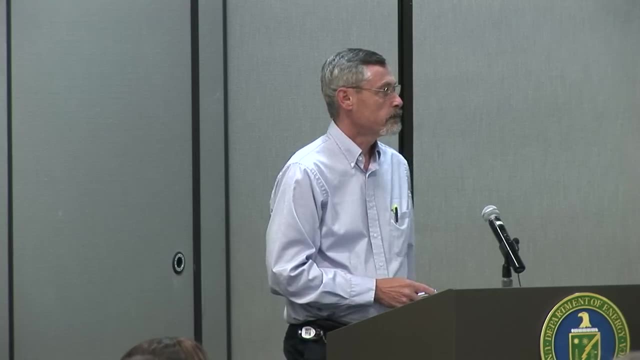 we were looking to say: can we separate those high heat components from the rest of the fission products? And yes, you can. What about the actinides and lanthanides? Because you may want to send the americium and curium. back in as a target to burn those, so you don't have to dispose of them. We're not looking to do that with the lanthanides now. So just to sort of show a few numbers of how well the process works: It raffinates the waste stream. 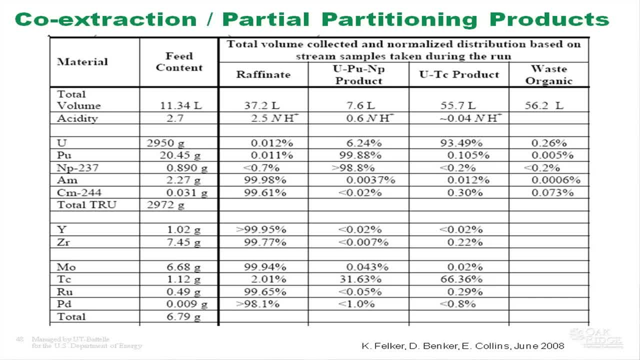 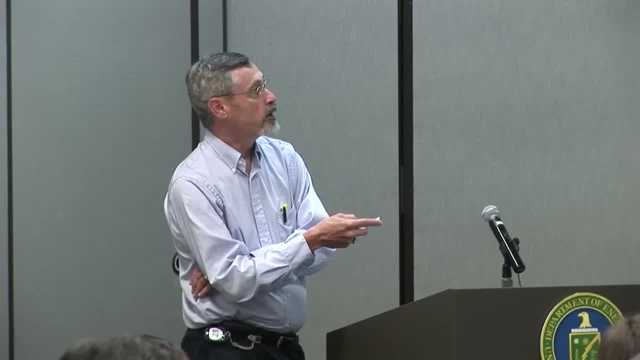 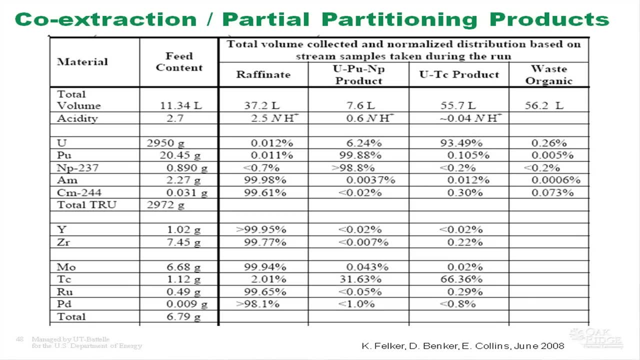 with the stream leaving the first cycle. So we're getting all the yttrium. We're getting this. Notice that most of the technetium goes out with the uranium and plutonium streams. We get a split of the uranium between the UPU nep. 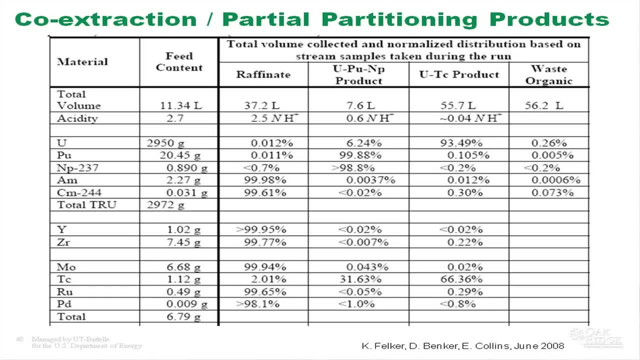 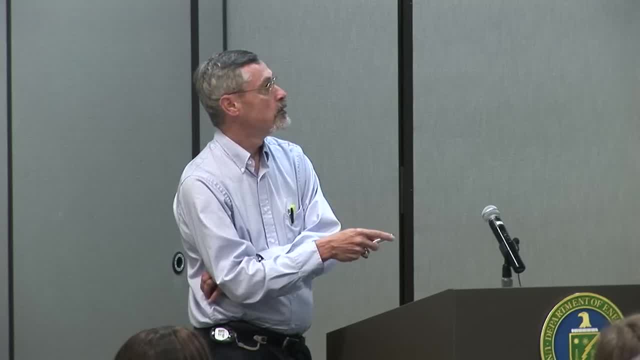 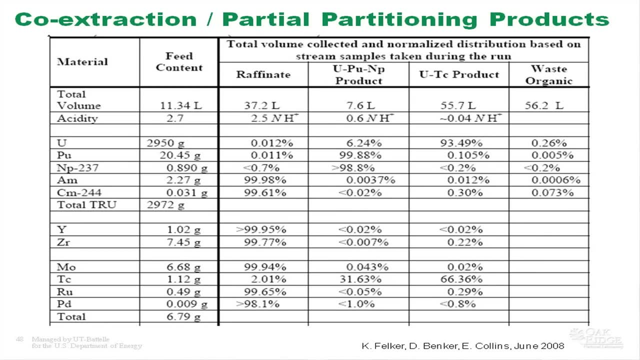 It contains something. It's not a pure stream by any means, And these percentages are a percentage of this number, not a percentage of the composition of that number. So we're getting virtually all the plutonium where we want it. We have a little over here. 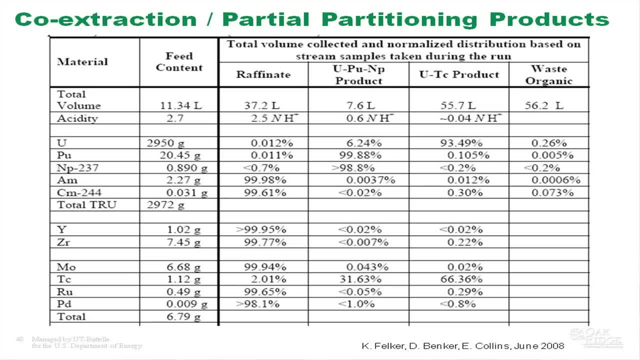 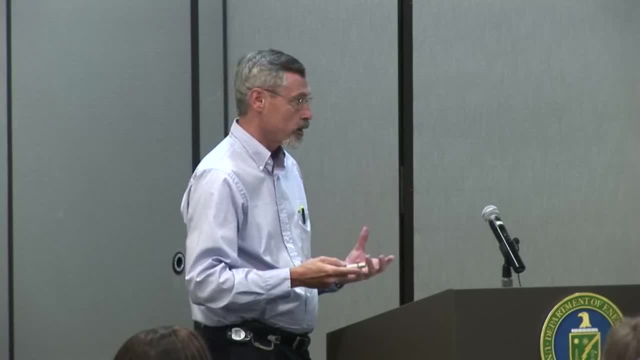 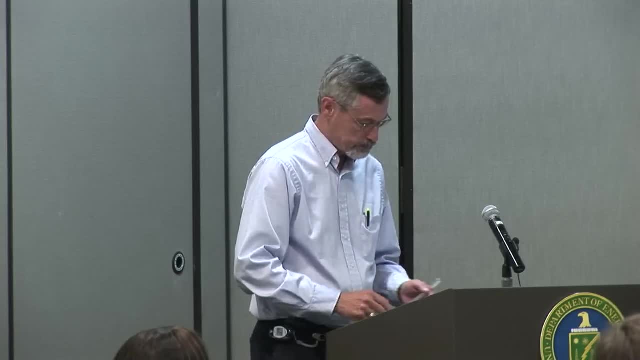 We polish off with a further cleanup. if we wanted that at the uranium, Very little stayed in the organic. We stripped everything out of the organic phase. So things are going where we want them to in the partial partitioning cycle. Now a word or two about product purity. 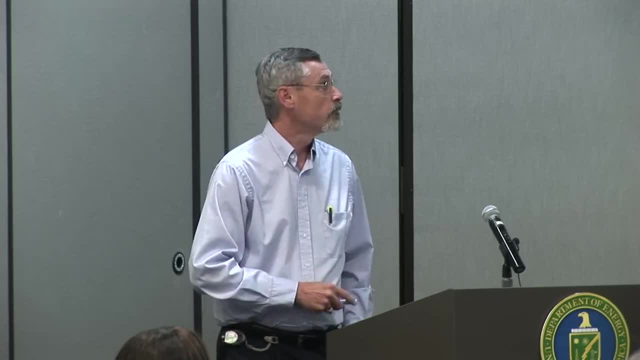 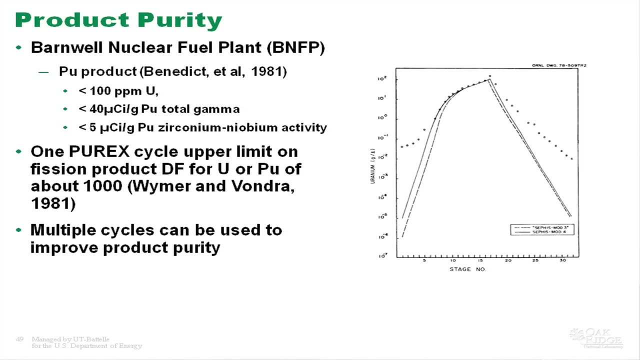 It's great you separate it, but how well do you have to separate it? The product specs at Barnwell in the PU product: less than 100 parts per million uranium. Less than 40 picocuries total gamma activity in the plutonium product. 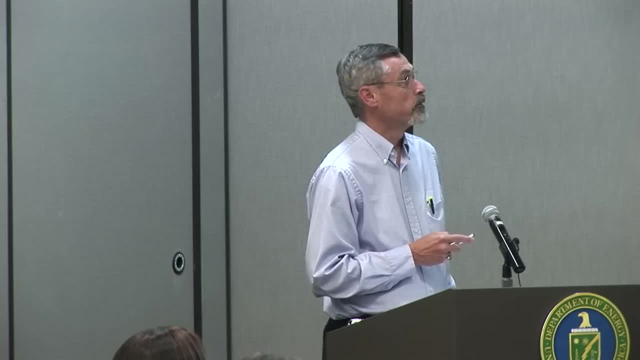 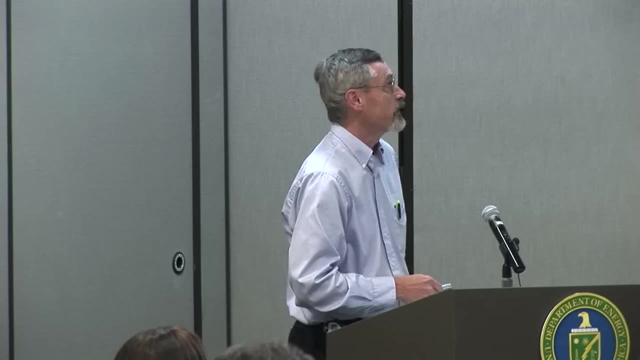 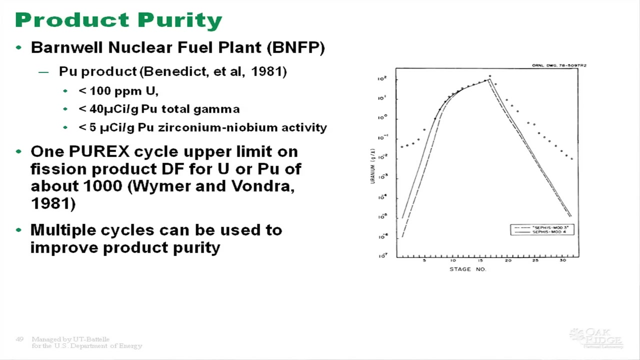 and less than 5 picocuries of zirconium niobium activity in the product. Those were the product specs from Barnwell. Now that plant never operates, We don't know if it actually achieved that. Typically, one Purex cycle can get you about a DF of 1,000.. 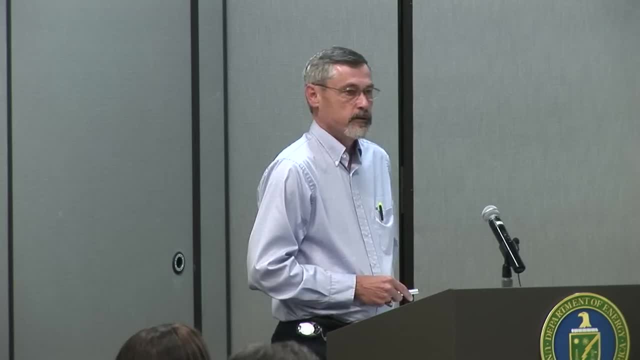 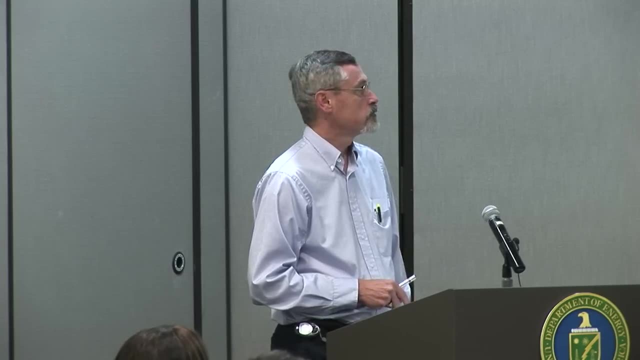 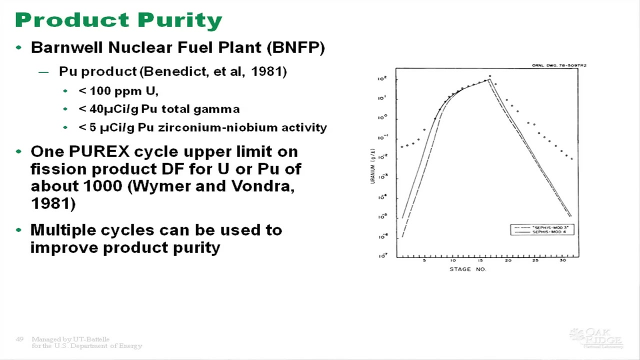 Or does it matter? It doesn't matter, This is just a composition at the end. So it's how much? what are the trace impurities in that product on a gram-per-gram basis? So multiple cycles can be used to improve that product purity. 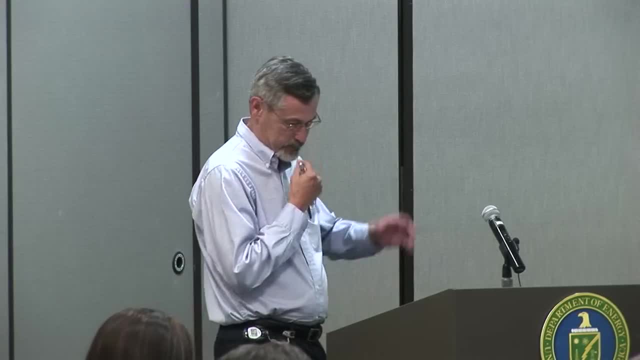 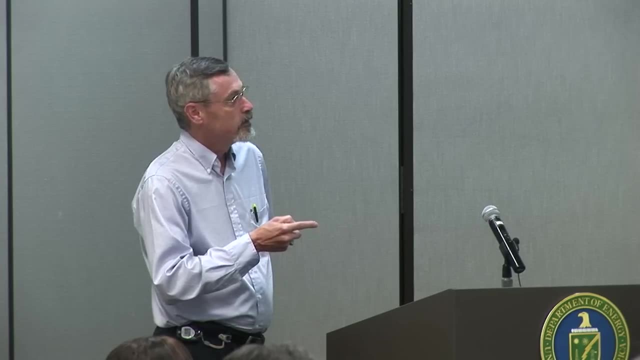 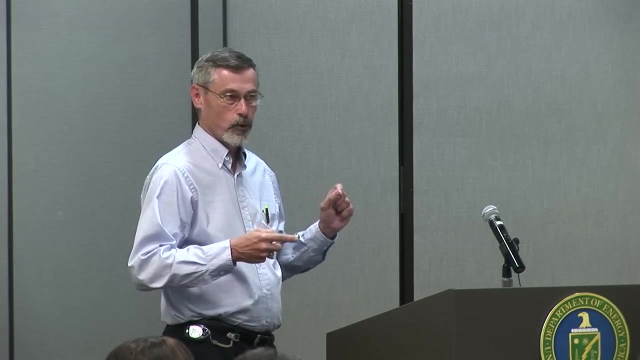 This is basically here just off on a tangent, talking a little bit about modeling and how well you can predict some of the separations. These curves are the models, This data- when you get down to very low compositions- is where the models don't work real well. 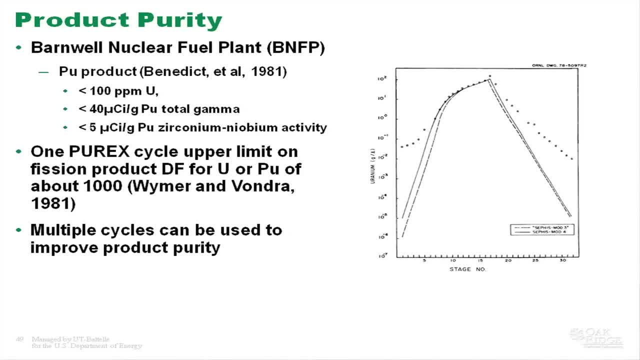 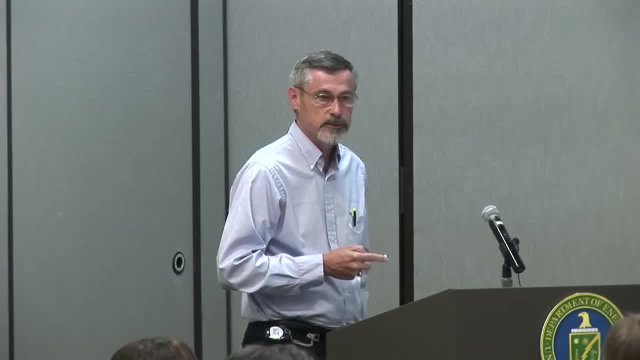 So Dave DePaoli is going to be coming tomorrow, I believe, to talk about modeling Some of the trace components at very low compositions when we're trying to do the separations. that's where there's a real need for better understanding. 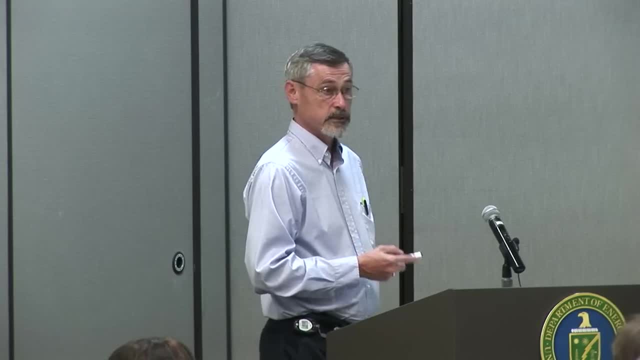 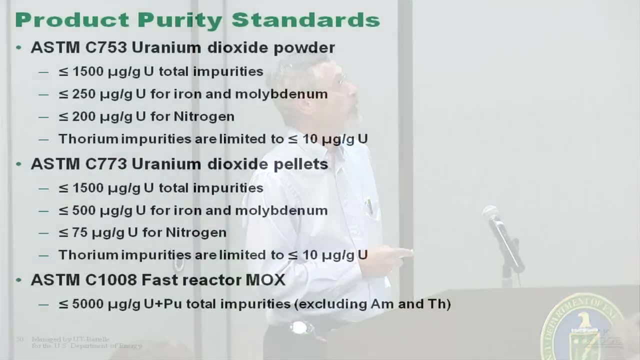 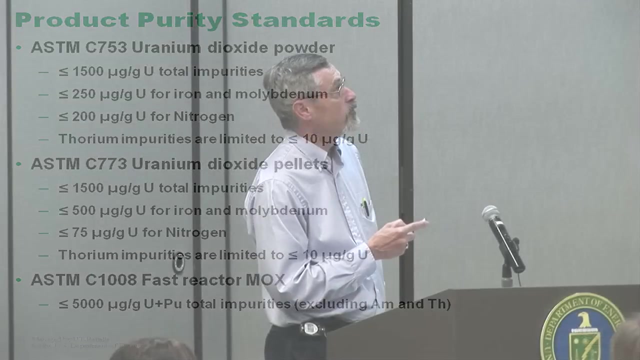 of where do these trace species go and how well do we do the separations? These are product purity specs from ASTM Numbers to look at. Notice that the iron goes up as you go from the dioxide powder to the pellets. The nitrogen numbers go down. 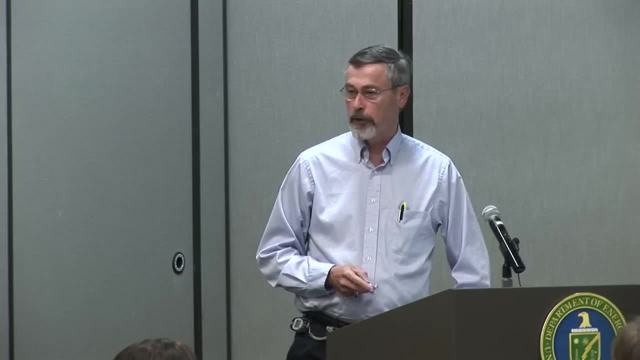 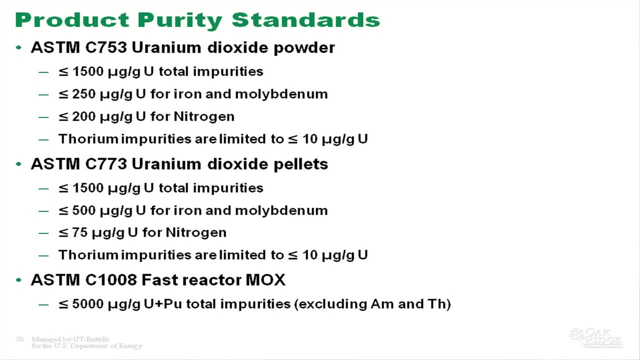 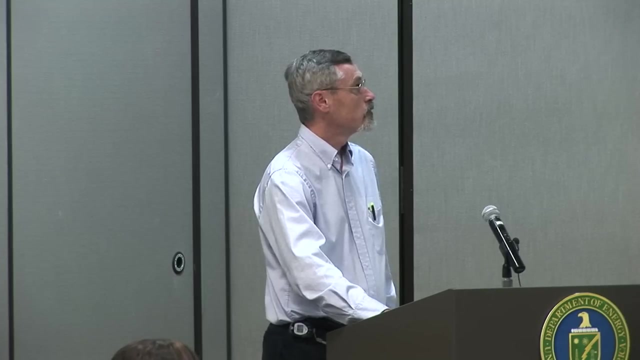 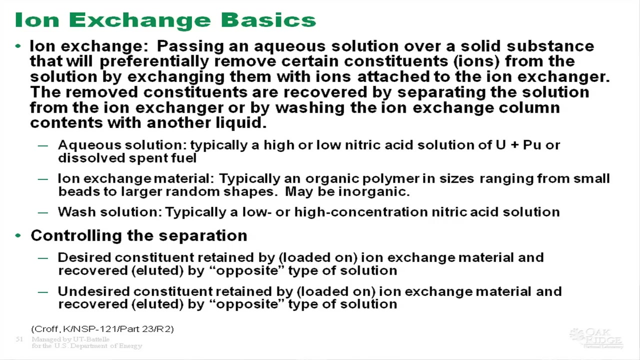 Nitrogen is an important one because of the ingrowth of carbon-14.. That's where it comes from, from nitrogen-14. And so you want to keep this number as low as you possibly can get it. Iron exchange processes: These are another separations technique. 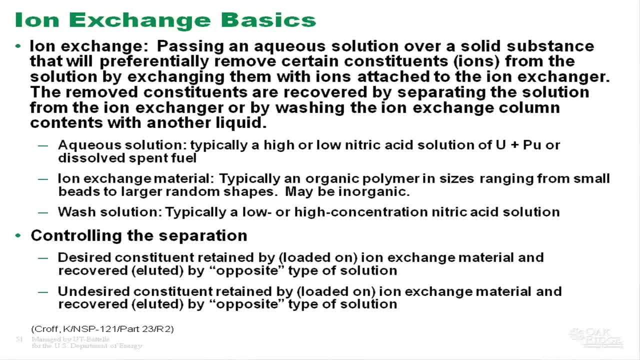 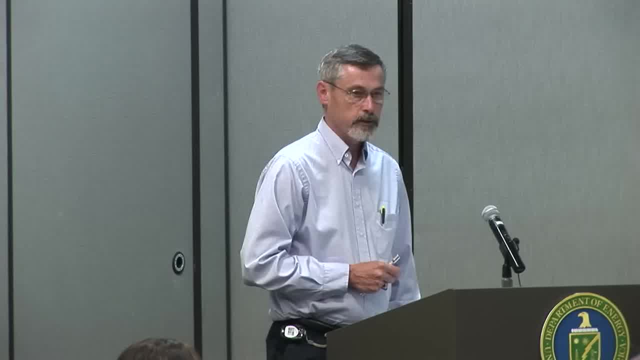 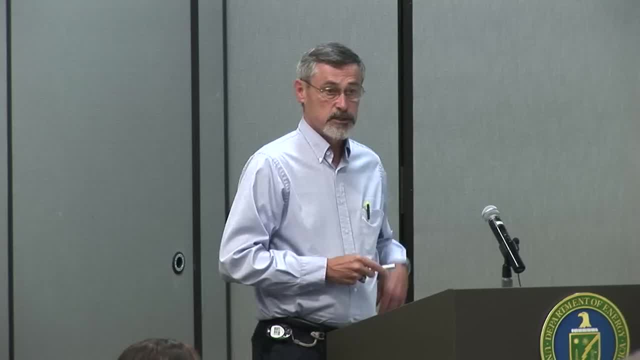 They're typically used in the polishing of the product, And typically you're either trying to recover a very small amount of material from a very large stream. Typically that's in both cases. One: you're trying to recover something because you want it from a very dilute stream. 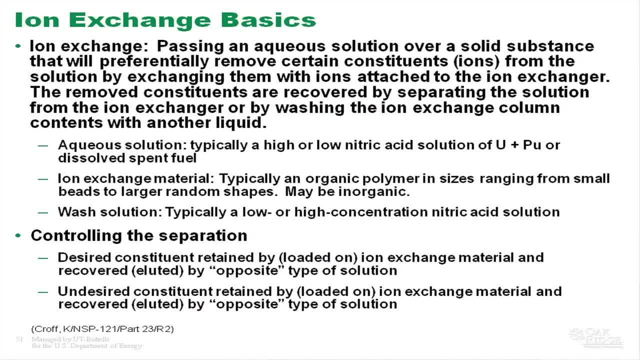 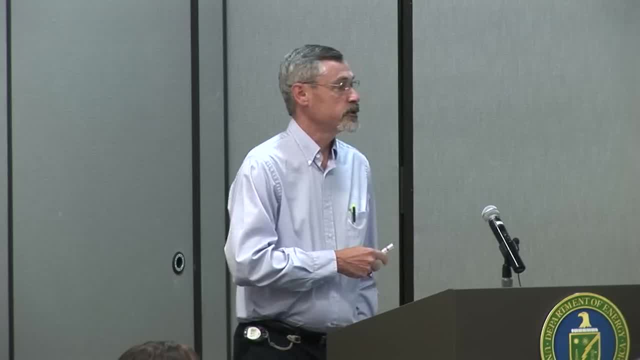 or you're trying to remove very small quantities of stuff you don't want from a stream, So you typically This is a resin material, It's in a column And you typically are passing either a high acid concentration or a low acid concentration. 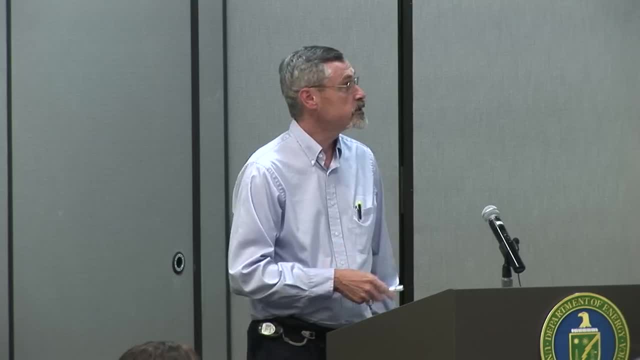 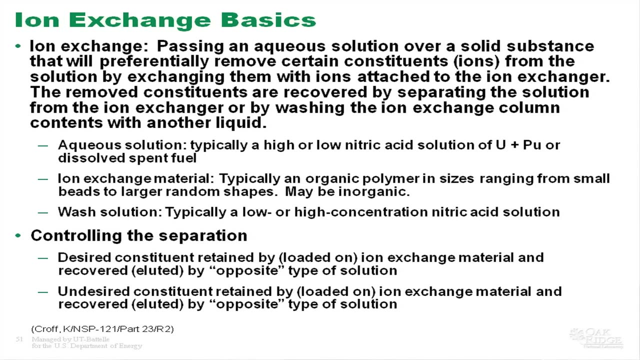 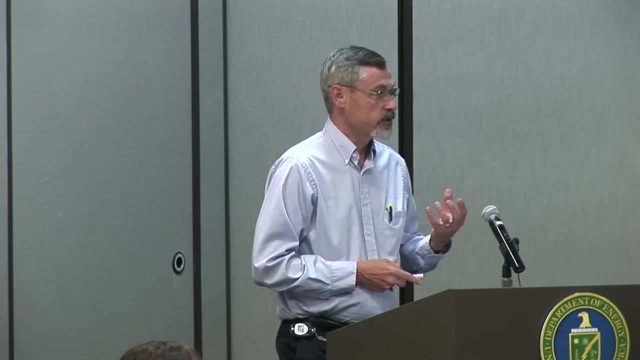 with your material of interest. through this, It ion exchanges with an ion in the resin. That ion leaves with your solution, And then your material is loaded with the species you've removed: The. In one case you're controlling the separation to remove a desired constituent. 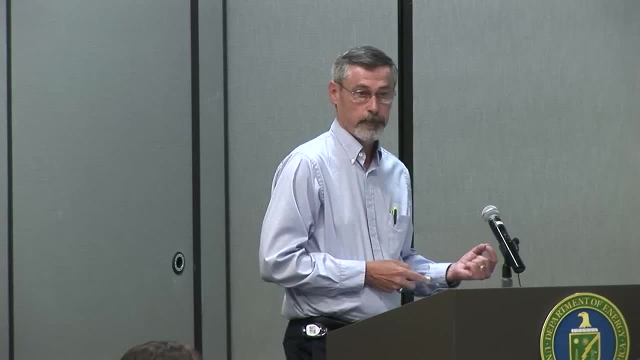 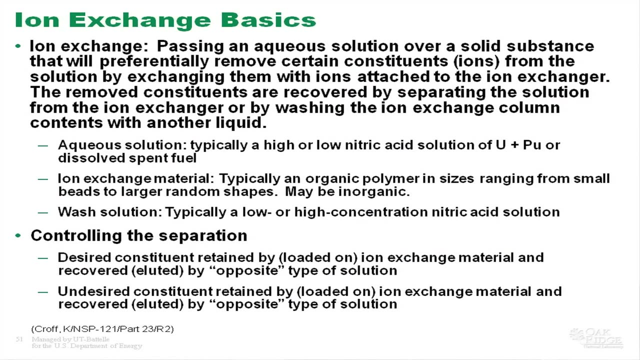 Let's say we're trying to recover technetium from a product and we want that as a separate stream. It's very dilute in our product, So we're using ion exchange to recover that and then we elute it to put it into another form. 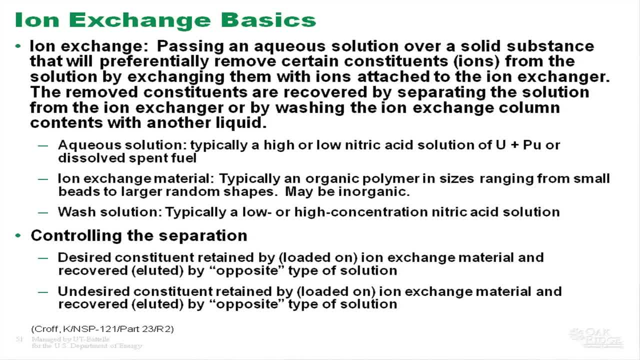 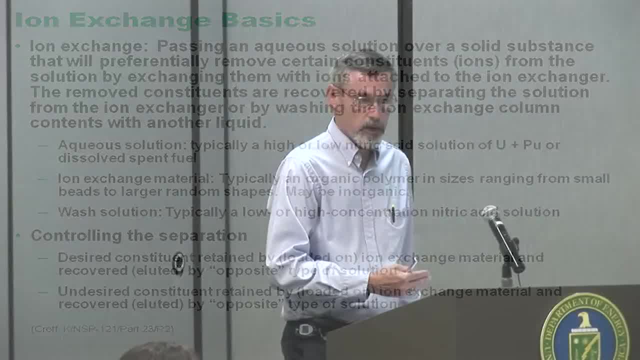 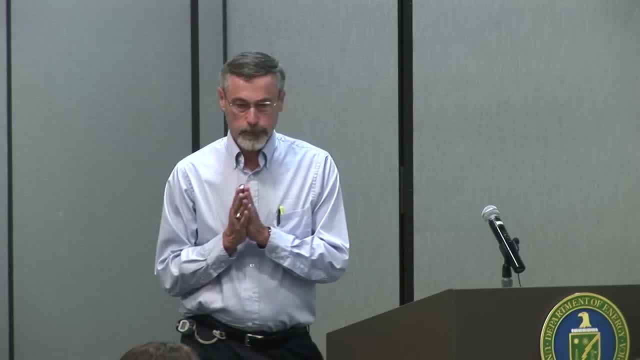 Or we're trying to remove something, just a trace impurity, and now we're limited by how much that material will hold and we may or may not recover that off the resin. The resin may be disposed of- Most common example that you'll run into. 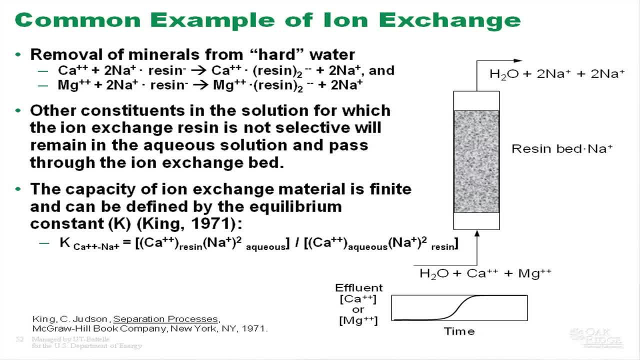 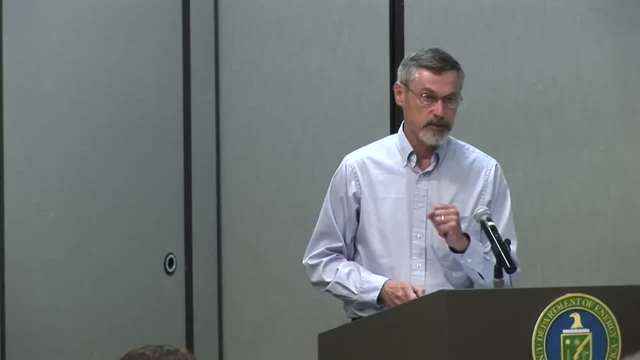 is a water softener. If you have a water softener at home. that's an ion exchange process. You load sodium onto the resin. Calcium magnesium displaces the sodium. The sodium goes into your water. The hardness- The minerals that cause the hardness in water. 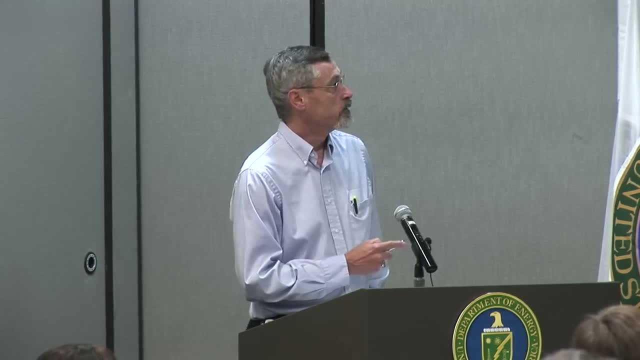 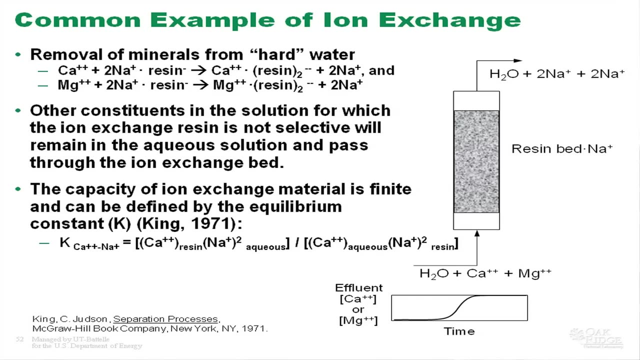 are loaded onto the resin. This equation will give you the capacity of the material, And so, in essence, that material has a finite capacity, And you'll see that nothing comes through for a period of time, and then you reach the breakthrough of that bed. 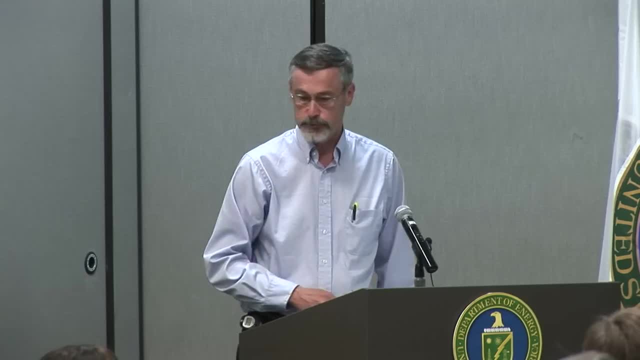 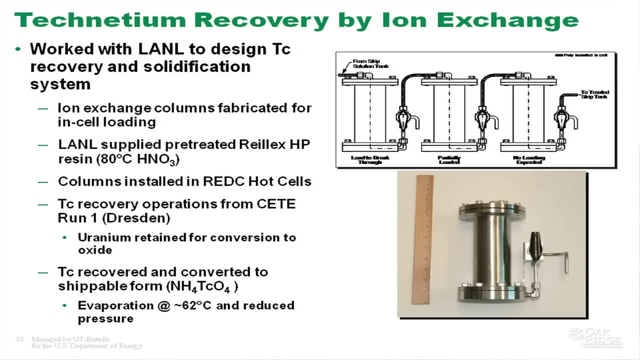 and then, when your capacity's exceeded, everything else just passes through. I mentioned technetium recovery. during the work in the AFCI program, we recovered technetium as a material for a, ultimately going into the waste as a separate stream. 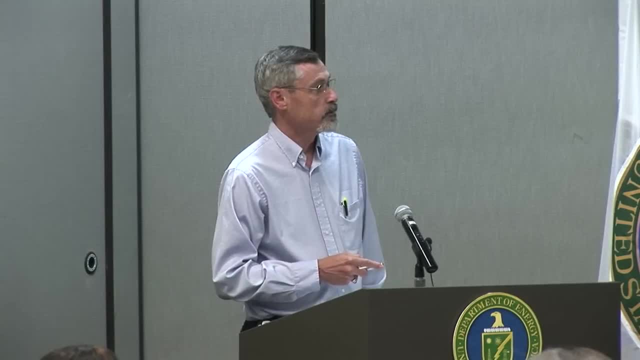 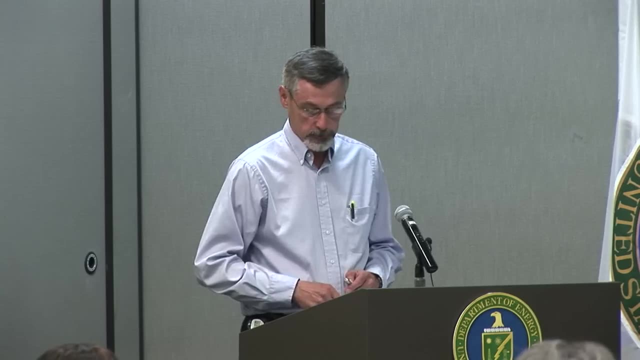 We used a Rilex resin to do that. They're just small columns loaded with Rilex resin and then we recovered that as an ammonium per technetate that we shipped to from Oak Ridge to Lannell. How did you get the technetium off Rilex resin? 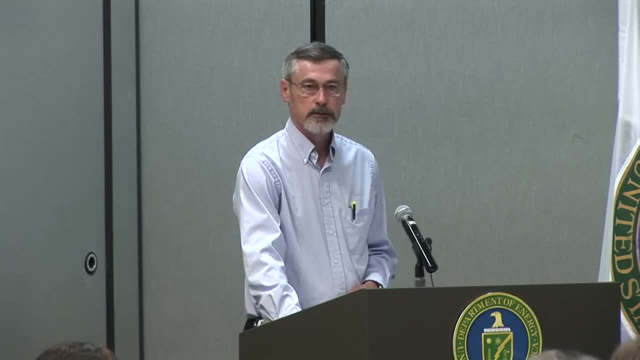 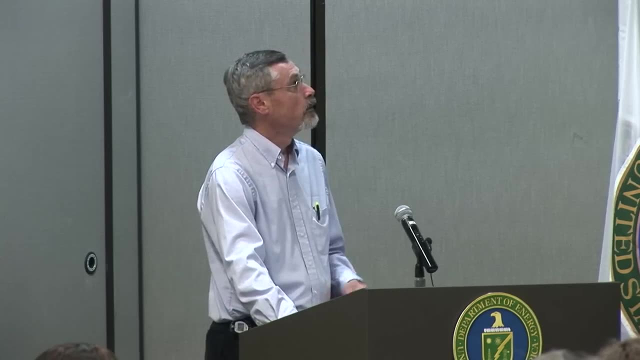 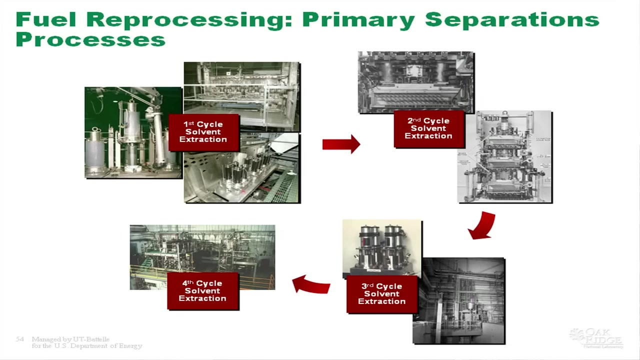 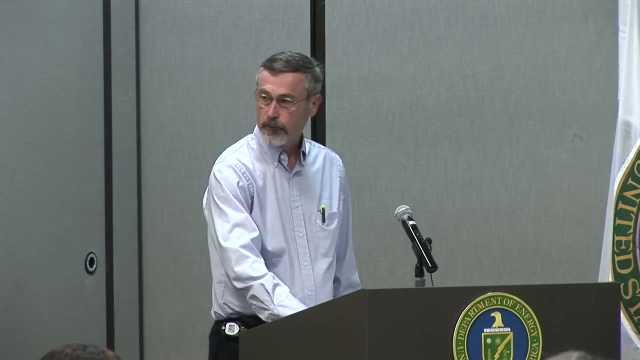 Uh, basically it was an ammonia solution. We just extracted it off the resin. So there are various types of contactors: centrifugal contactors, uh in various sizes, mixer settlers and a pulse column. All are viable solvent extraction processes. 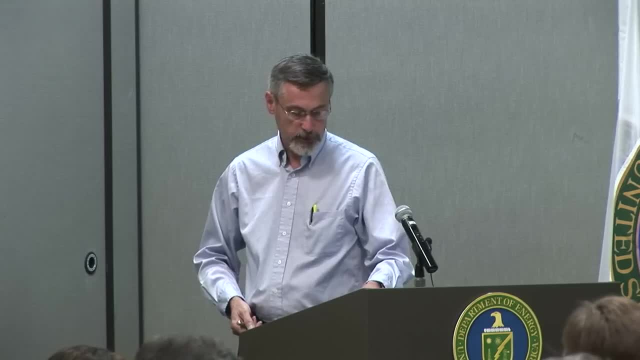 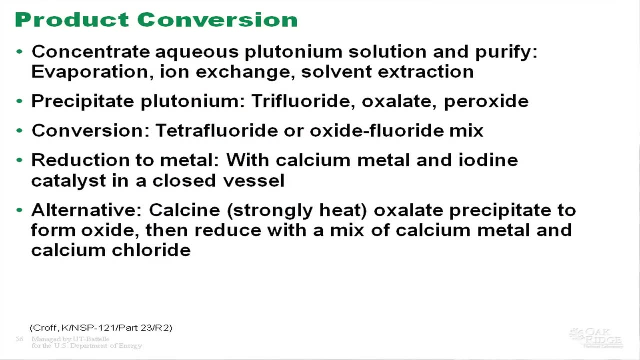 So once you've got it off, it's still in the solution. your next step is you've got to convert it into a solid. And as you convert it into a solid, uh, you probably go through these steps. You're going to concentrate that solution. You're going to do that either by evaporation, by ion exchange or solvent extraction. You then precipitate it uh, typically with fluorine or an oxalate or peroxide. Um then you will convert that uh. 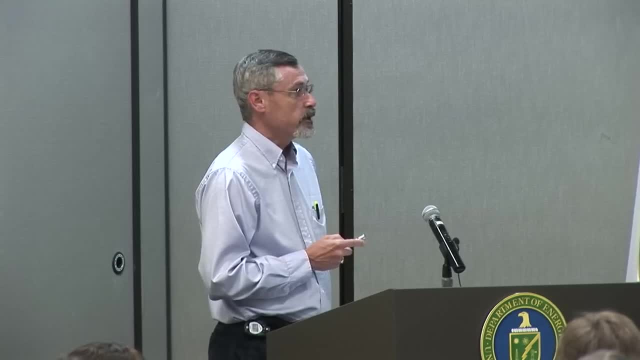 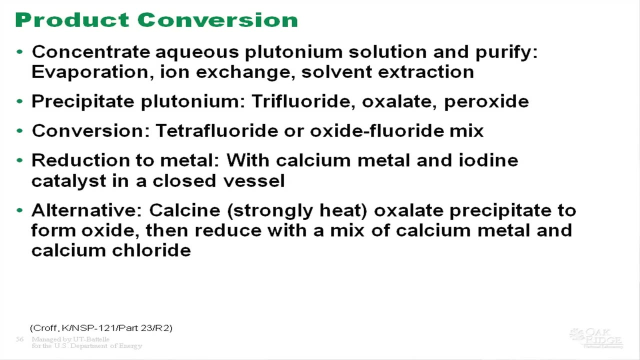 to a tetrafluoride or oxide fluoride. Then reduce it with by adding uh, magnesium metal with some iodine as a catalyst And you put that in a closed vessel. You heat it to ignition. The calcium metal converts to a. 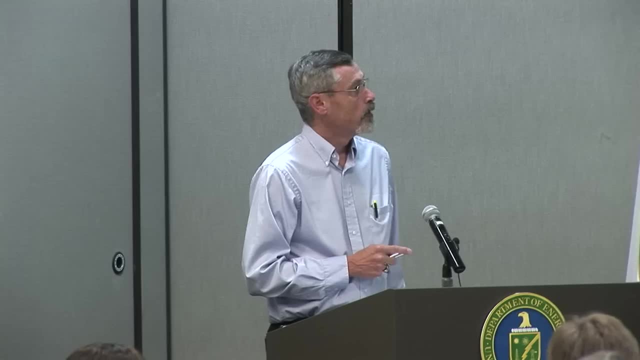 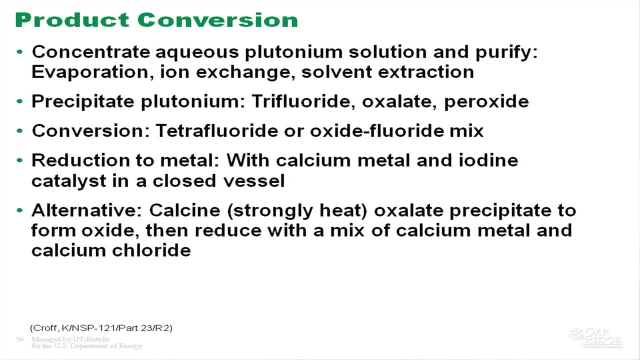 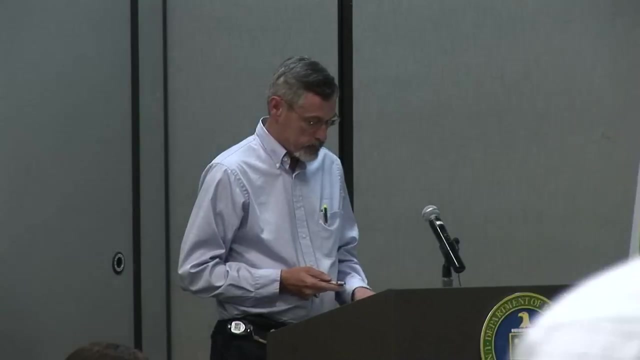 uh, calcium chloride, uh or calcium fluoride, And the- in this case plutonium, is converted to the metal. That is sort of the the way one typically would come up with a, a plutonium metal, But uh. 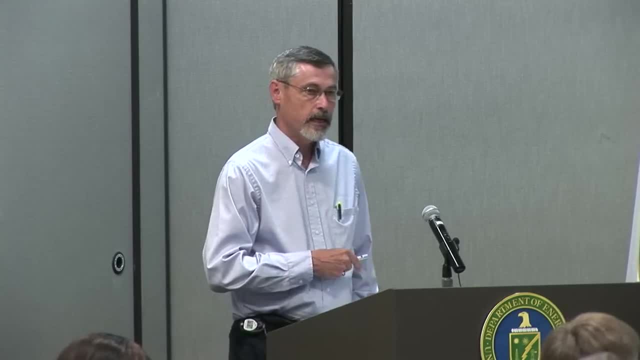 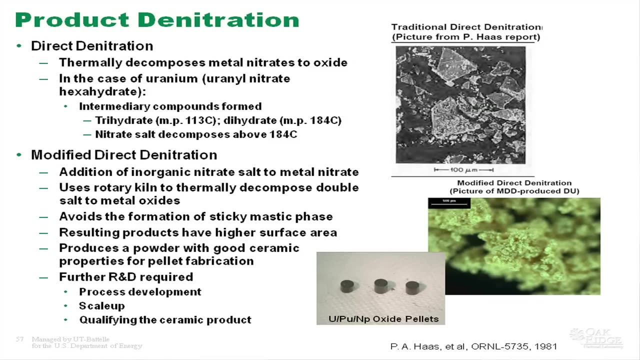 other processes that have been developed. uh, you can denitrate that if you're in a nitrate solution. Direct denitration will decompose the uh uranyl nitrate As it does that. it goes through uh. 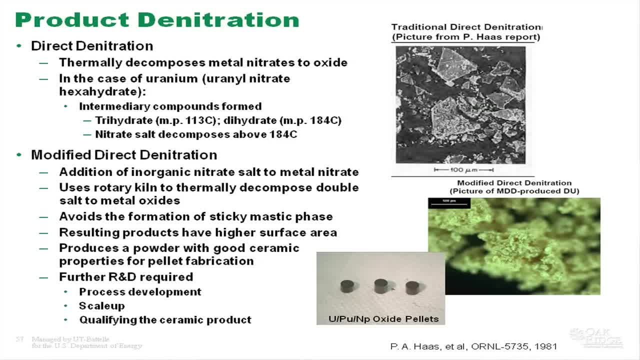 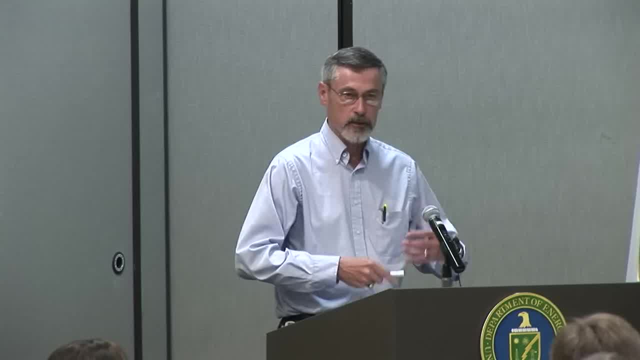 a trihydride, a dihydride and finally it decomposes when you get above 184 degrees C. What you end up was: it goes through a mastic stage, It goes through a very sticky stage And then you end up with this glassy material. 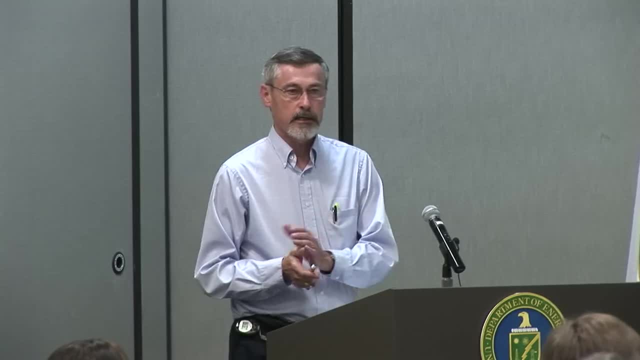 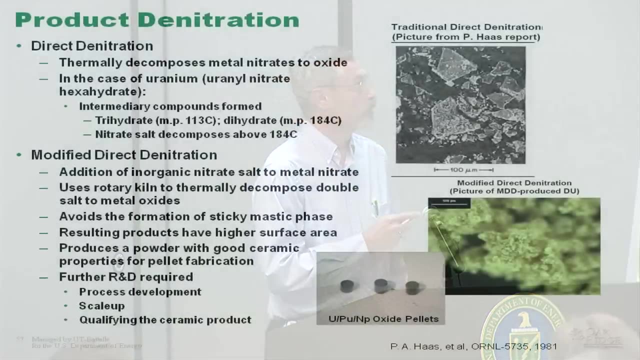 that you ultimately have to grind. Grinding is not necessarily a good process. You have lots of dusting. So a process was developed called modified direct denitration. We added inorganic salt to the metal Nitrate. We use a rotary kiln. 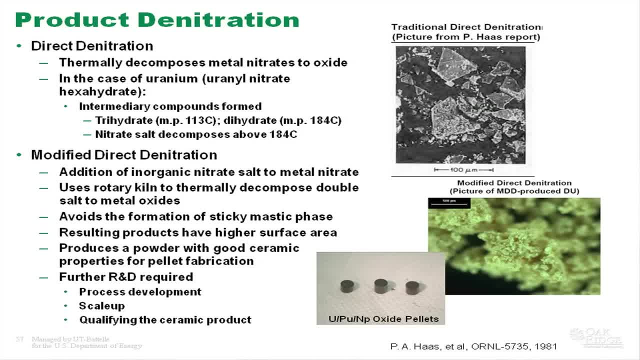 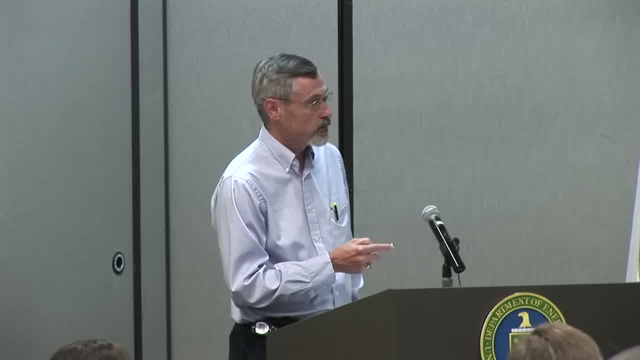 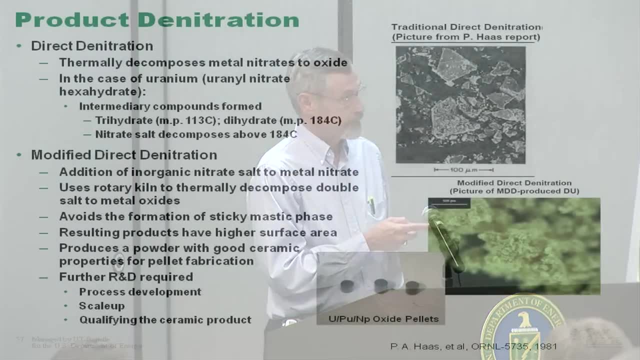 And we decompose that double salt. As it decomposes, it avoids that masty, sticky, nasty phase And you end up with a product that looks like this. No additional grinding is needed. It has a very high surface area And we've demonstrated that this can be converted directly into 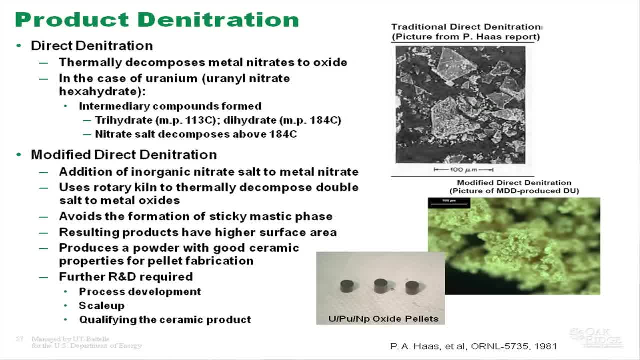 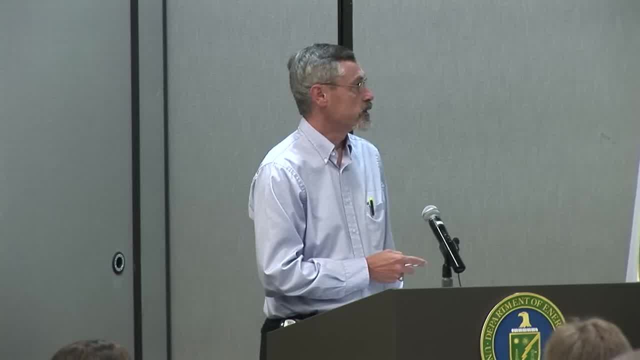 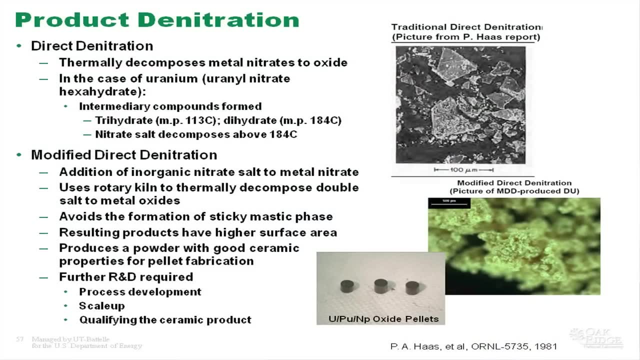 can be pressed into pellets. These have not been sintered. These are, uh, the mixed oxide pellets out of that demonstration run from several years ago. But certainly further developments needed in this area, for process development, for scale-up, for qualifying these products. 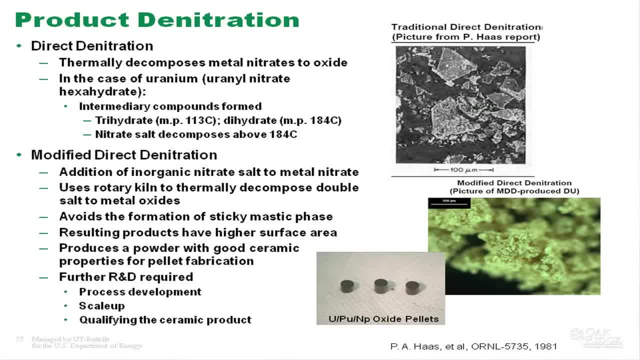 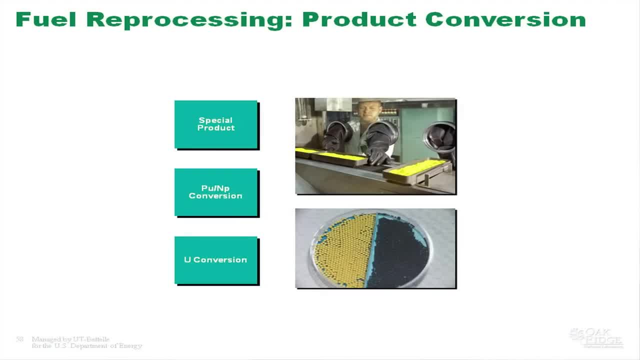 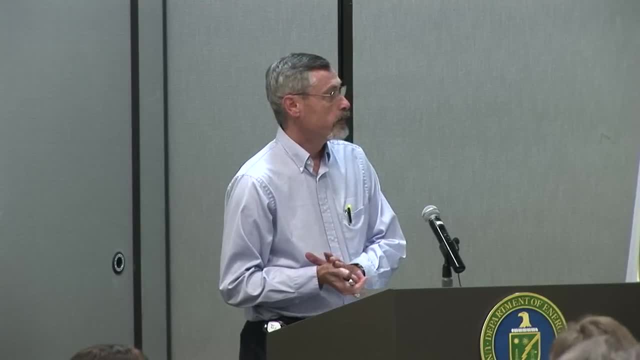 But the advantage of this process was that we certainly avoid the grinding step, And which is a big plus. So, product conversion: You want to go from that liquid phase to the solid phase And we are now down into supporting systems. 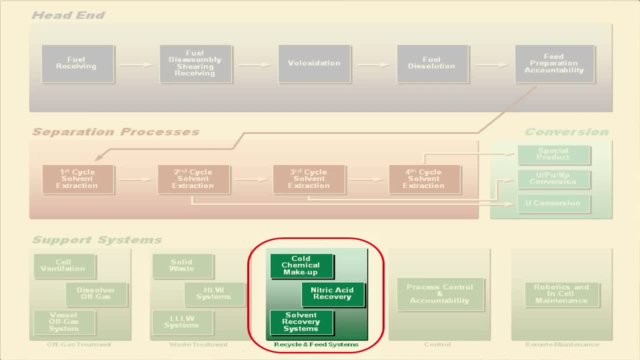 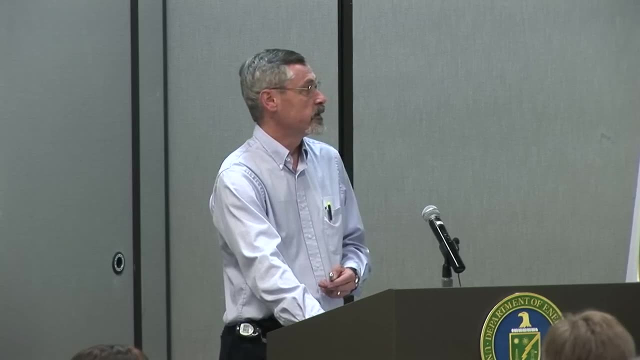 And in the supporting systems. we're talking about things like cold chemical makeup, which I won't touch on, but that's basically. how do you feed the plant? How do you make up all those solutions that you need to feed the plant: Nitric acid recovery and solvent recovery? 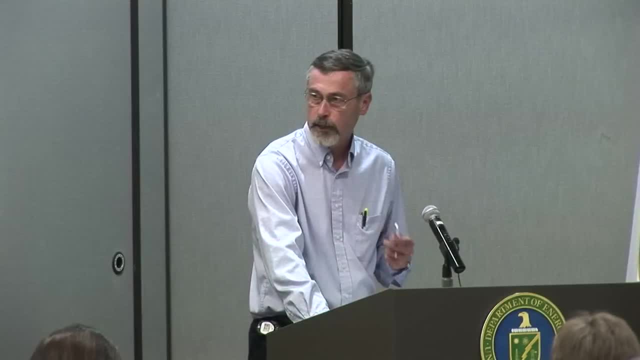 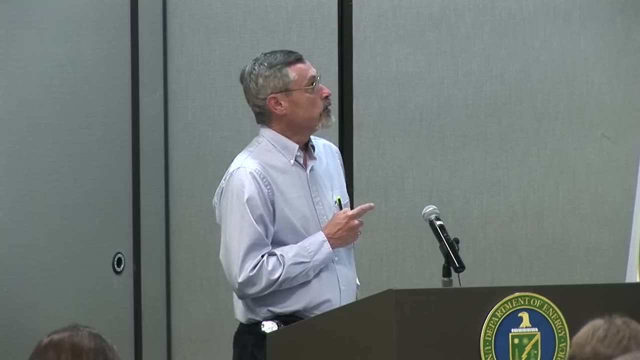 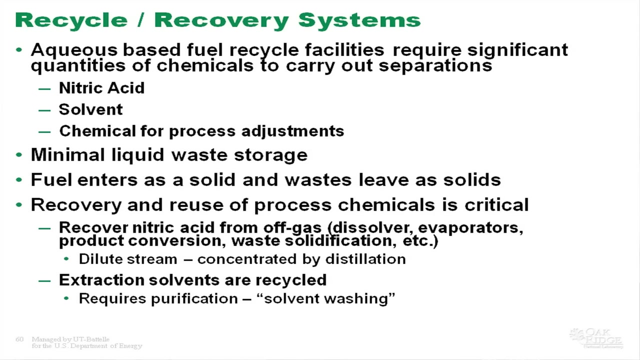 Those are important because you want to recycle as much of the chemicals you add into the plant as you possibly can And you're going to use it for your nitric acid. You're going to use that chemical for process adjustments. You want to minimize the liquid waste storage from the plant. 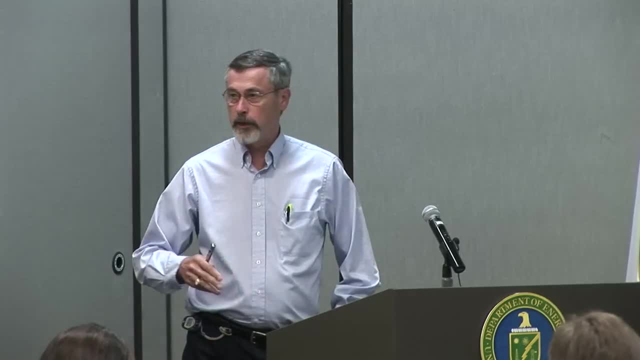 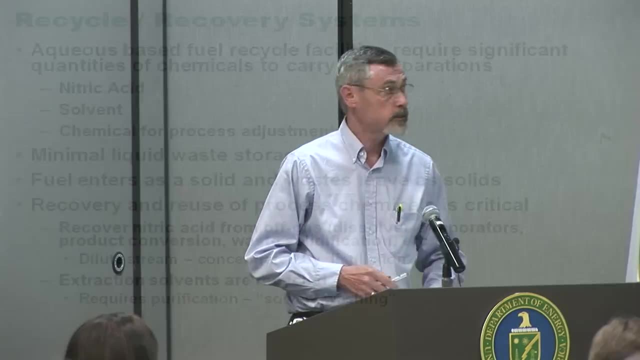 The fuel enters as a solid and the waste leaves as a solid. So what you're left with is: how do you deal, how do you manage all of your solutions inside the plant? And the recovery and reuse is a critical part of that. We recover nitric acid. We recover nitric acid from the off-gas system, from evaporators, from a product conversion step- Remember that was taking a nitrate solution to an oxide. The nitrate comes off. That's a large portion of where that nitric acid went. 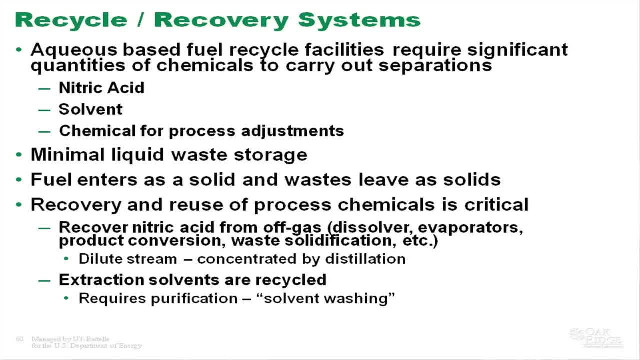 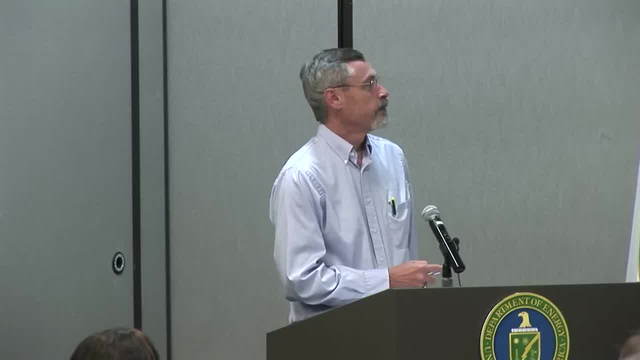 Half of it went into the off-gas stream during dissolution. The other half, of the nitrate, went with the product. So we want to get both those halves back. And then we have a lot of dilute streams that are processed. You'd like to concentrate those dilute streams. 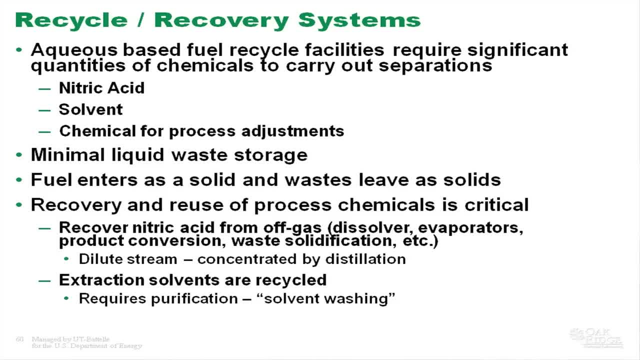 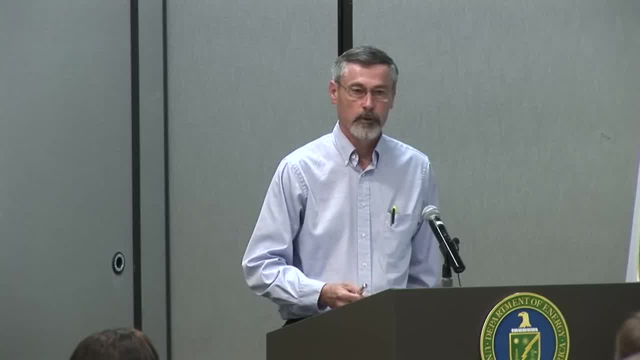 concentrate the acid back up, put it back in where you want it. The extractants are sometimes expensive and we'd like to recycle those. We have to clean them up, remove those hydrolysis and radiolysis products. How do we do that in most cases, 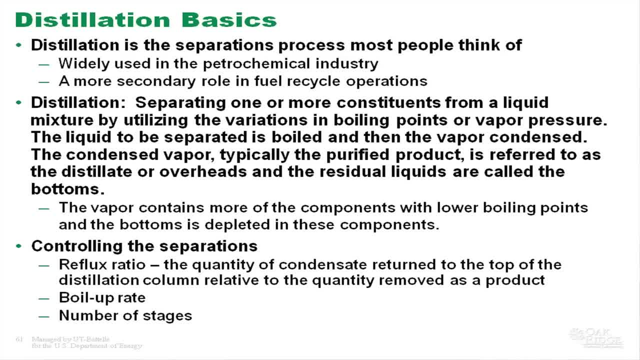 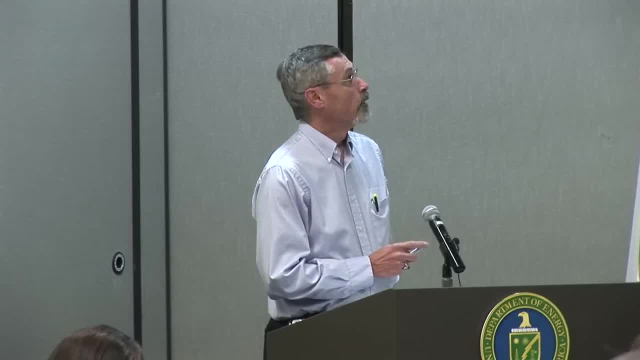 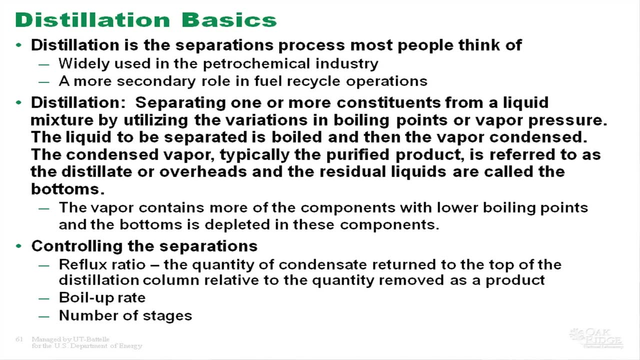 Distillation Pretty common industrial process. It's the primary process in the petrochemical industry. In fuel reprocessing it's more of a secondary role. You separate materials by taking advantage of the variations in vapor pressures. You boil the liquid and you condense the vapor. You do that repeatedly, And as you boil it, those with the higher vapor pressure come off first. They're condensed, and so you're able to effect a separation. Vapors contain the components of the lower boiling points, and the bottoms are depleted in these components. 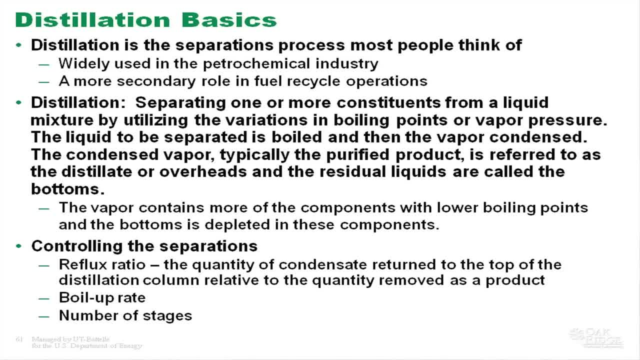 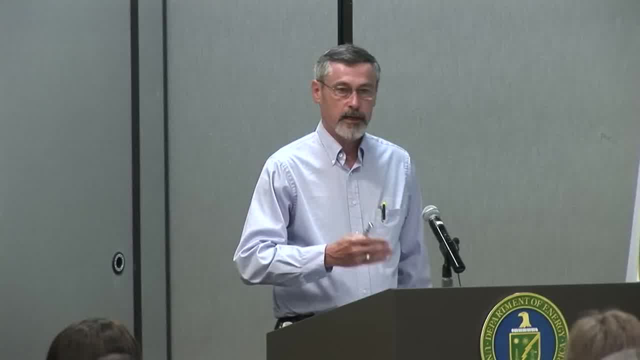 So you've got the bottom of the distillation column. That's where your heavies collect. Those with the lower vapor pressures are down at the bottom. So if we're concentrating nitric acid, you tend to boil the water off the top. 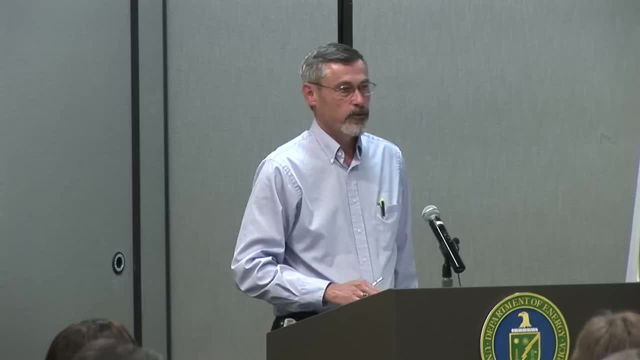 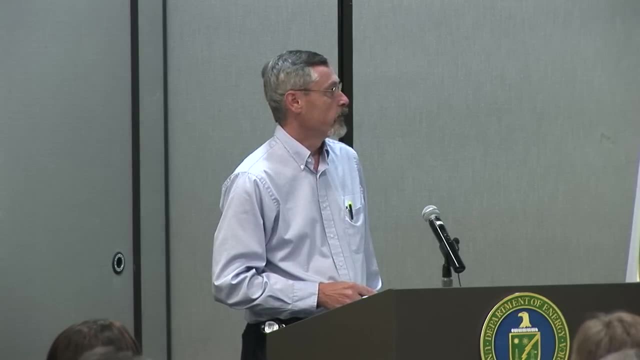 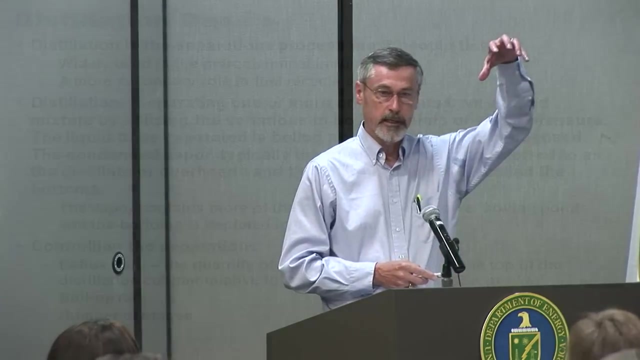 and the nitric acid is at the bottom, Except it has a little thing called an azeotrope where you can only get to a certain concentration without doing rather extreme steps. You control distillation by controlling the reflux ratio. You've got a condenser at the top. 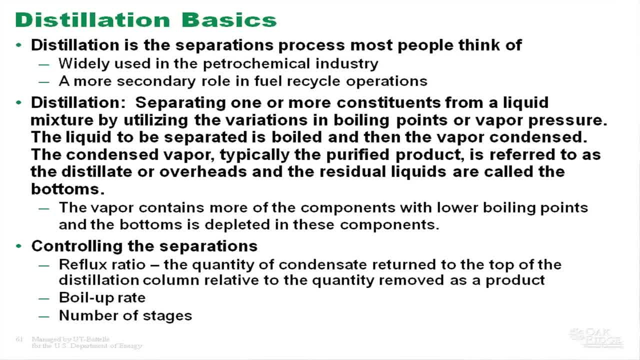 How much do you send back to the column versus how much do you take off? The boil-up rate, how much comes up from the reboiler at the bottom and the number of stages, How many of these boiling condensing, boiling condensing steps? do you have in your condenser? What steps do you have in your column? Primary applications: nitric acid recycle. A 800 metric ton per year plant requires a million liters of concentrated nitric acid a year. That's a lot. It accumulates corrosion products. 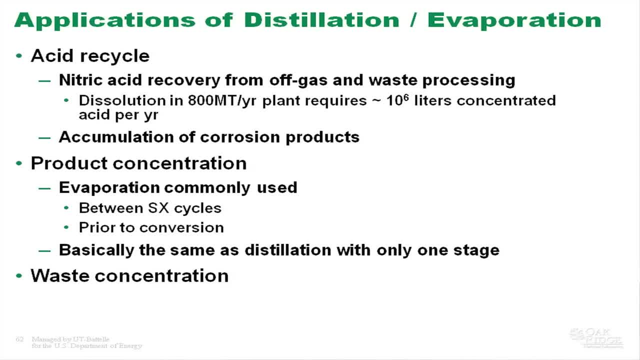 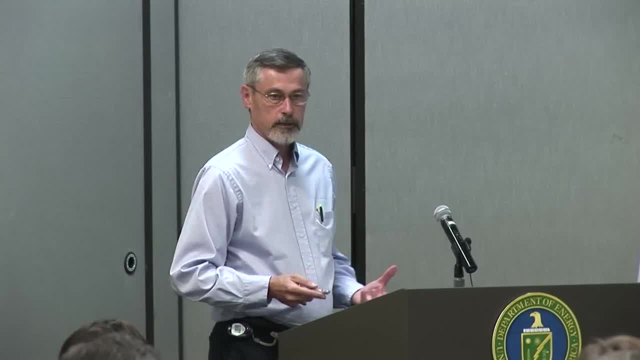 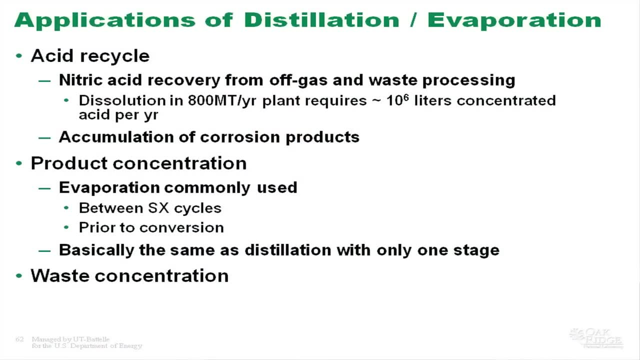 Those will be collected in the bottoms of the tank. You do have to remove corrosion products. Your nitric acid eats away at your plant, So those will collect in your solutions. We concentrate the product. There's evaporation potentially between solvent extraction cycles. 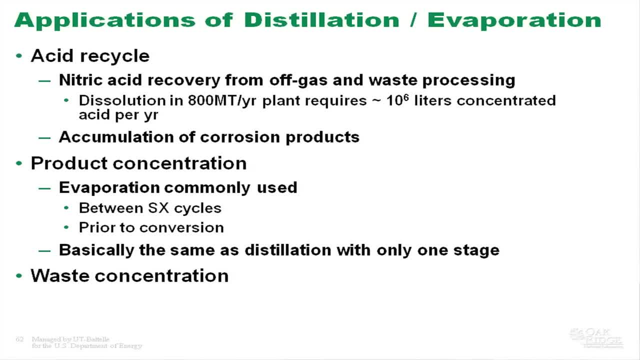 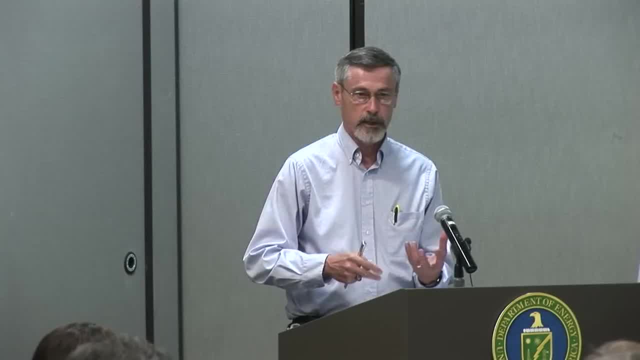 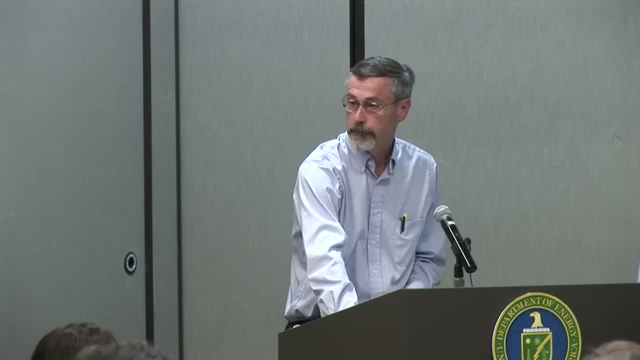 and certainly before the product conversion steps. It's basically this is evaporation, That's basically distillation for only one stage. You have a tank, you heat it, you have vapors coming off, The materials stay in the tank And then in waste concentration before you go to a. 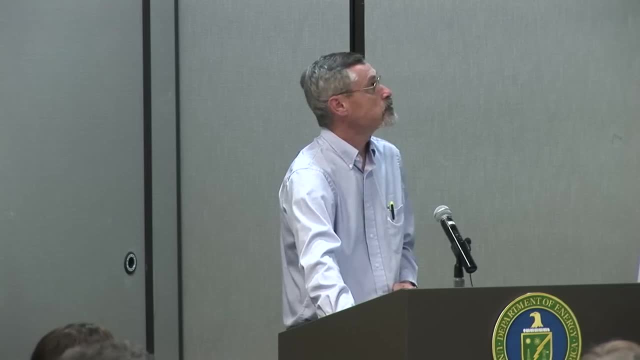 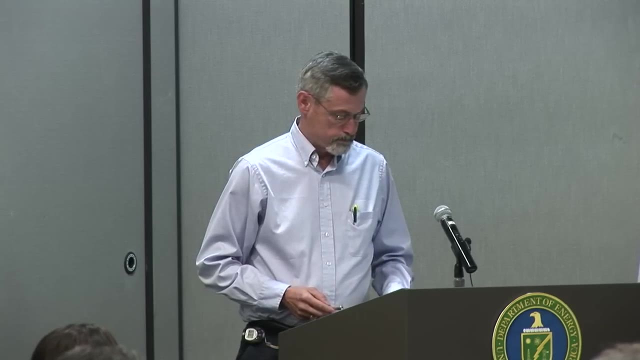 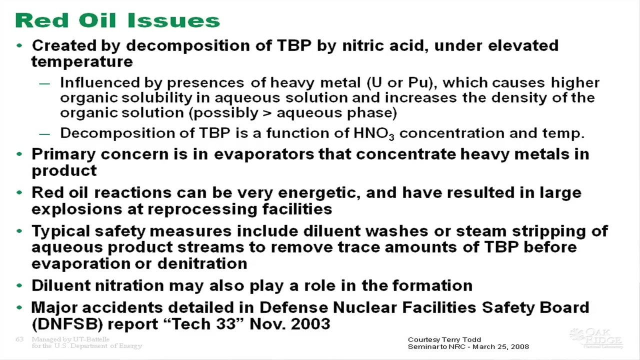 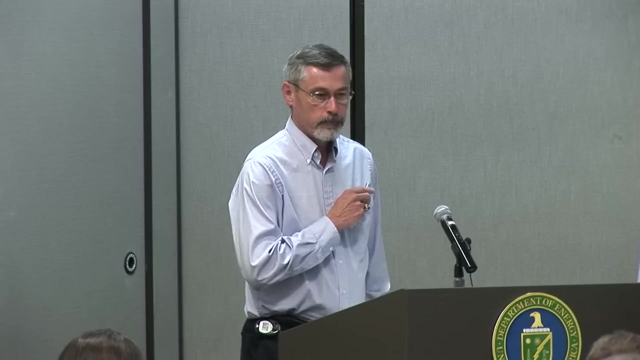 let's say a vitrification system. That's not all without some concern. You may have heard of red oil. Well, red oil occurs by the decomposition of tributyl phosphate in the presence of nitric acid at elevated temperatures. The most notable case is the incident at Tomsk. 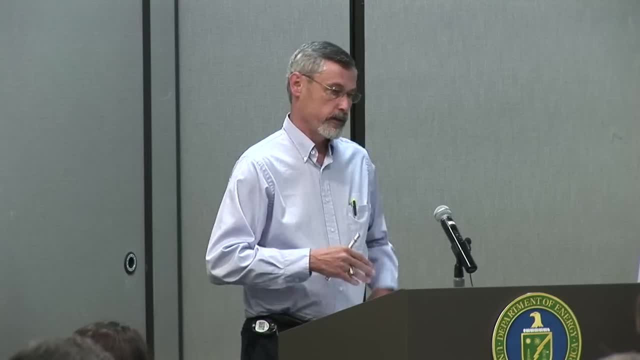 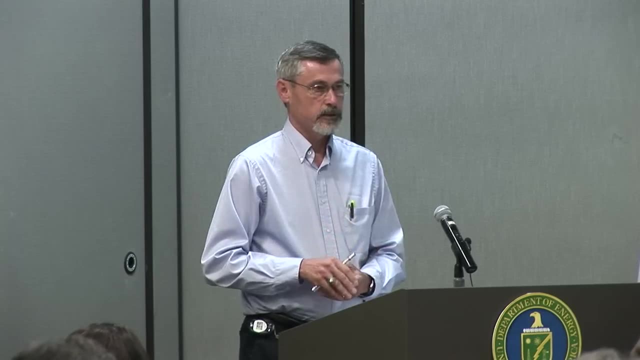 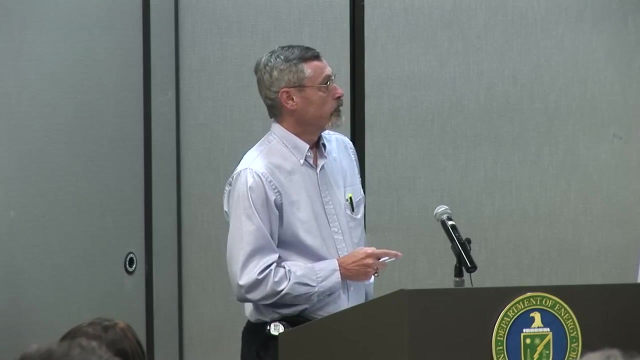 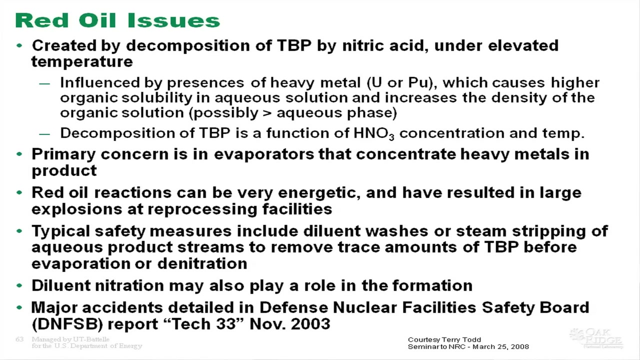 where they managed to trap a layer of organic in a vessel, heated that vessel up, It nitrated, It exploded. They blew the wall out of the facility. They can be very energetic And the typical approach is you use something called diluent washing. 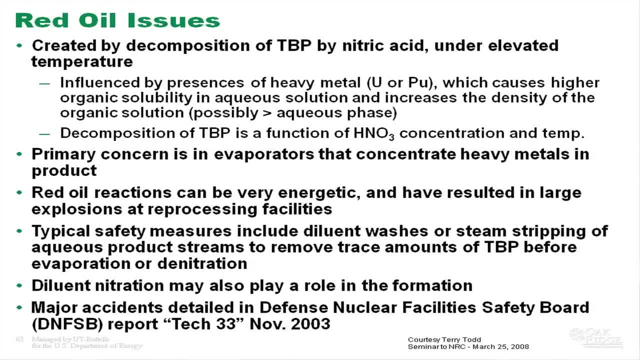 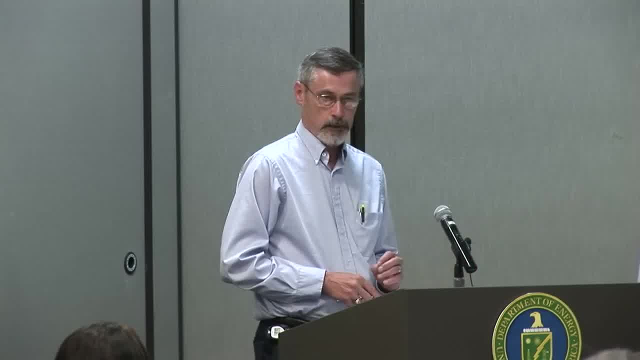 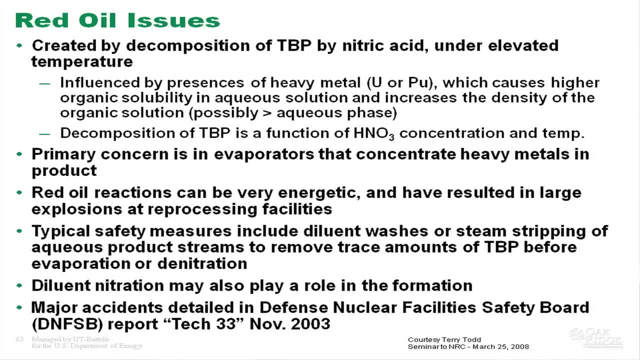 which I'll come to, or steam stripping of the aqueous product stream to remove any trace organics that may be carried with the aqueous phase Early on. I implied that we're looking at immiscible streams. They are immiscible. but they may, through the design of the equipment, have a small amount of carryover of very fine droplets and they also can dissolve small quantities of the organic into the aqueous phase. So there is a small amount that makes it into the aqueous phase. 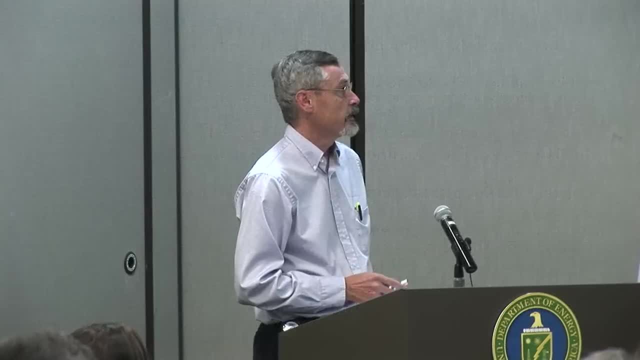 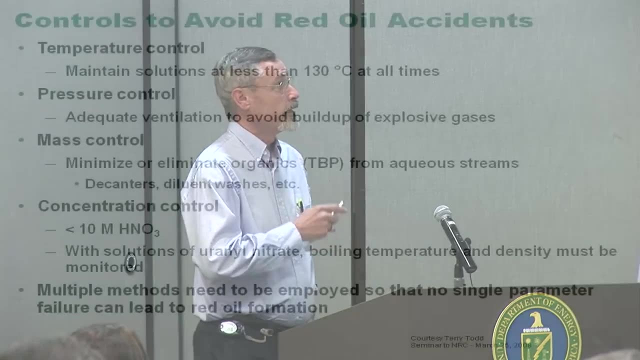 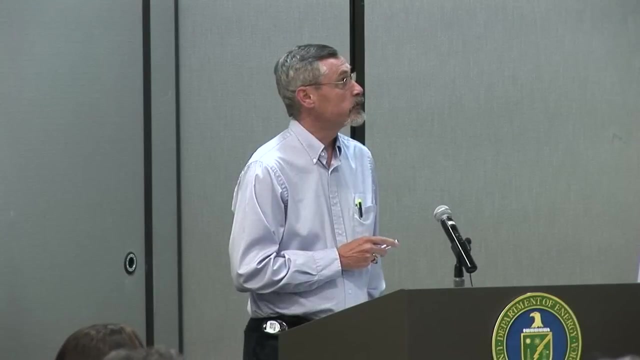 and we want to remove that before we go to an evaporation step. So we control that by maintaining, by doing evaporations at temperatures less than 130 degrees C, controlling the pressure, adequate ventilation so you can't have a buildup of pressure in a tank. You minimize the quantity of organics that could get into the aqueous stream. decanters, diluent washes. You control the concentration- Don't let it get above 10 molar nitric acid- And you may apply multiple methods so that you don't rely on a single method of failure. 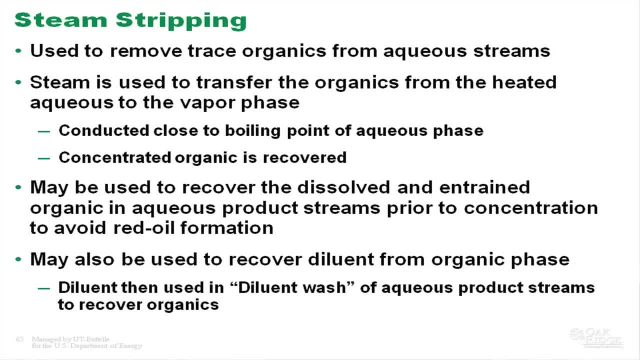 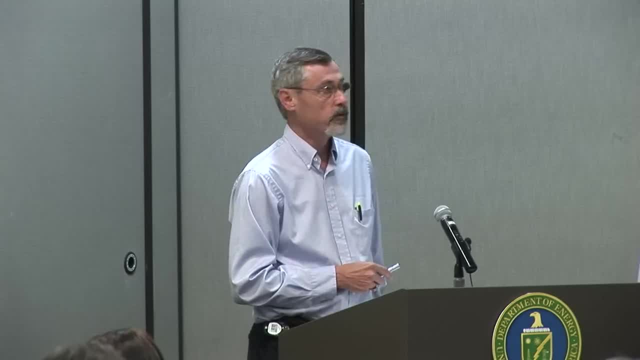 Steam stripping is basically applying steam to a system. The vapors collect the organic phase. When you heat that, you pass steam through an aqueous phase and the steam carries over some of the organics. You may then use that to recover the dissolved or entrained organics in the aqueous product streams. We also have used steam stripping to recover diluent from the organic phase. The diluent is that kerosene, and typically it's 30% TBP, 70% kerosene. 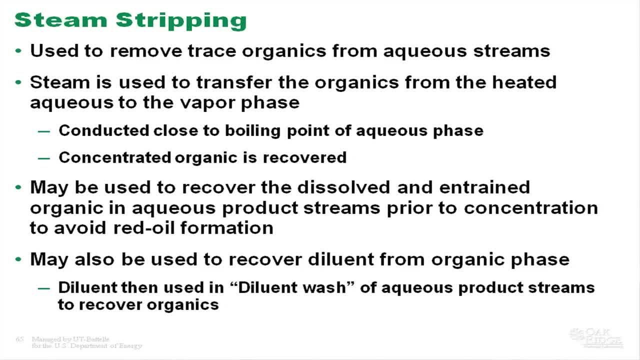 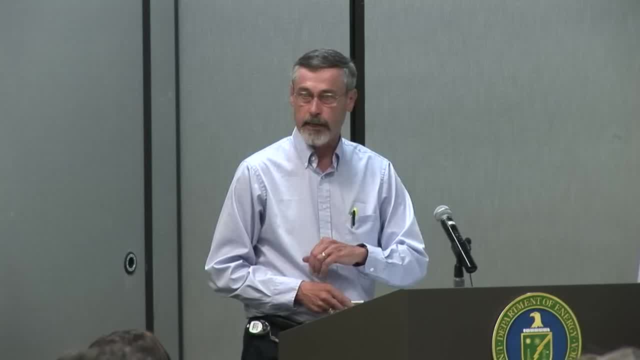 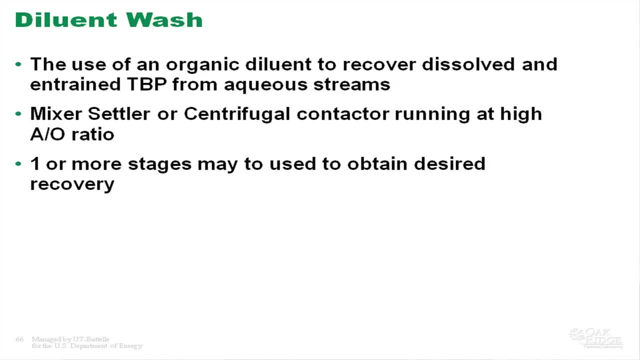 If we're going to do diluent wash, we may want to recover diluent from that material. use that to wash the aqueous phase It goes back in and we're not adding extra diluent to the plant. Diluent wash is basically another solvent extraction system. 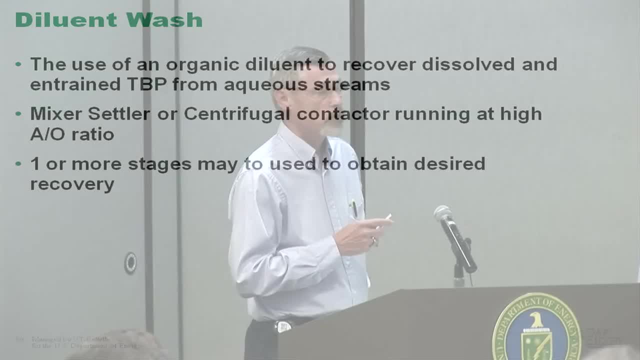 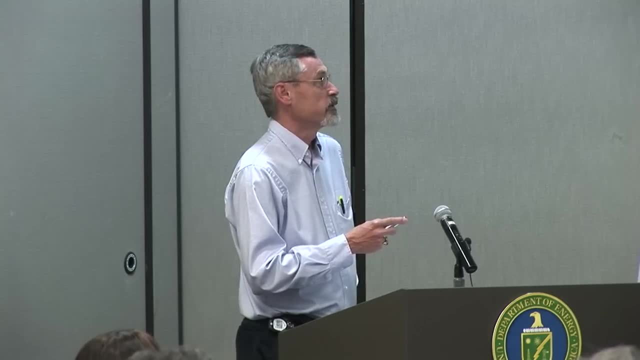 It's a very simple step, except that we're washing the aqueous phase with the organic diluent. It pulls the TBP out of the aqueous phase. We do it in several centrifugal contactors or mixer cellars running at a very high aqueous-to-organic ratio. 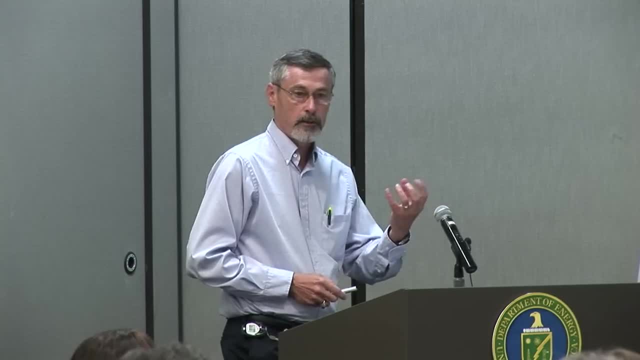 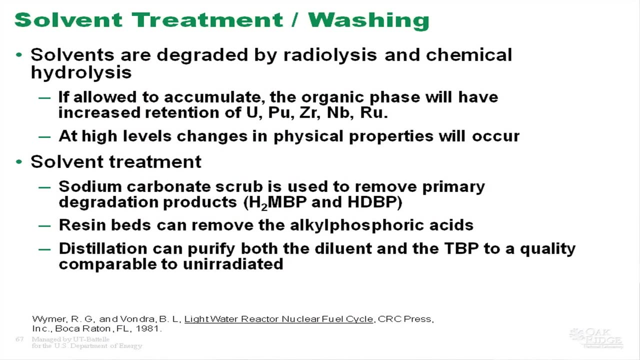 And we may use one or more stages to that Very high aqueous-to-organic means. you've got a very small amount of that organic phase trying to gather up that small amount of TBP. The other step is to remove those products that are created by radiolysis or chemical hydrolysis. 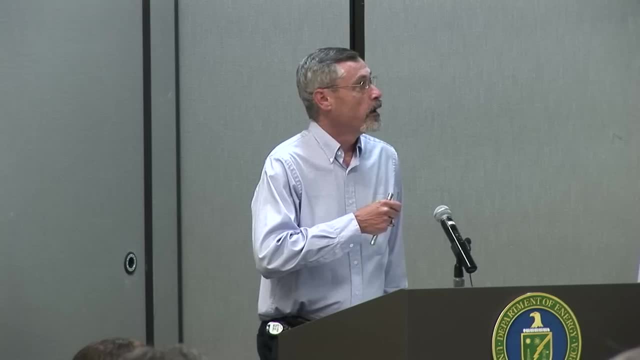 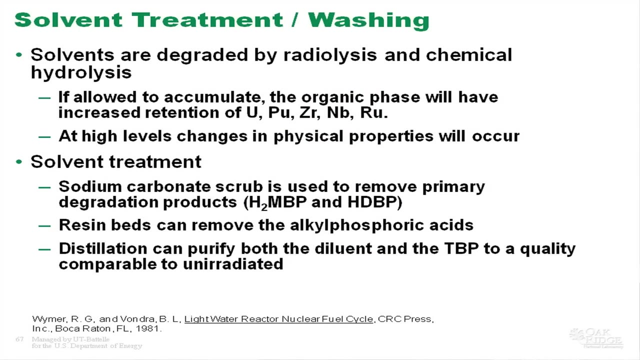 that, if allowed to accumulate, will tend to accumulate a number of species in the organic phase that you don't want there and that you can't remove Typically solvent treatment. the first step is a carbonate wash That removes the DBP. 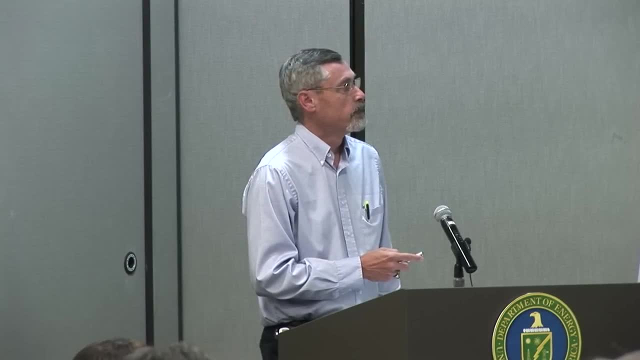 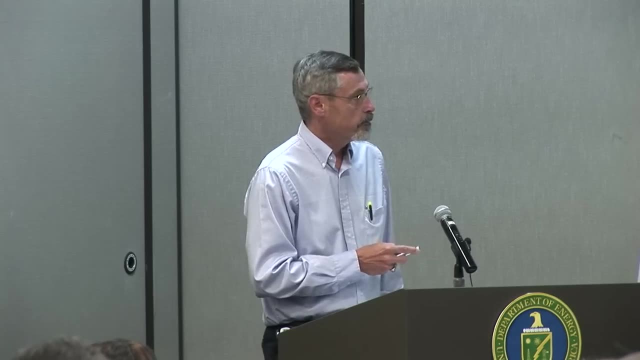 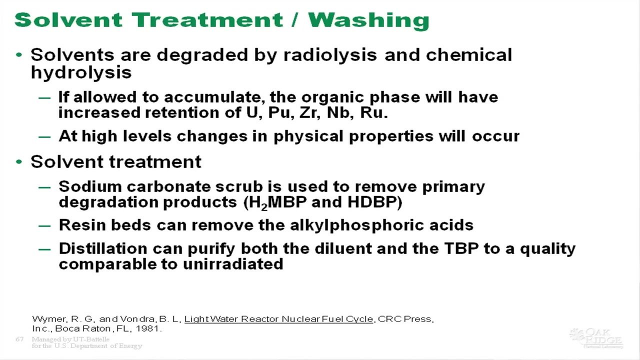 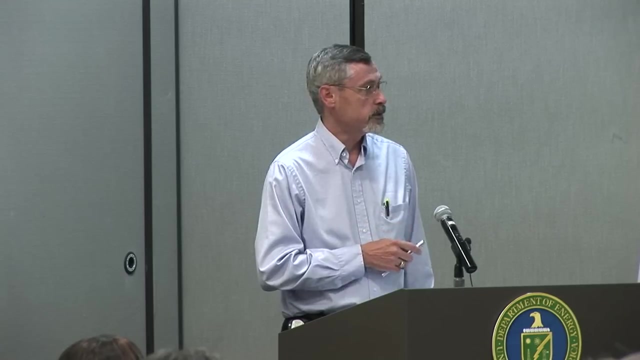 the dibutyl phosphate and the monobutyl phosphate from the tributyl phosphate. You can then pass that through a resin bed to further purify it And finally you can, by distilling the organic phase, return it to virtually the quality. 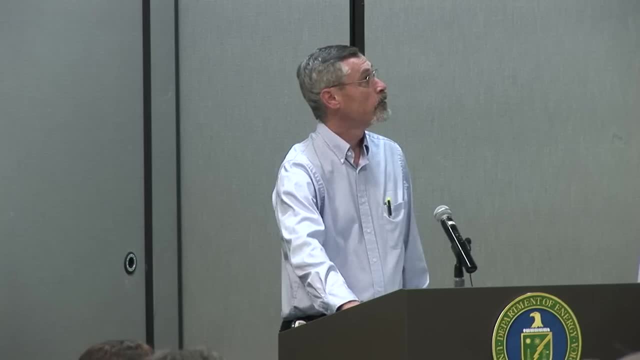 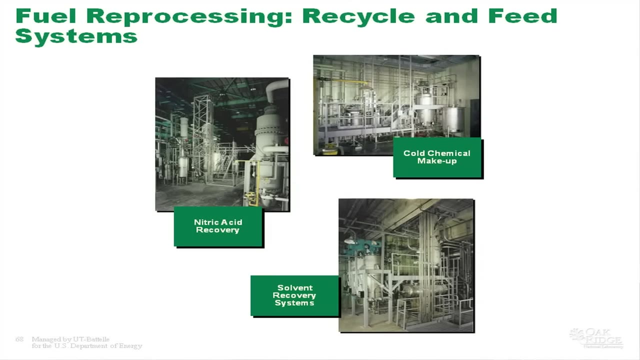 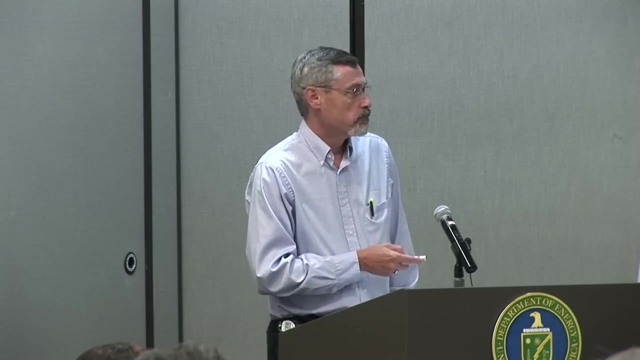 of unirradiated material. So what do those processes look like? Pretty standard chemical engineering: pieces of equipment, Distillation columns, tanks for making up chemicals, blend water, blend, nitric acid, blend, reducing agents, whatever. you need pretty standard stuff. 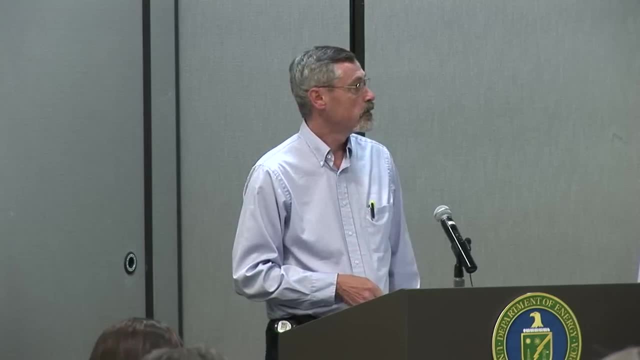 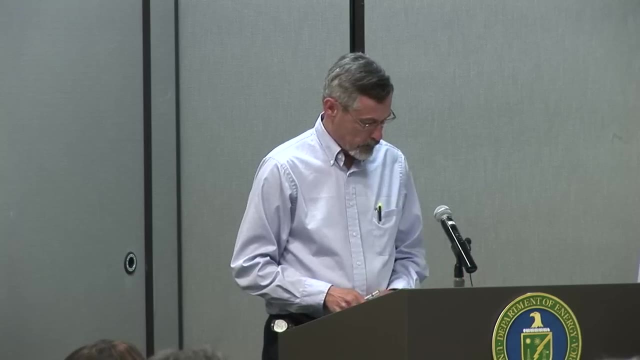 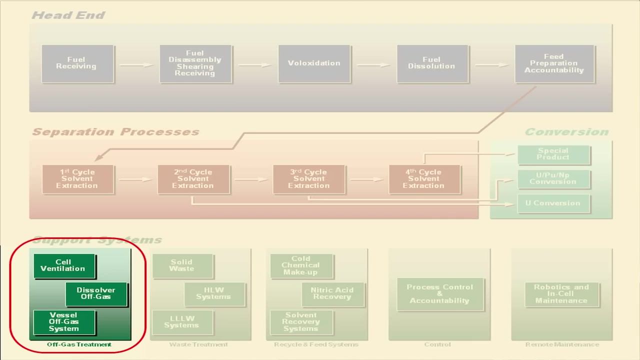 Solvent recovery tends to be mixer cellars, And our last major topic will be off-gas treatment, And it's important because that is a stream that you can't accumulate in the facility. You release volatile components virtually every step along the way. But, unlike the aqueous solutions which you can contain in a tank, these are emissions that leave the plant and are carried, certainly, by the winds. The typical species that we're worried about are tritium, with a 12-year half-life. carbon-14, with about a 6,000-year half-life. 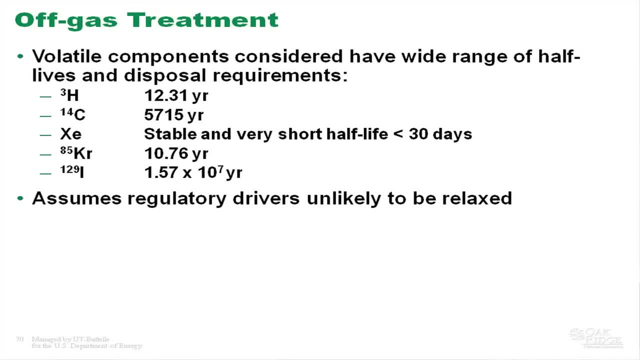 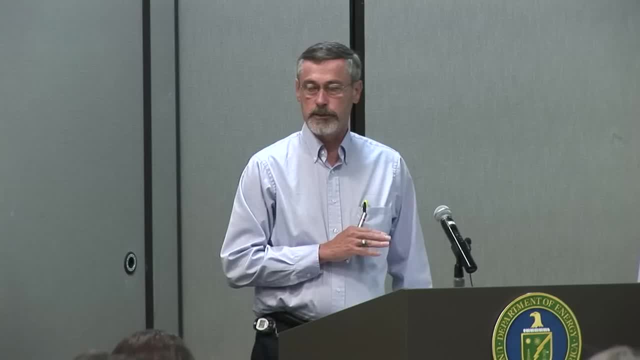 Xenon's up here, but there's no xenon isotope with a half-life greater than 30 days, So all the xenon we're talking about is stable Krypton with about an 11-year half-life. Krypton-85,. excuse me, 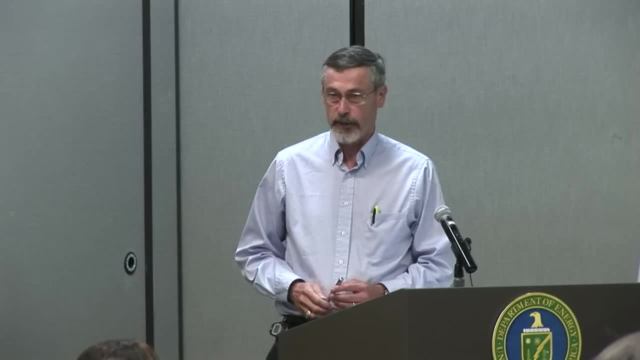 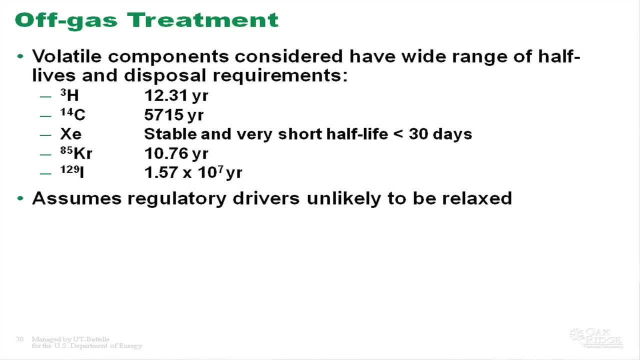 and iodine-129, with a 16-million-year half-life, Some of these- and we're assuming that we're going to be having to capture most or all of these, based on the fact that I'm assuming that regulatory drivers are unlikely to be relaxed. 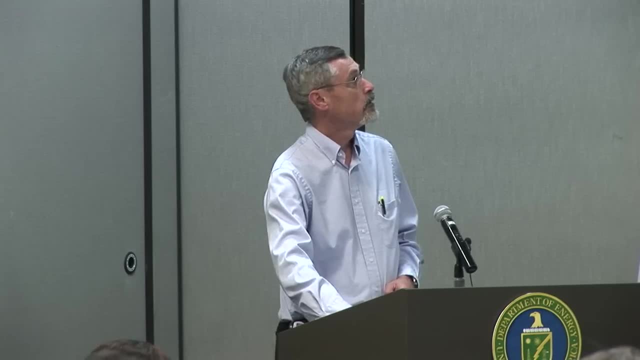 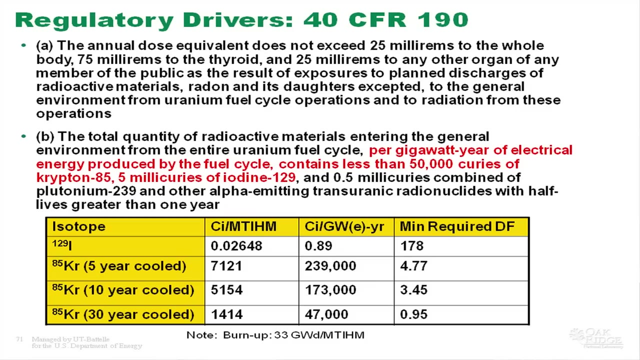 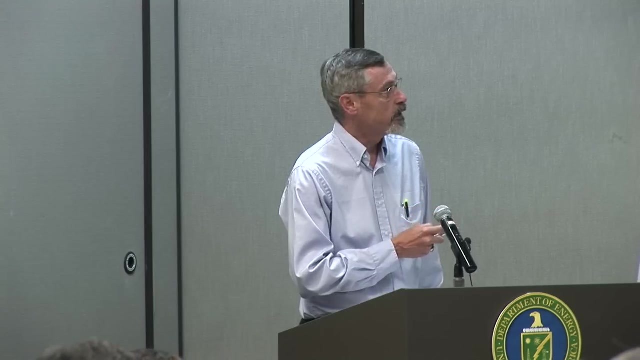 on the emissions from the plant. What are some of those? what are those regulatory drivers that we're talking about? And there are really three that I want to mention. 40 CFR 190 is a unique regulatory driver because of these words: It's the release of Krypton-85 and iodine-129. are based on the energy production from the fuel. So it's 50,000 curies of Krypton-85 per gigawatt year of electric from the fuel cycle. It doesn't say where in the fuel cycle. I'm assuming it's all from reprocessing. but if it's anyplace else, that limits reduces the amount that can be released from the reprocessing plant. Five millicuries of iodine-129 per gigawatt year electric. Doesn't matter what size the plant is, it's based on the burn-up of the fuel. 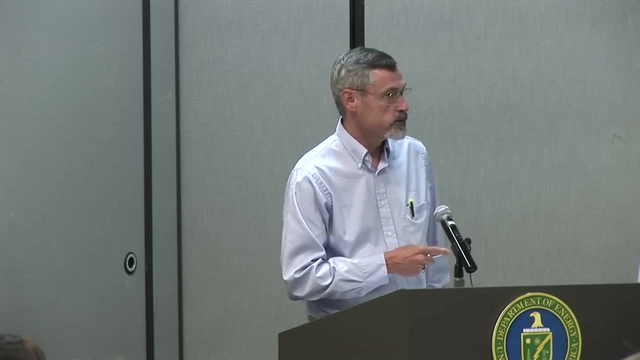 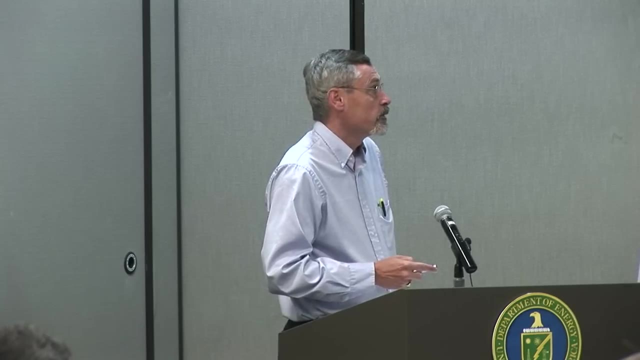 So, if we look at, what do those numbers mean in terms of recovery efficiencies or decontamination factors that we have to have in the off-gas stream? How much do we have to recover For iodine-129,? 60 million-year half-life? it doesn't matter how old the fuel is, it's still all there. We have to have a minimum DF of 178 for this age fuel And it tends not to change much with burn-up of the fuel because while the total mass of these materials 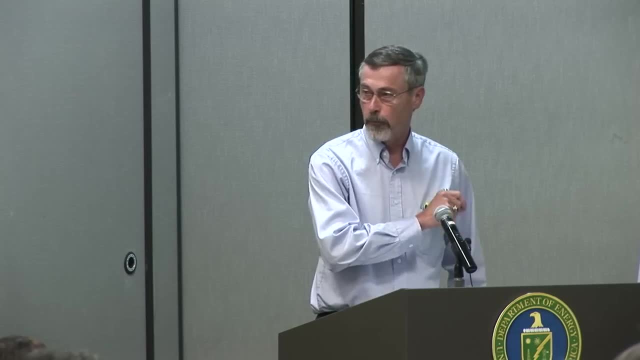 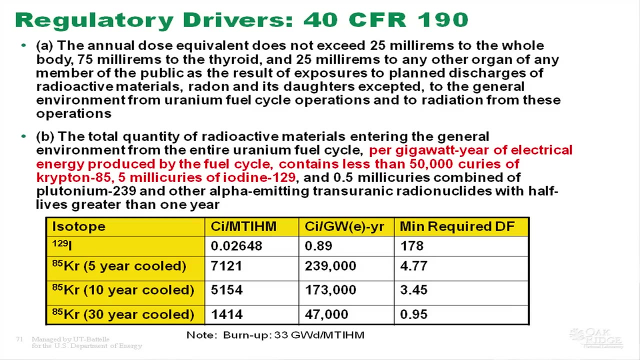 increases with burn-up. you also have more energy produced by the fuel. so the gigawatt year electric goes up. So DF of 200.. No engineering margin. no, nothing on this. We've got to get less than a half a percent. can be released. For krypton cooled five years fuel cooled five years, we need a DF of about five. That's not too hard to obtain. If we go to 30-year cooled fuel the DF drops below one That says we may not. 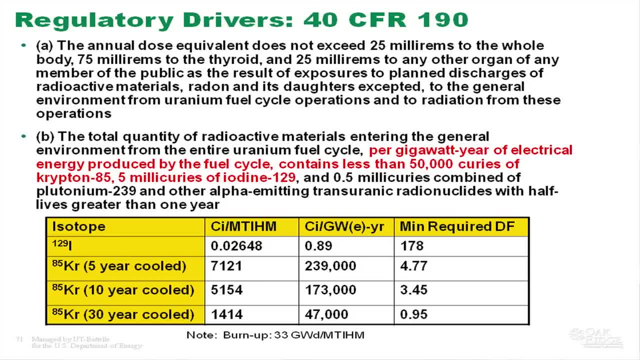 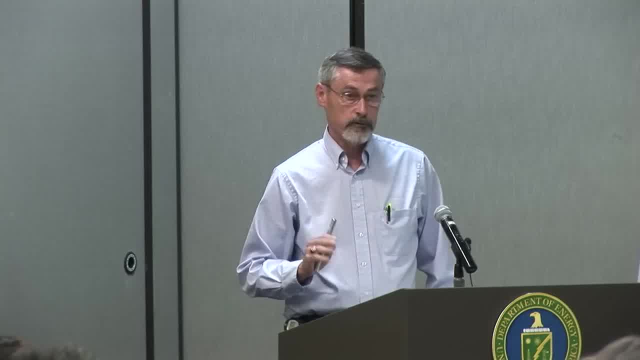 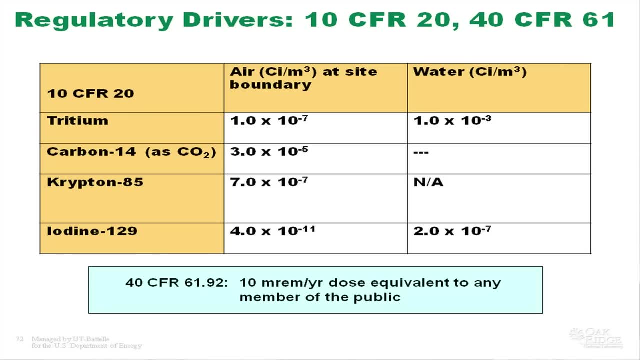 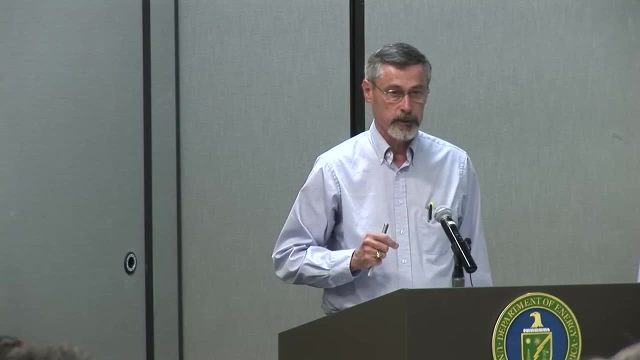 based on this regulation, have to capture krypton-85.. Remember, no engineering margin. Two other regulatory drivers: 10 CFR20, 40 CFR61.. 20 CFR20 gives you concentrations for these species at the site boundary. Now, what don't I know. 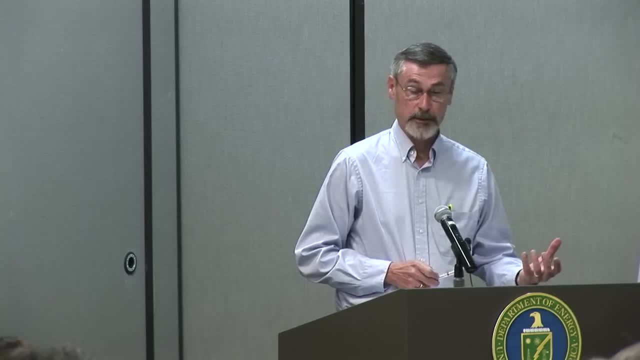 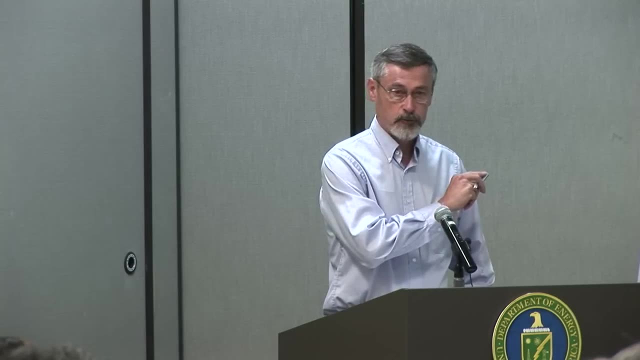 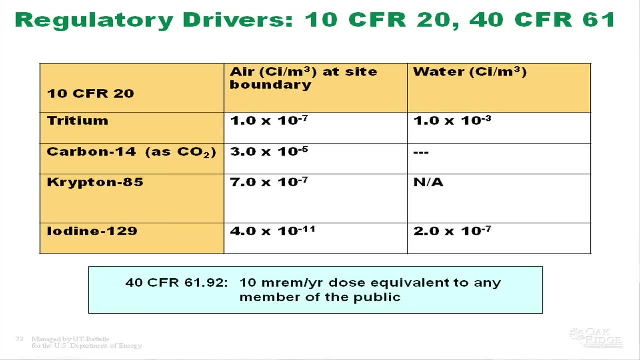 I don't know where the site is, I don't know what the meteorological conditions are, and I don't know how big the site is. I also don't know how much fuel I'm producing or processing. So these numbers are dependent on at least those four factors. because the more fuel you push through the plant, the more you're going to release. These numbers didn't change, So I'm going to have to. that will drive me to higher rates for recovery factors because of the limits of the site boundary. 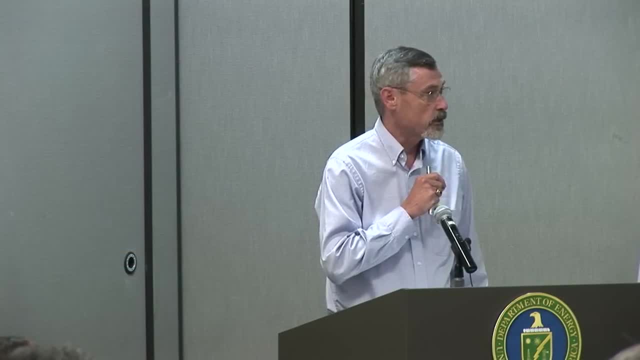 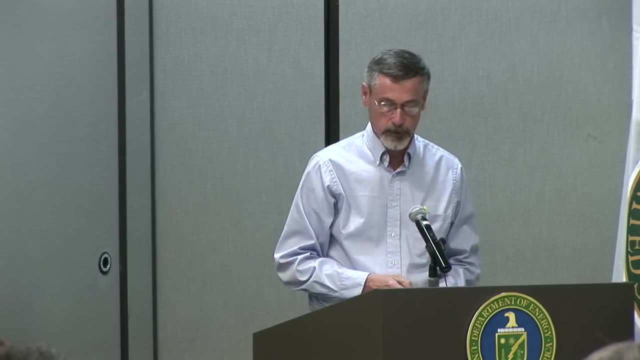 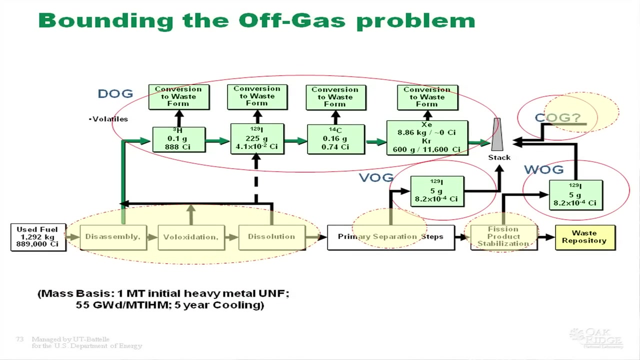 40. CFR60 is very much the same way. It's based on dose to any member of the public. Again, the more material you process, the higher the recovery may have to be. All right, now we're just going to focus on the recovery of the volatile components. 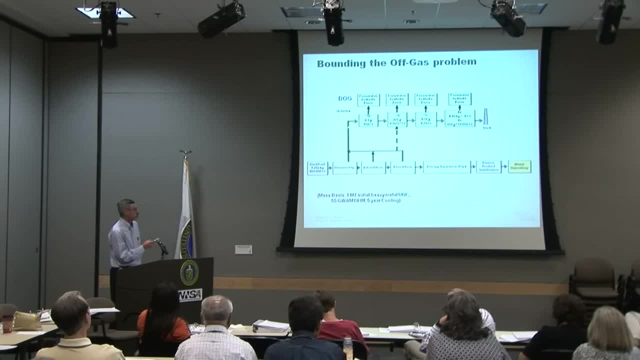 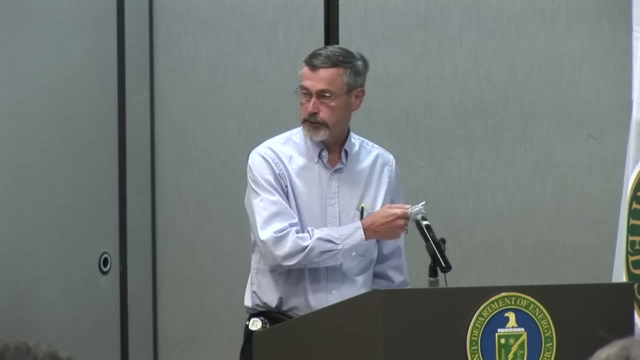 Got the fuel thing. Where can they come off? You can get releases from disassembly. When I chop the fuel up, I'm going to release some of the krypton- Alan talked about that yesterday, being in the gas plenum- If I have voloxidation. 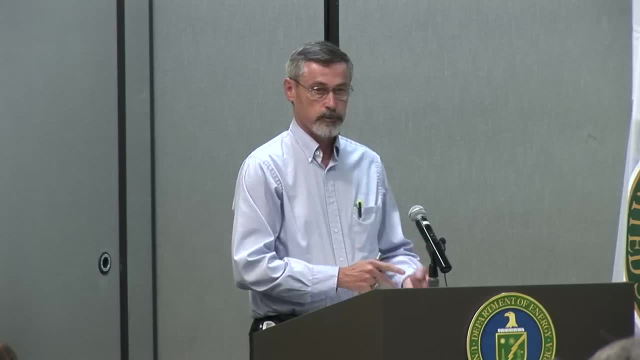 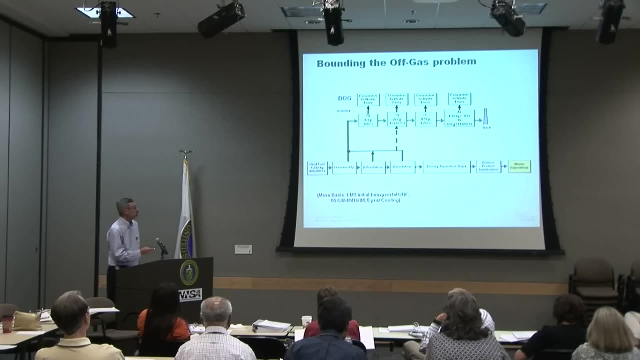 I'm certainly going to release the tritium. If I do dissolution, it's. krypton, iodine, carbon-14 are all going to be released into that off-gas stream. Well, I have very. that's a tenth of a gram. 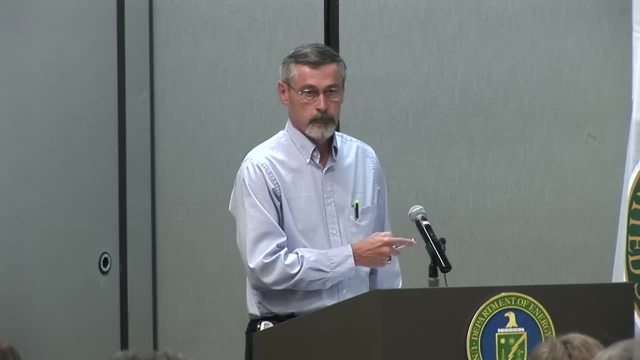 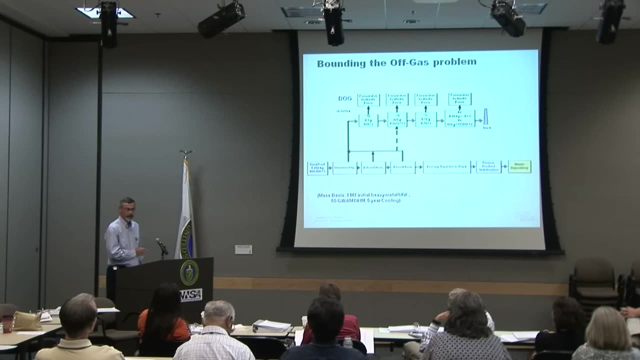 that I've got to capture. per kilogram of material or per metric ton of material- That's two fuel assemblies- I get a tenth of a gram. I've got to go after that and get a DF of maybe 100.. Iodine I've got to get. 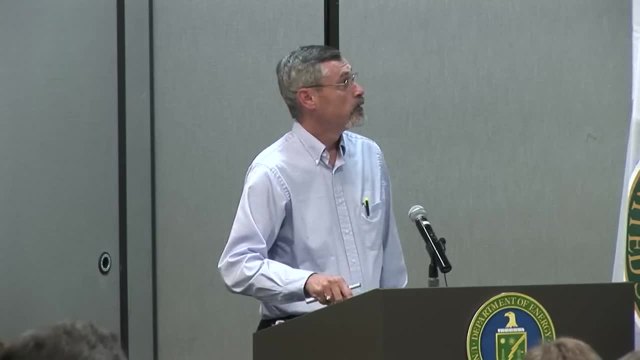 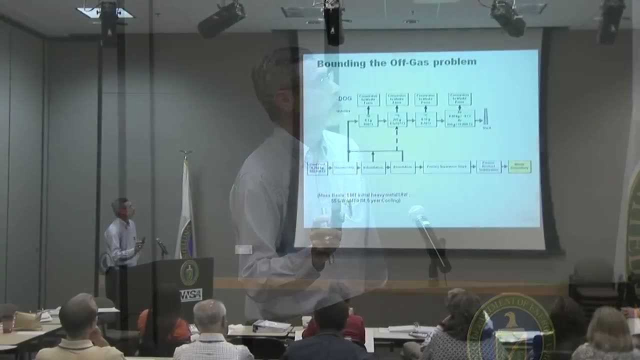 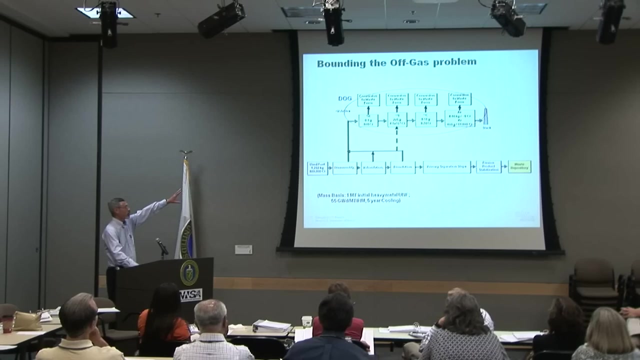 all but a gram or two. It's a pretty tough challenge there. Well, click, click, click. okay, So that's what I'm going after. on the head-end off-gas system, Click. But I have other streams, All of these other tanks. 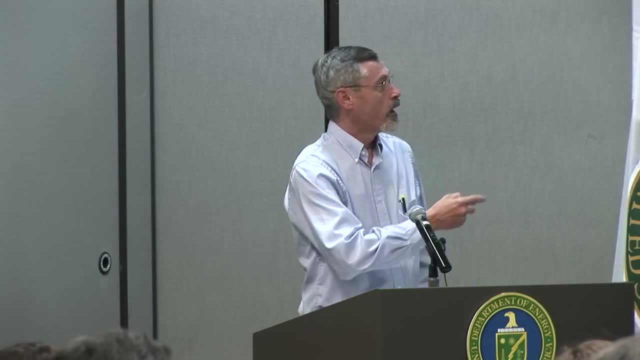 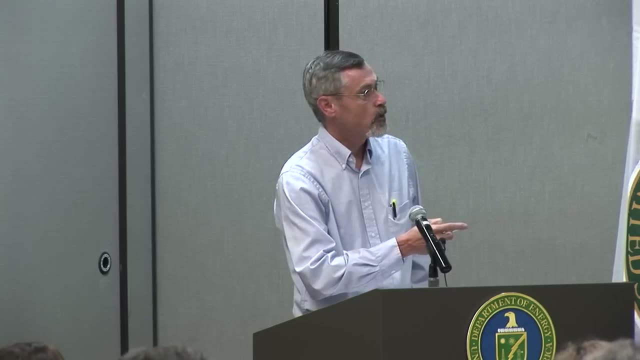 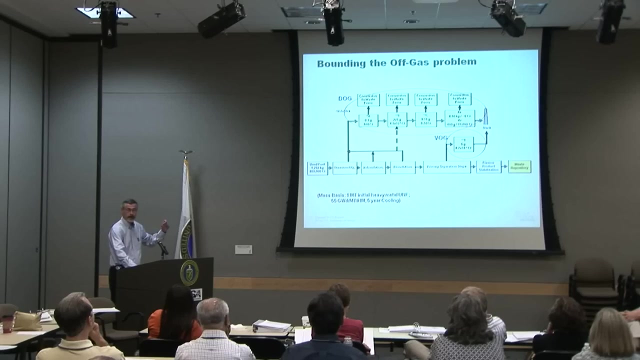 have ventilation systems on them. Iodine may move down through the dissolution process and into the separation steps. So I have a small fraction of the iodine click that may have to be recovered To get to that very high DF And I'm probably targeting at least a DF of 1,000. 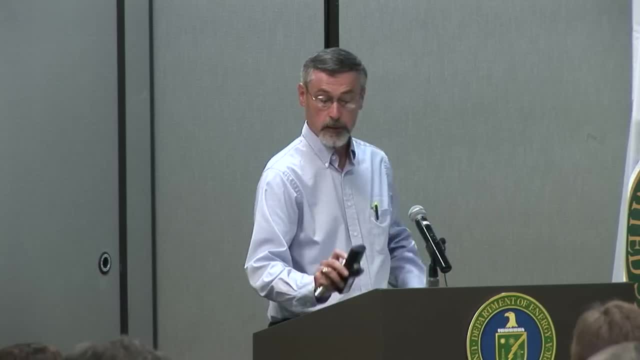 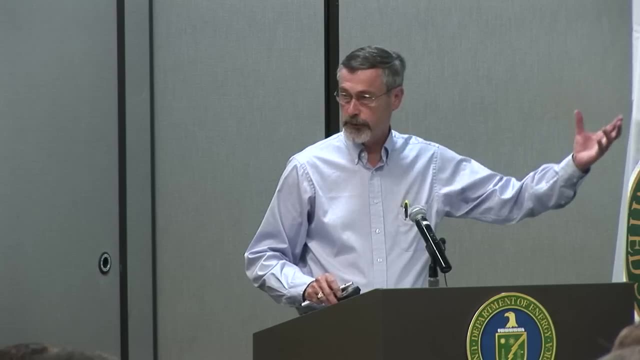 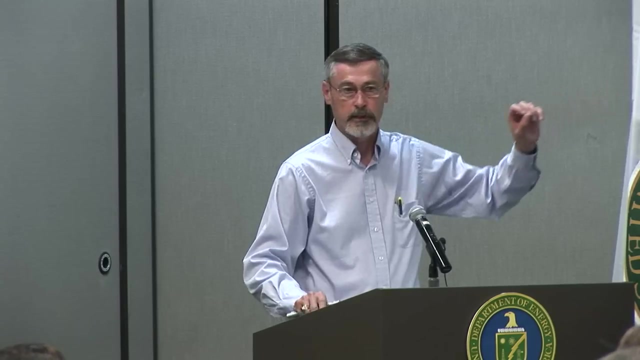 to have an engineering margin of five in there. So click Now when I get to the waste processing. any that was not released during the tankage may come off during the waste processing steps. Again, I have to capture it here because it's per gigawatt-year electric. 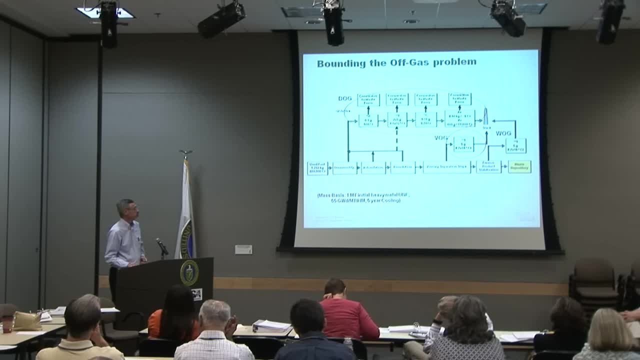 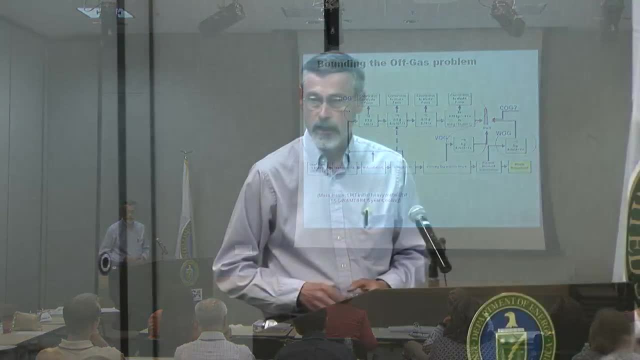 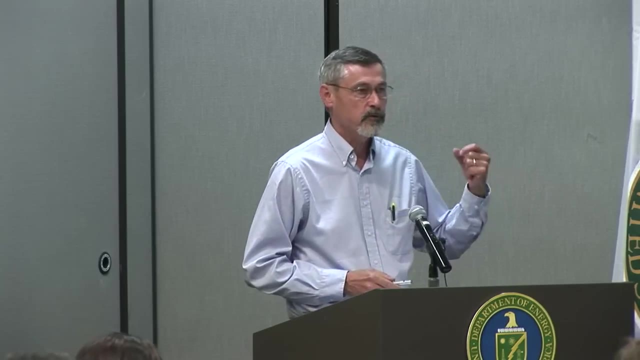 It's not a composition issue. So click And click again. What about the cell off-gas, This whole, this hot cell? Any releases into the hot cell have to be managed. They have to be treated also. So click, Have to manage those streams. 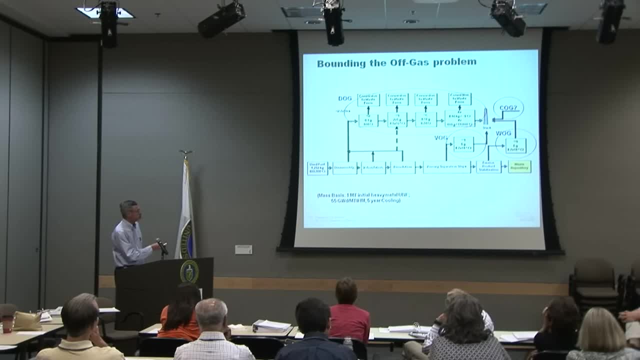 What's happening as we go from each of these? This is a fairly small off-gas stream. This is larger, Becomes much more dilute. This is even larger And this is probably the largest one of all. So what do you want to do? 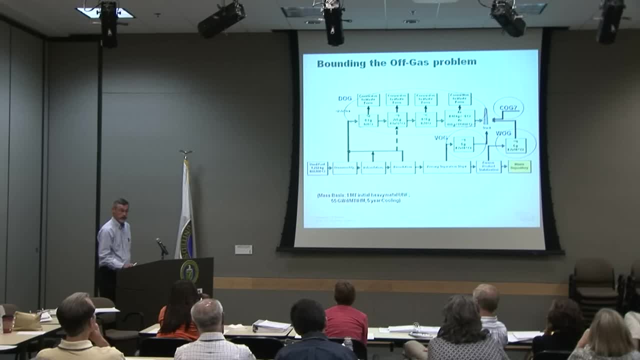 You'd like to manage these streams in as concentrated a form as you possibly can Click. So it's: how do you control these processes to evolve what you need into the off-gas system? Click, Click And click. So that's where the source terms are. 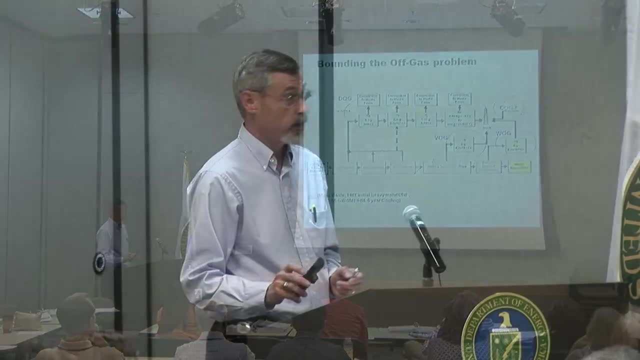 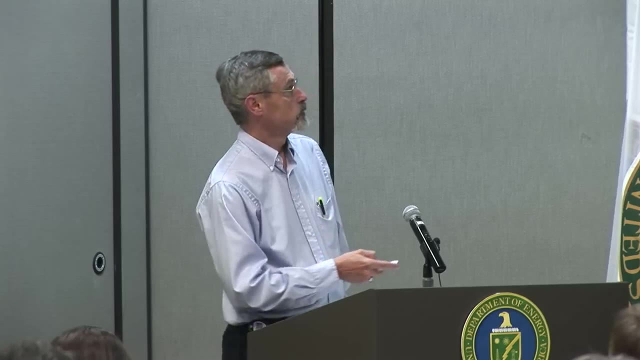 That's what we really want to know, And we don't know them all real well. So, click, We do know what the compositions are of the streams We're looking. Okay, So we're looking at krypton-85, but that's a very small amount of the total krypton. 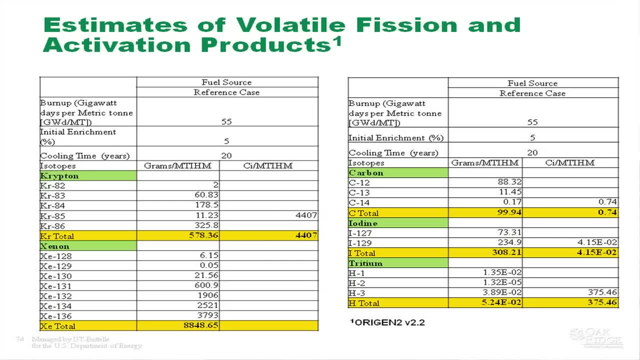 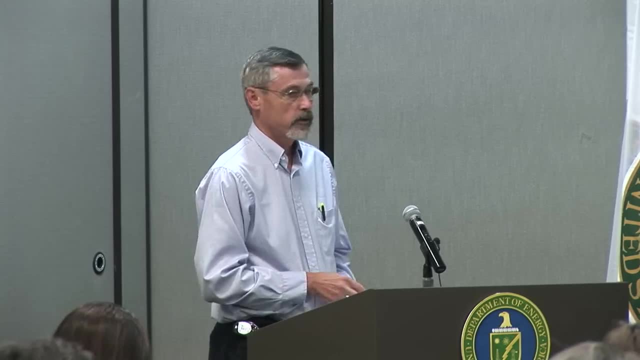 Xenon, not radioactive, but it's going to come off with krypton. Eight kilograms of that material. Gram quantities here: Carbon-14, very small, Dwarfed by the carbon-12 and the carbon-13.. Okay, Click. 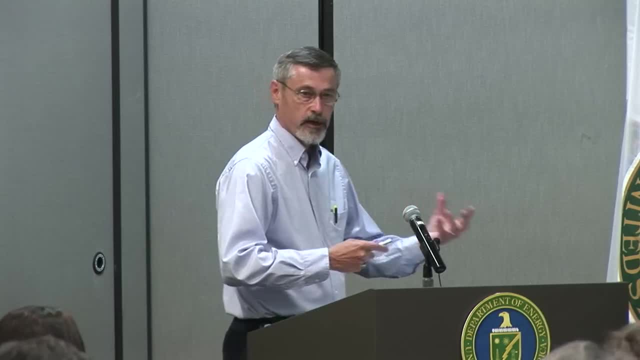 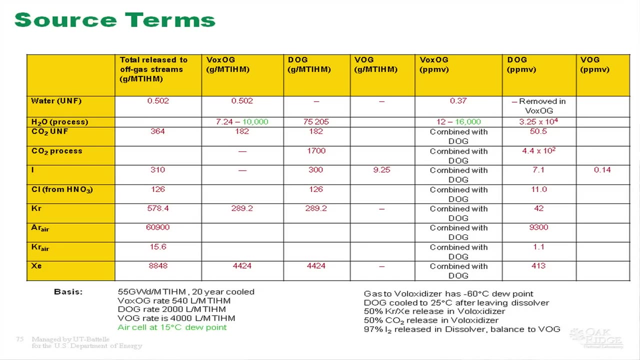 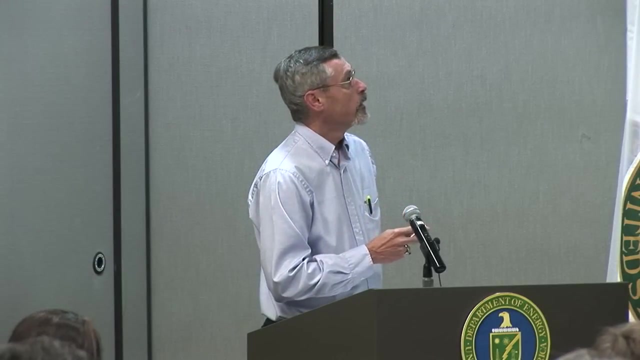 Now it comes down to the questions of what's the concentration. This is what I've got to go after In the. These are the grams released per metric ton into each of the streams. Half a gram of water from the fuel, The processing stream. 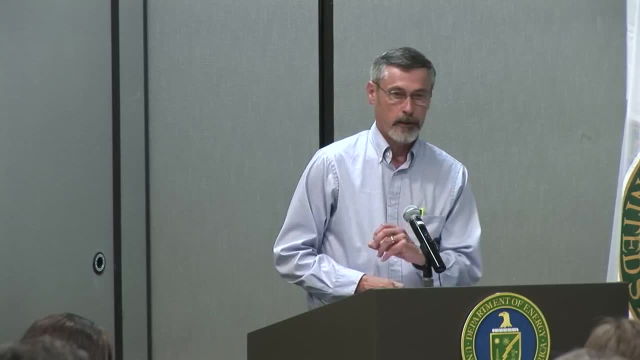 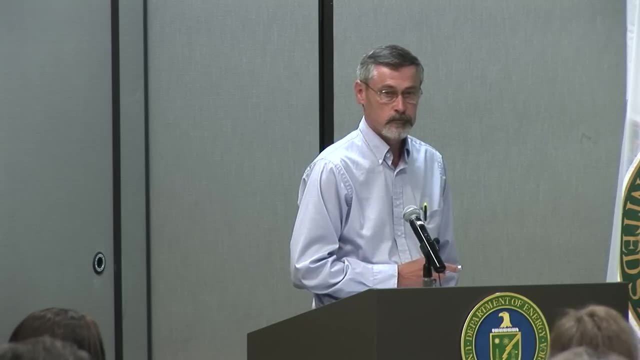 and I'm assuming in this case I've got a DF or a dew point. How wet, how dry is that gas? Minus 60 degrees C, That's really dry. Las Vegas this time of year doesn't have air that dry. 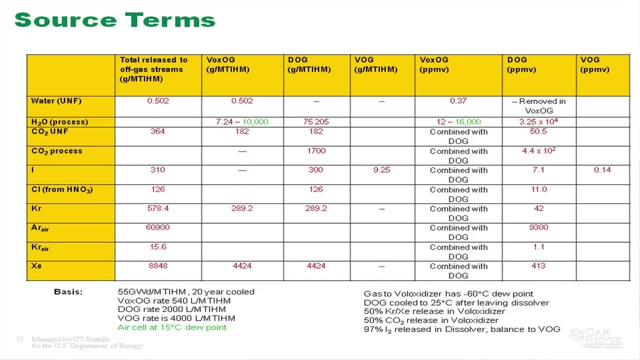 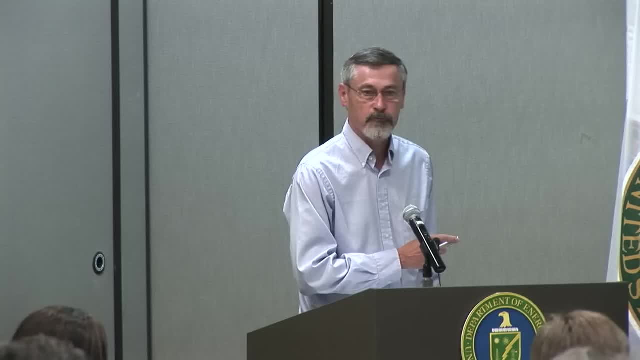 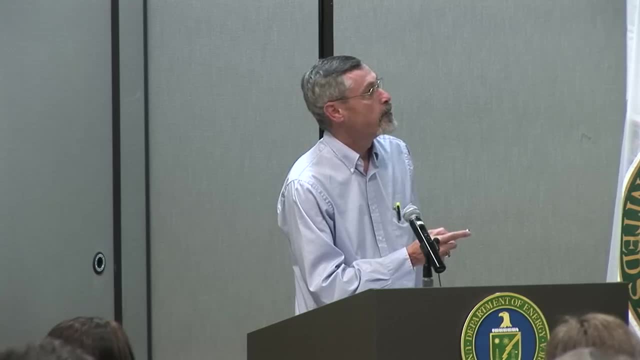 If the cell is at about a dew point of 15 degrees C, that's 10,000 grams of water blended with my half gram I'm going after. It just gives you an idea of the concentrations we're dealing with. I'm talking fractional parts per million. 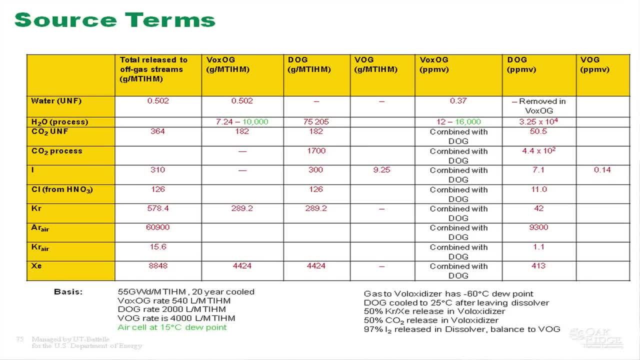 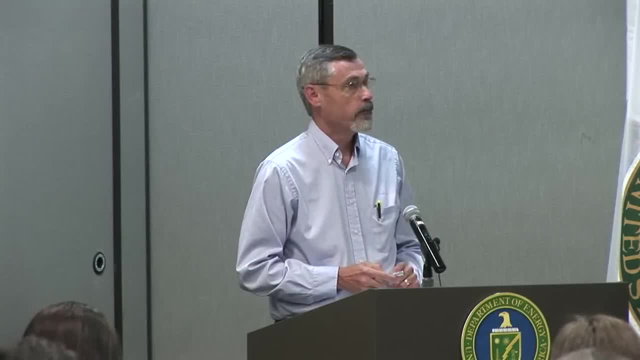 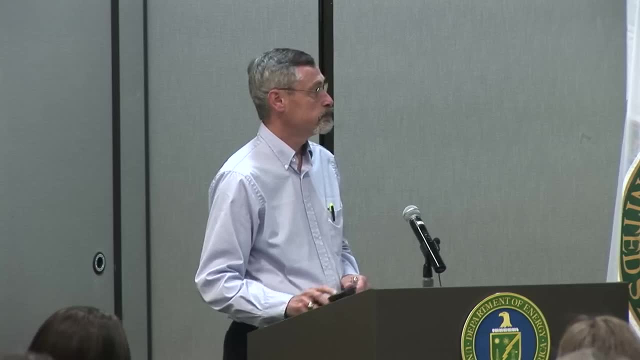 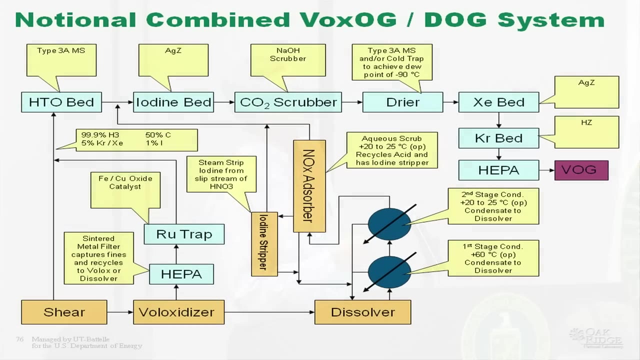 in those off-gas streams and I've got to recover. I've got to recover 99% of that fractional part per million. That's the challenge in the emission control systems. Okay, Click. So what do these look like? What we have this is the dissolver off-gas system. 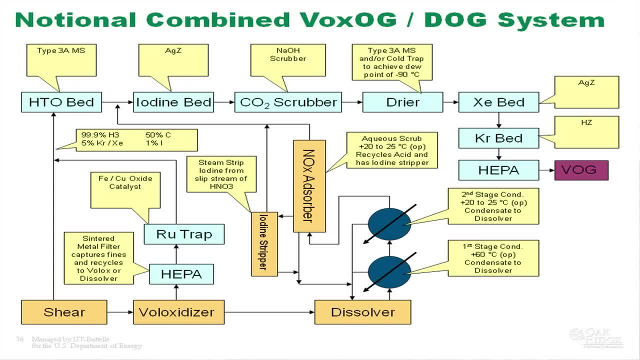 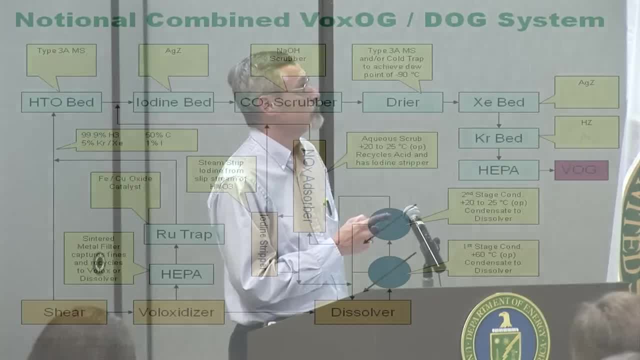 You're going to condense some of the water vapor. You want to limit the amount of water vapor you send up to this off-gas capture system. We have a bed to capture tritium, probably a molecular sieve. It dries. 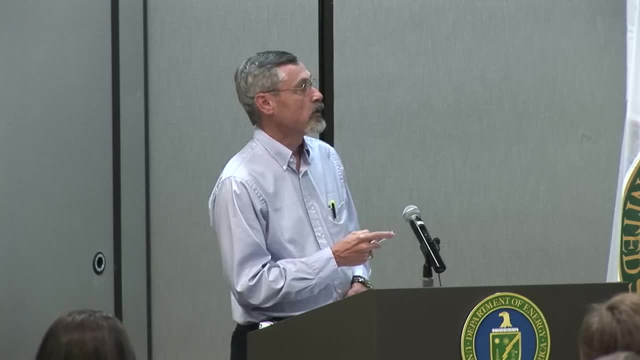 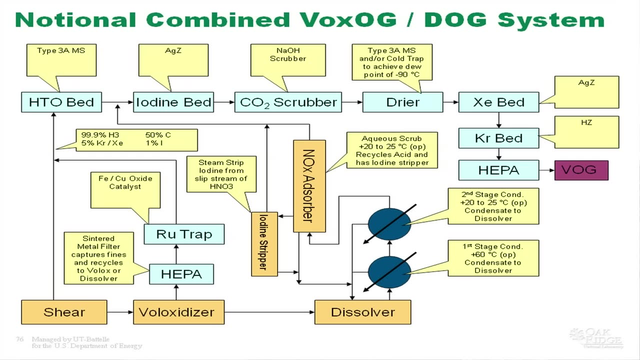 We have silver mordantite for iodine capture, We have a scrubber for CO2 capture, We have a bed, or we use a cryogenic system for krypton and xenon capture. Pretty simple-looking system And each of these processes. 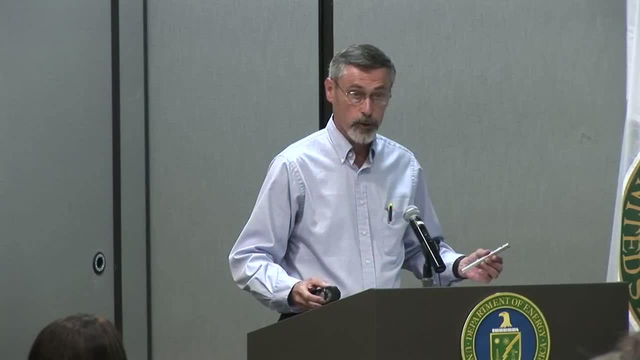 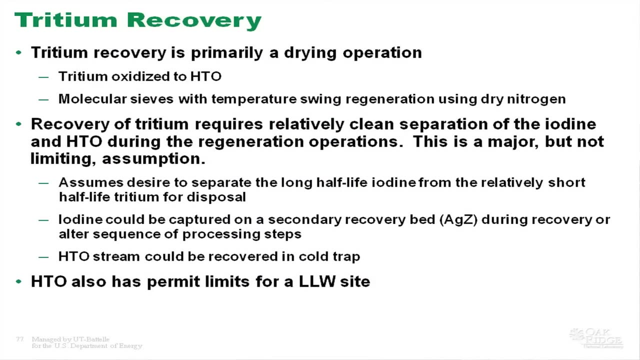 has been demonstrated and we can get DFs of the order we're looking for For tritium. as I mentioned, it's a dryer. The issues here is if we're going to dispose of a very short half-life material like tritium. or a half-life of 10-plus years. we don't want it to capture iodine, which has a half-life of 16 million years. That makes it a different type of waste form. So you want to do a fine job of separating. 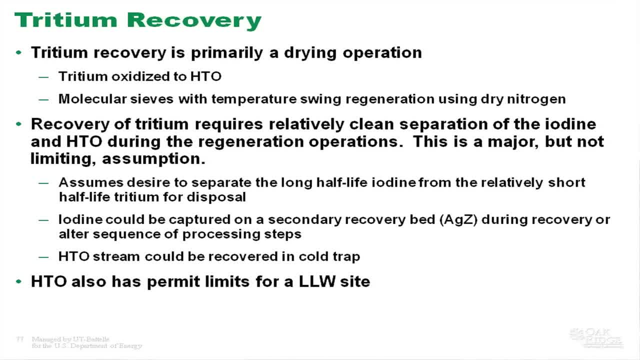 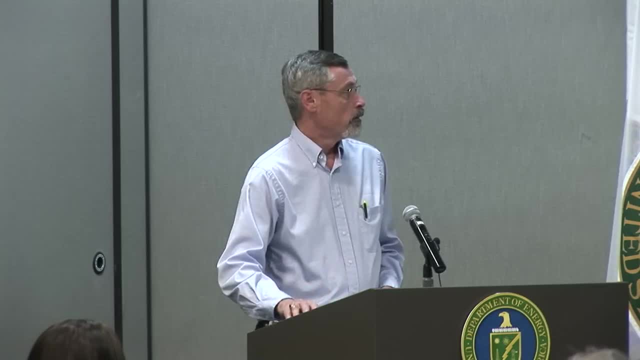 We need high selectivity And we may have to recover the iodine and the tritium together and then perform a separation to have a stream. we can dispose of the tritiated water one way and the iodine a different way. Okay, next. 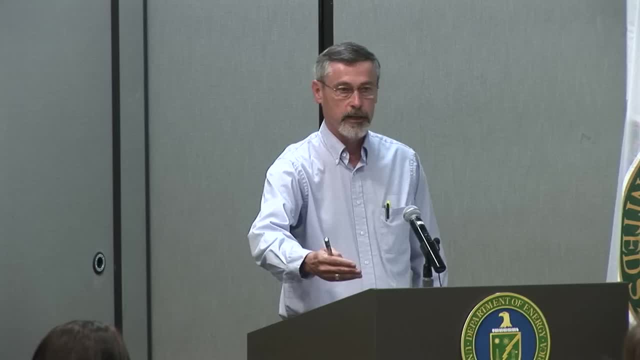 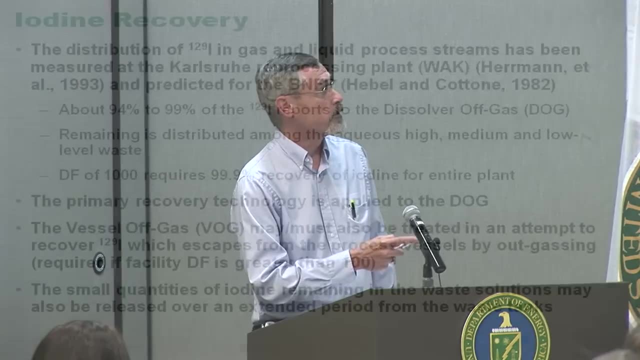 is not evolved from the dissolver, That makes it into the rest of the plant. That's not where we want it. We'd like to capture it in the head-end process. So doing whatever we can in the dissolver to drive off the iodine is very important. We have to recover 99% or 99.9% of all the iodine fed to the plant. That's a big number, especially if we only get 94% coming off the dissolver off-gas, and now we have these very dilute streams. 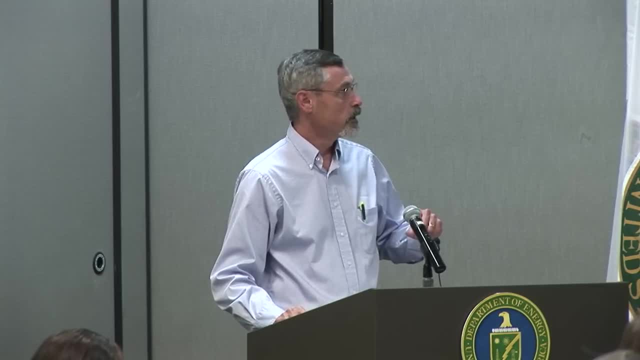 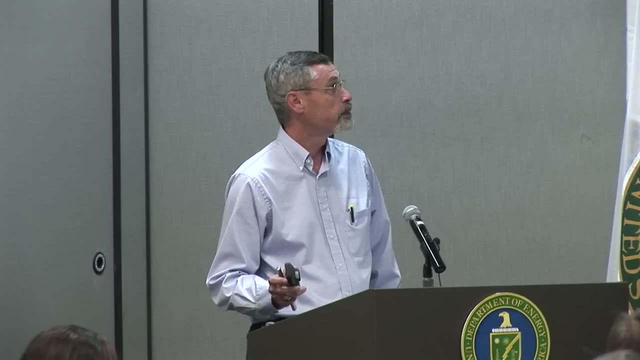 later on to capture. So that's where the vessel off-gas line comes in and small quantities in the rest of the waste. solutions are going to be released over extended periods of time. Carbon-14 recovery- Carbon-14 is the one radionuclide. 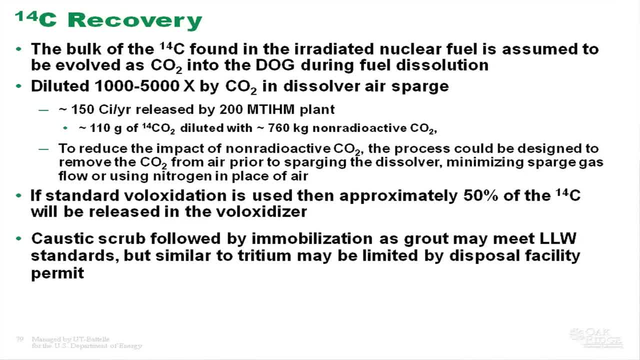 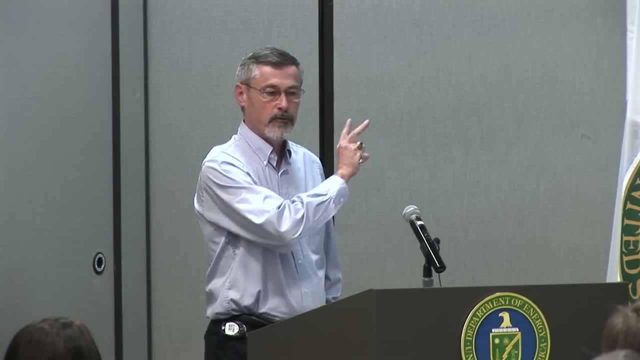 that we may not have to capture at all. It tends to be below the limits, as we've done most of our analysis. So carbon-14, it's up here. I don't know if we're going to have to actually capture it. It depends on the size of the plant and any changing regulations, But it's fairly simple. Caustic scrubbing is a well-developed industrial process. Again, you want to sequence these processes so you don't capture things you don't want to in each of them. 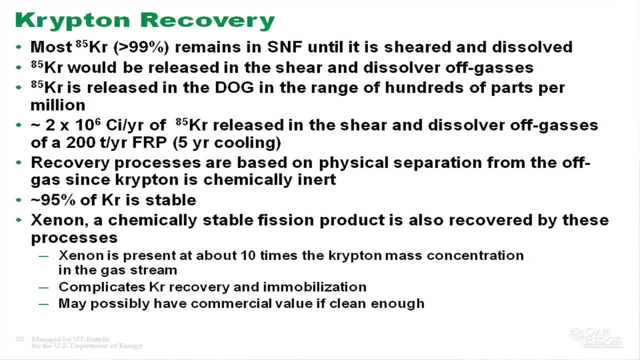 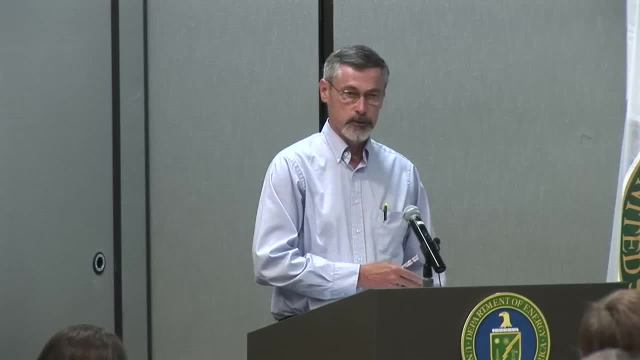 Krypton is a potential problem. It's a noble gas, so you have a limited number of ways to go after it. You can cryogenically recover it, You can do some selective adsorption, but it tends to be more of a cryogenic process. 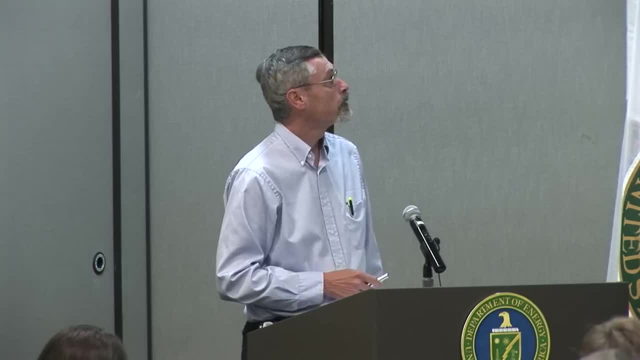 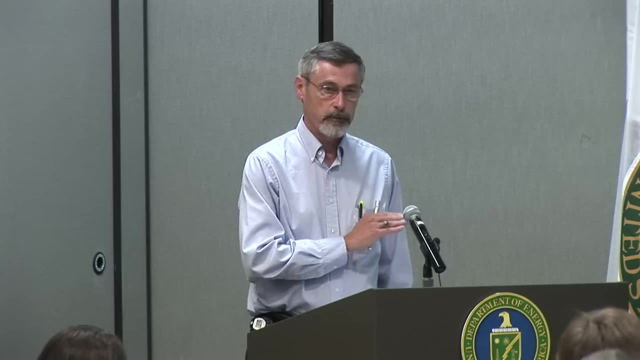 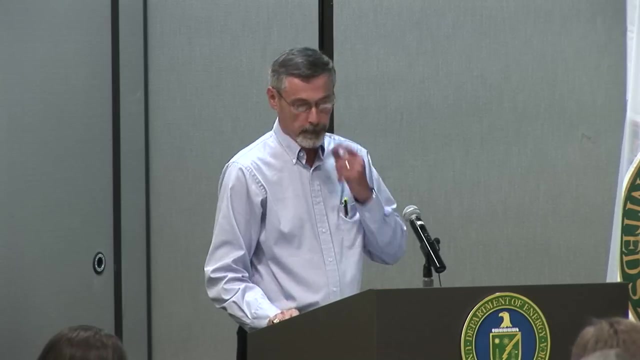 You slow it down on these beds and then you have to regenerate them. It is the one that produces the highest heat turn and it decays to rubidium, which is a very corrosive liquid if you put it into storage. Well, remember the block diagram. 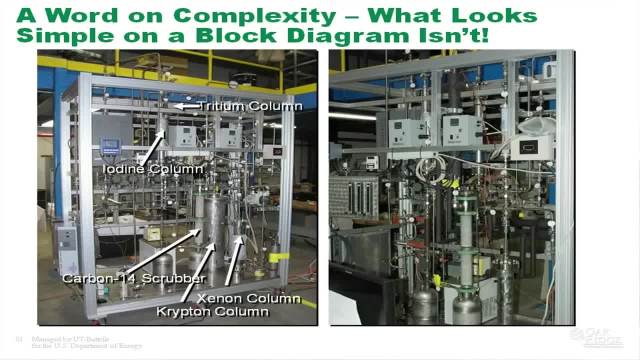 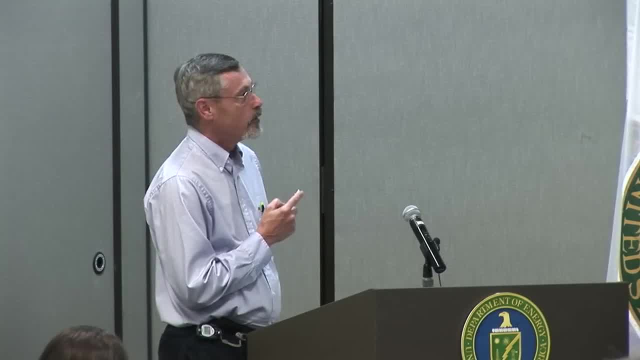 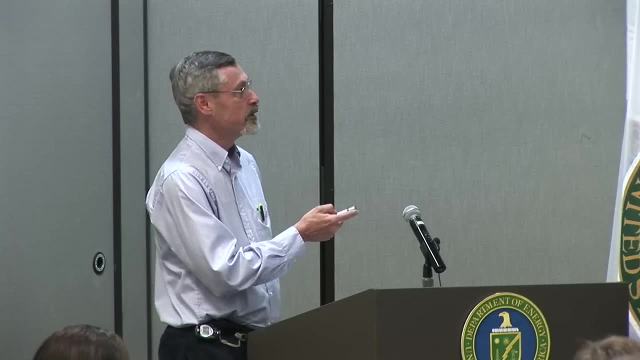 where I said, it's a pretty simple process. So what looks simple on a block diagram, when you turn it into hardware isn't always that simple. So this is a small experimental rig where we integrated each of those steps and there's the tritium column. 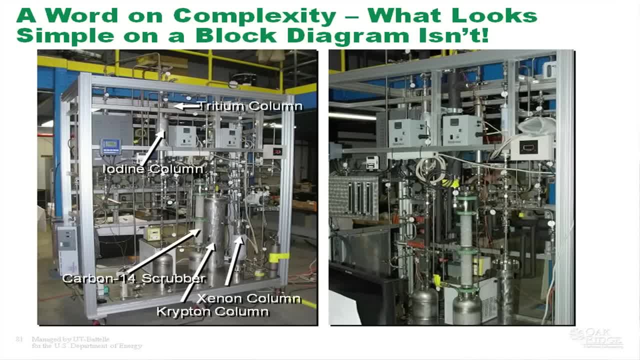 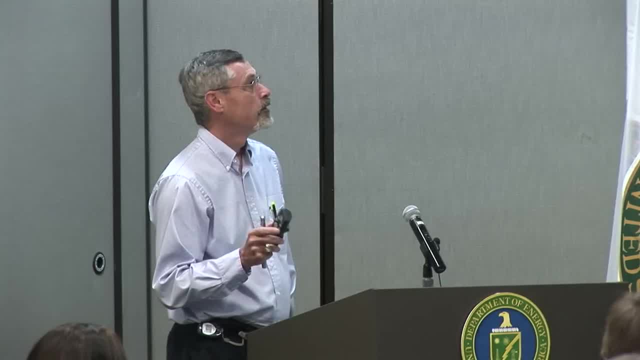 It's buried behind all the piping and the instrumentation: the iodine column, the caustic scrubber and our xenon and krypton traps. And I've already touched on many of these things. I'll point out one item here. 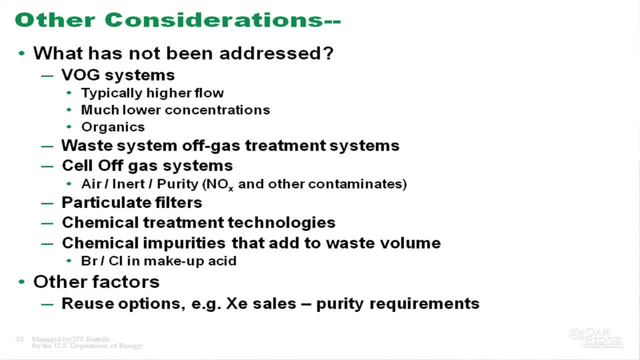 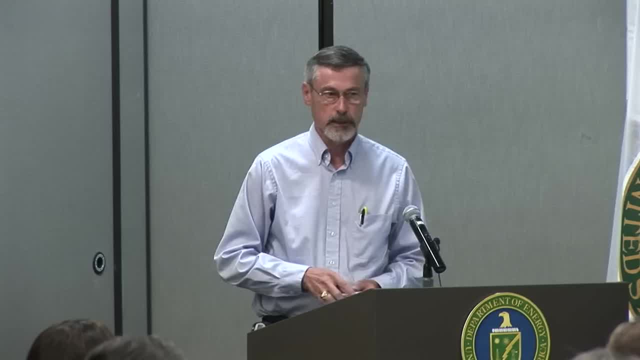 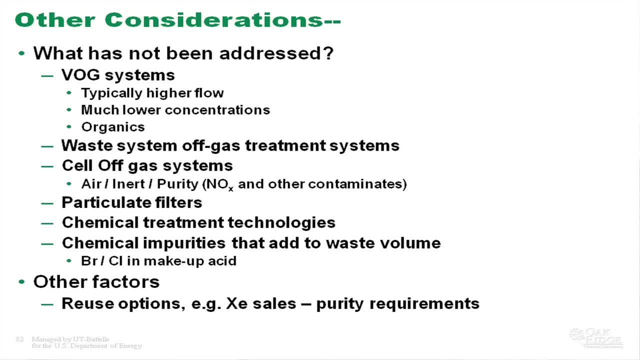 the chemical impurities. Remember I talked about we had to bring in potentially a million gallons of nitric acid. Well, a million gallons of nitric acid also brings in significant quantities of chlorine and bromine as impurities, potentially on the same order of magnitude. 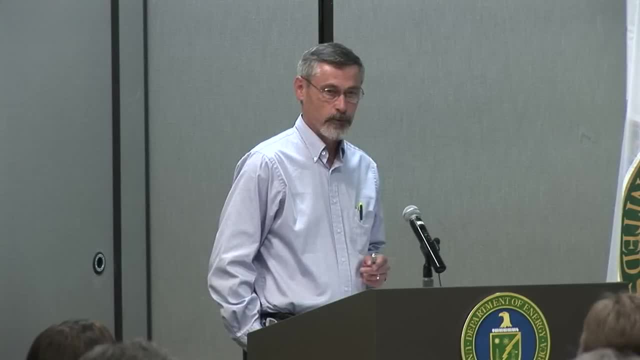 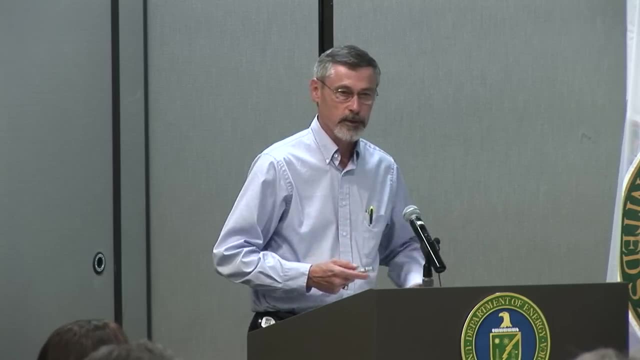 as the iodine in that same amount of fuel. They're halogens. They come off, They are evolved. They have to be trapped right along with it. That'll consume your capacity of your iodine bed. Some other factors you might consider. cancels. How can we sell the xenon? That's one of the largest of the fission products mass-wise, There's eight kilograms of krypton per metric ton. It's worth- last time I checked- about $5,000 per cubic meter. 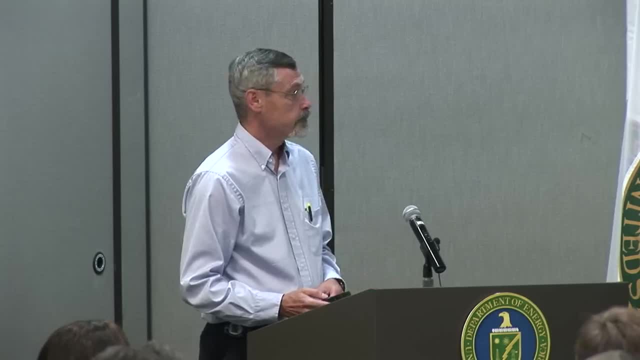 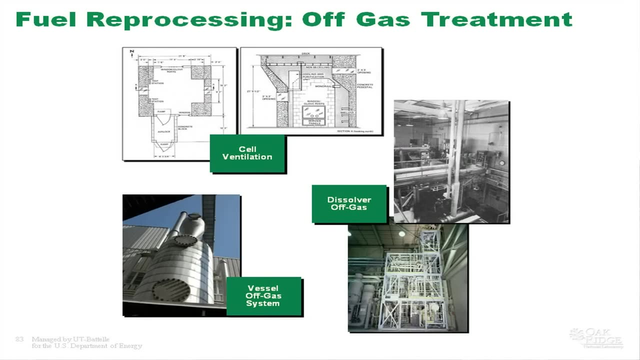 If it's pure enough, maybe there is a market for that. So some more pictures. Cell ventilation: How tight is your cell? What leaks into that? How much carbon dioxide comes in there? Dissolver off-gas systems, primarily looking at capturing the NO2.. 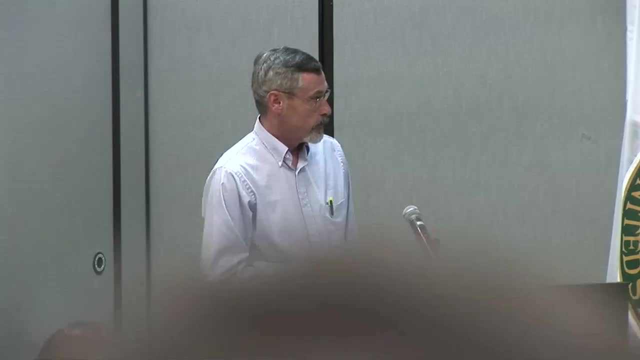 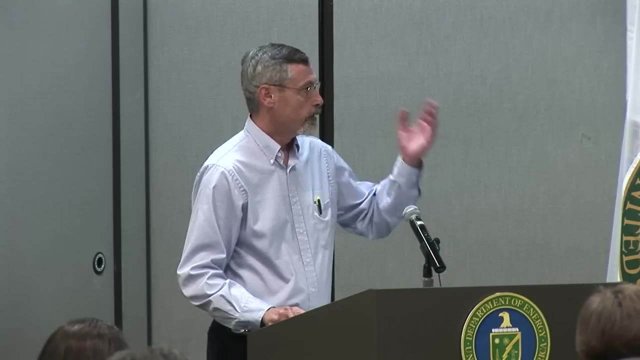 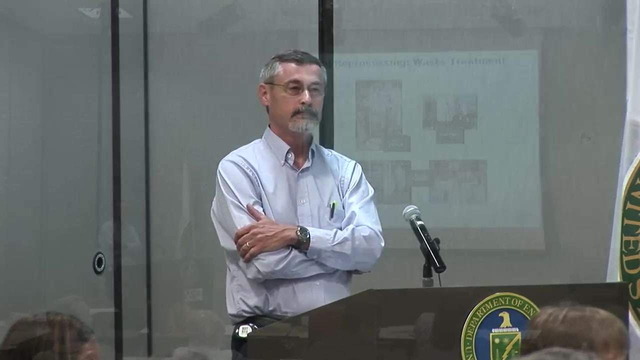 We didn't talk much about that. Other systems for treating the off-gas And the vessel off-gas is a fairly large stream. So other systems we'll just touch on in a few words. Yeah, You might want to point out. 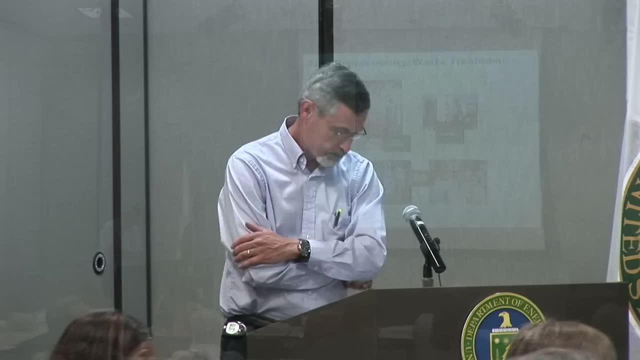 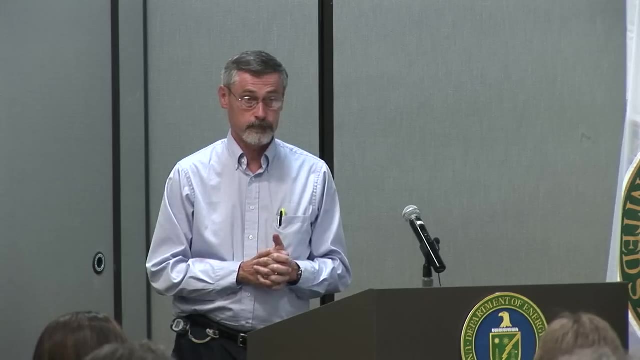 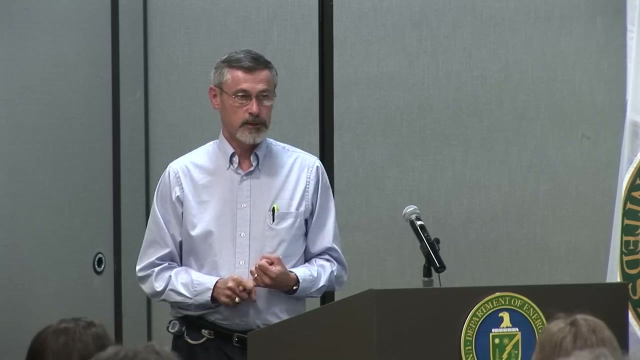 what's done in an operating plant. Okay, That's a good point. There is no operating plant that goes. after all, four of those Iodine is captured in some cases. Some cases it needs to be released to the sea. La Hague did that. Thorpe will have to capture carbon-14 if they extend their operation. They do capture iodine. Ricoccio captures iodine, Idaho did iodine and for economic reasons captured some krypton, but not for emission control but primarily to sell the krypton. 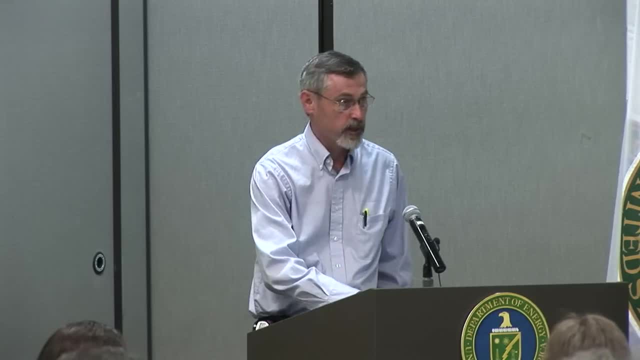 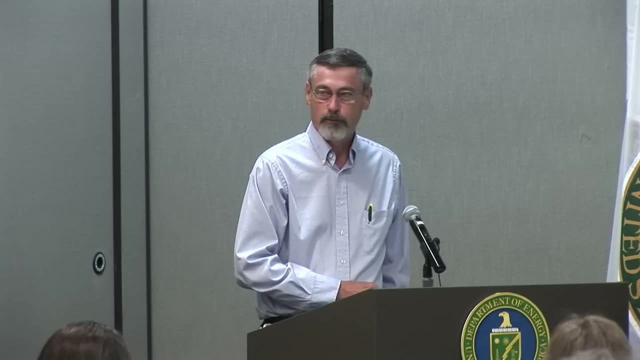 One of the things: if you ever went out to the Idaho chem plant during the heydays there, you could tell if they were operating. There was a brown plume that stretched You could see for miles. if the plant was operating. That was the NO2.. So Tritium, Tritium, zero into the sea. So we don't. I don't think any of our plants are going to be built on the sea, So I think we don't have that as a disposal pathway. and I don't think it would be environmentally acceptable for us. So I do think that any plant built in the US we're going to have to consider at least three of those four and maybe all four of them. Is there a way to do them all in one system? 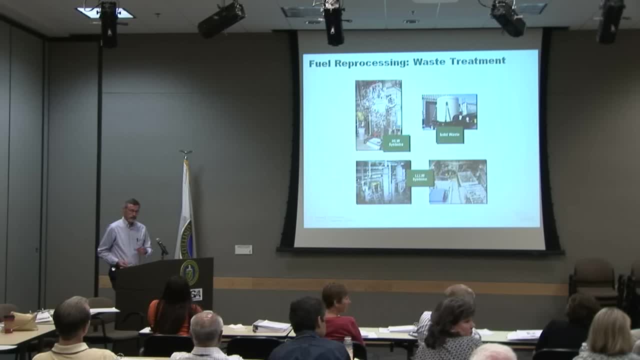 Can they all wind up in one stream rather than what you're doing? I look at that off-gas system that you have designed up there and building it on a production scale. you'll never operate. It'll be down forever because of the complexity of the system itself. 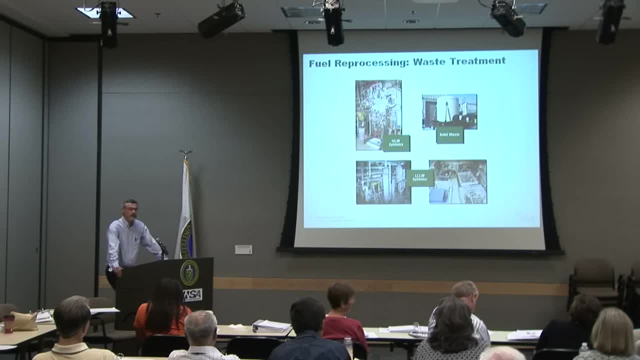 I mean we're facing the situation where we're facing the same things right now, just with simple iodine removal at Hanford, and it complicates the off-gas system to the point that it makes it almost impossible to operate, And you're looking at four very complex systems there. 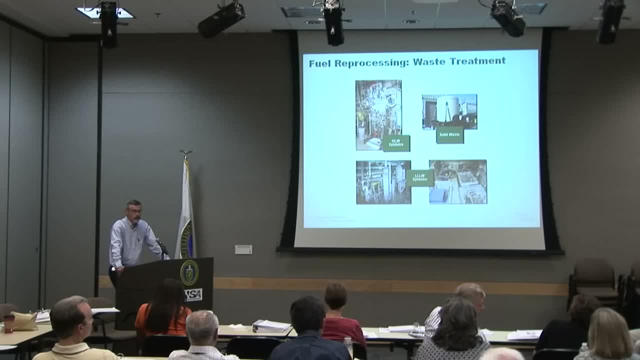 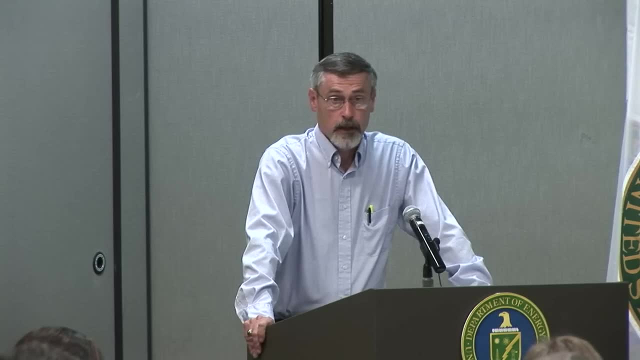 trying to operate them all continuously at the same time and balance that ventilation system. That's a That's a tough job. It's a real tough job, And I think what you're going to do is you're going to try and do as much as you can. 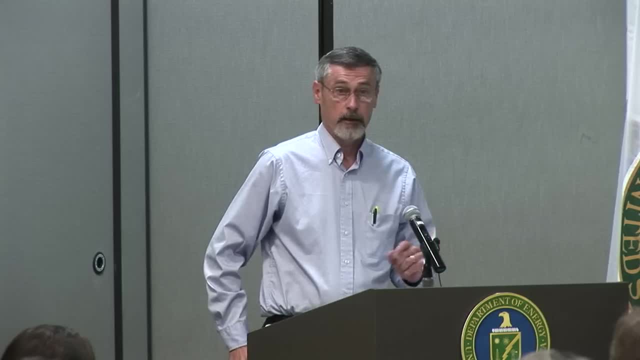 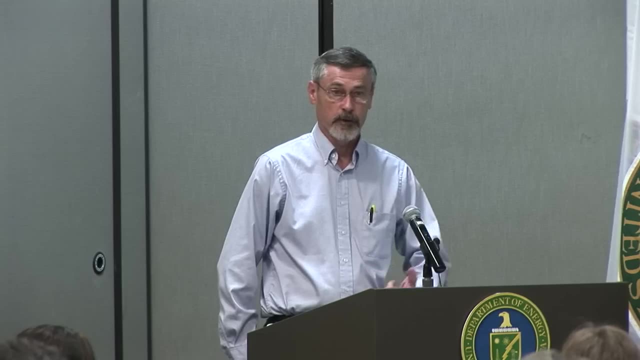 in as small of a stream as you possibly can. That's where voloxidation and some of the advanced voloxidation may come in. if we can drive off all the iodine, if we can drive off all the xenon and krypton, 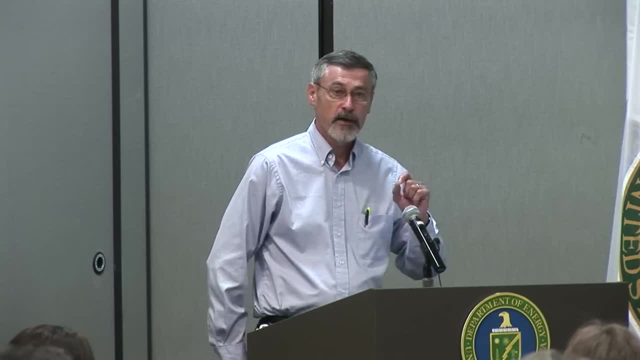 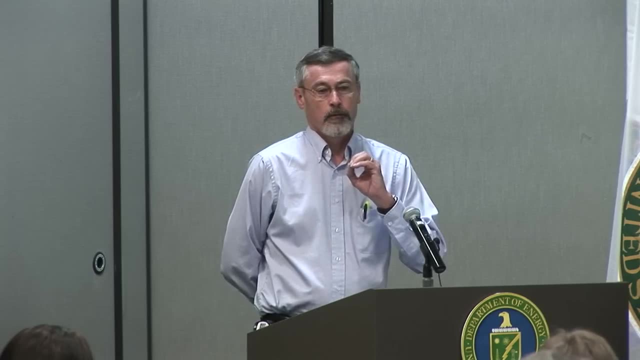 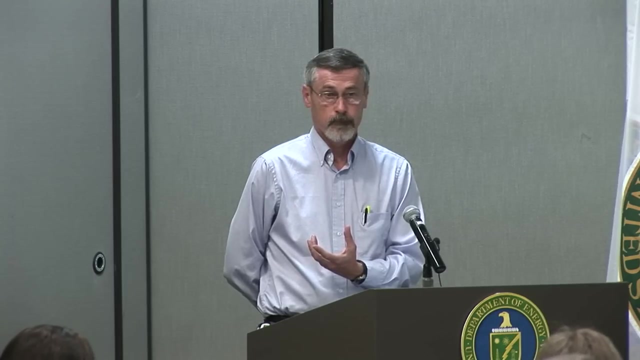 all the tritium. We may just have one small stream to deal with, but I'm not sure if the answer to your question is there a single process that will capture all of the All of the species, Or can you make them go into one stream? 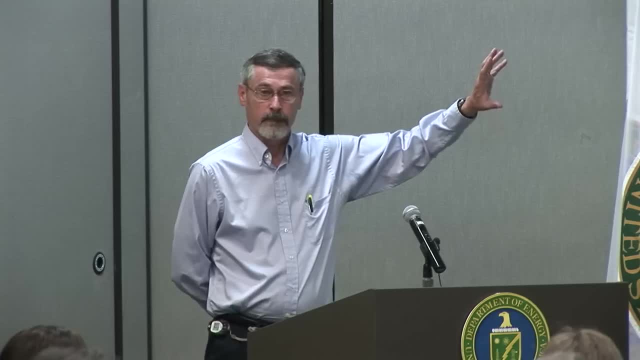 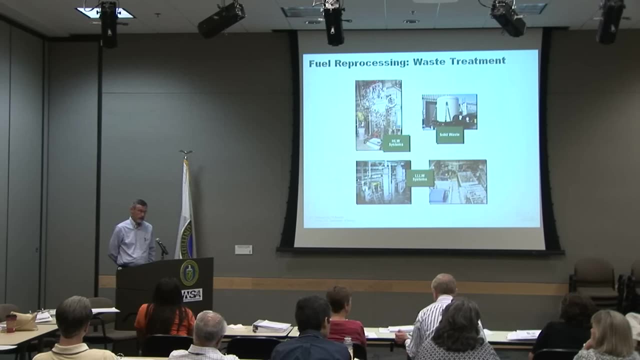 That's what I'm trying to do is get them into one stream, That desol, That voloxidation off-gas stream. if we could do that. But even if you do voloxidation in your current flow sheet, you're going to have three different separations techniques. 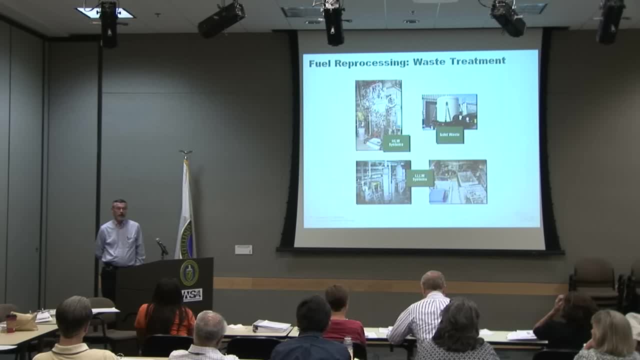 to get the items that you're looking for? Yes, And I'm just looking at it going from an ops perspective- that stuff. The other thing is: how are you going to dispose of all of it? I mean, you're going to have four different products. 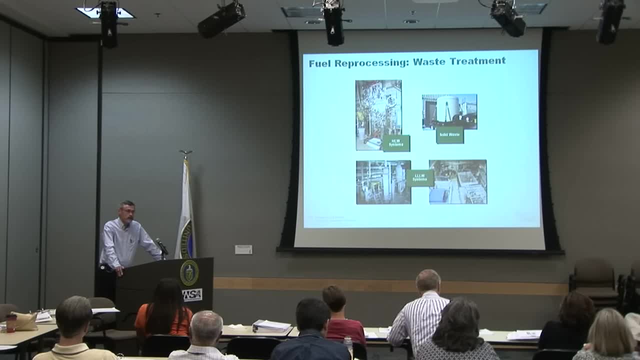 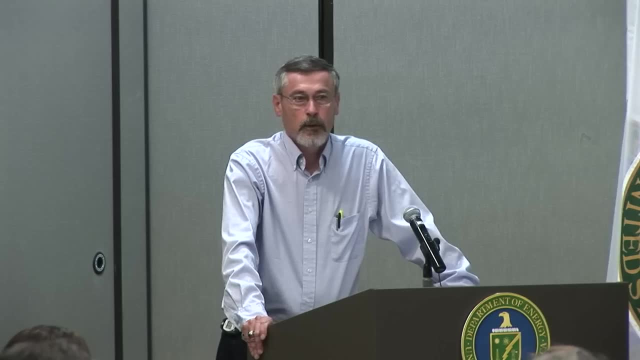 Yes, that are going to have to be disposed of. Are they going to? Do you assume it's going to get made into glass? Do you assume it's going to get? Where is it going to go? The Each of those, I think. 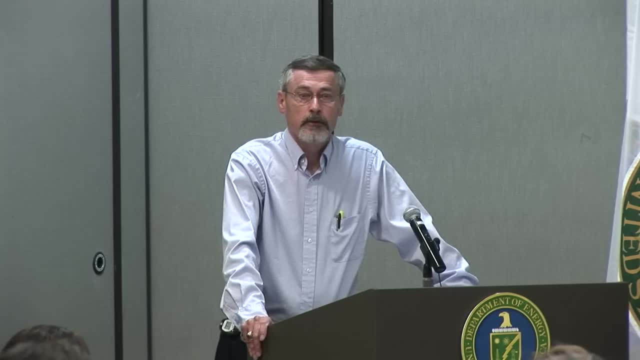 may have a different stream, that we go to The iodine. I believe We're looking at a potential glass waste form for iodine. I think John will get to that in his discussion. Krypton may be stored in gas cylinders for decay. 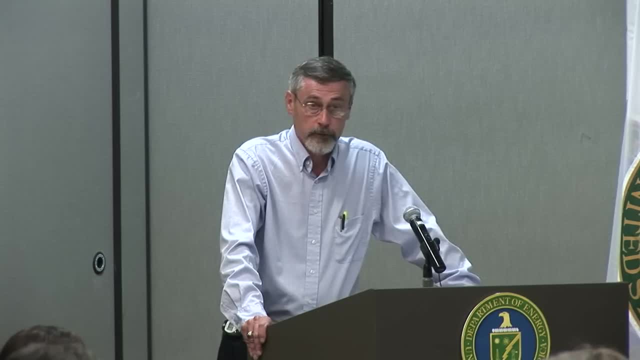 It. Storing it any other way becomes rather difficult. although we are looking at some silicon carbide sputter deposits for krypton, The tritium- you may put that into a grout- It's a relatively short half-life. 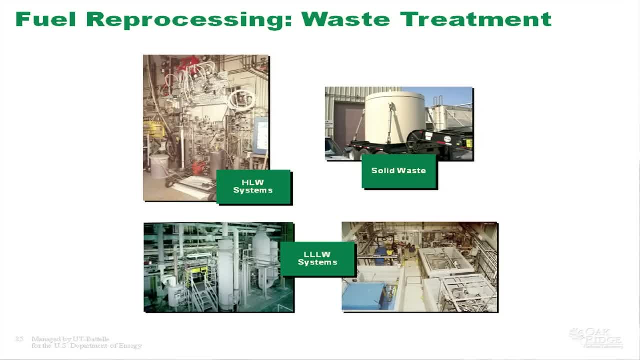 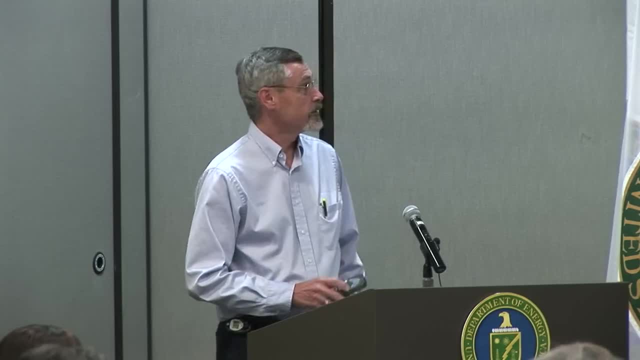 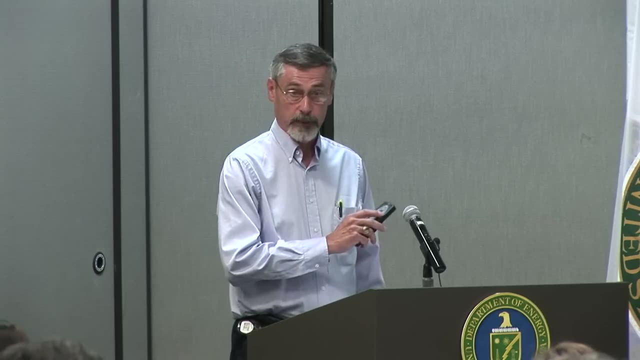 You may be able to manage that for 100 years. I agree. All right, I've got the hurry here. Process control: we didn't touch on but a very important part. the process control is a very important part of operating a plant. 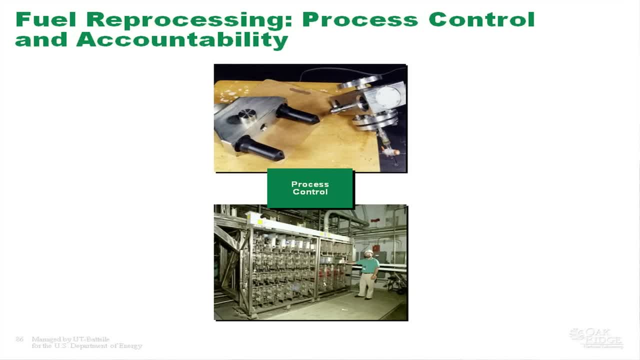 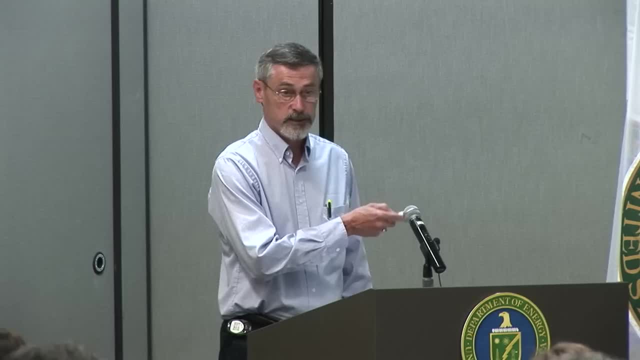 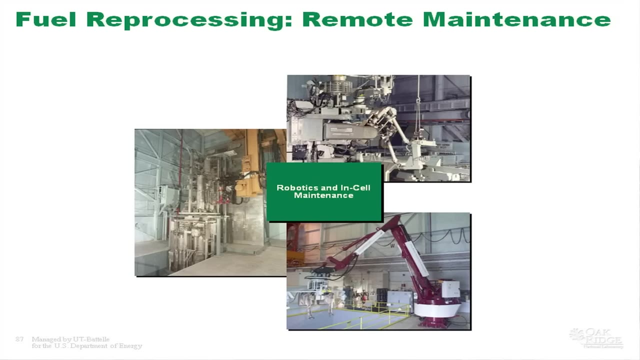 Every one of these pieces of equipment will have multiple instruments on them to monitor their conditions. This instrument control system here was just for one bank of centrifugal contact. What's one cycle of solvent extraction Robotics? We have to maintain all of this equipment in a hot cell. 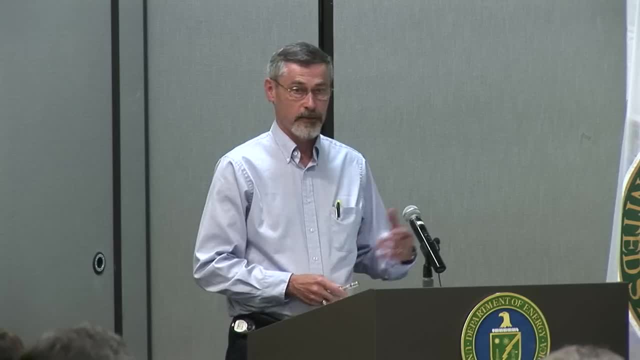 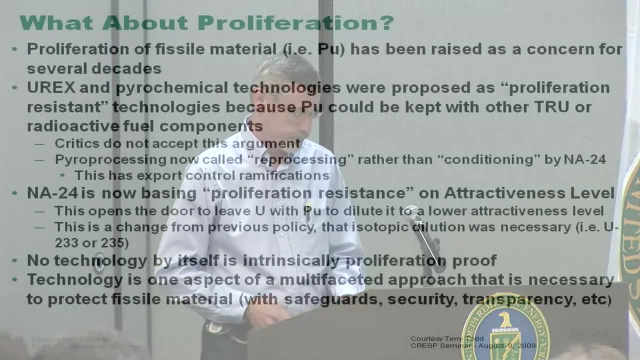 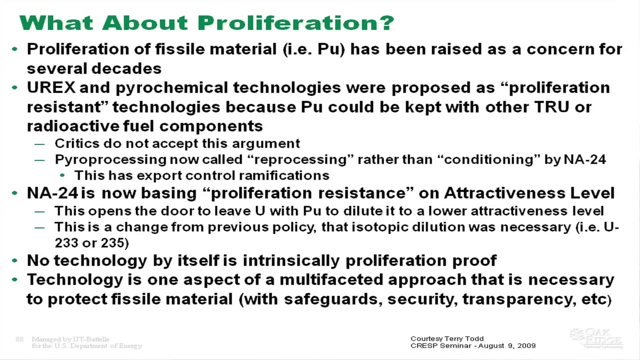 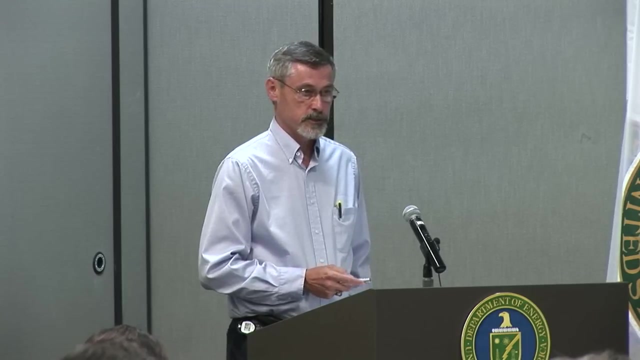 You can't forget about the operability of the system. Maintenance, I think, is very relevant to this. What about proliferation? I'm not going to talk much about this at all. Whenever you separate plutonium, you raise a proliferation concern. 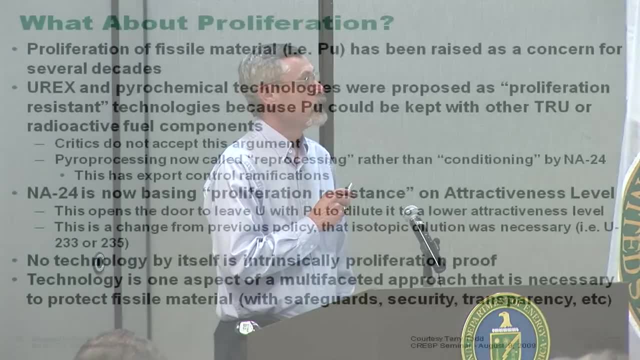 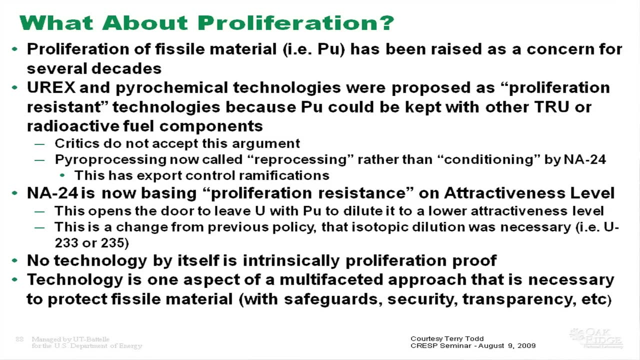 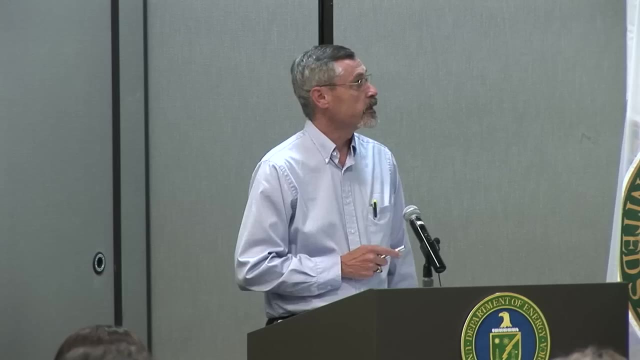 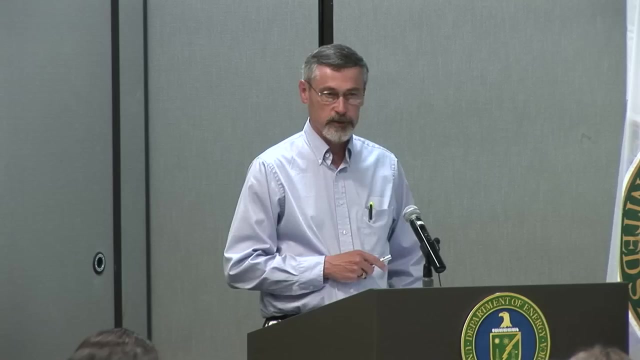 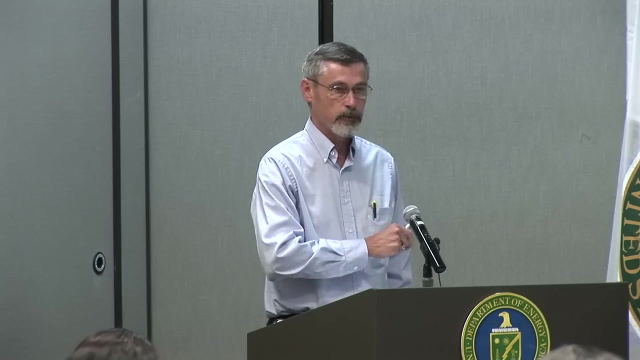 And the Eurex processes and the pyro processes have been proposed as proliferation-resistant because we're keeping the plutonium with other transuranics and radioactive constituents, And critics don't necessarily agree with this argument because you can still perform chemical cell separations to separate the plutonium from whatever you've put it in. 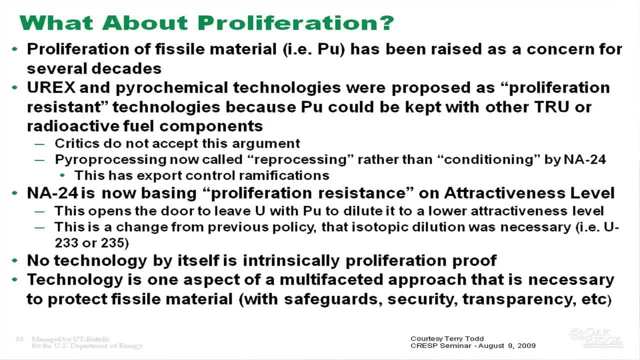 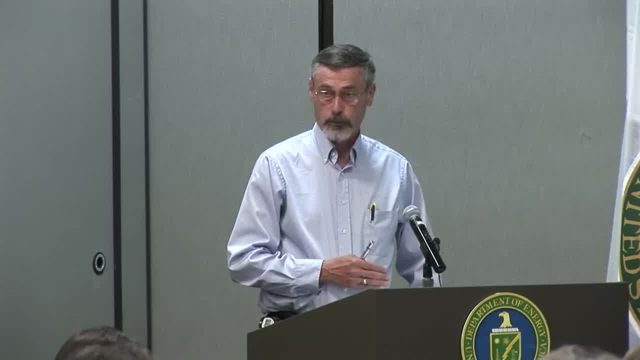 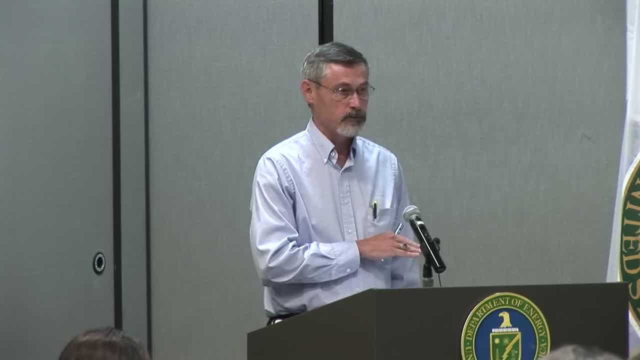 And the idea of keeping it with highly radioactive materials. I think before 9-11 we might have believed that that no one would put themselves at risk to recover these materials. I'm not sure that we can say that no one would put themselves at risk. 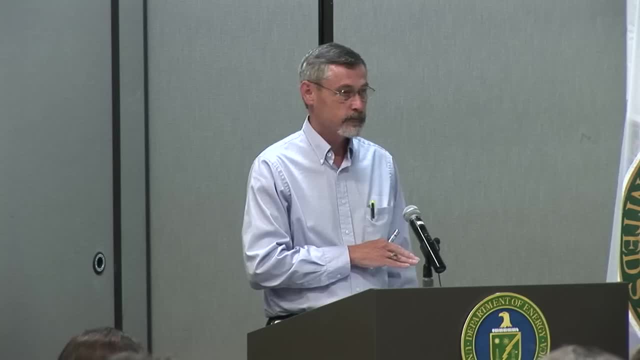 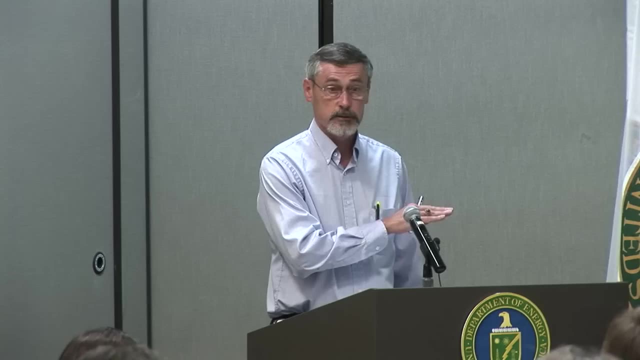 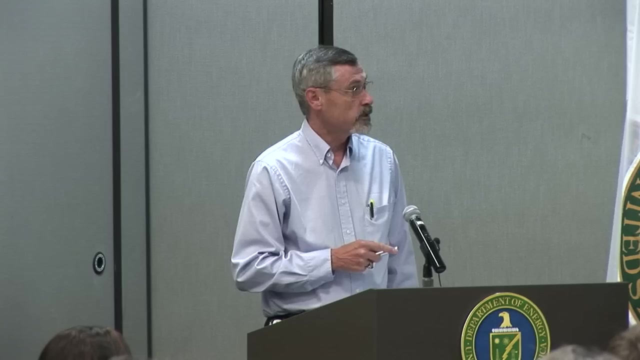 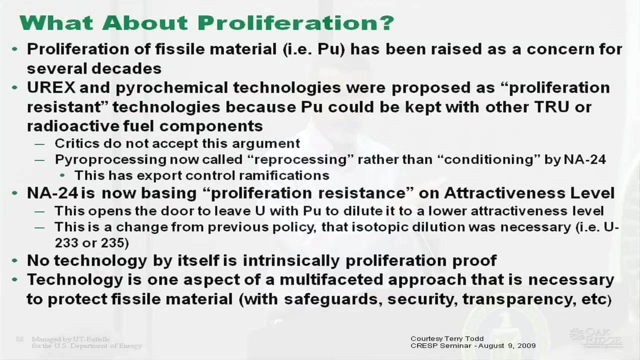 to touch some highly radioactive material, And the longer that we keep fuel in storage, the less self-protecting it becomes. NA24 is now basing proliferation resistance on attractiveness level, So that may change things a little bit, But I'm certainly not the expert in proliferation resistance here. 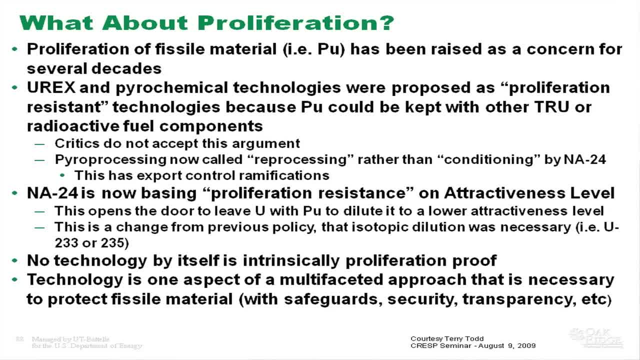 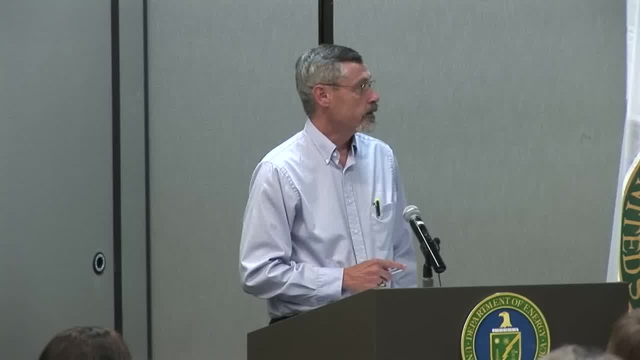 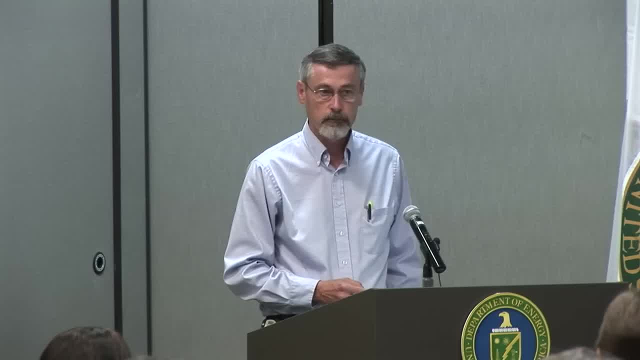 But no technology by itself is proliferation proof. I think we just want to face that fact That one is going to have to rely on many aspects to protect fissile material, Whether it's in a fuel assembly or whether it's reprocessed. The fact is there's plutonium in spent or used fuel. 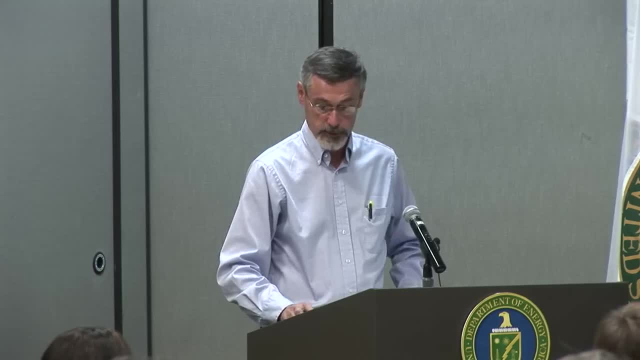 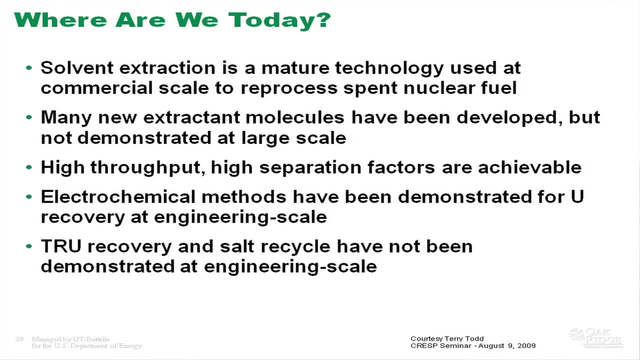 So we've got a couple with safeguards, security, transparency. So where are we today? Solvent extraction, which is the workhorse of separations, is a mature technology. It's used on commercial scale In a number of countries. there are many new extractants that have been developed. 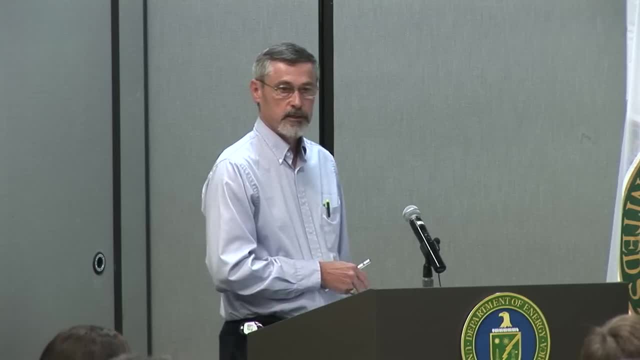 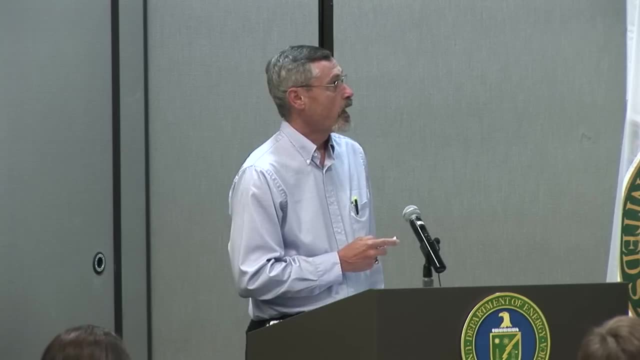 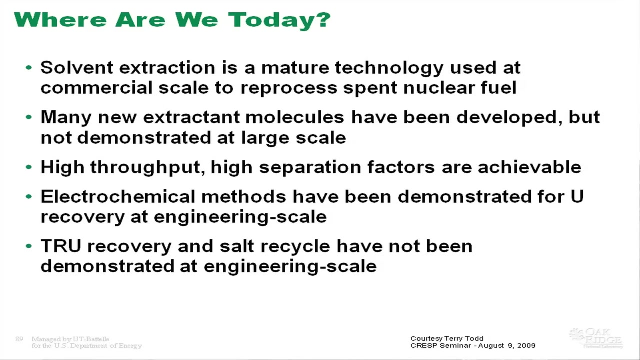 But they have not been demonstrated at large scale. These are the Truex processes, the FPEX processes. The high throughput and high separations factors are achievable. They're done commercially, And Mike Golf will talk about the electrochemical methods that they've been demonstrated for. 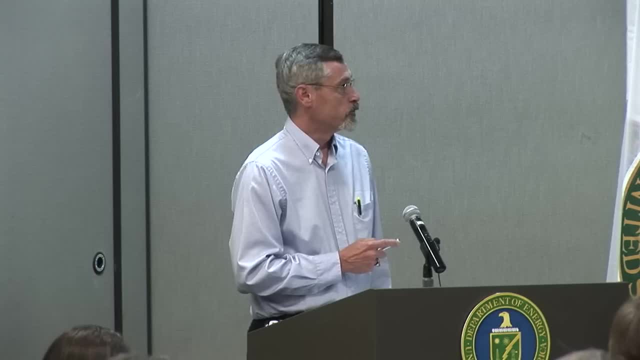 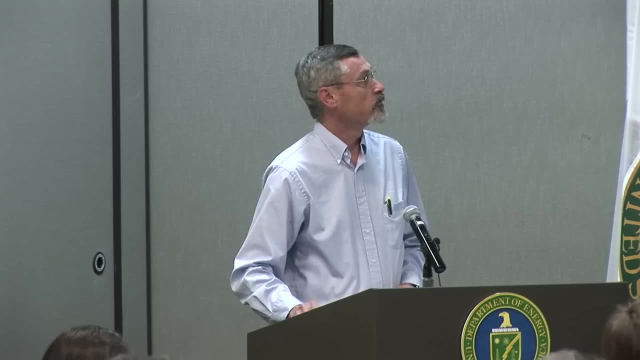 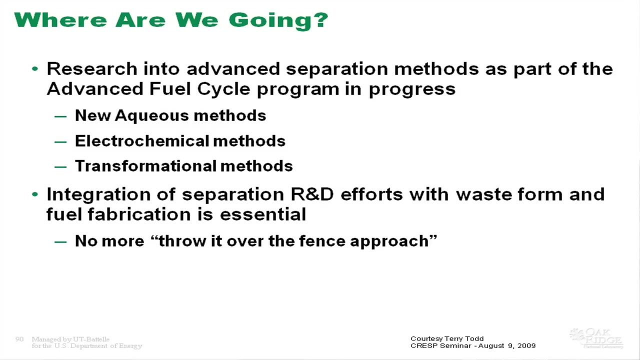 The uranium recovery at an engineering scale at Idaho. The true recovery in salt recycle have not been demonstrated at the engineering scale, But this is another talk for it a little later. Where are we going? We continue to look at advanced or new recycle methods, electrochemical methods, within the AFCI program. 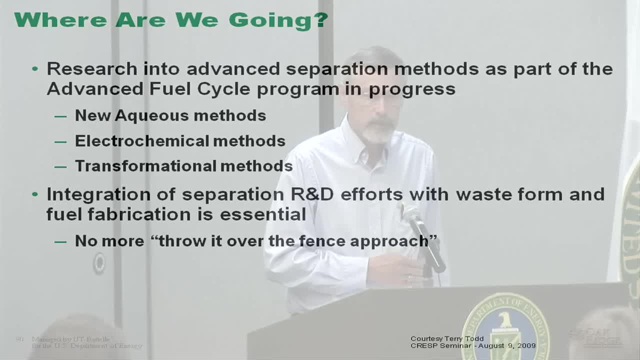 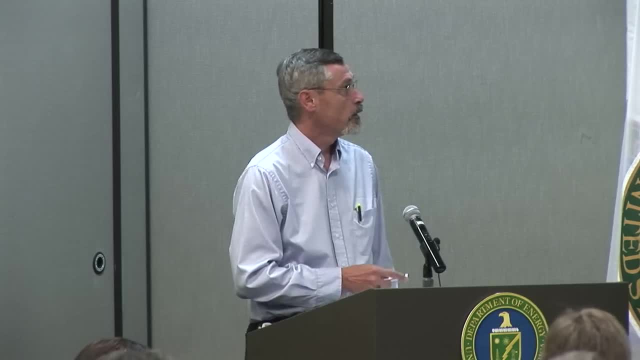 And transformational methods. Many of these are things we've looked at in the past, But we're looking at them again with a new, A new view for what they can offer us, And we're integrating the separations efforts with waste forms. 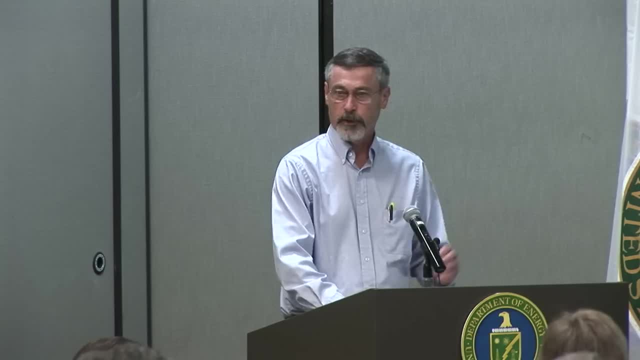 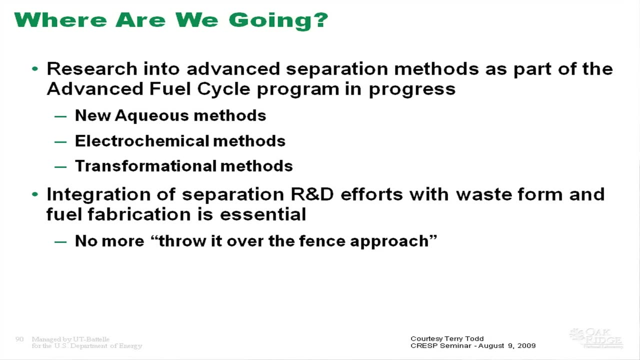 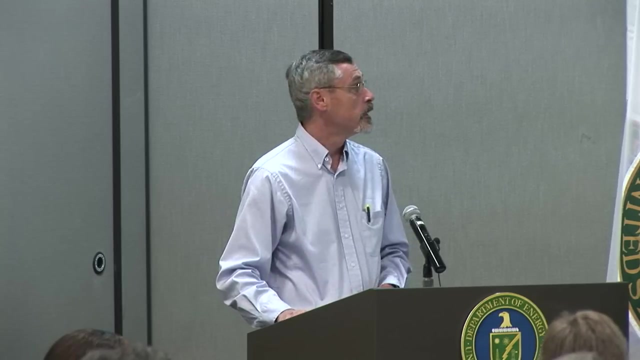 It's no longer necessarily a case of: well, we're done with our separations, Here you go, John. take our waste, do something with it. I think we have to look at how do we couple that waste form with. Can we do things simpler, better in the separations that make the waste form processing a lot easier? And what do we have to do in the way of separations to make it easier? And what do we have to do in the way of separations to make it easier? And what do we have to do in the way of separations to make it easier? 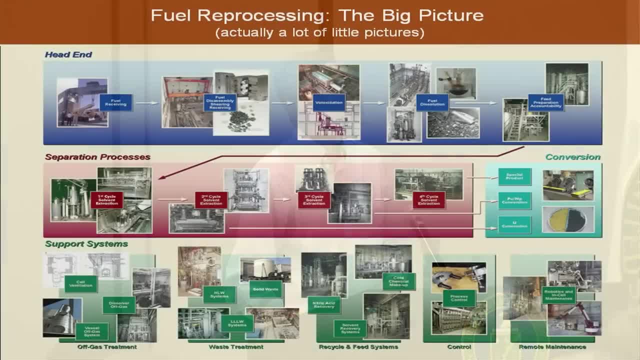 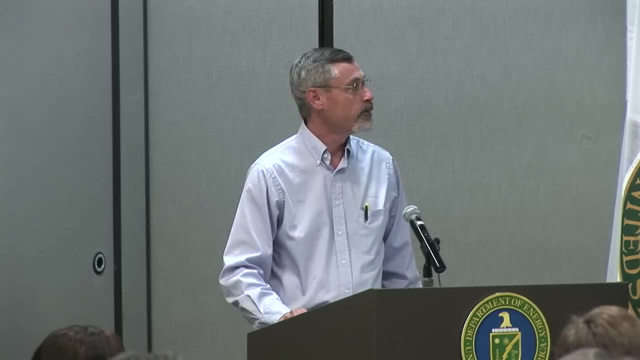 And what do we have to do in the way of separations to make better fuels. So that was fuel reprocessing. This is the big picture, Or should I say it's a lot of little pictures And input for this talk, pictures I got from a number of people throughout the DOE complex. 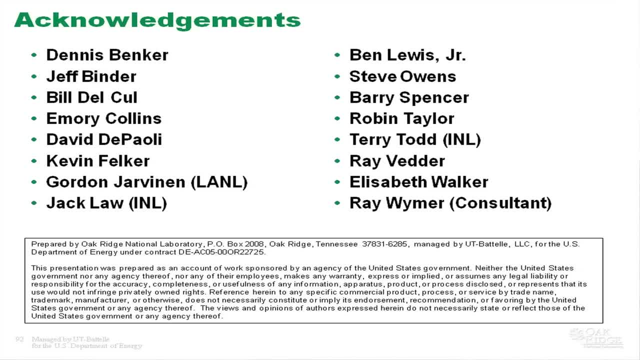 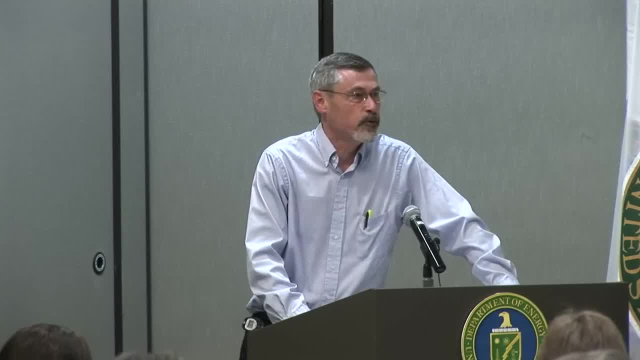 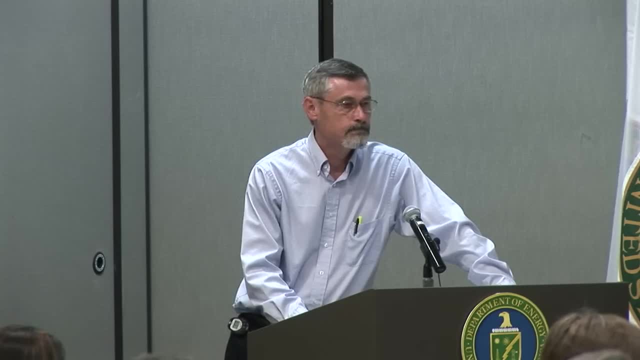 I'd like to thank all of them. A few of them are in the room, been here at various times And with that I'll now pass out the test. Oh, I guess it's time for your questions. Do you think that the future really is going to hit for electric chemical? because this is a kind of a qualified opinion on what it's for. 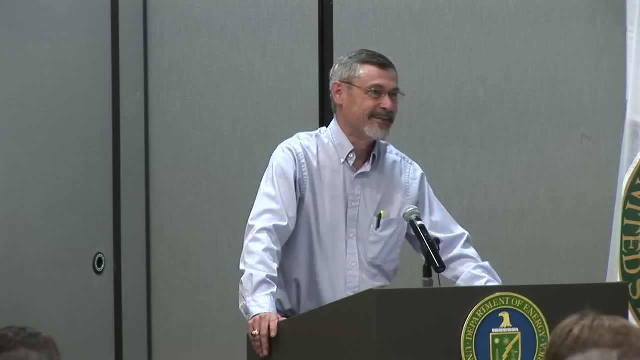 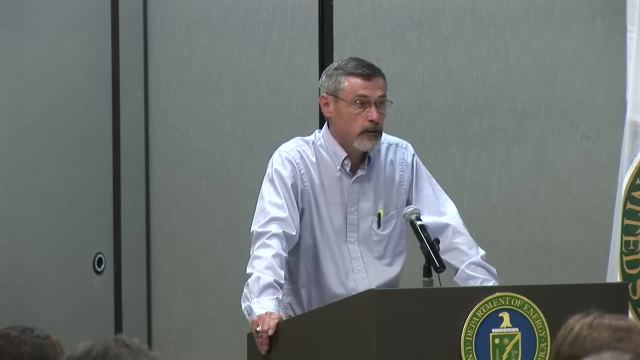 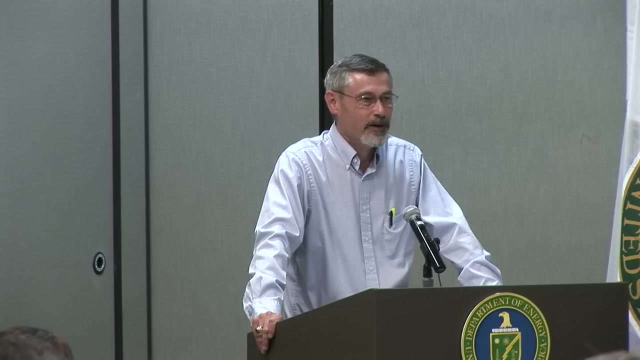 It depends on who you talk to. I'm more of an aqueous guy than an electric chemical guy. I think they both have a role And I think that maybe the future is a combination of the two. So, Mike, do you have any comment on that? 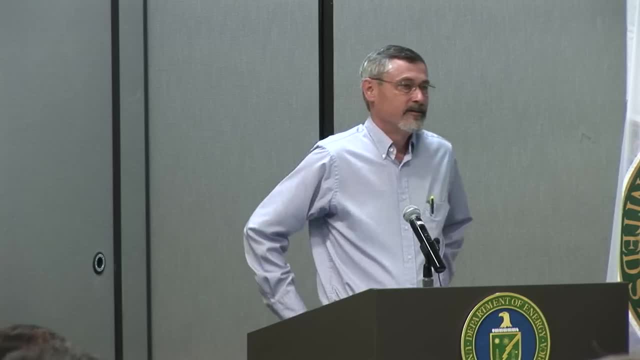 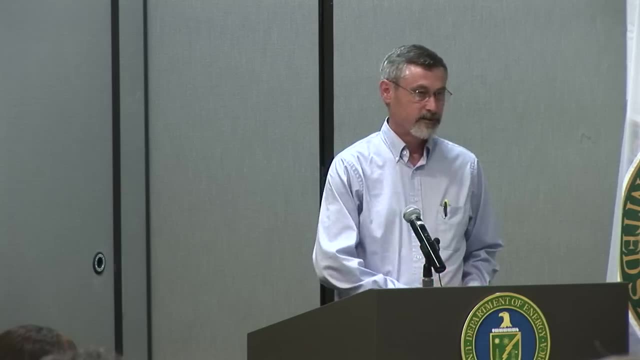 I have a comment, I agree. I mean they can coexist. There's some nice flow sheets that you've learned. Electric chemical is really made for recycling- a fast reactor, And you can combine them, use an aqueous process to recover trains. 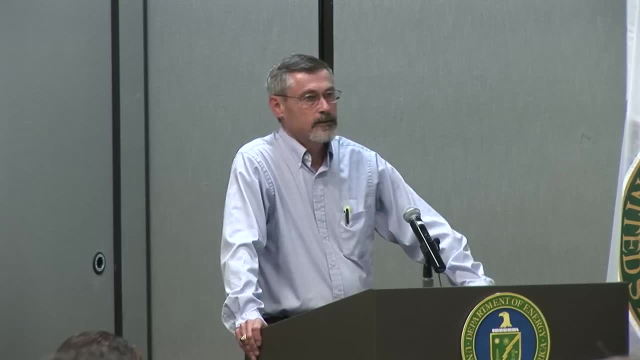 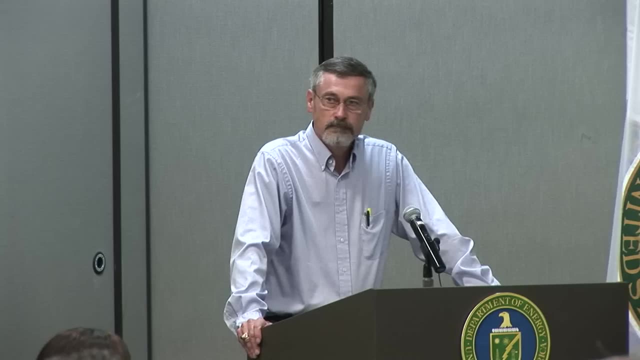 or an action-like water reactor, send them to a pyrochemical process to recycle into a fast reactor. So there are ways to blend them together. It takes advantage of both the technologies. They don't have to be mutually exclusive, Yeah. 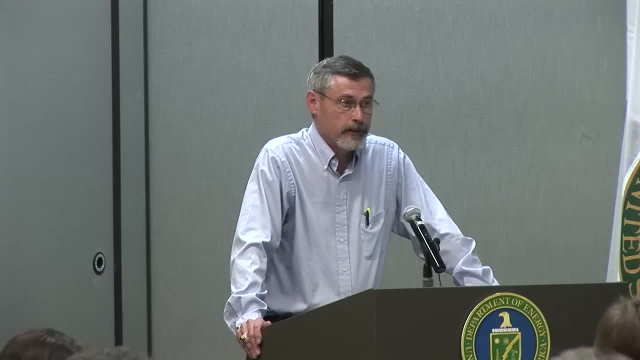 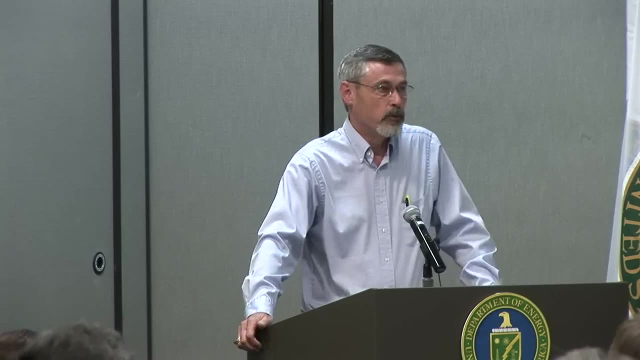 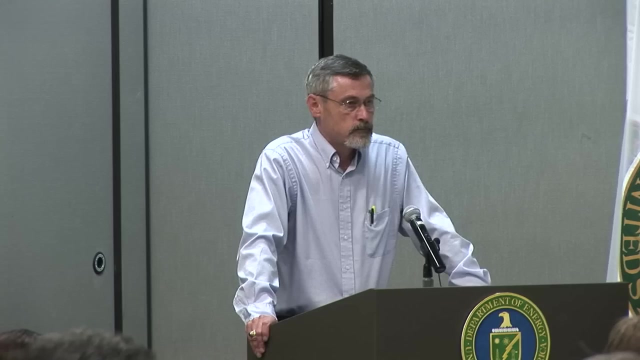 I don't think they are, And I think that may be some places where we really need to get the word out a bit more. It's either A or B. It really isn't an either-or, And your measure of success would be sustainability. you know the entire. 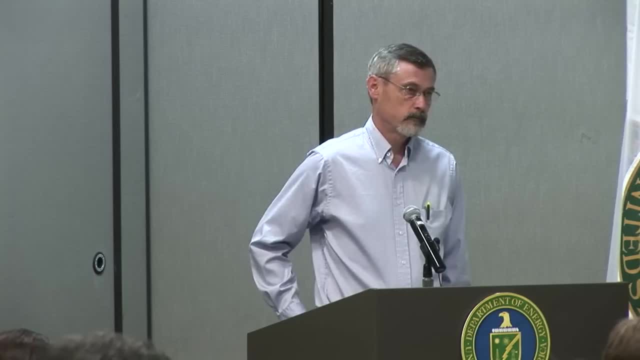 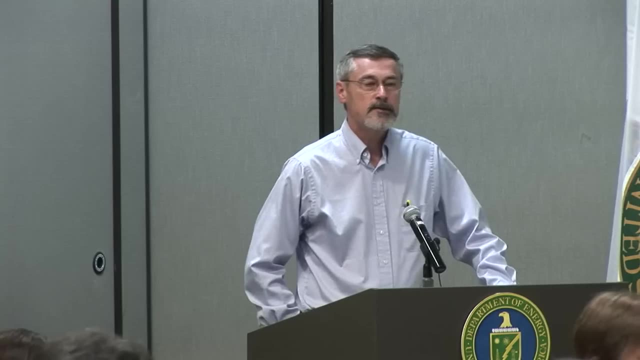 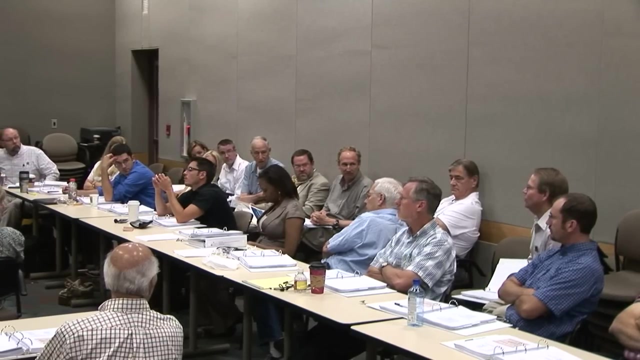 And sustainability, going beyond just resource sustainability, economic sustainability, environmental sustainability. Okay, Gordon, Do you have a comment? Just a comment that we have a lot of LWR fuel in storage. in general, You're not proposing to use electric chemical processes for all of that.